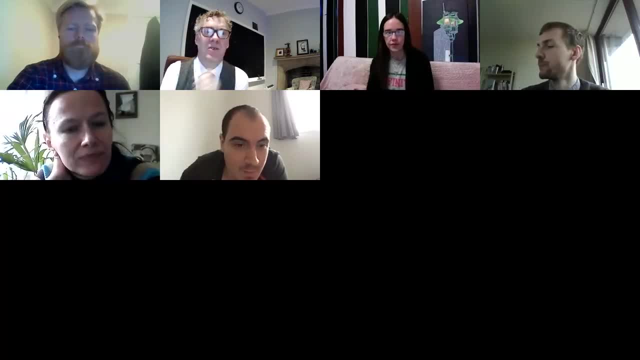 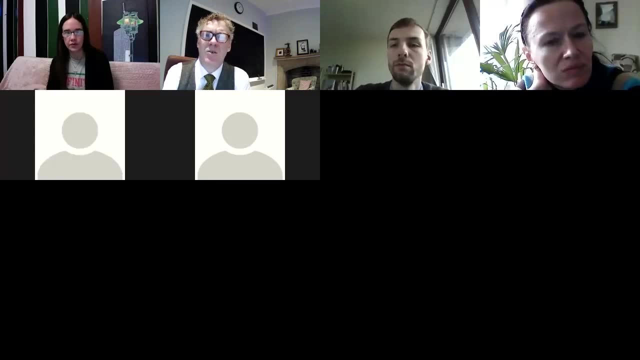 Cantor's ideas on cardinality and the ordinals and transfinite arithmetic as well as transfinite recursion, And one should really think of set theory as its own subject. It's a wellspring of mathematical thought, It's a sort of its own independent subject with its own questions and 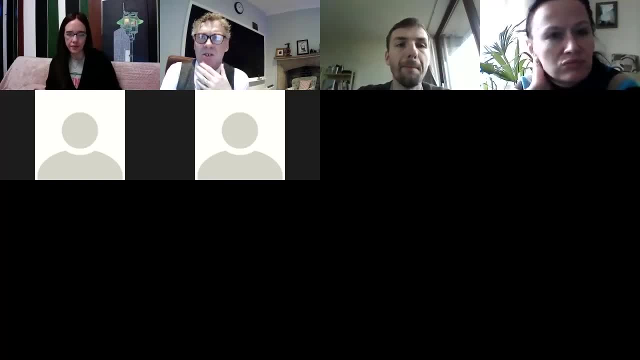 problems and methods. But also set theory provides a tools and conceptual framework for mathematicians in general to deal with arbitrary mathematical structures. So there's sort of two roles that set theory is playing. On the one hand it's its own subject with its own questions and answers. 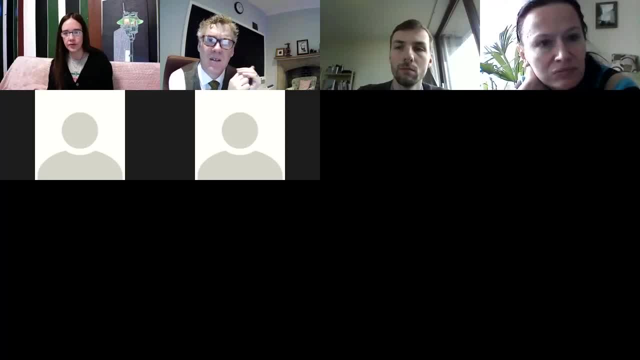 But on the other hand, it serves this role as a foundation of mathematics, as a kind of ontological foundation, a common forum in which one can view other mathematical constructions as taking place. Okay, and on both sides, really on both aspects of that duality, set theory is engaging. 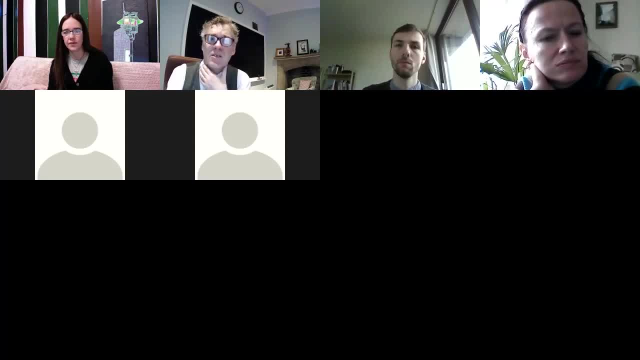 with explicitly and fundamentally philosophical issues. On the on its own side, of course, it's intimately concerned with the concept of infinity, which formerly was always considered as primarily a philosophical concept. But on the other hand it's a kind of ontological concept, And so it's 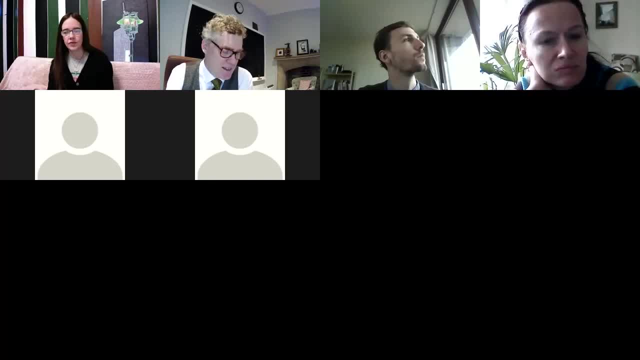 intimately concerned with the concept of infinity, which formerly was always considered as primarily a philosophical issue. And in fact that set theoretic view of infinity has been so successful that one can't seriously undertake any kind of philosophical discussion of infinity without explicitly engaging with the set theoretic conceptions. But on the other side, on the role, 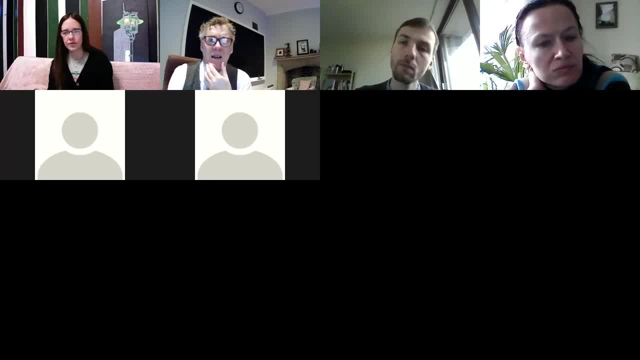 of set theory as a foundation of mathematics, it's even more explicitly engaged with philosophical issues. For example, what role do axioms play in the foundational theory, Or by what criteria are we to add or remove axioms from a foundational theory? And may we judge the truth of strong axioms by the fruitfulness of their consequences? 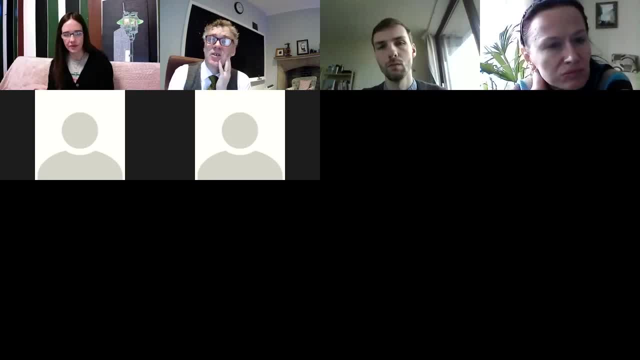 Are the axioms of set theory describing a unique intended set theoretic universe or is there a sort of multiverse of set theoretic conceptions? And is the set theoretic universe a completed totality or does it have ultimately a character of potentiality? Okay, so these are the kinds of 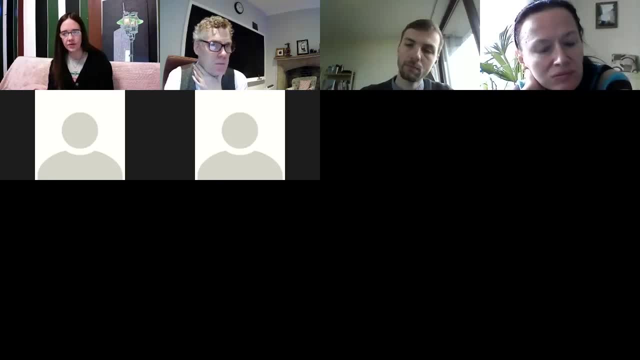 questions that one is maybe going to be engaged with. So I'm going to start with the set theoretic conceptions. So let's start, though, really by talking about a particular problem which saw the birth of many fundamental set theoretic ideas, and that's the Kander-Bendixson. 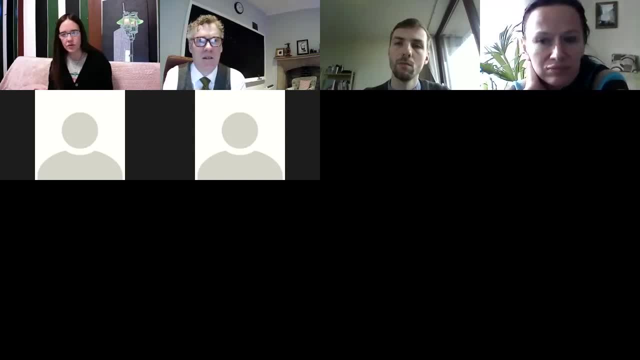 theorem. So this is the arising in Cantor's 1872 investigation of what's known now as the Kander-Bendixson process. So this is the process by which you iteratively cast out isolated points from a closed set of reals. So if you have a set of real numbers, or maybe it's a subset of the plane- 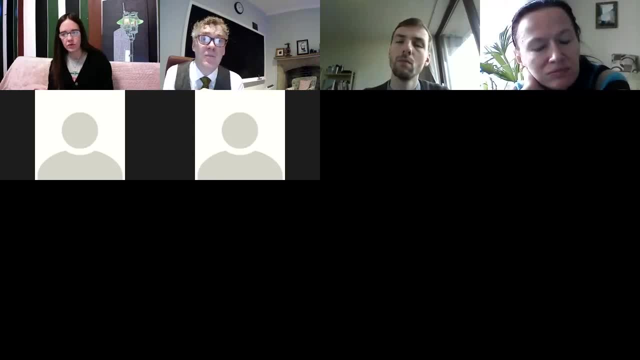 or in some finite dimension, it doesn't really matter. a point is isolated if it's an element of the set that stands alone in some small neighborhood, So you can put a in an open neighborhood around it, so that that point is the only point in that set And the process. 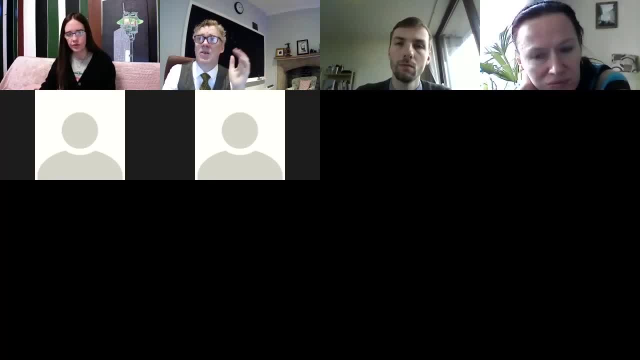 of building the derived set is the process of casting out all the isolated points from your initial closed set. So let me just illustrate with an example. So I have here a closed set of reals that I've drawn on the board. You can see there's two red points here and each of those red 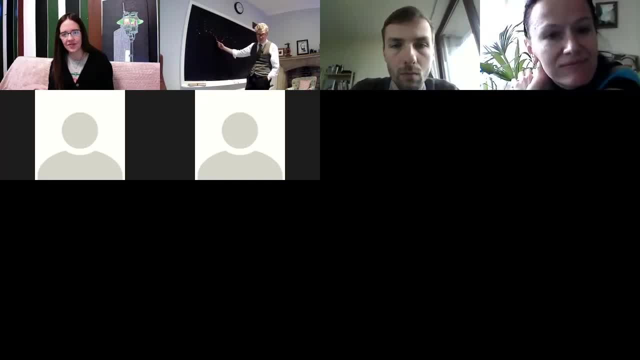 points is a limit of these white points. So there's a sequence converging to this red point and another sequence on this side converging to that red point. But each of these white points is itself the limit of a convergent blue sequence of dots converging, So the red points are not. 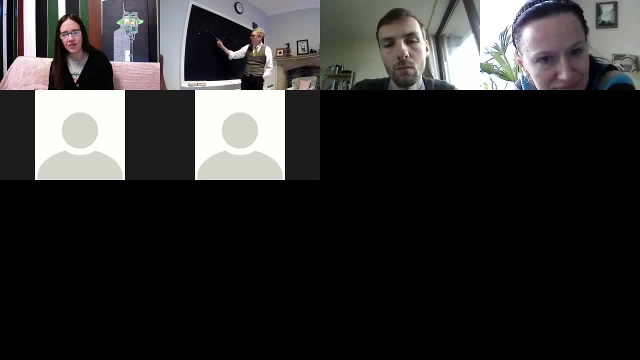 isolated because they're a limit of the white points and the white points are not isolated because they're the limit of the blue points, But the blue points are isolated. so around each individual blue point I can put a little open neighborhood so that that blue point is the only point in the neighborhood. So if I started with 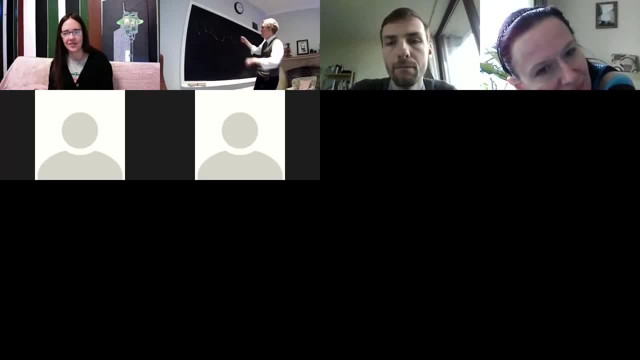 this set, which is a closed set, and I cast out isolated points. at the first step, I would be throwing away all the blue points and then I would have just these white points and the red ones, And then I could do it again, because the white points were not initially isolated. 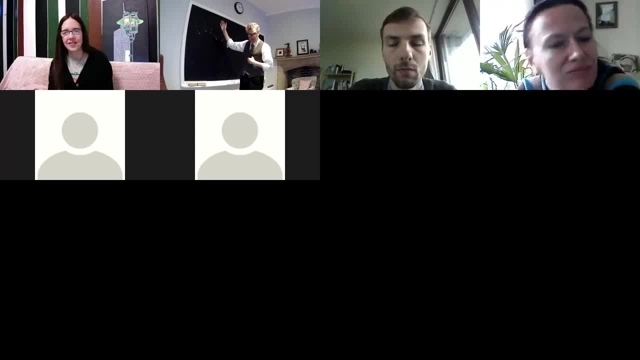 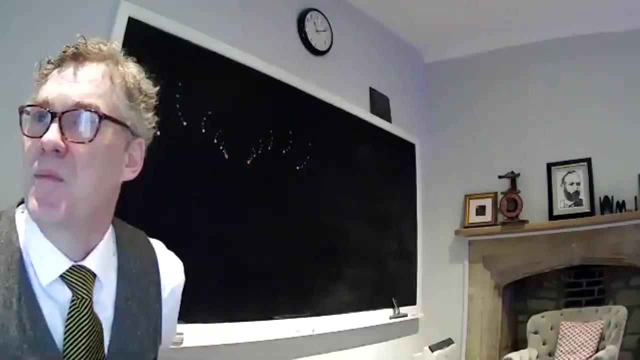 but they become isolated after I throw away the blue points. So, on the second step, I would be now casting out all of the all of the white points. You know what I have to change my view here? I'm recording but I'm not in the speaker view. Okay, so that's going to be a little better, Okay. 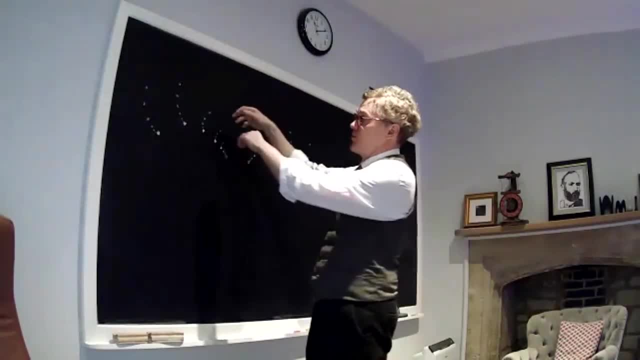 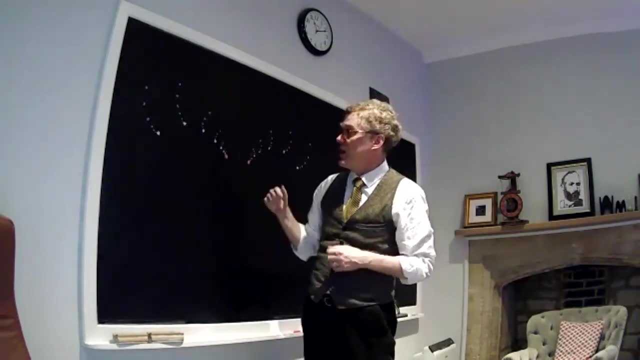 so at the next step, on the first step, I throw out, I cast away the blue points, and then now the white points become isolated, and then I throw away the blue points, and then I cast away the red points, And so on the next step, I would cast away the white points, and then all that I would have 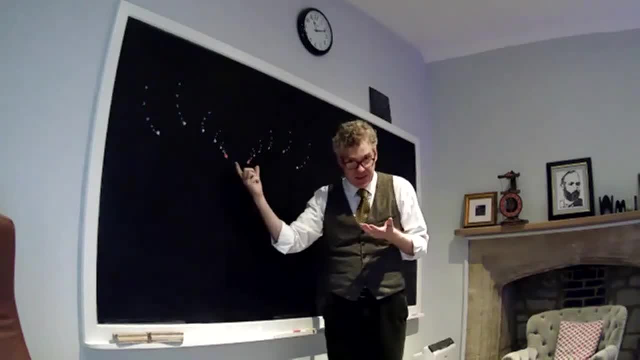 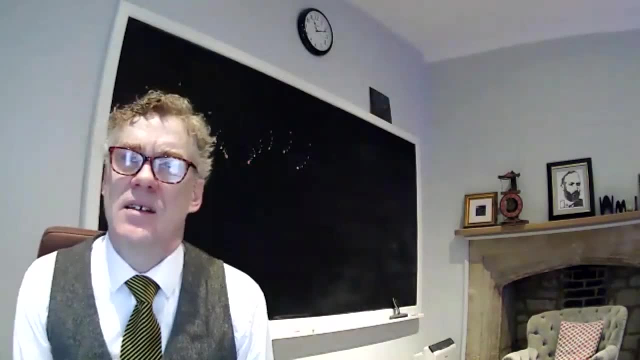 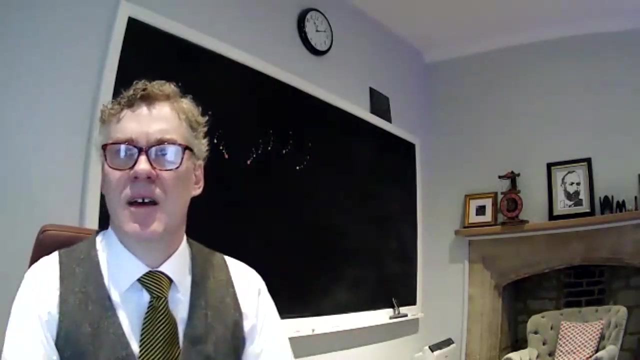 left are these two red points, and they would then become isolated and I would cast them out on the step after that. So the point is that once you cast out the isolated points, then you you might have more isolated points after this, And if you just iteratively cast out, 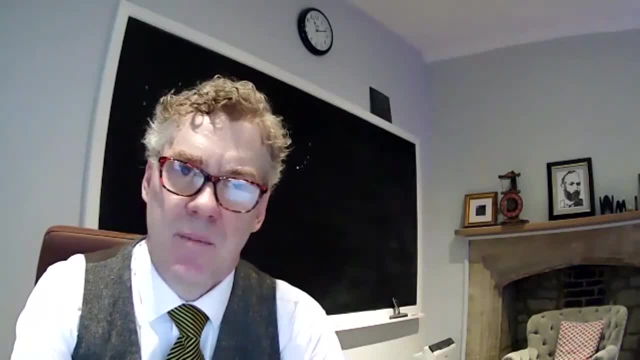 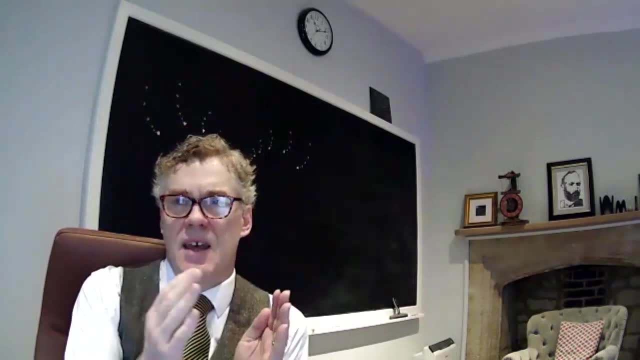 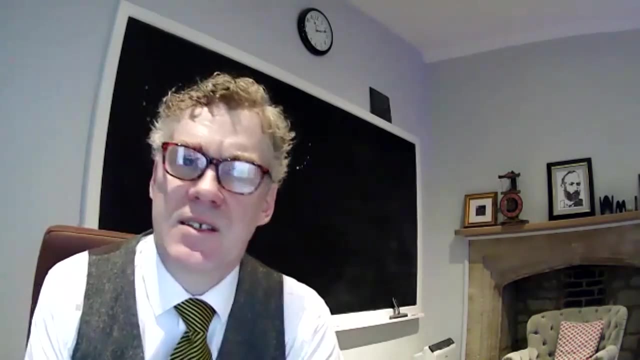 isolated points. this is called the Kander-Bendixson process. So the rank of the set is the number of steps it takes before it stabilizes. Maybe eventually we get to a set that has no isolated points. That's called a perfect set. A perfect set is a closed set. 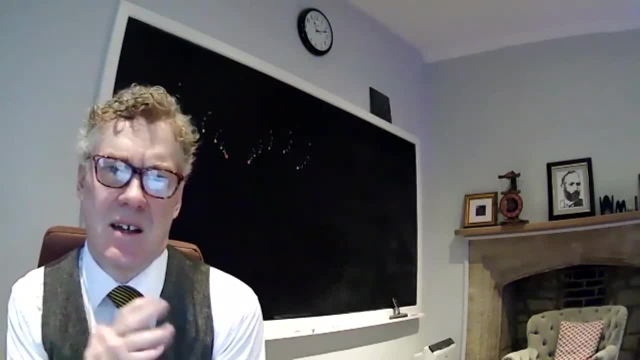 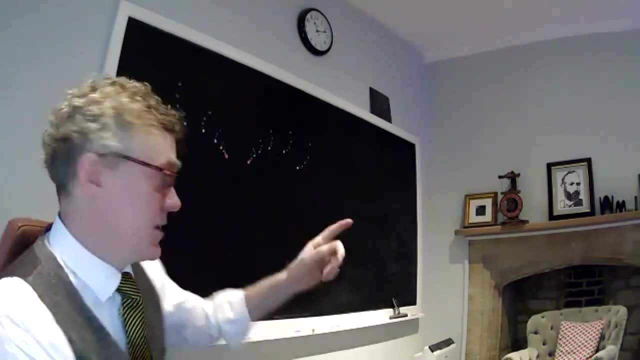 with no isolated points. Now you can easily construct, say, points that have rank seven, that take seven steps before it stabilizes. This one stabilized in three steps. First we threw out the blue, and then the white, and then the red, and then we didn't have anything left. so it's stable at. 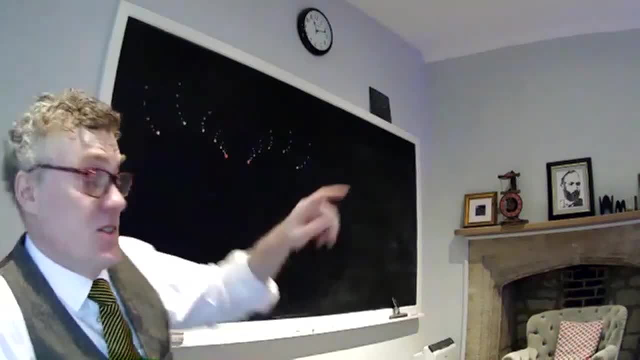 that point. But you can. by iterating you can get to a set that has no isolated points and then the. by iterating this we could have had yellow sequences converging to the blue points, or something. we could have made the rank one higher, and we can keep doing that. So you could probably 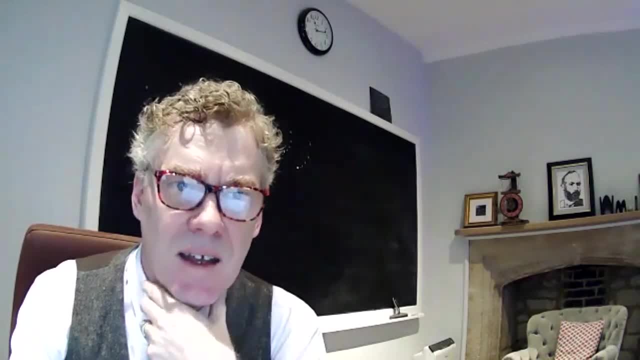 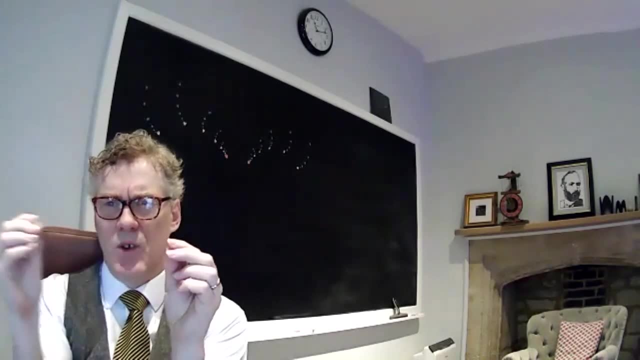 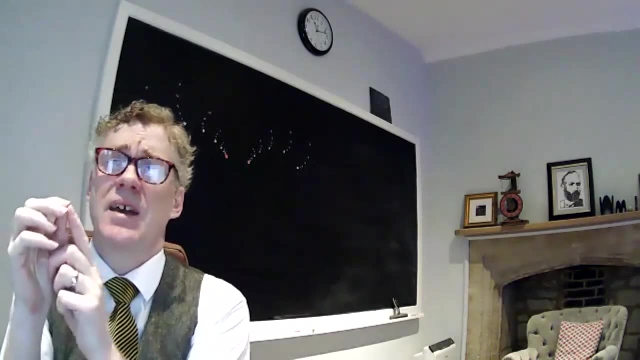 make sets of rank n for any finite n, And what Kander realized was that actually sets can have infinite rank, because you could imagine a sequence converging, say x0, x1, x2, x3 and so on, converging to a limit point and maybe xn has rank n. Okay, so it takes n steps before you get. 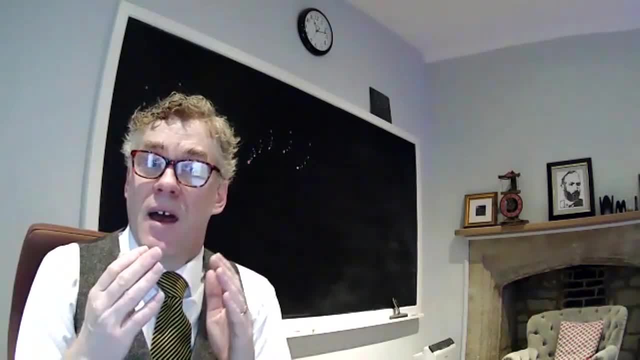 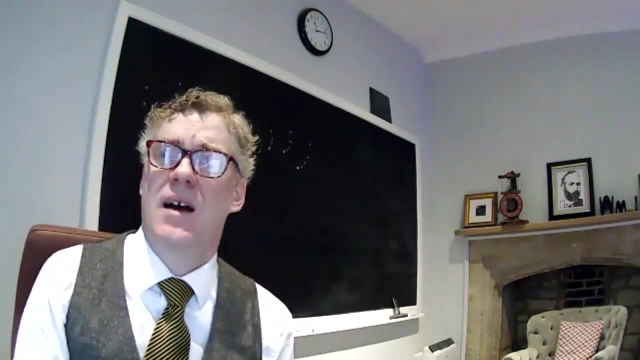 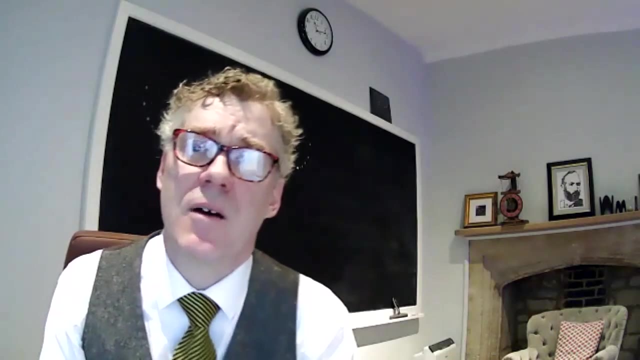 rid of xn, x, of n, And so the final limit point will not be cast out by any finite stage, but it will become isolated. It can become isolated at that after all those finite stages, at stage omega, what we would call omega now. And so Kander realized that it's quite strange and bizarre that 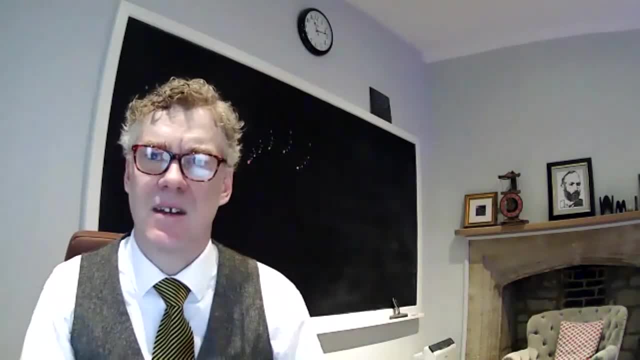 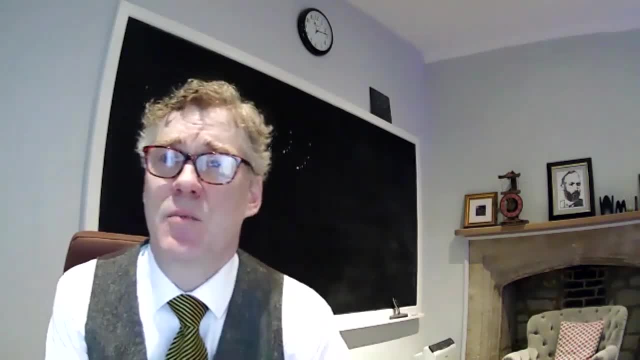 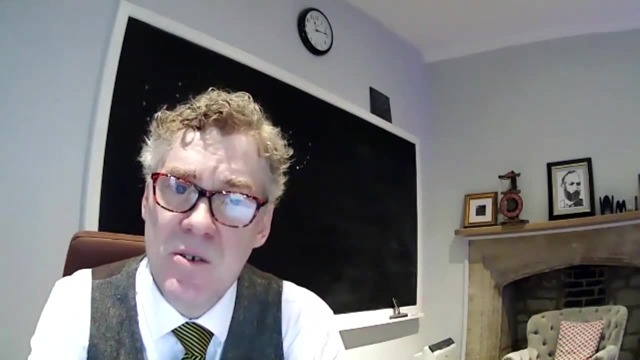 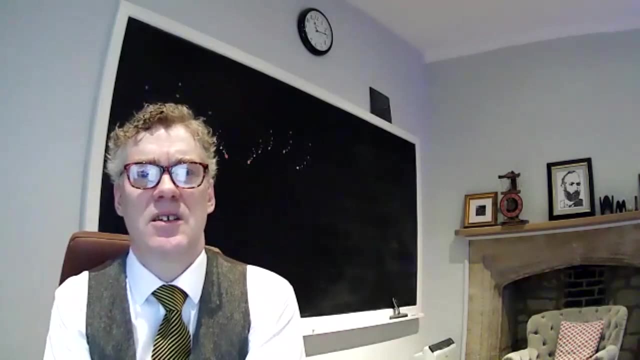 infinitely many times we're not done. We can still have isolated points after that, and you can keep going more steps after infinity, So from omega to omega plus one, or omega plus two, And so the process is inherently transfinite. And so Kander realized that, in order to describe the construction, 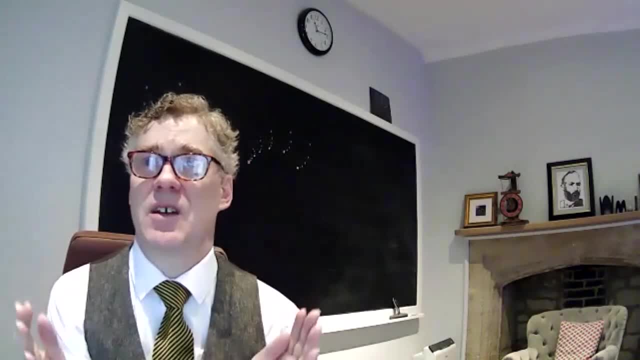 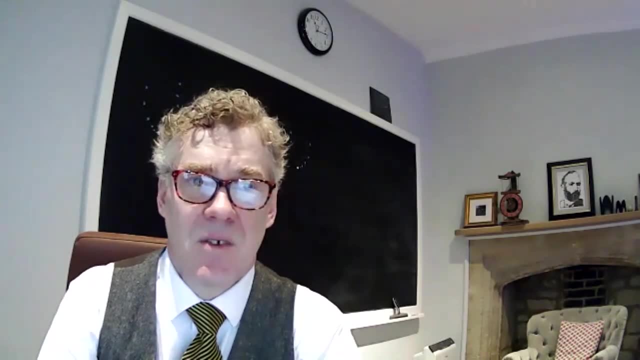 even. he needed a way to talk independently about the stages of the construction. What are these stages of construction by which we're iterating the Kander-Bendixson derivative? And in this way he came to the ordinals, because really the ordinals are providing exactly what. 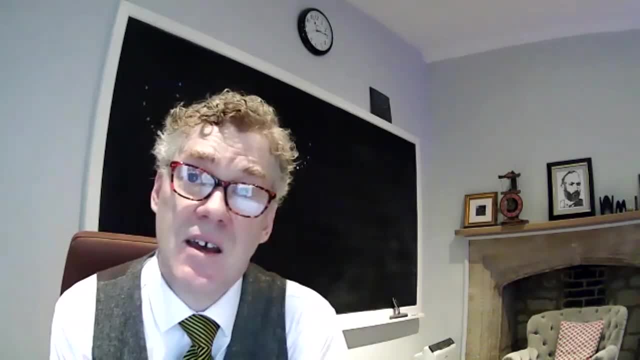 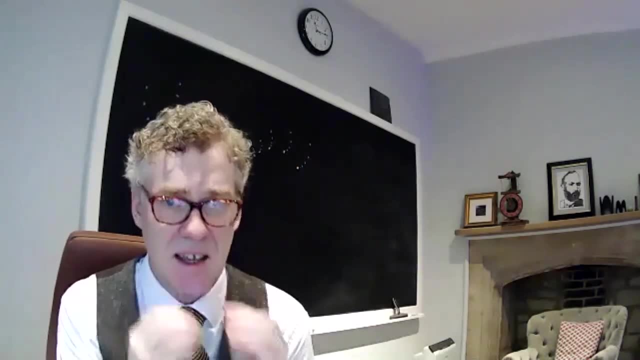 you want, in order to iterate transfinitely a process. So he came to the concept of well, orders and ordinals and transfinite recursion, and all of these ideas are at the very center of set theory today and they're all present, really, in the Kander-Bendixson theorem. So we 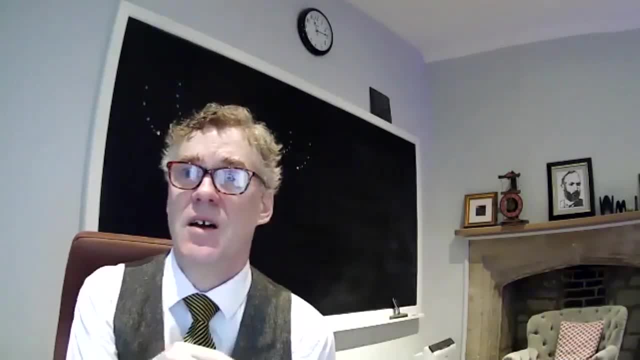 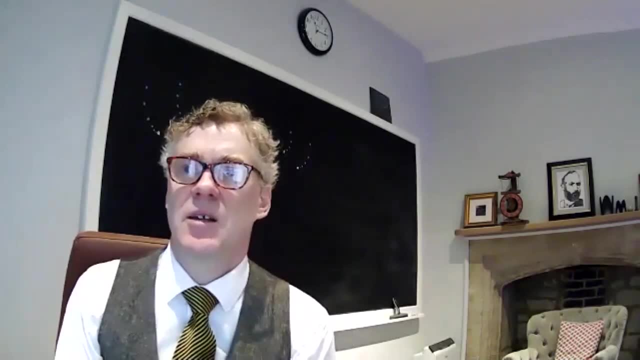 define a transfinite sequence of closed sets c sub alpha and the next set c sub alpha plus one. For any ordinal alpha is the obtained by casting out the isolated points of c? alpha, and at limit stages you just keep whatever you haven't cast out yet. So it's the intersection of the sets that 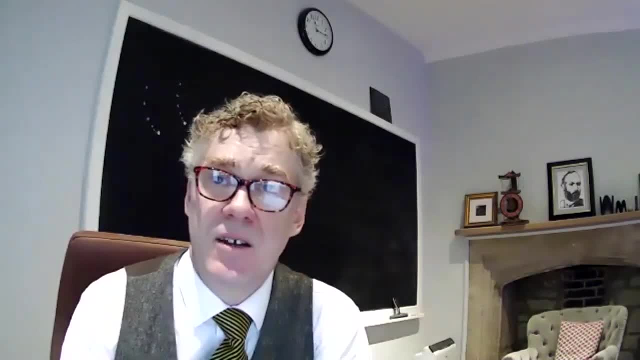 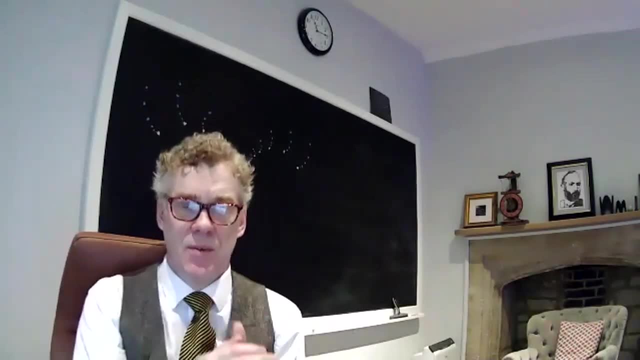 you've built so far, and this is a transfinite definition of the Kander-Bendixson process, The theorem. the Kander-Bendixson theorem is the claim that for any closed set of real numbers- and in fact, it doesn't matter if you're in some finite dimension or even countable dimension. 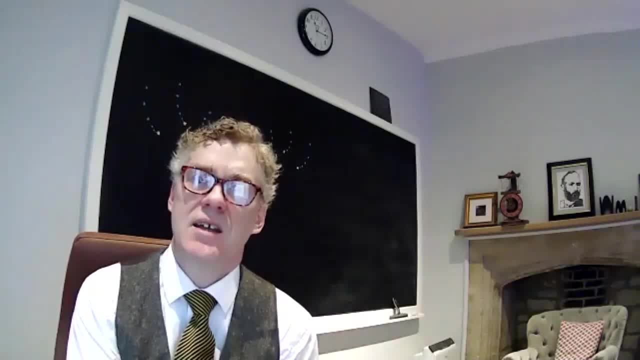 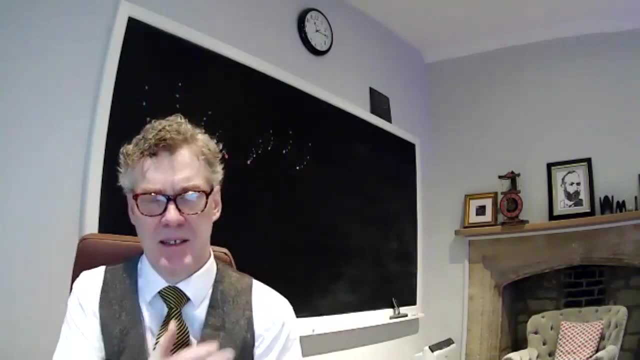 for any closed set, there's some countable, some countable ordinal stage by which the process stabilizes. I don't mean that it stabilizes at omega, I mean it stabilizes at some countable ordinal stage. and the way you can prove that is: 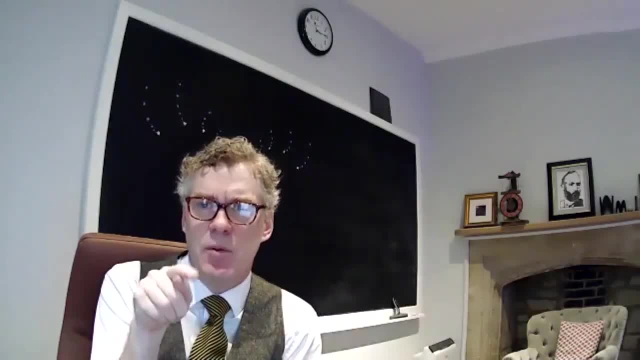 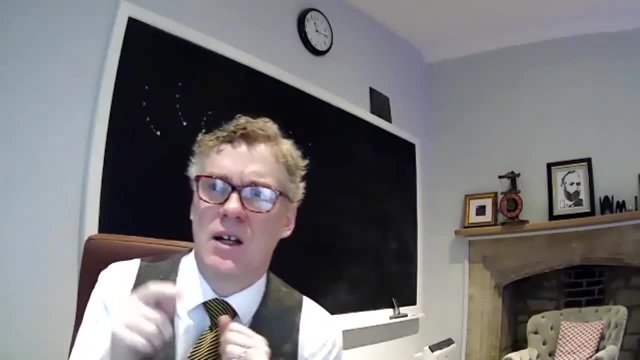 every time you cast out a point it was because you had a little neighborhood of that point in which that point was the only one. and we can put a little rational neighborhood, say a little rational interval or a rational ball in the higher dimension, with a rational center and rational radius. 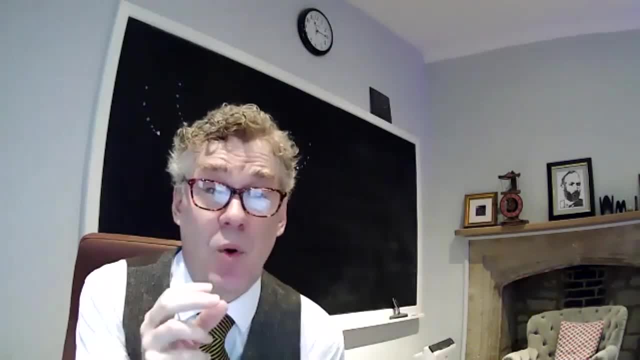 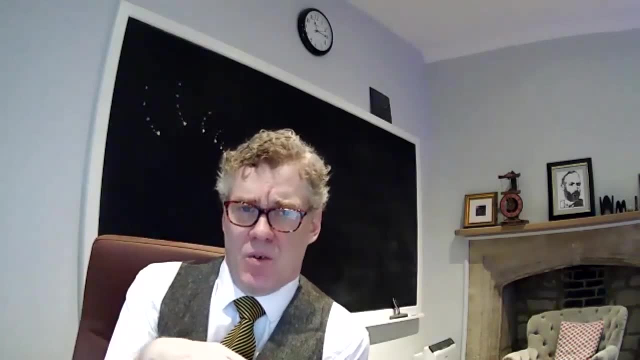 So that that that ball is the reason why that point was isolated, or a reason why we can see that point was isolated. and the point is that every point that's ever cast out will will be determined by the ball that we associated with it. We're never going to. 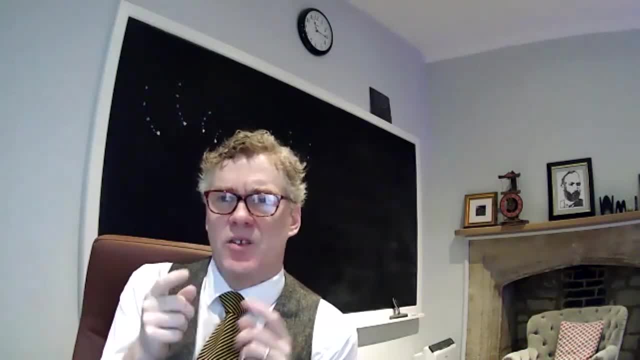 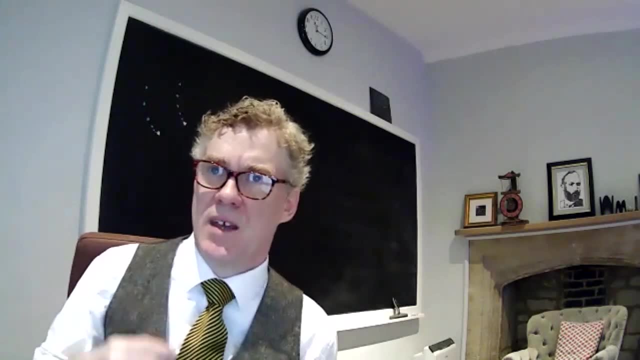 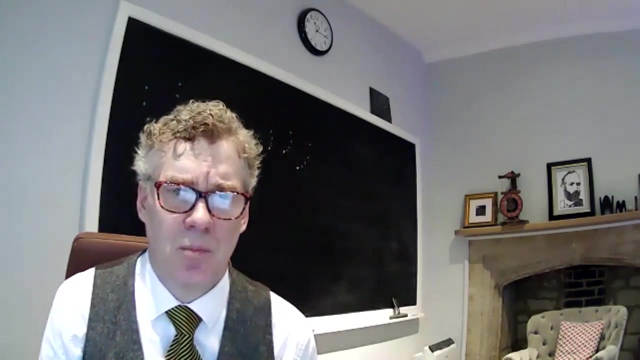 associate that ball with another point, because at all the earlier stages there was more than one point in that ball and at all the later stages there wasn't any point in that ball, precisely because we cast it out. So therefore we can associate every cast out isolated point with a rational interval. 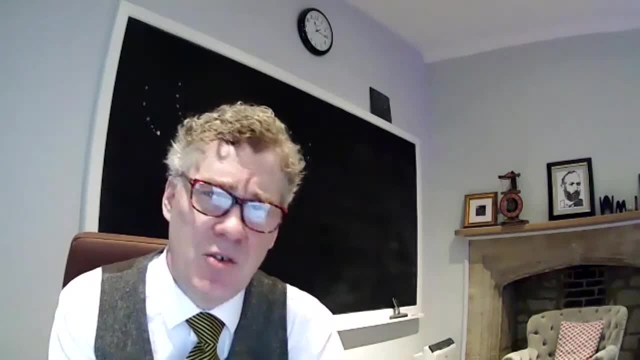 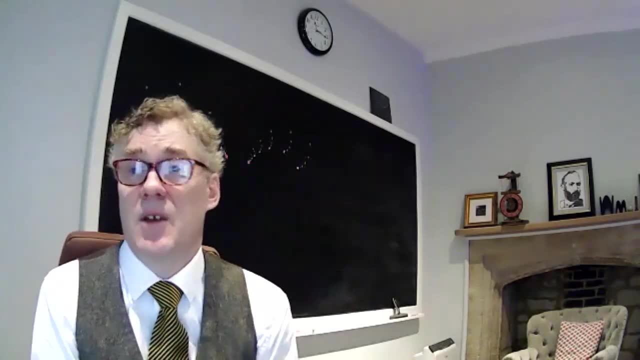 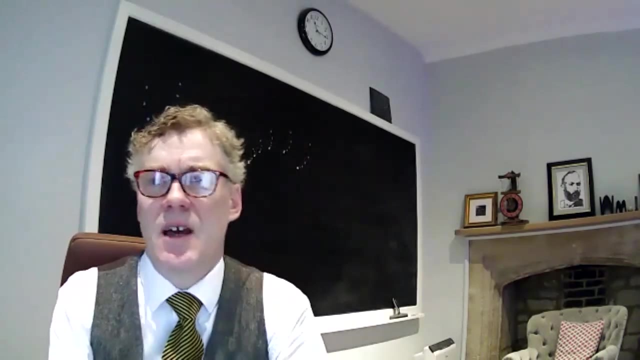 but there's only countably many rational intervals. So therefore there are only countably many points that will ever toss out And therefore that will happen at some countable stage. So it follows that every closed set of real numbers is the union of a countable set. 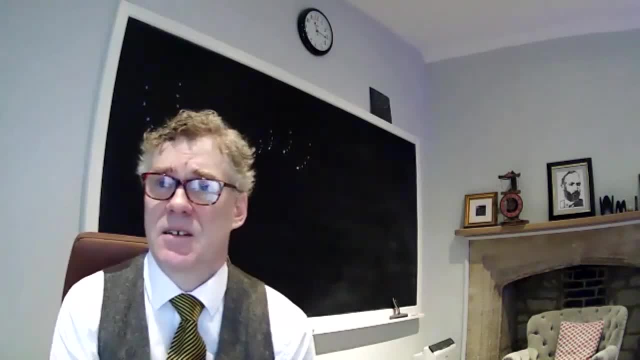 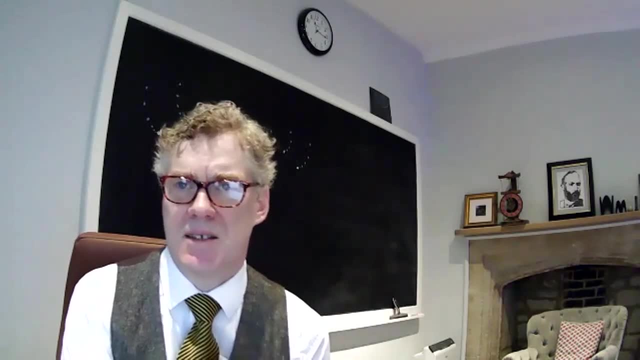 the ones that are cast out- and a perfect set, which is a set with no isolated points- Maybe it's empty. And Cantor made a remarkable conclusion based on this, because he had already proved that every perfect set, every non-empty perfect set of real numbers. 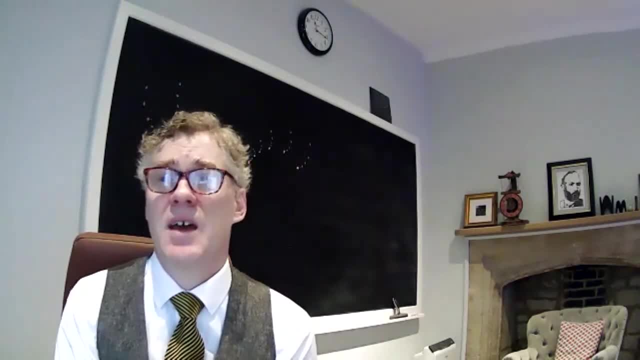 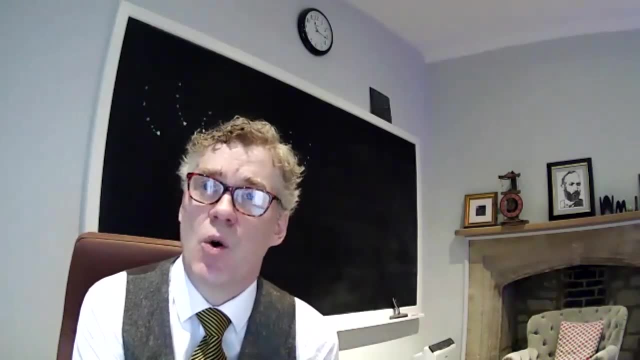 is equinumerous with the whole set of real numbers. So it follows, therefore, that every closed set is either countable or else is equinumerous with the whole set of real numbers. And this is a sort of a proto version of the continuum hypothesis. 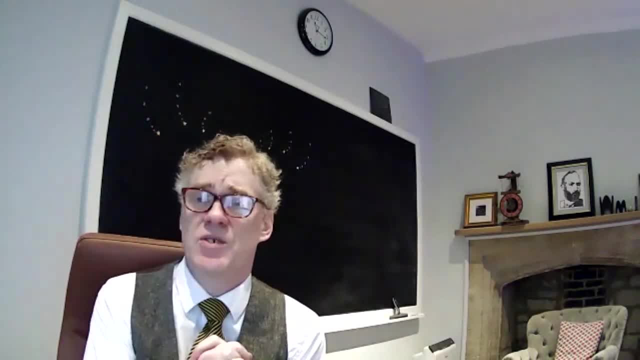 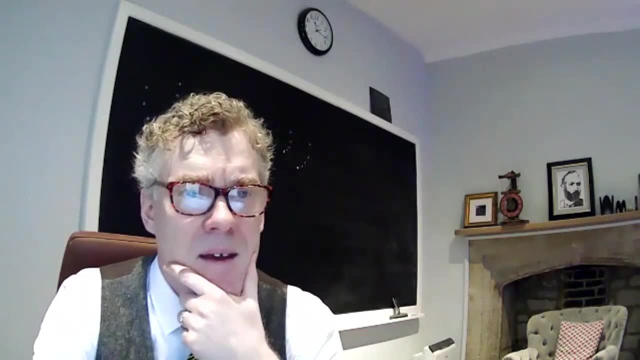 namely Cantor's, proving the continuum hypothesis holds for closed sets. It's a theorem. for closed sets, Every closed set is either countable or else equinumerous with the whole real line. Okay, so let's move on now to the view of set theory. 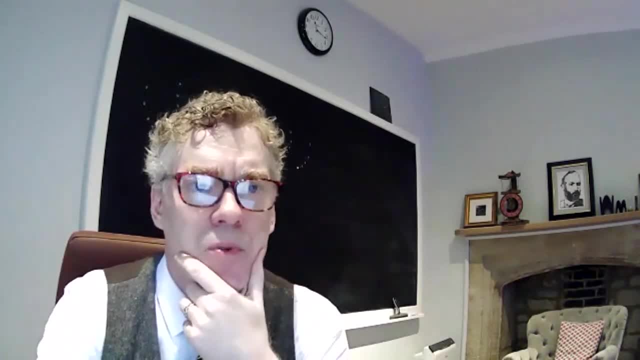 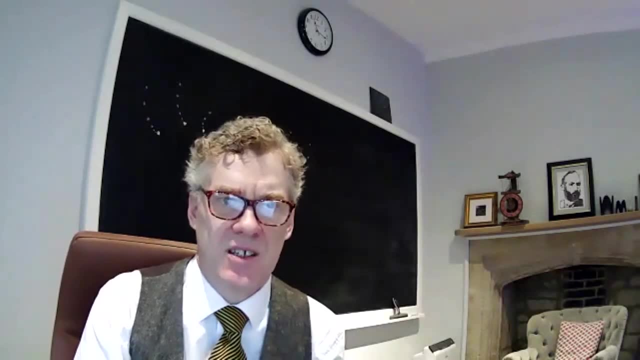 as a foundation of mathematics, this sort of other prong, other role that set theory plays. I mean, at first, of course, set theory was just used as a tool, brought into other subjects, but eventually the capacity of set theory to express arbitrary mathematical structure was realized. 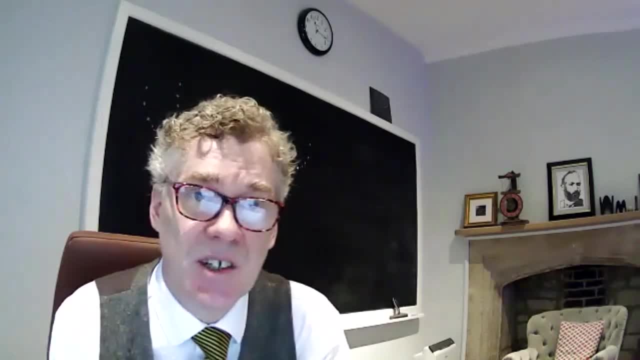 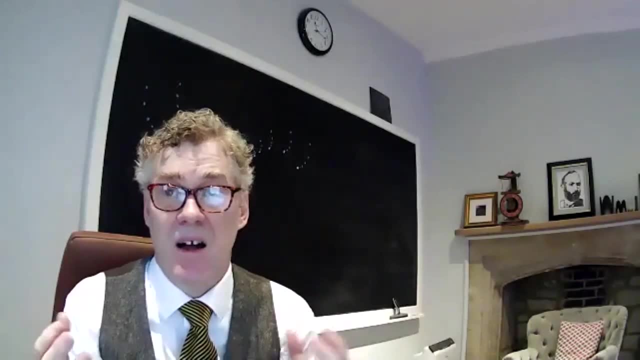 And mathematicians began to look on it as a kind of foundation or unifying role. So Penelope Maddy described set theory as providing a metamathematical corral. It's a sort of arena inside of which one can introduce arbitrary mathematical structures. 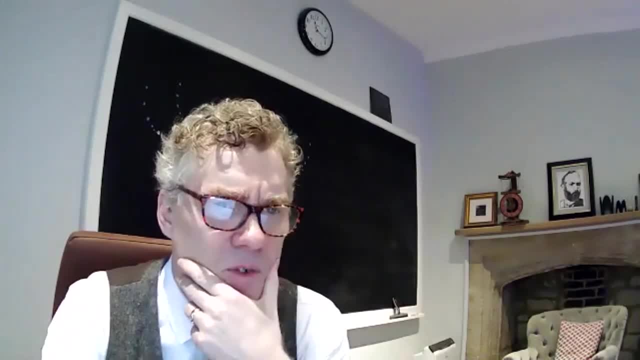 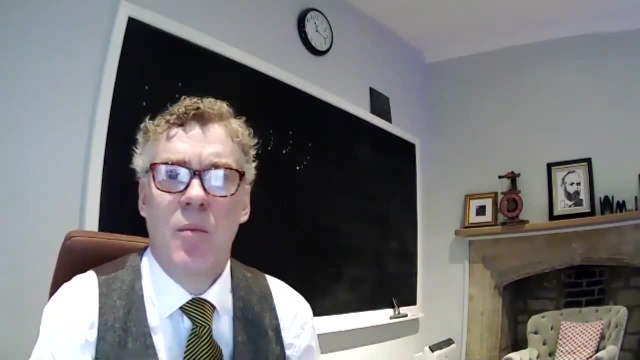 and undertake analysis there For the birth of set theory. she points to Karl von Stout's early resolution of the use of virtual objects, So points at infinity. it was mysterious, What are these points at infinity that people that people talk about in geometry? 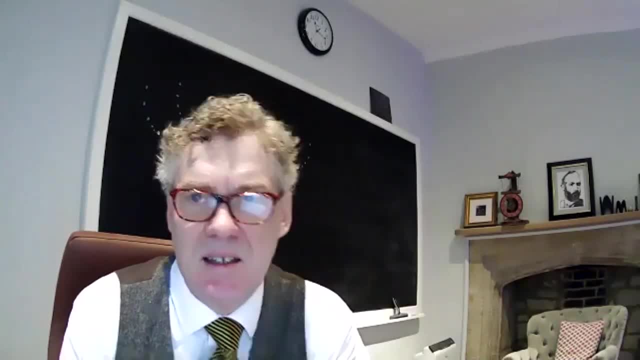 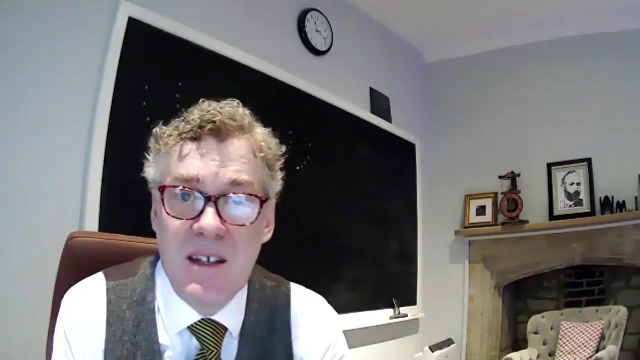 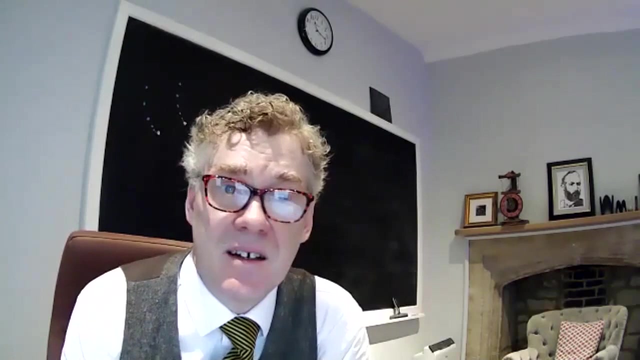 And he built them, And the way that he built them was: he defined the geometry. to take the point at infinity, identify the point where two horizontal lines meet, as what we'd see now is the set of lines parallel to those lines, the equivalence class of the parallel lines. 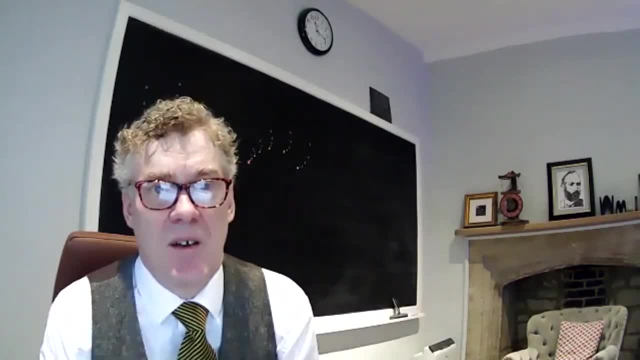 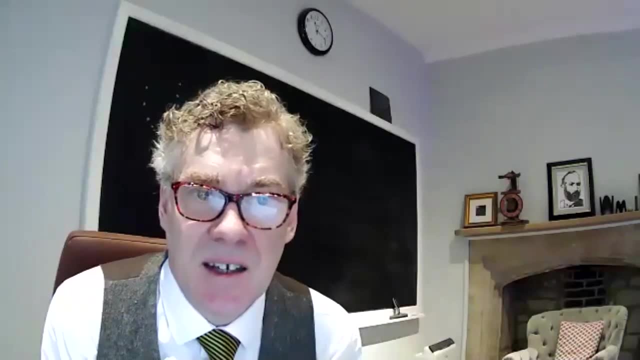 So she says, in this way von Stout managed to build surrogates for the heretofore suspicious, possibly dangerous new items like points at infinity. And as time went by, it became clear that the construction tools needed for this building process were actually set theoretic in character. 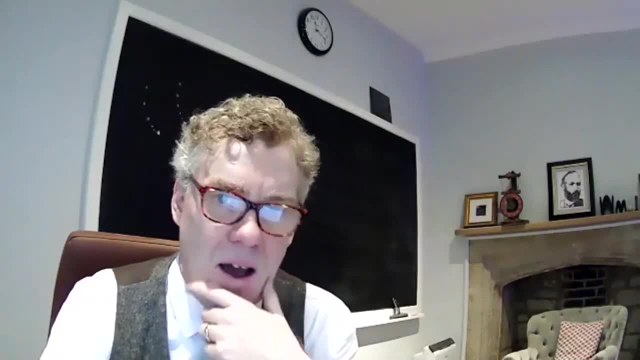 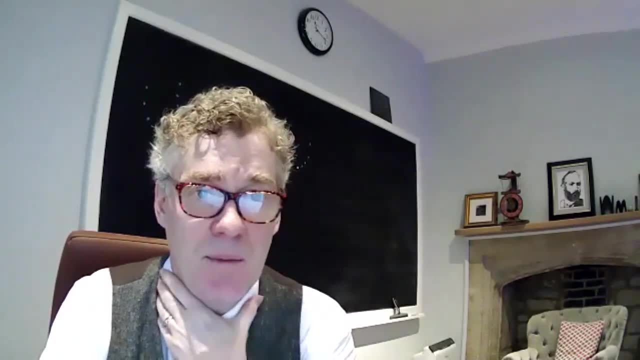 So a little bit later Hilbert had said- I mean after- the role of set theory in providing this sort of framework for mathematical analysis and understanding. Hilbert famously said: "'No one shall cast us from the paradise that Kander has created for us'". 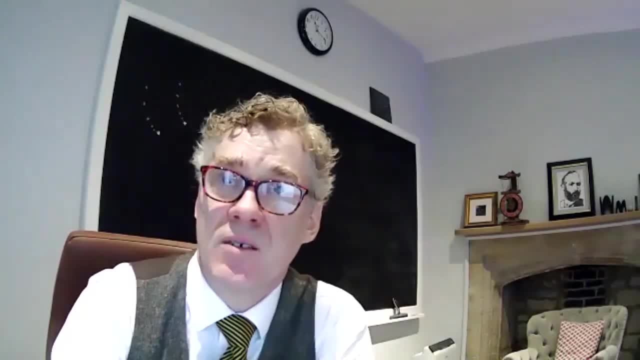 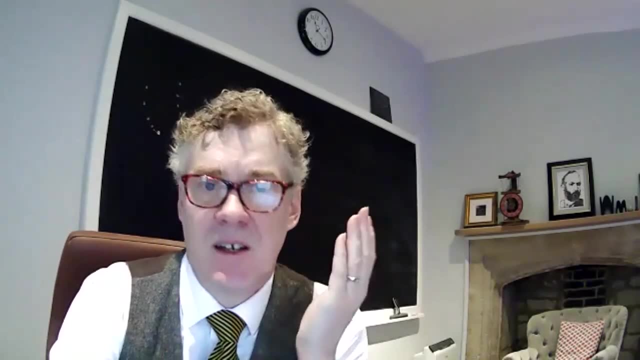 So he thought those tools were so fundamental and important that we will never give them up. Of course, in the 20th century, to become precise in mathematics often came to mean to specify one's mathematical structure in a set theoretic fashion. What is an order? 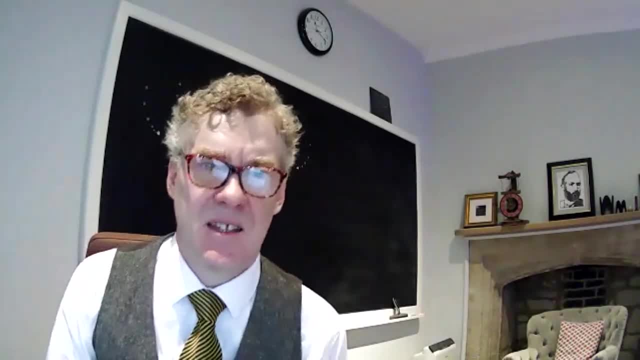 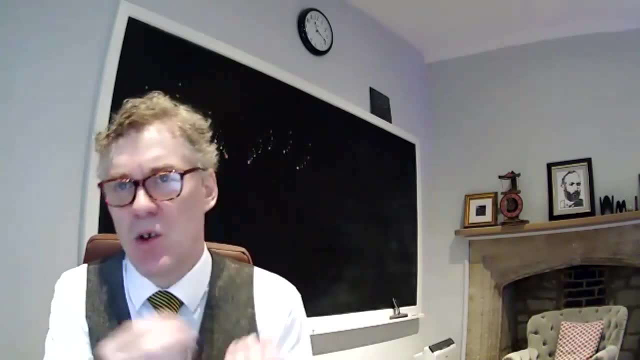 Well, an order, it's a set with a binary relation on that set. that's reflexive and transitive and anti-symmetric. Well, what is a binary relation on a set? Well, it's a set of ordered pairs from the set. 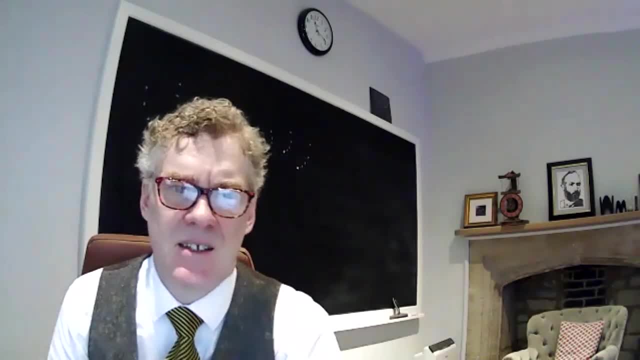 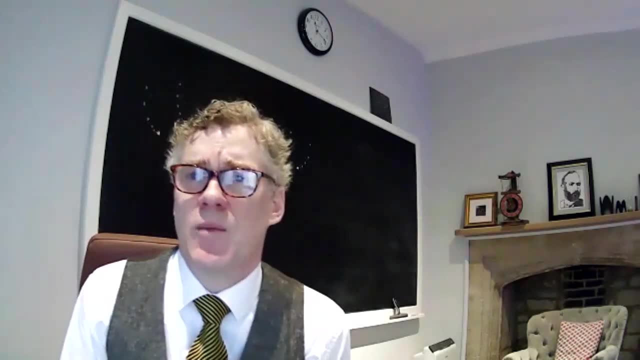 or what is a group? Well, it's a set with a binary operation that has certain features, it's associative and it has an identity element, an inverse element, and so on. So if someone presses you, what is your mathematical structure? 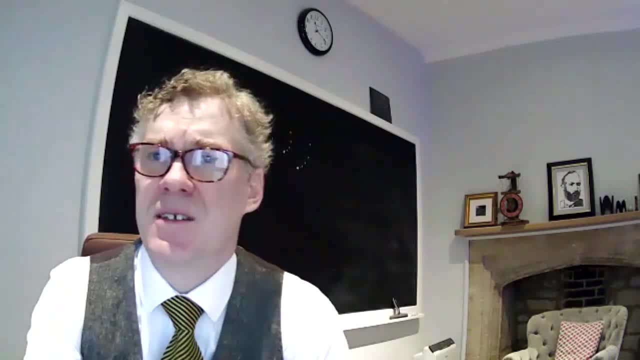 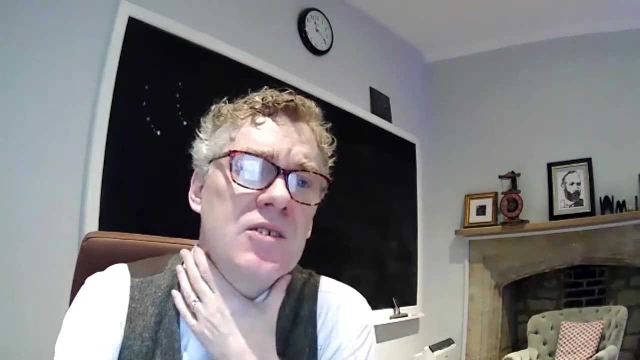 Then oftentimes the answer was that it's a set of a certain kind, or a set with some other sets that are associated with it, And so the answers were given in set theoretic terms. So Moscavacus describes the process of faithful representation that occurs in mathematics. 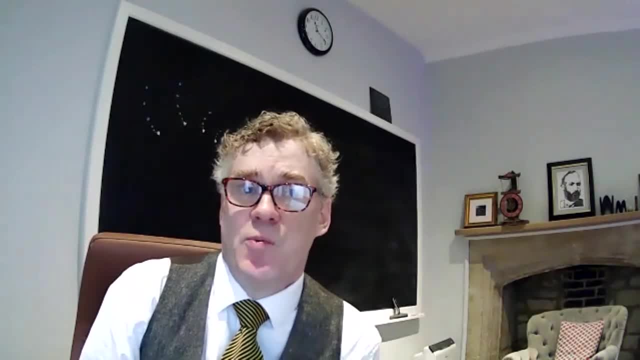 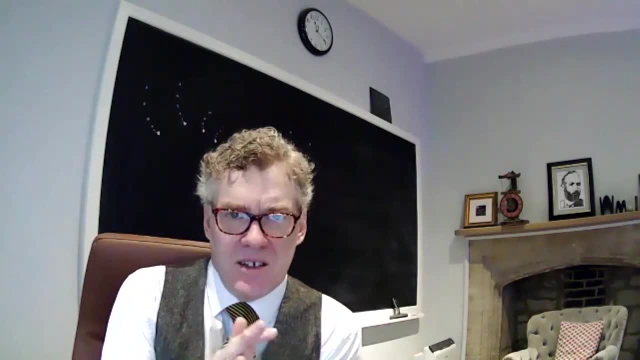 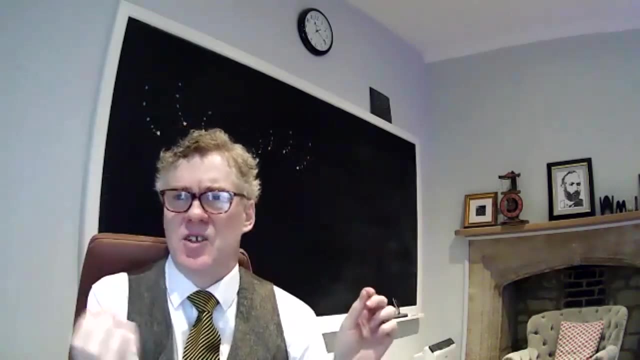 when we use one kind of mathematical structure or conceptual framework to represent mathematical objects that arise naturally in another. And you can view sort of Cartesian geometry really as an instance of this. We previously we think about geometry and collections of points and so on, and Descartes realized: look. 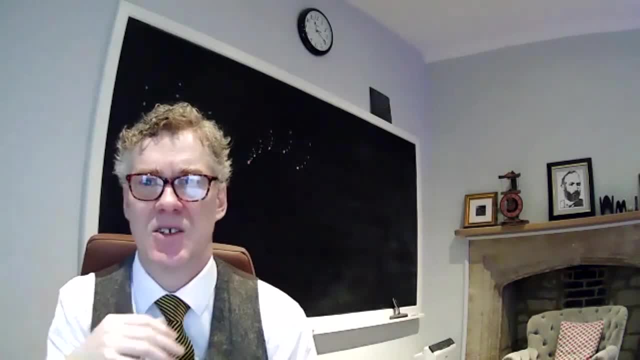 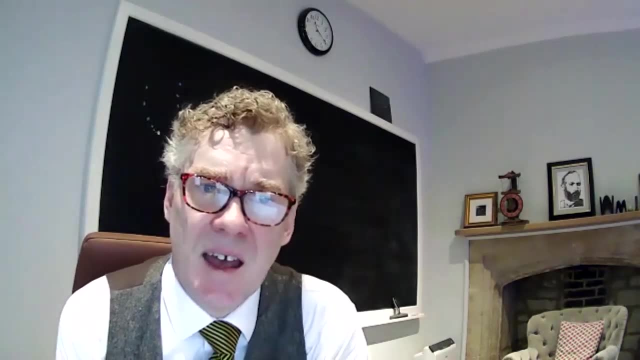 we can identify the point by its coordinates, So we can sort of faithfully represent points with pairs of real numbers or triples of real numbers in three dimensions. And so today we typically identify a point in the plane with its coordinates X, comma, Y. Yeah, there's a point in the plane. 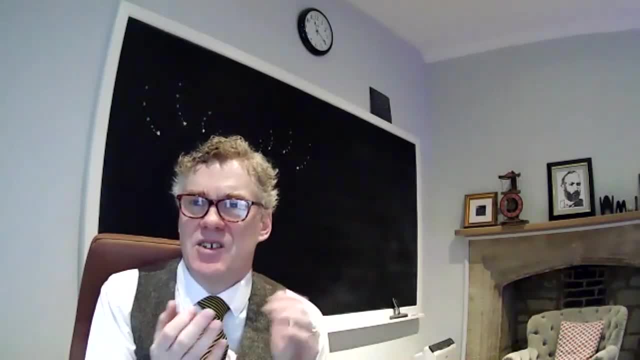 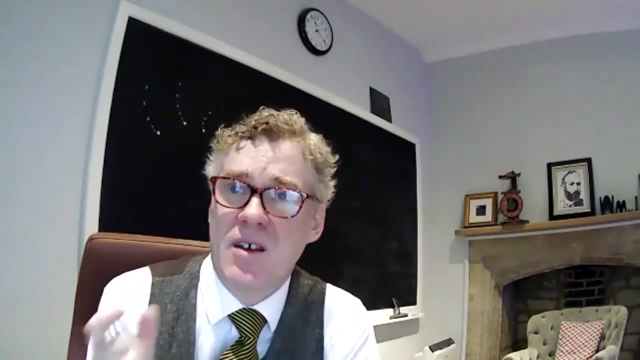 But of course, historically there wasn't any such, I think, identification and really what's going on? is this a faithful representation? We don't have to insist that points are the pairs of real numbers, but we can fruitfully analyze them as if they were. 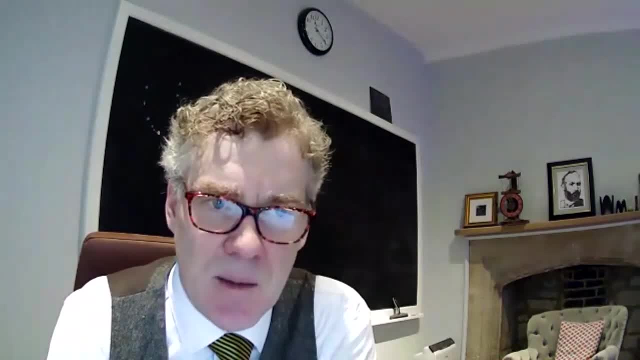 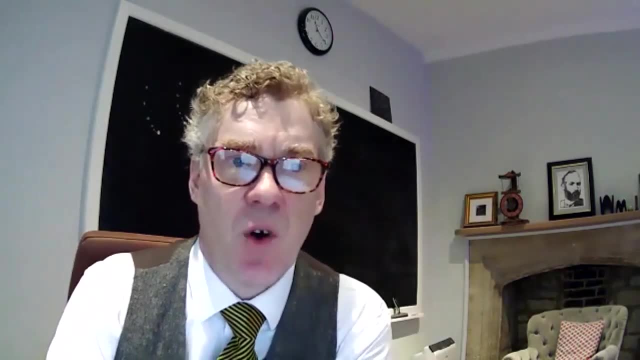 This is faithful representation. So he says specifically about set theory. this is Moscavacus. we will discover within the universe of sets faithful representations of all the mathematical objects we need, And we will study set theory on the basis of the lean axiomatic system of Zermelo. 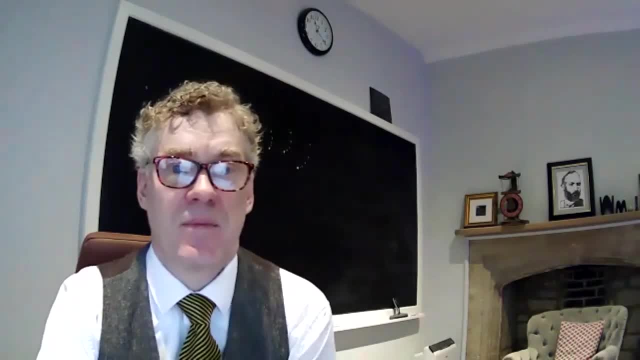 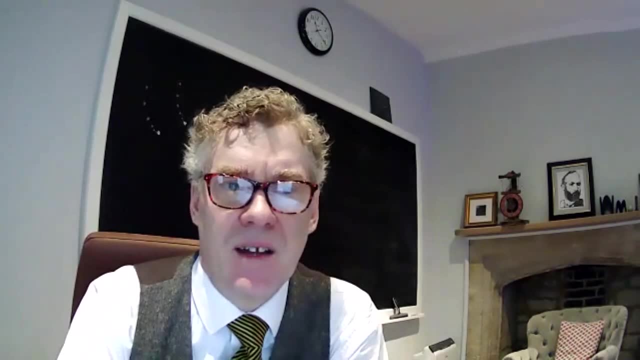 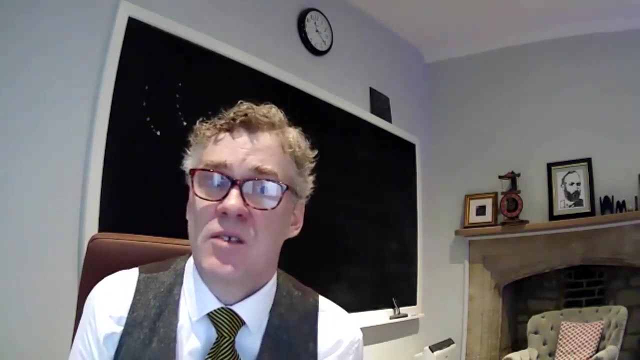 as if all mathematical objects were sets. Okay, now, of course, one can take set theory merely as one of many possible foundations in mathematics. So there's other possible foundations that you might seek out, for example category theoretic foundations or univalent foundations. 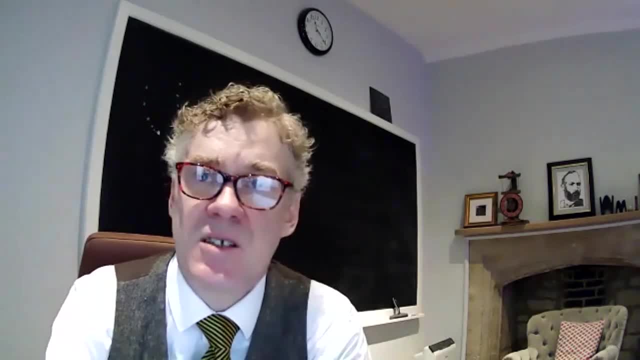 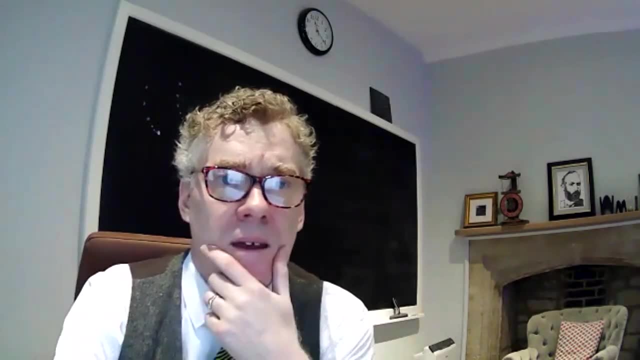 in homotopy type theory and so on. Set theory is just one of these possible foundations, but historically, in the most of the 20th century it was the main and perhaps the only one for a long time: The rise of set theory. 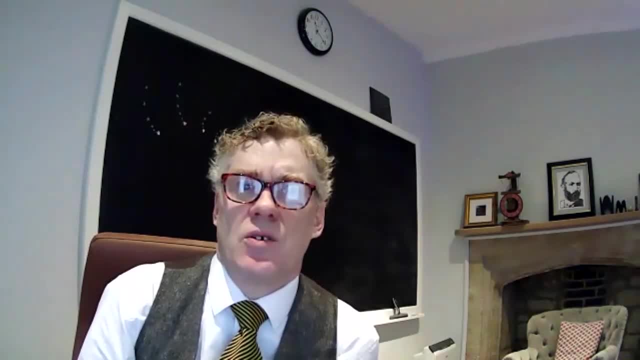 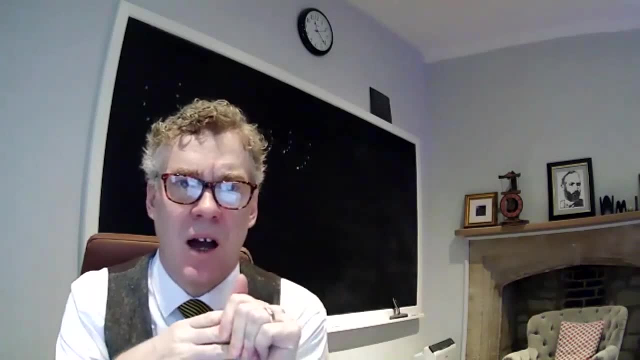 as a unifying mathematical foundation was an important historical development, because it's very common in mathematics to seek to apply results from one area of mathematics in another. Maybe you wanna apply results and theorems from topology in order to prove results in algebra, or something like that. 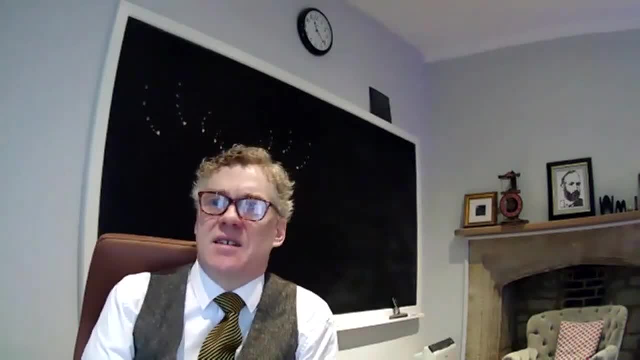 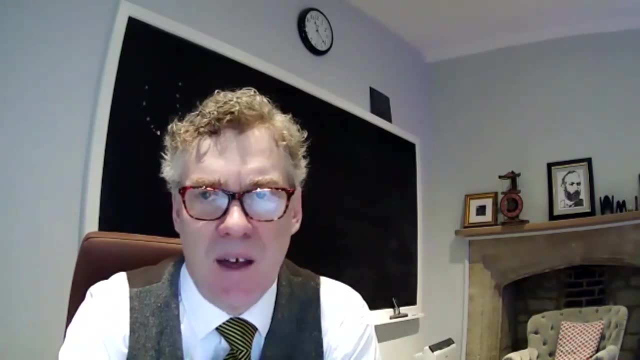 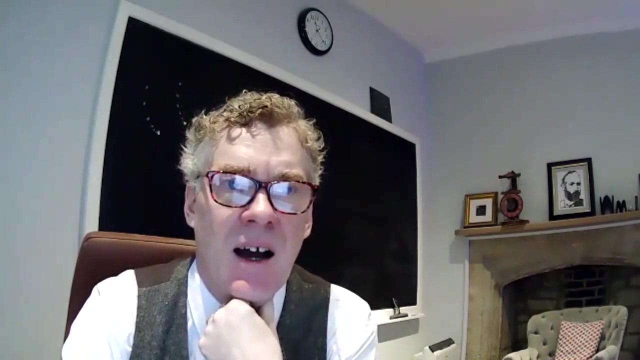 And that practice would be logically incoherent, right Unless both subjects were viewed as taking place in a single form or a single mathematical framework. So one can easily imagine a balkanized mathematics where math is divided into separate realms, each with its own fundamental axioms with it. 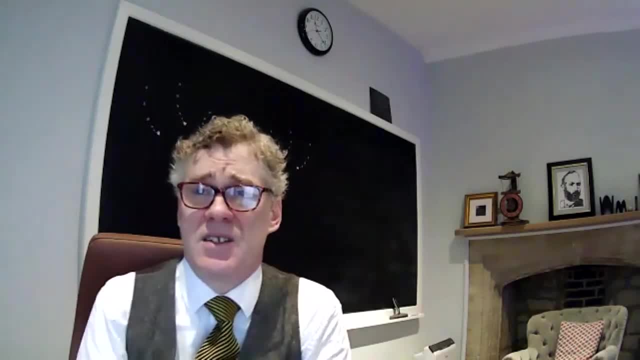 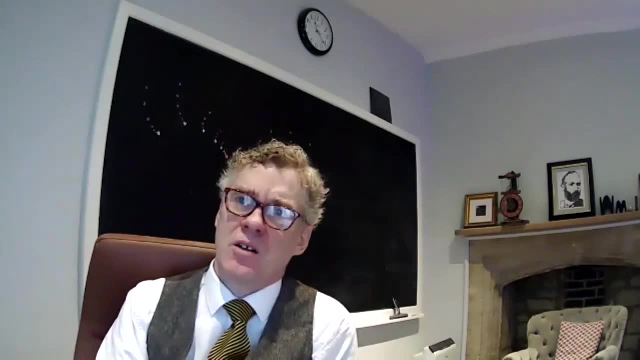 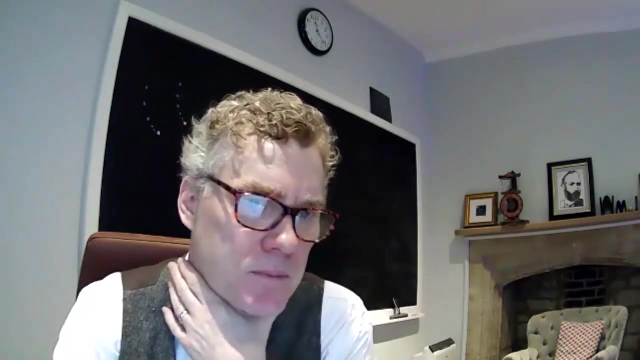 but without any common underlying theory. I mean, it wouldn't seem unreasonable to have imagined that the subjects of geometry and algebra analysis might have been sort of totally separate mathematical efforts, without it being sensible to transfer results from one area into the other. Okay, so let's talk about the specific axioms. 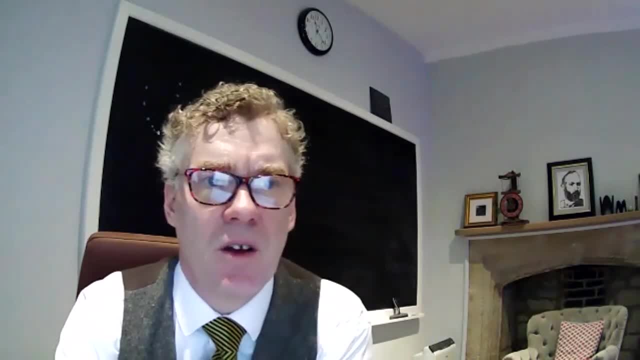 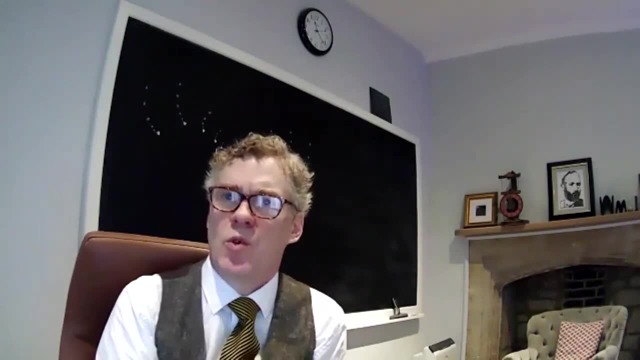 Okay, so let's talk about the specific axioms. Okay, so let's talk about the specific axioms of set theory that were introduced. So what are the core principles of set theory? Cantor worked in an intuitive set theory. He didn't have any formal system or formal axioms. 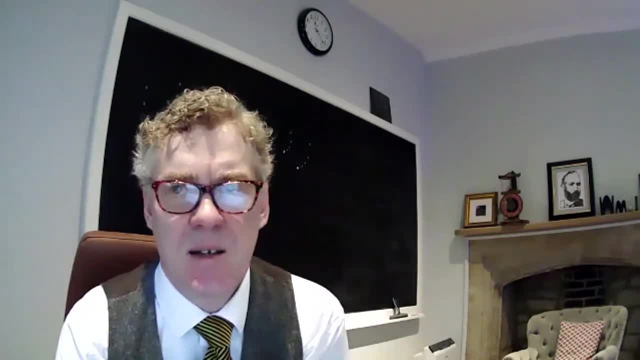 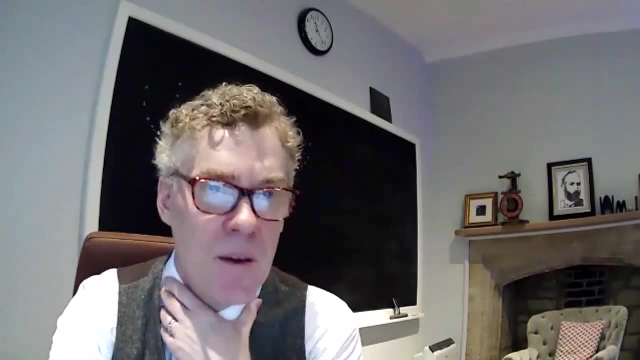 but later there were several different formal set theoretic systems that were made, for example, by Frege and ultimately by Zermelo and others, including Frankl and Bernays and Gödel and von Neumann, So at the very center of set theory, of course. 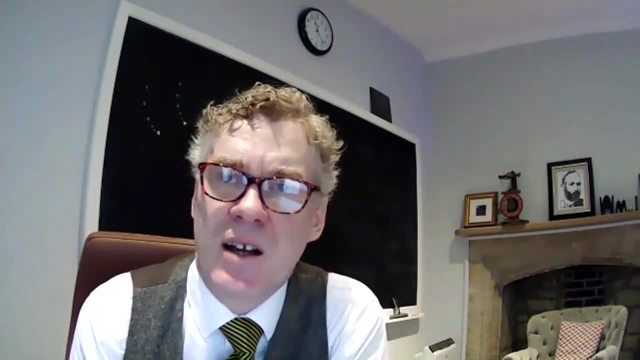 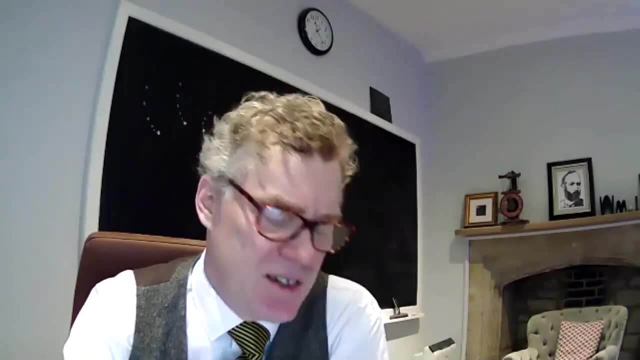 is the idea that one can consider a collection of things as a single abstract thing. a set is a single abstract thing, a set Consisting of those things and only those things. But which collections can you have, Which collections can you bring together in that way? 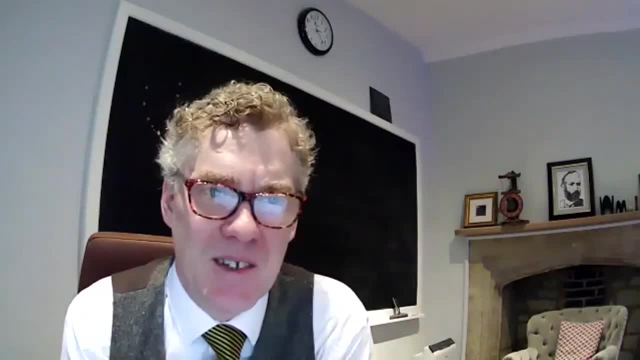 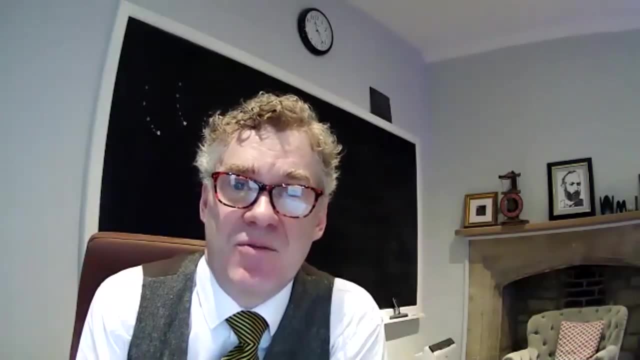 And the answer, of course, is well, all of them. of course. If we have a way of describing or conceiving of a collection, then, according to the naive version of set theory, then we can form the set consisting of just those objects. 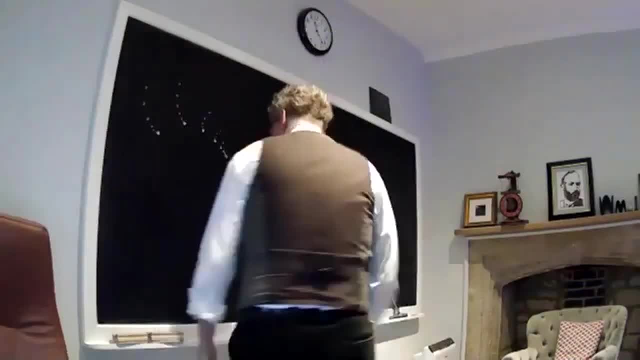 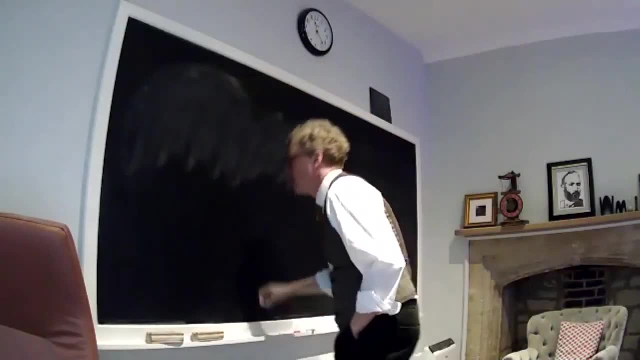 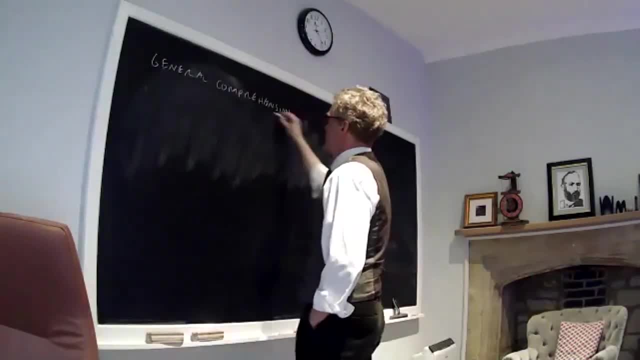 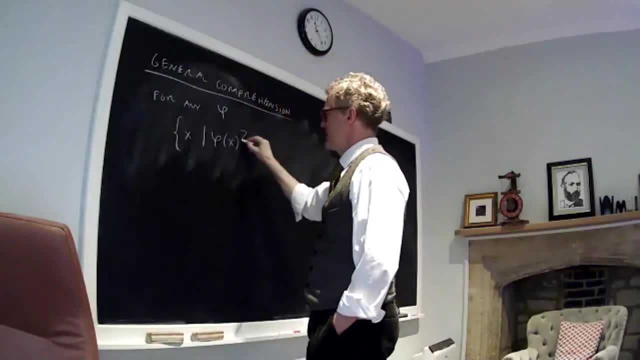 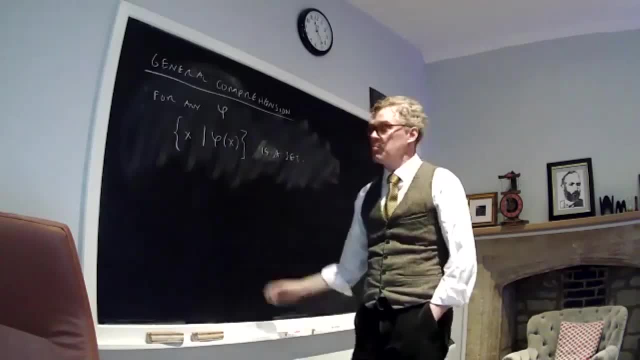 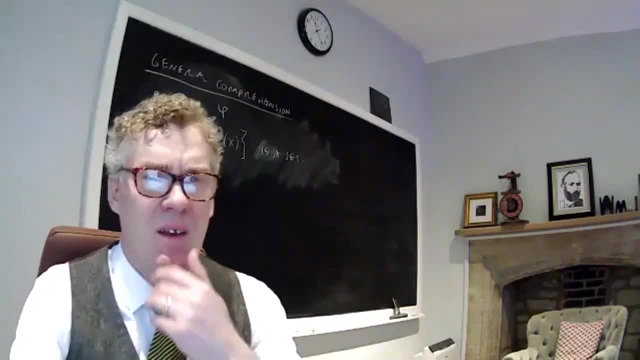 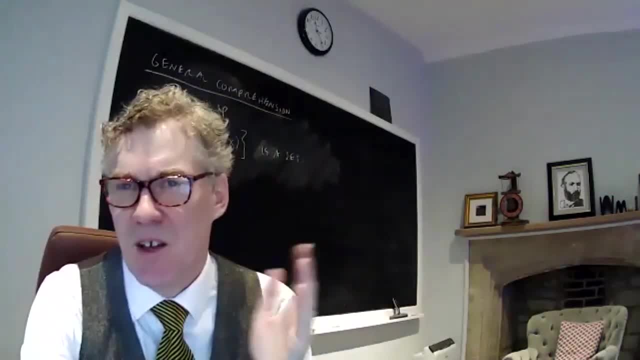 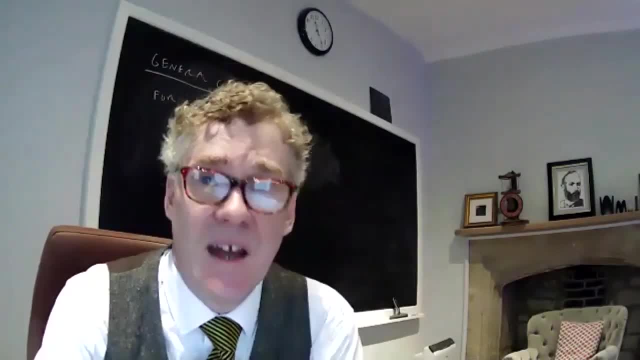 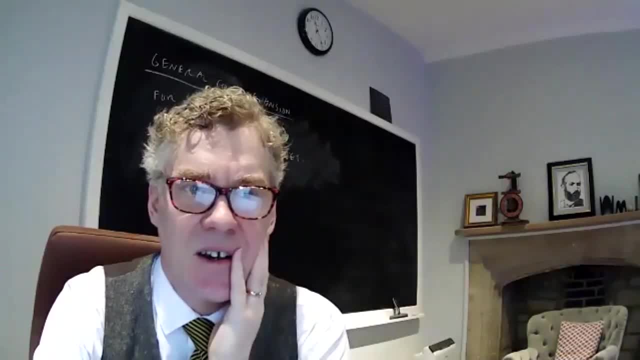 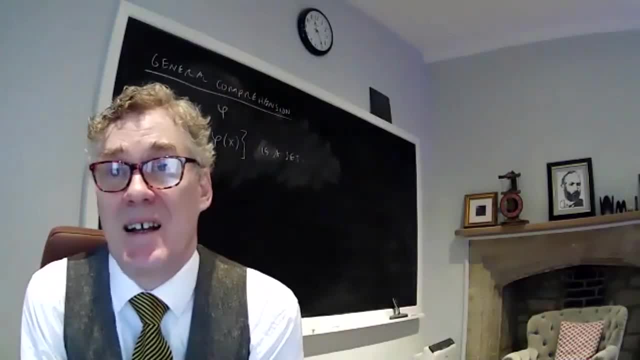 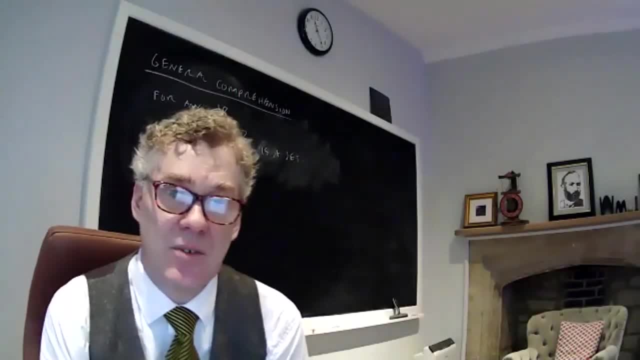 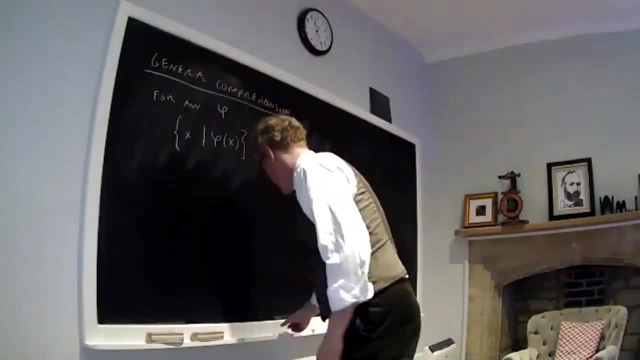 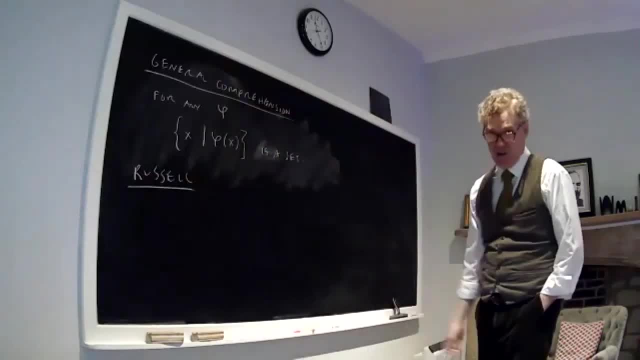 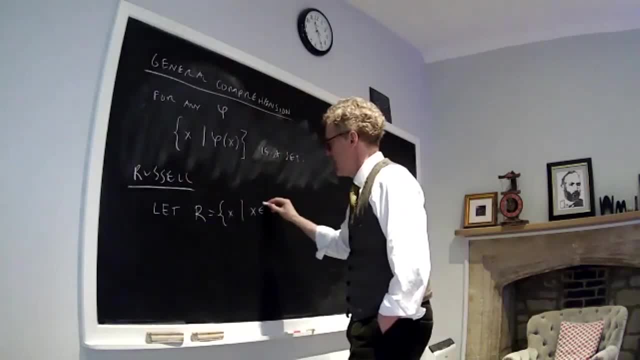 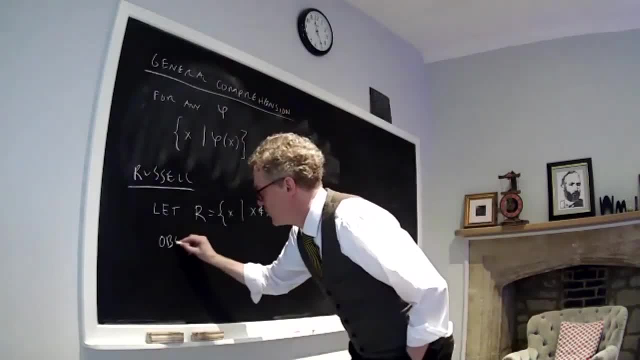 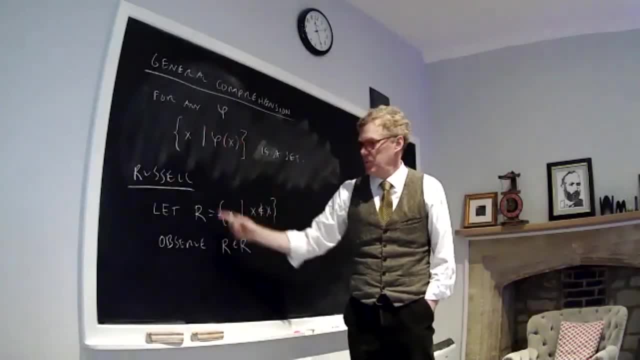 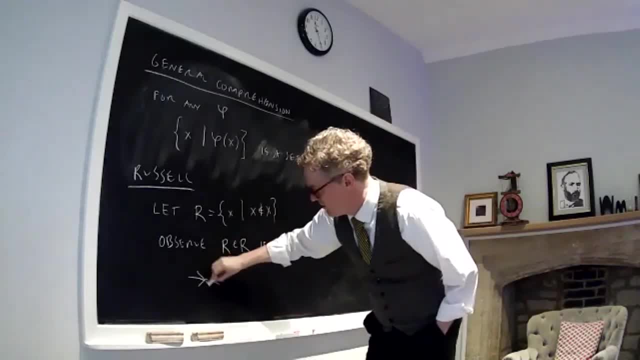 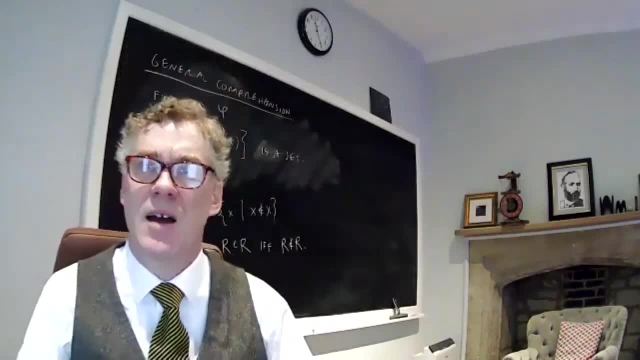 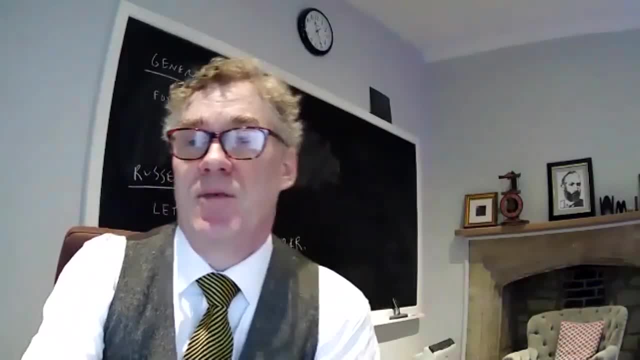 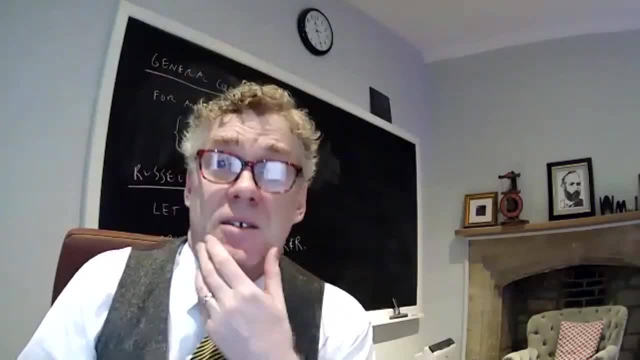 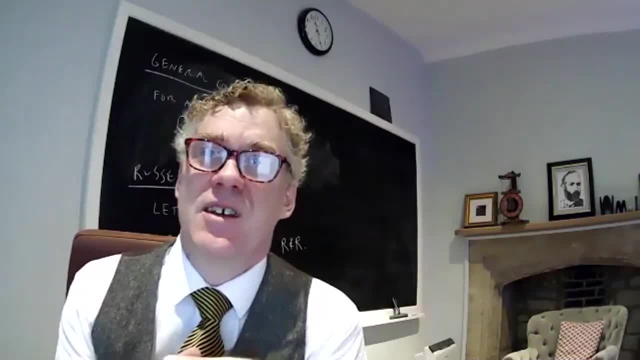 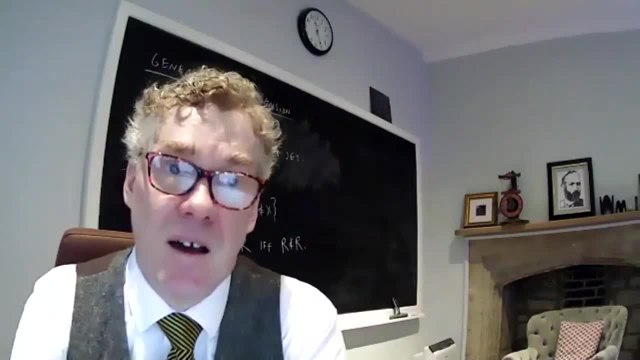 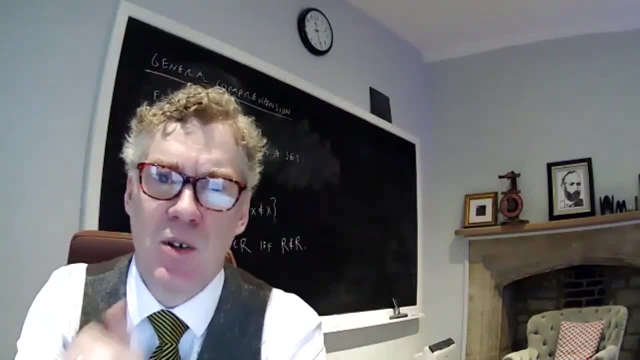 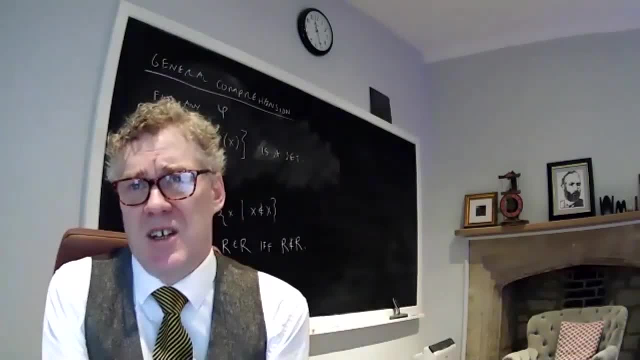 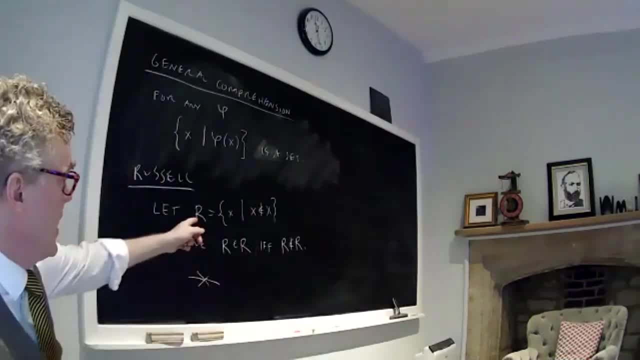 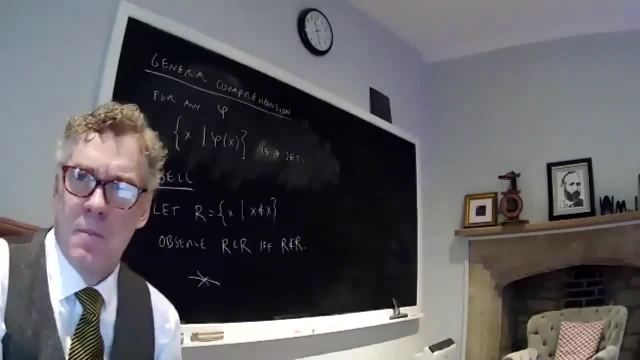 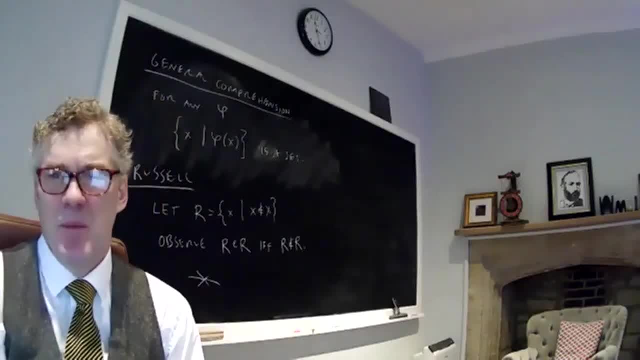 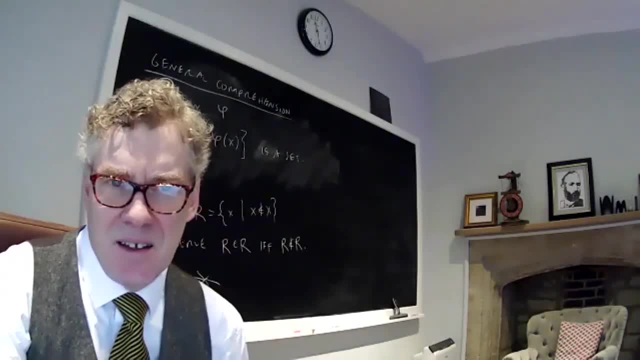 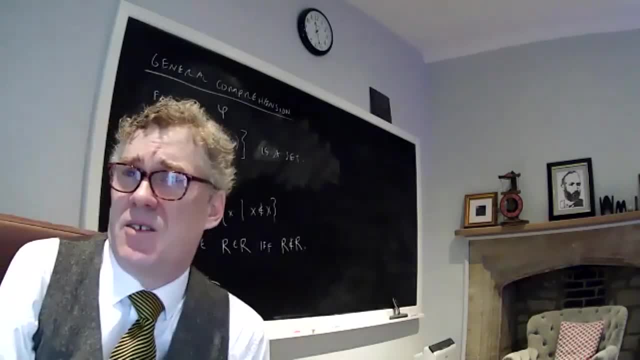 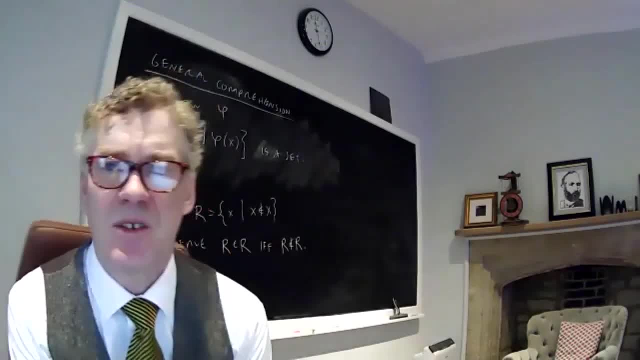 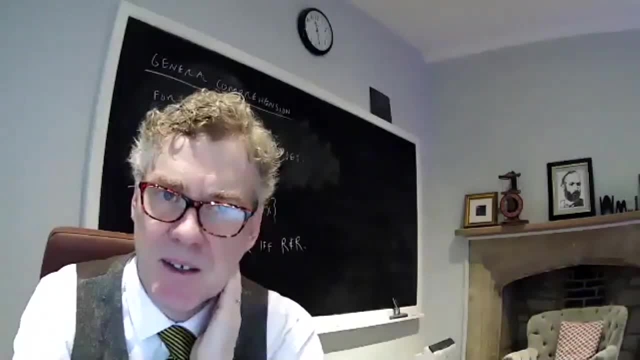 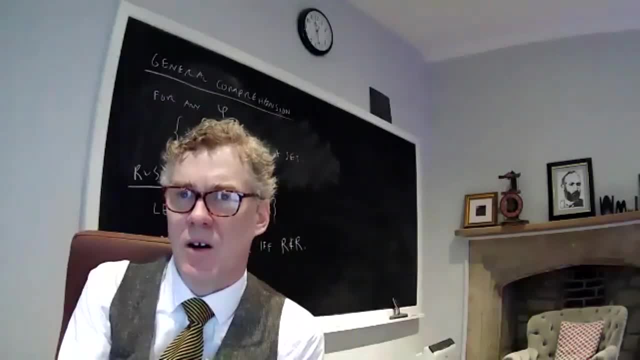 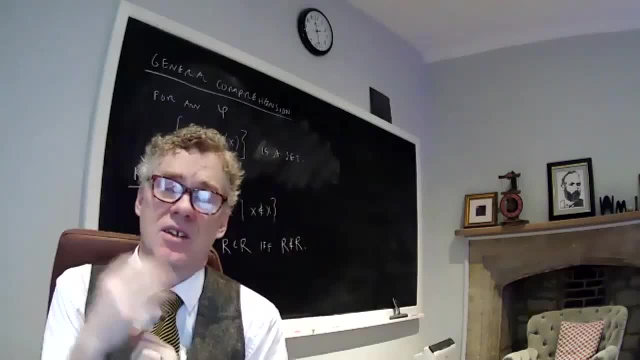 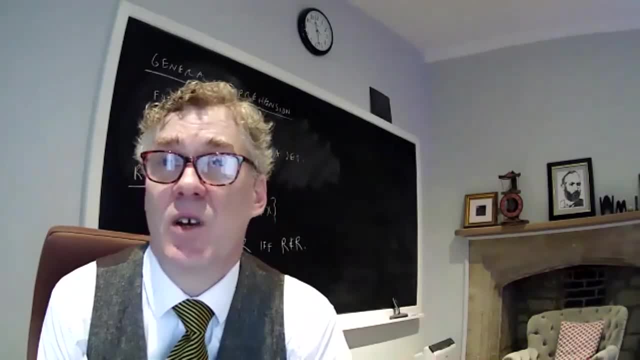 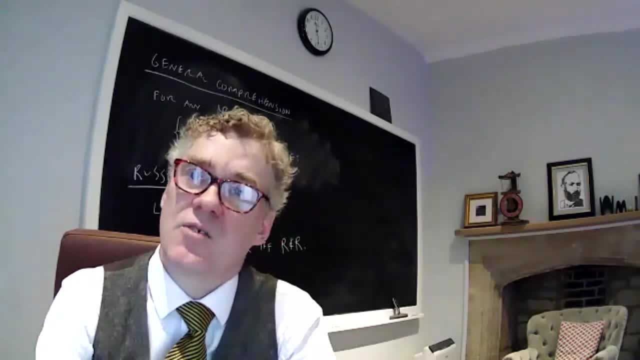 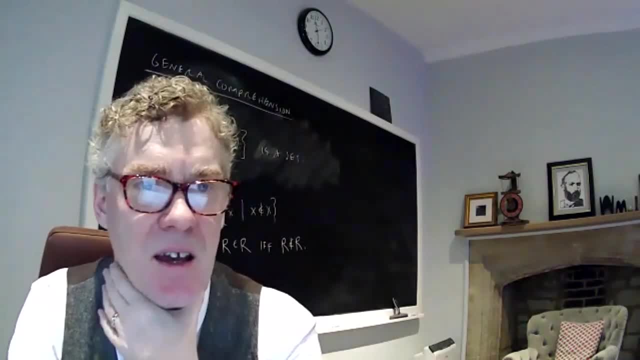 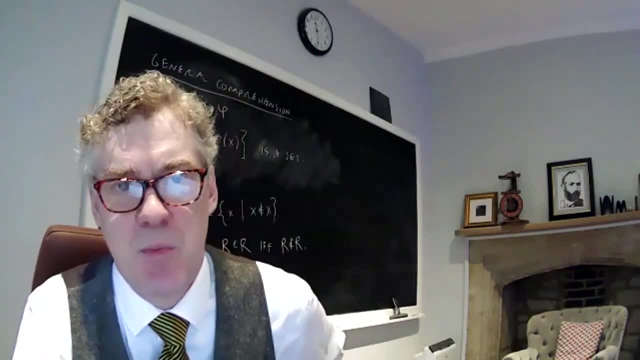 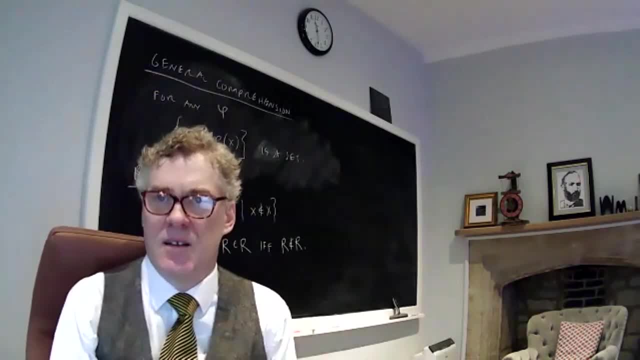 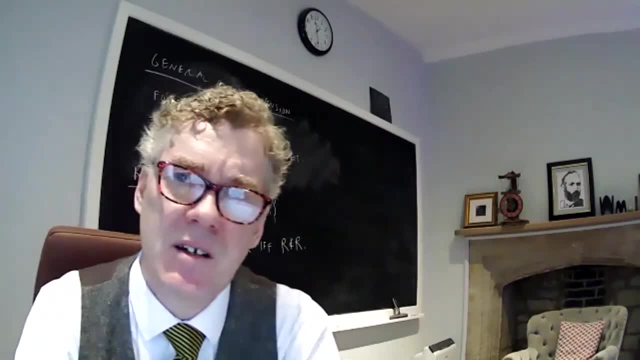 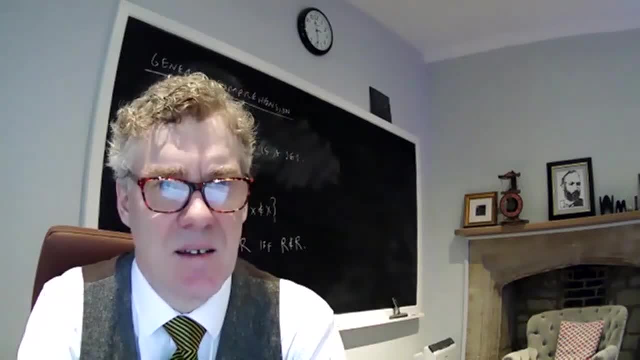 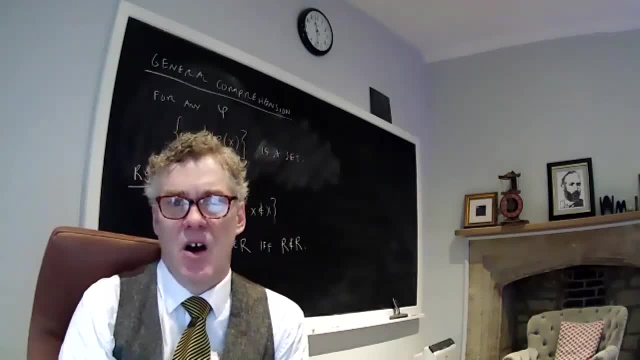 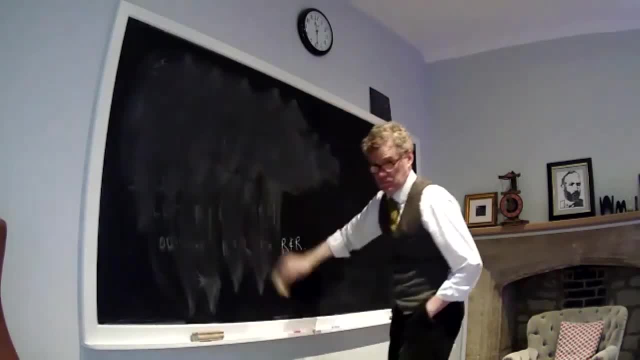 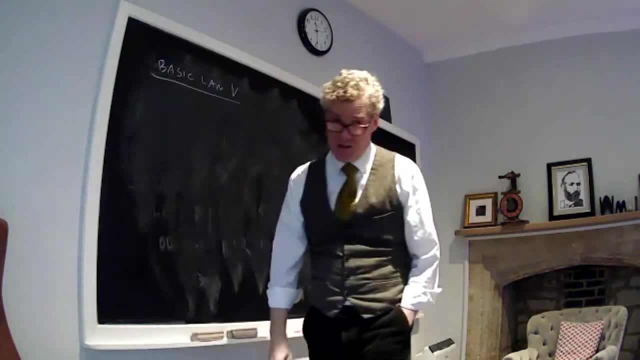 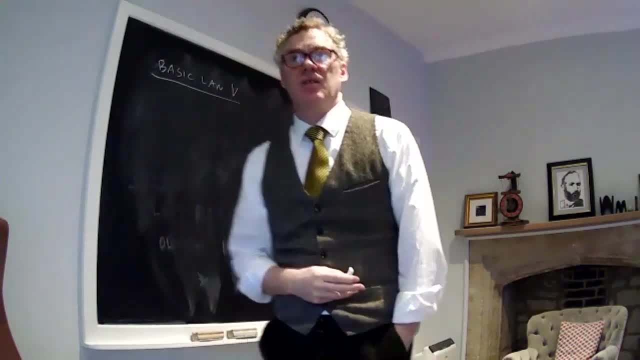 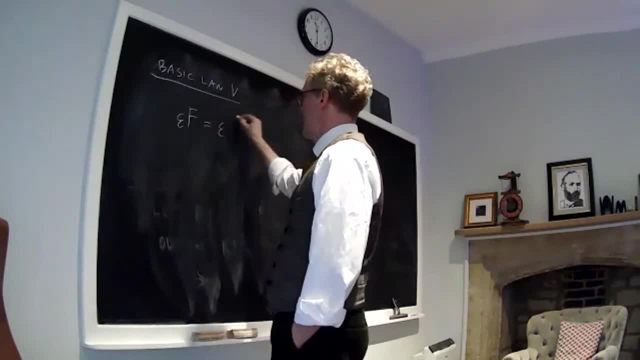 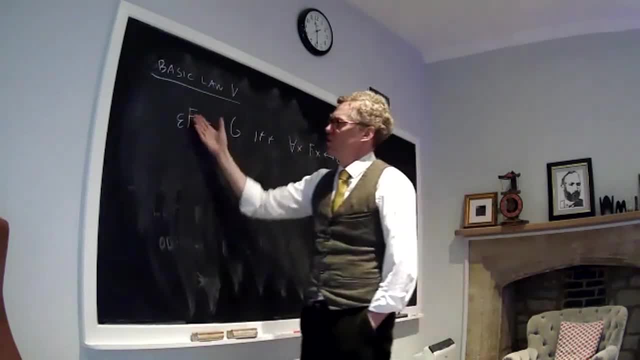 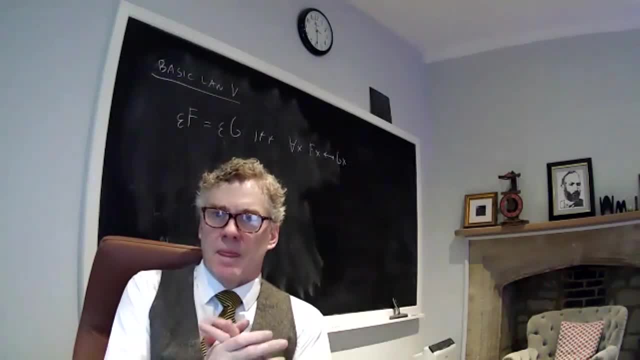 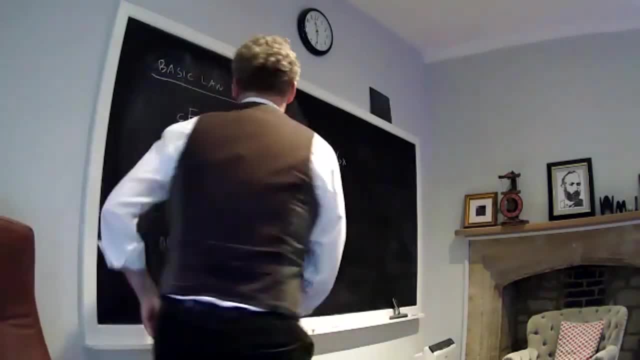 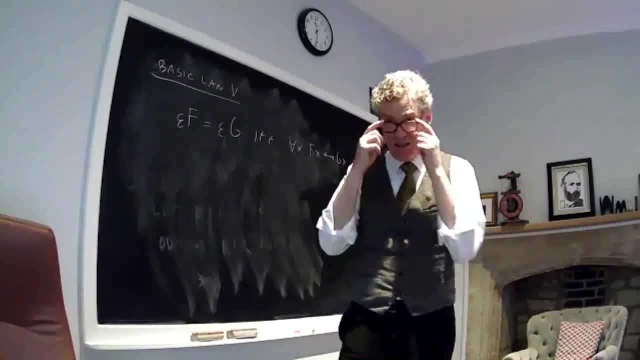 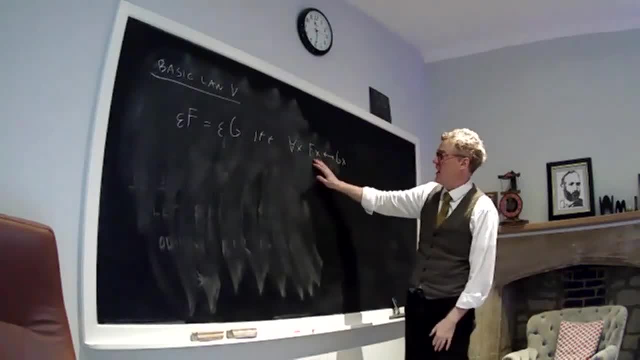 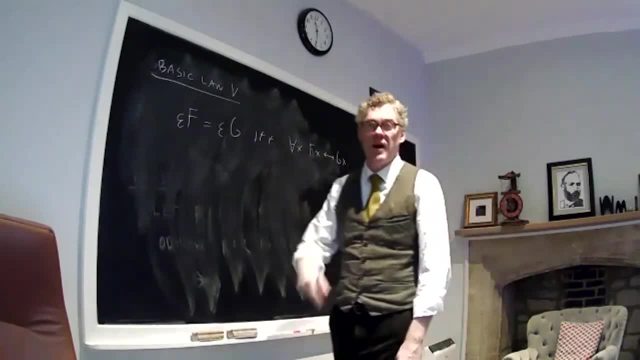 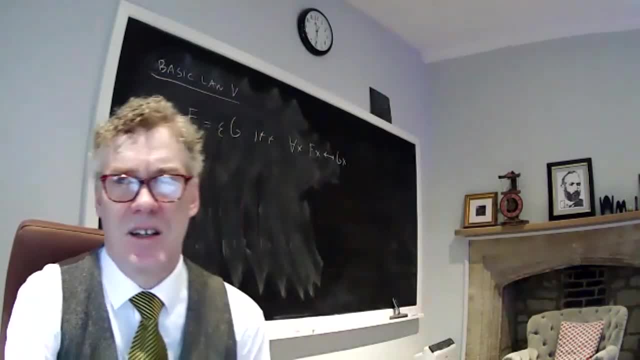 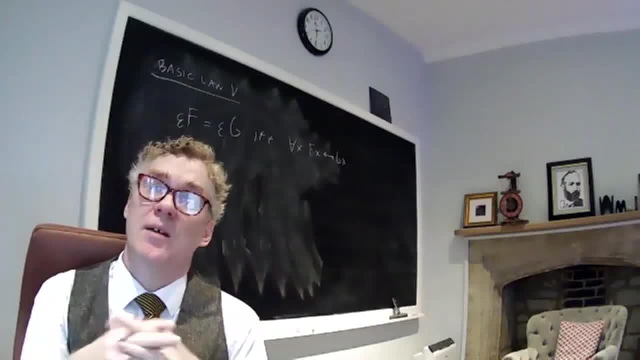 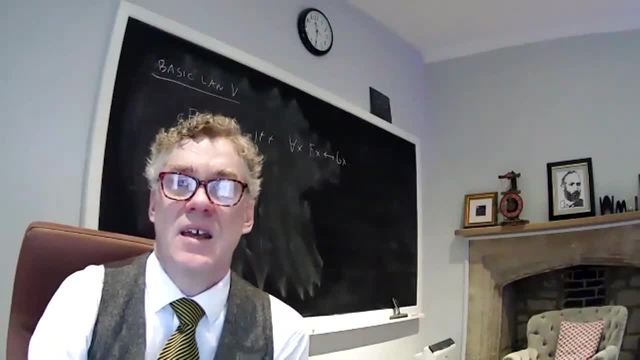 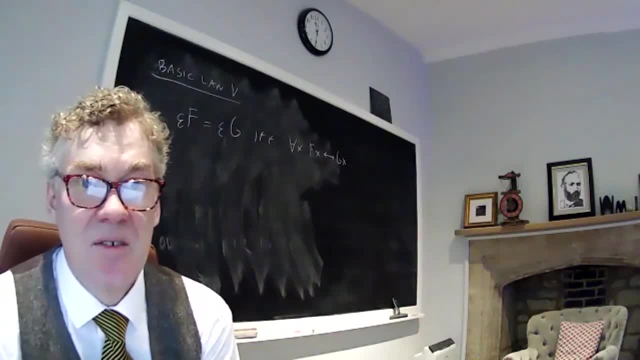 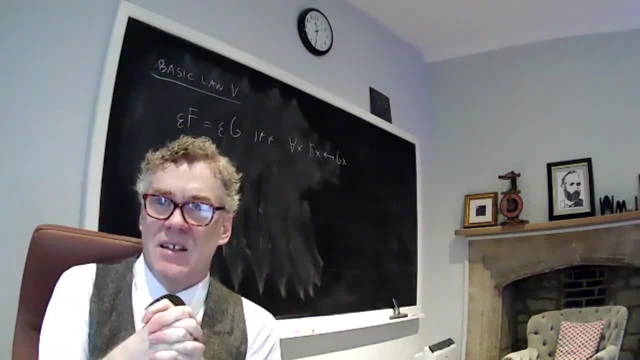 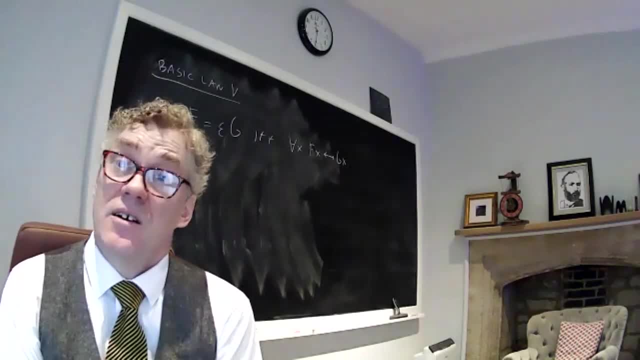 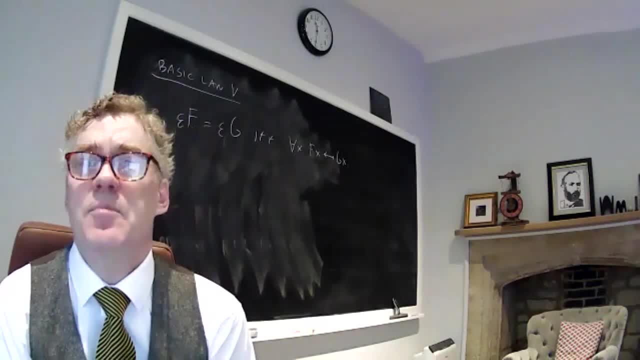 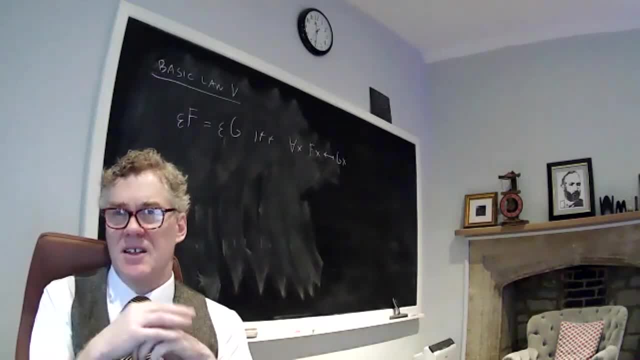 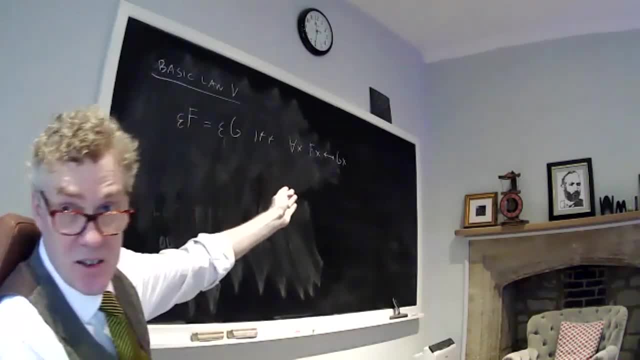 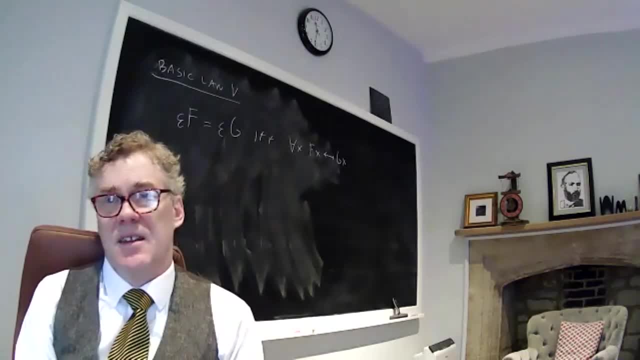 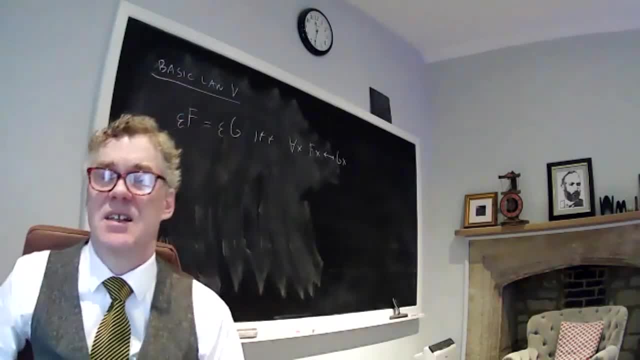 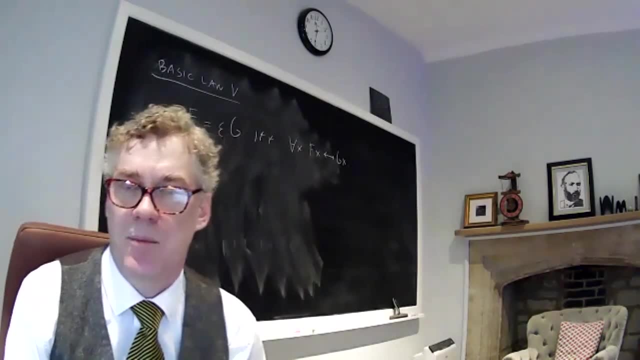 Okay, so general comprehension. Okay so general comprehension. Okay so general comprehension. I can't remember precisely the distinction between whether it's something is a mathematical object or whether it's just a concept that that can be treated as a predicate of objects. 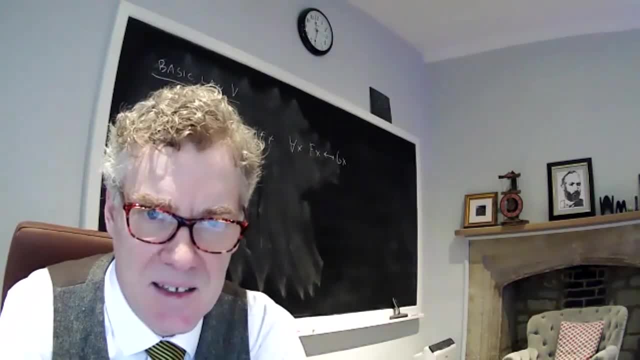 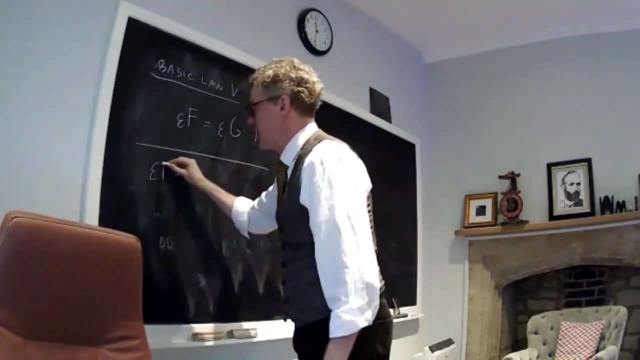 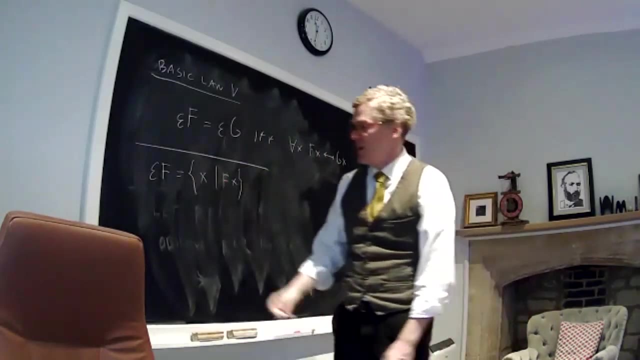 Okay. so in the current class theories we generally think of, okay in contemporary, in contemporary classes, the extension of a concept F is just the class of all x, such that f. but we don't really go this as a set mythoph beleza class, and so classequal ticket ultimately. 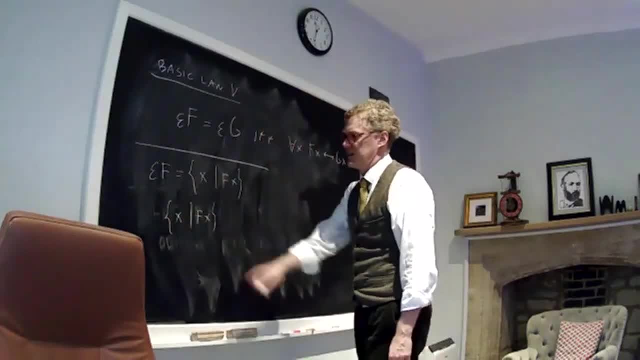 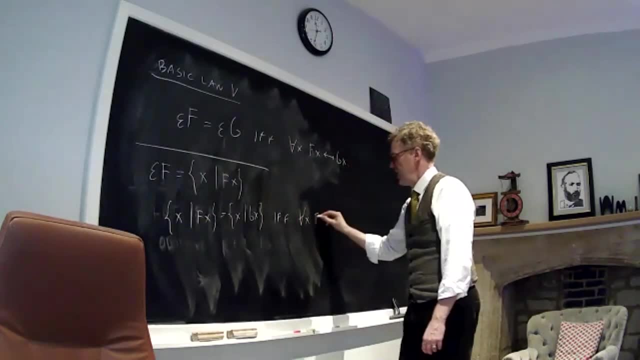 is the claim that that the class of elements x, so that f of x, is equal to the class of elements x, so that g of x. just in case for all, x, f of x if and only if, g of x. It looks identical to the basic law of five. 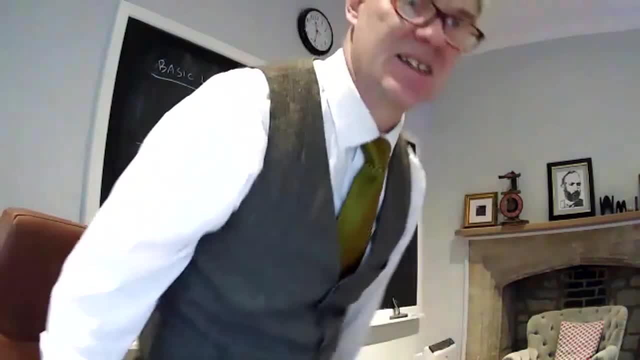 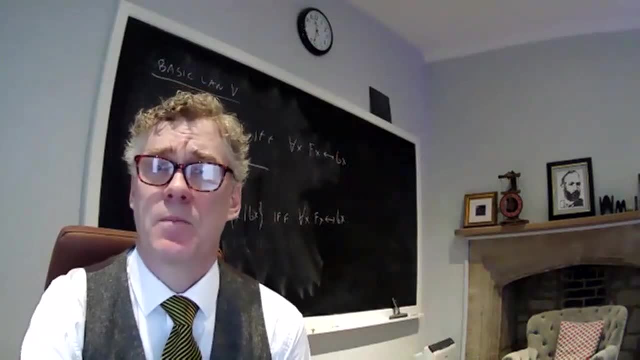 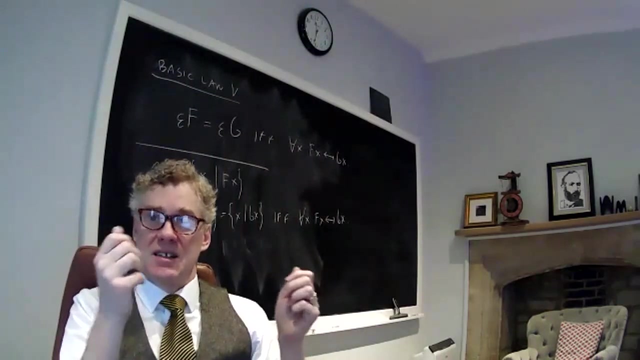 but this is now taken as an axiom, the axiom of class extensionality. Two classes are equal, just in case they have the same elements. Okay, so one should really place the blame of the inconsistency on the general comprehension principle, around the idea that every predicate determines. 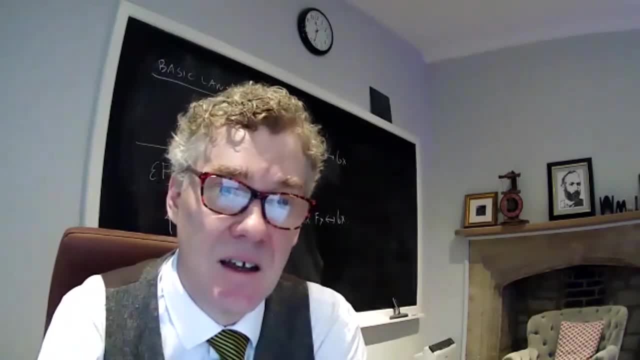 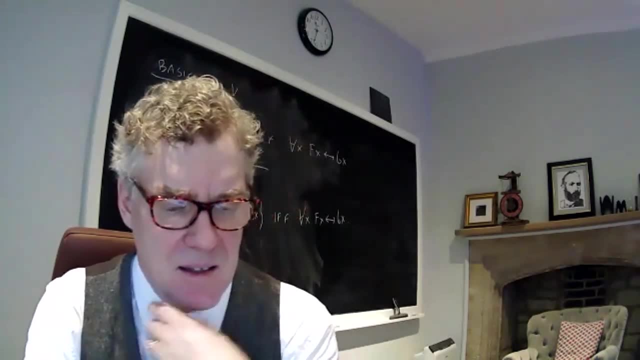 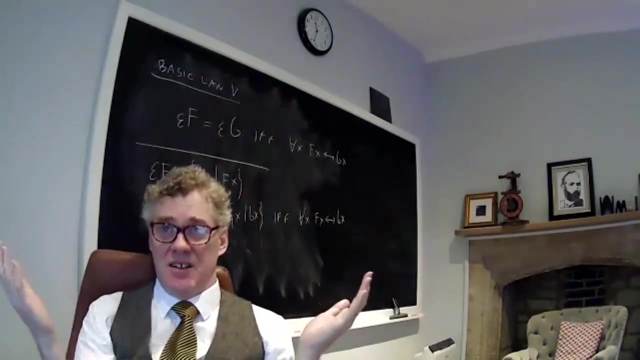 a set object, which is the extension of that property. Okay, so let's consider all right Russell's refuted general comprehension. it's inconsistent. So what is to be done? I mean, is the objection destroying set theory? Have we destroyed set theory? 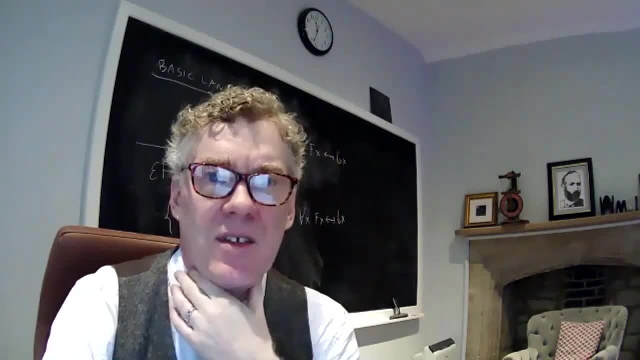 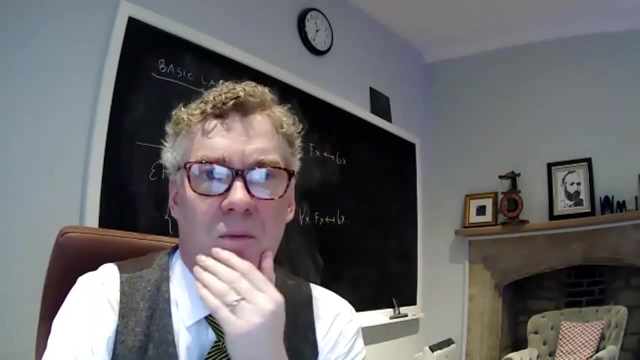 So, no, let's think a little bit more carefully about the nature of the set theoretic universe that we've been imagining, And if you do so, then you're gonna arrive at an account of what's called the cumulative hierarchy. This is a vision of how the set theoretic universe 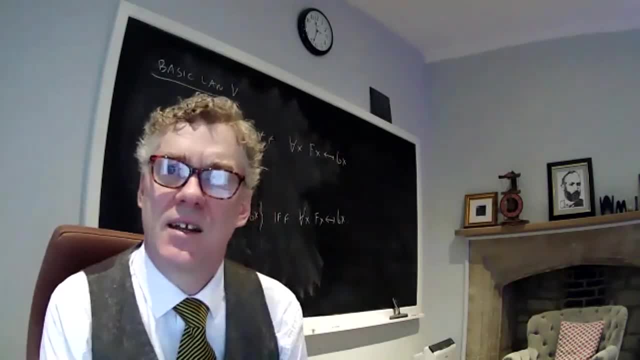 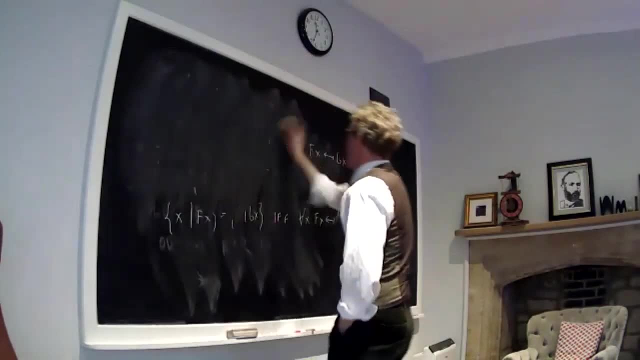 is formed in a cumulative hierarchy of set construction. So maybe we start with say: some objects that aren't sets, the error elements. So maybe, maybe you have some, oh okay, some oddity. Maybe there are few that aren't sets, that aren't set. Then we talk about the perceptions in your dolls. Maybe there are a few that aren't sets, but not the even edge. So maybe we start with say some objects that aren't sets, the irr elements. So maybe you have some arguments. 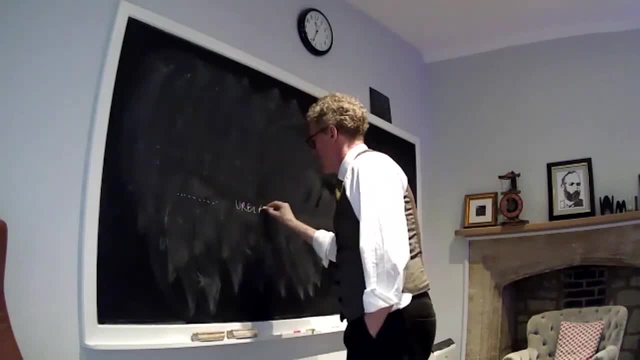 Across theseissy on students. two or three, subtract Y plus, if plus or minus, I minus. y plus G plus R, squared given. look for plus X, some ur-elements, those are mathematical objects, primitive objects, atomic objects that are not sets okay. 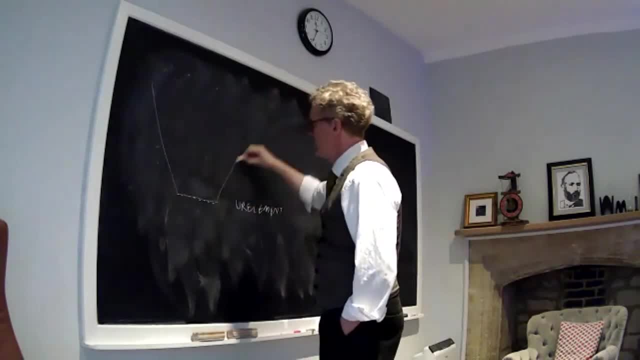 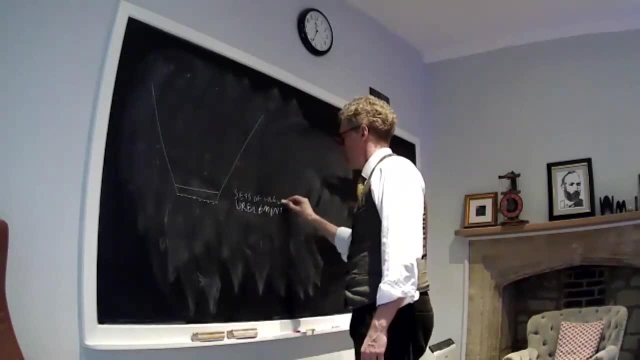 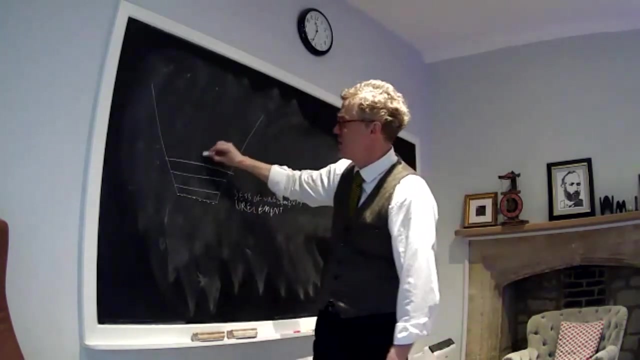 And then you build up the set theoretic universe from them. So at the next level you have sets of ur-elements And then at the next level you have sets of sets of ur-elements and then sets of sets of ur-elements and so on in a transplanted hierarchy. 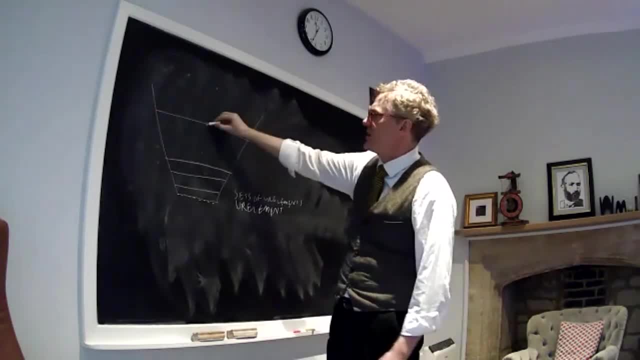 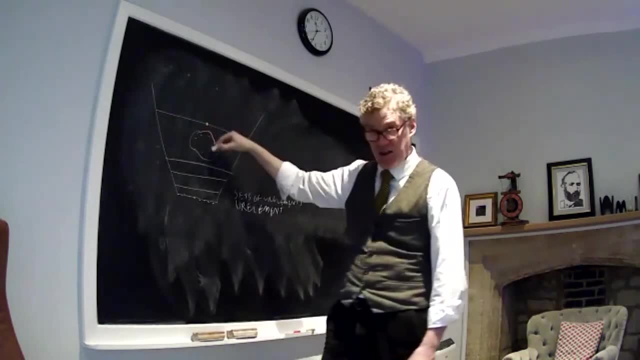 So sets are sort of born at a stage in this hierarchy, just in case all of their elements already exist. So when a set comes into existence, it's because its elements already have come into existence at an earlier stage. And in this way we're accumulating more and more sets. 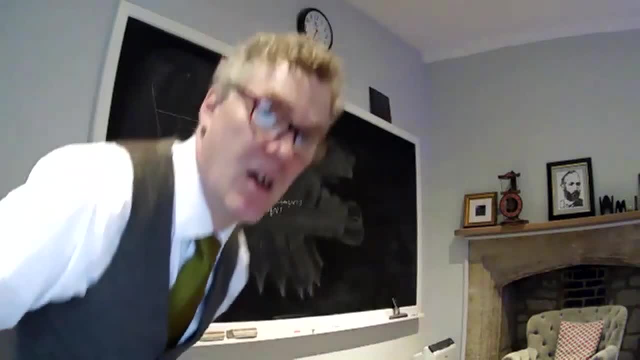 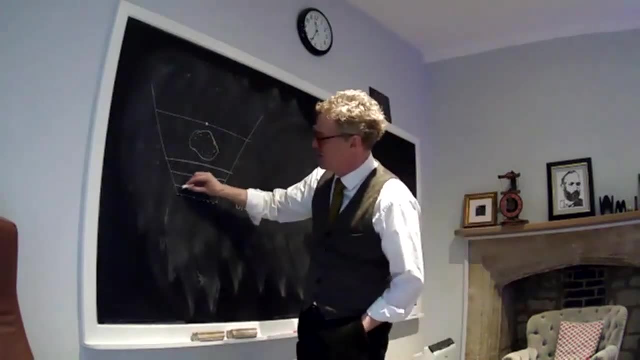 into the universe. This is the cumulative hierarchy picture of the set theoretic universe. We can think about what happens with sets that don't use any ur-elements. Of course, we can have the empty set and then set the set contained in the empty set. 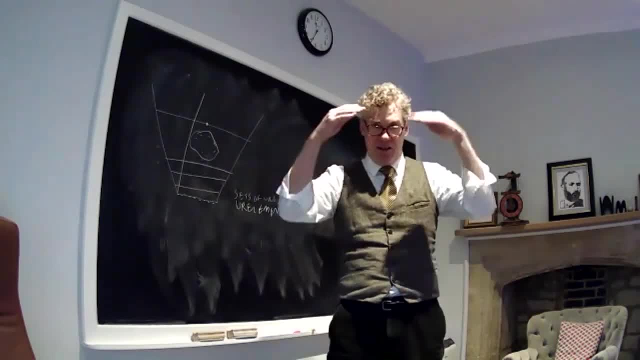 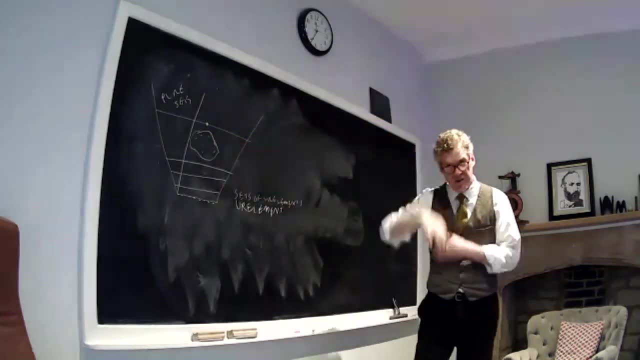 and the set contained in the empty set and the set contained in the empty set and so on. We can look at what's called the pure sets that don't have any involvement with the ur-elements in their hereditary membership History, and that's the kind of set theory. 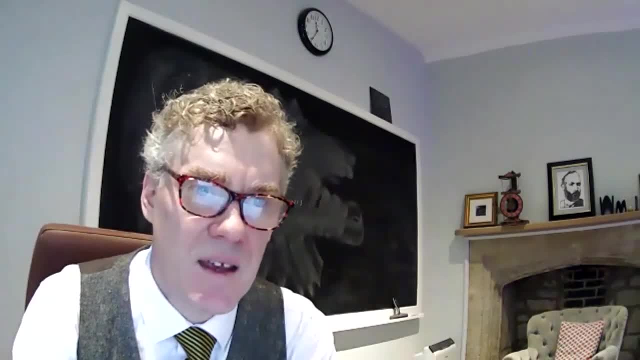 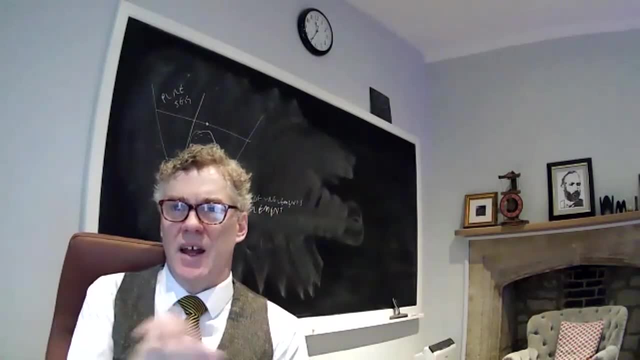 that you would get if you didn't start with any or elements at all. Now, of course, set theory is quickly realized that we don't actually need your elements for any purpose. So it in the fundamental set theory foundational role, any mathematical structure that can be represented in the cumulative hierarchy. 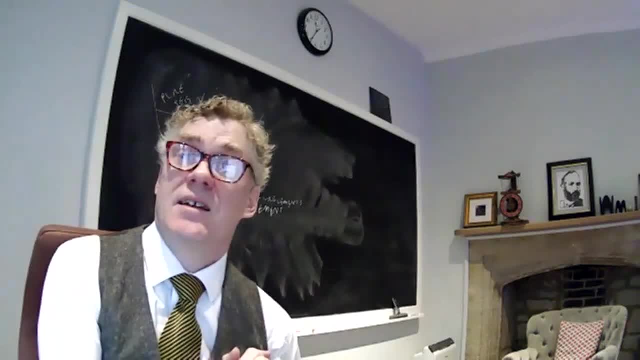 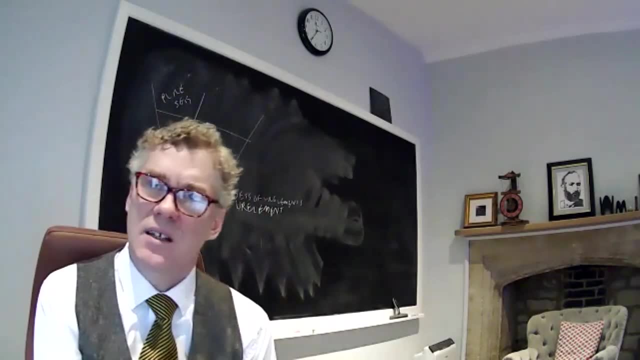 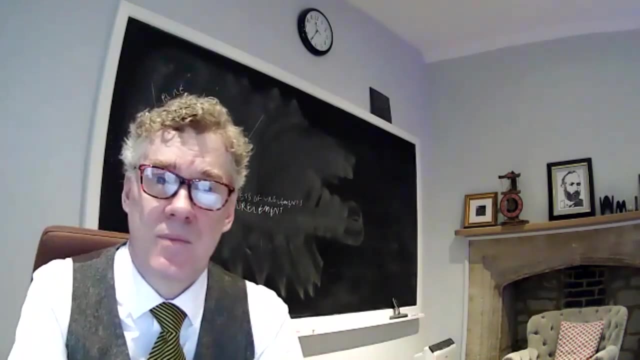 with or elements can also be represented by a set in the, in the pure sets, without using the elements, and so the set theory becomes sort of cleaner and more elegant and simpler if we, if we don't use any or elements at all, they're not needed for any mathematical purpose. okay, and so? 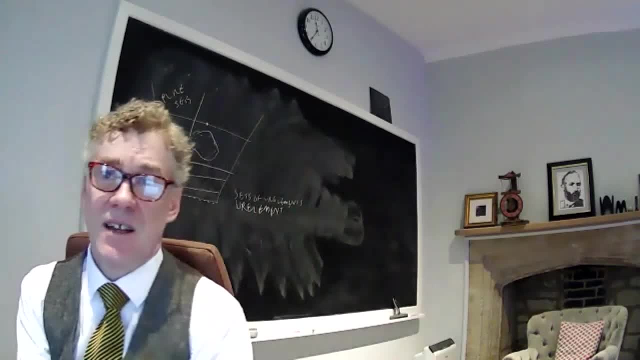 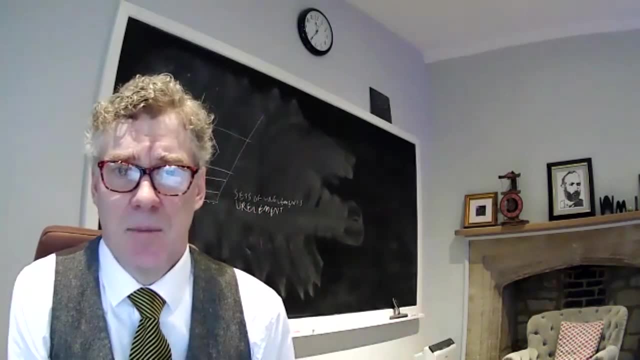 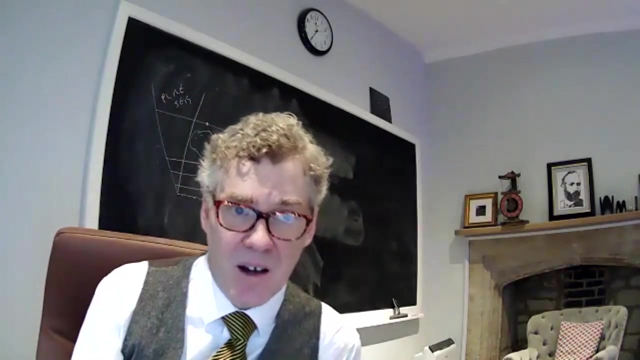 the typical axiomatizations of set theory that are considered now don't have any elements. every thing is a set and, on this view, every mathematical object, the entirety of mathematics, consists of sets, or sets of sets and sets of sets of sets, and so on in this vast cumulative hierarchy. so 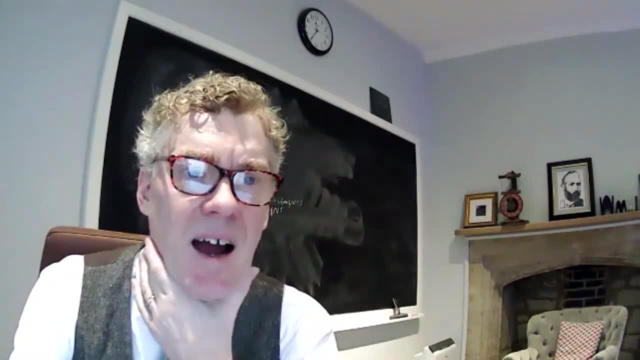 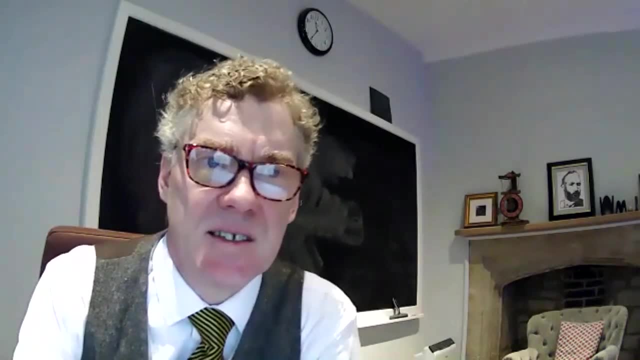 terlakis sort of makes fun of this situation by highlighting the curiosity of it, he says. i find it extremely counterintuitive, especially when addressing undergraduate audiences, to tell them that all their familiar mathematical objects- the stuff of mathematics, in barweiser's words- are just 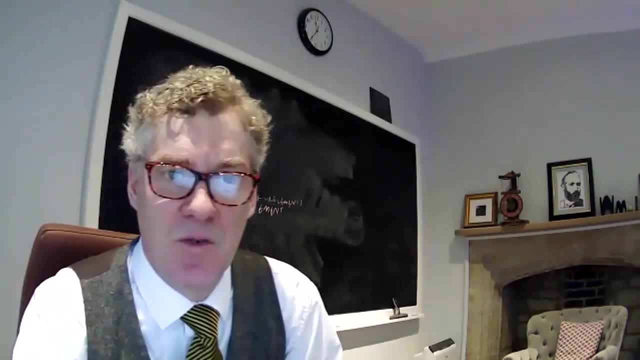 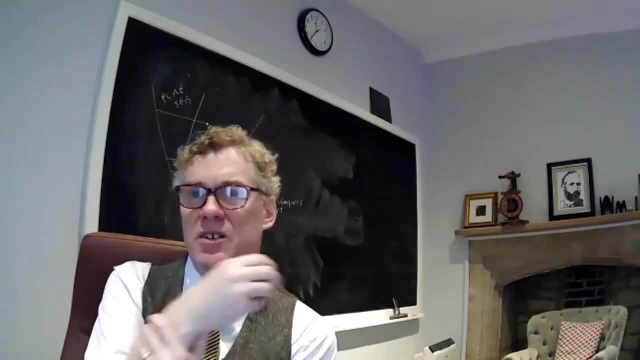 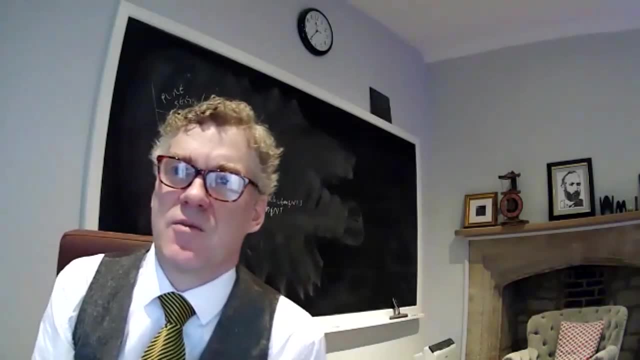 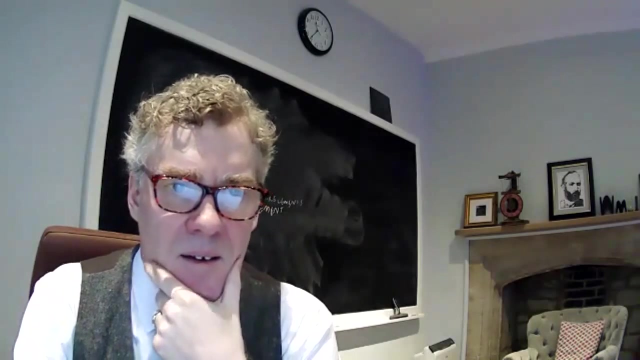 describing is this sort of pure set construction, where every set consists of other sets that consist of sets and so on, all the way down until you get the empty set, and so it's just boxes of boxes, of boxes of boxes, but ultimately empty when you go all the way down. okay, so let me make a 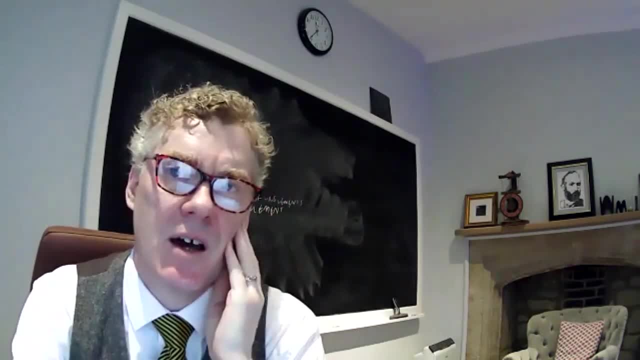 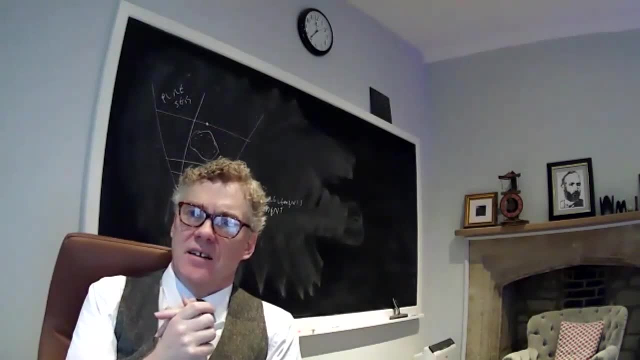 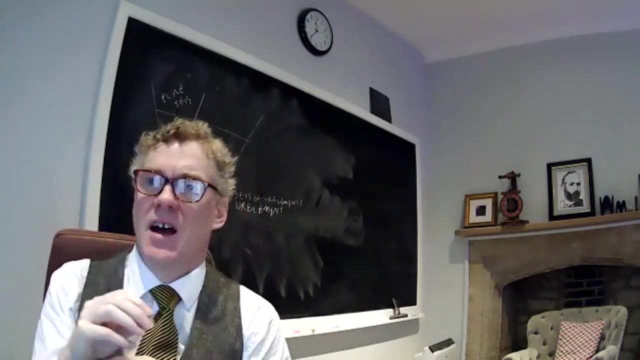 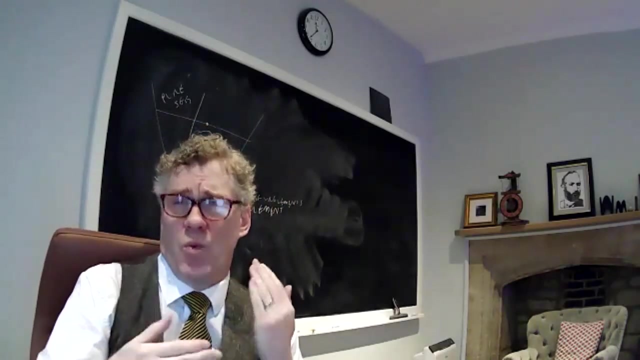 critical point about this cumulative hierarchy vision of how the set theoretic universe is formed, and namely, if we have this cumulative hierarchy understanding, then we don't get any support at all for the general comprehension principle, because in this cumulative hierarchy a set comes into existence only after all of its elements do and therefore we can't seem ever to form the set of. 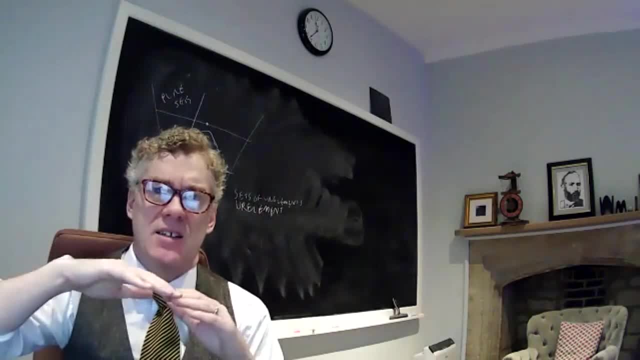 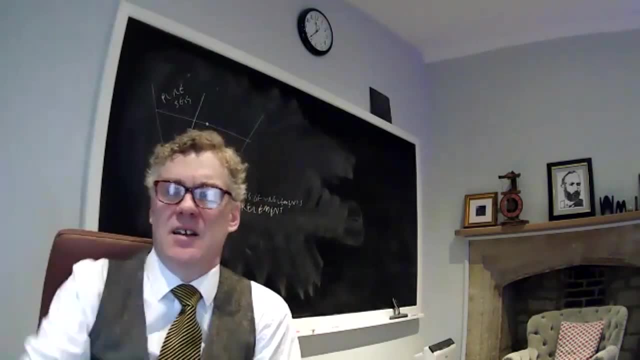 all x such that phi of x, unless we knew already that all the set of all x, such that phi of x, all of those x's, would come into existence by some stage. but if those x's are going to be sort of co-final or unbounded in the, in the hierarchy itself, then we don't expect ever to form the set. 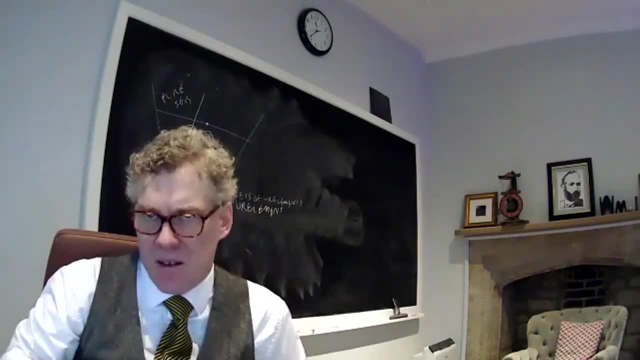 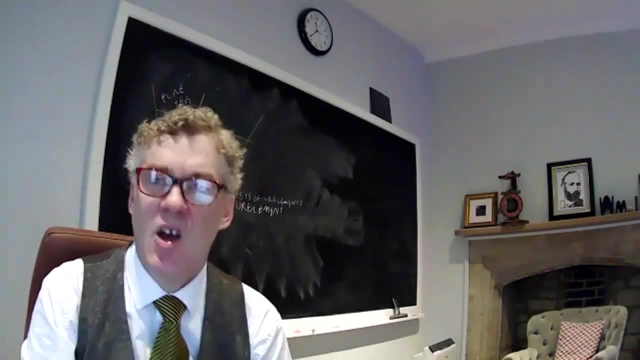 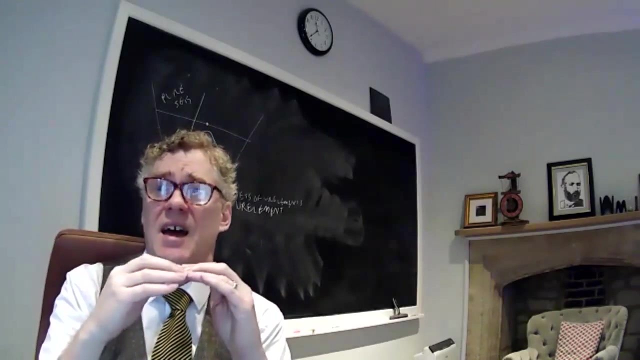 of all x, such that phi of x, because that that the elements will never be completed, all of them, and so we can't ever get it at a stage where we can form that set. furthermore, we never expect to see x element x, because in the cumulative hierarchy the sets come into existence only at a stage after. 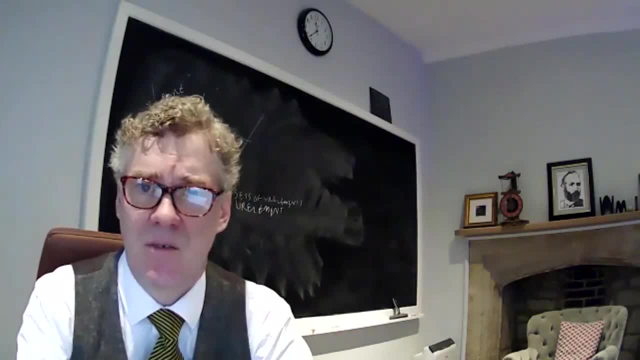 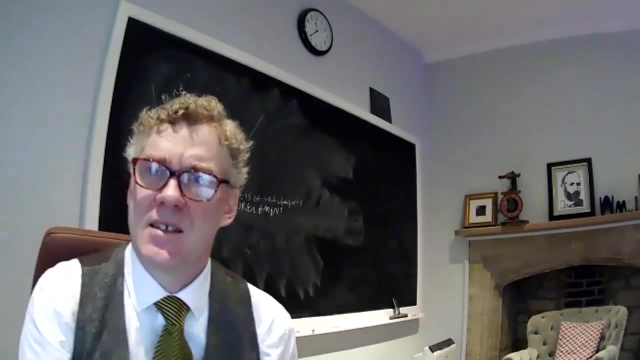 their elements do, and therefore we don't expect to form the set of all x such that phi of x do, and so therefore x can't ever be an element of x. so the idea is that there's this sort of well-founded hierarchy of stages in the cumulative hierarchy, and this is a fundamentally different. 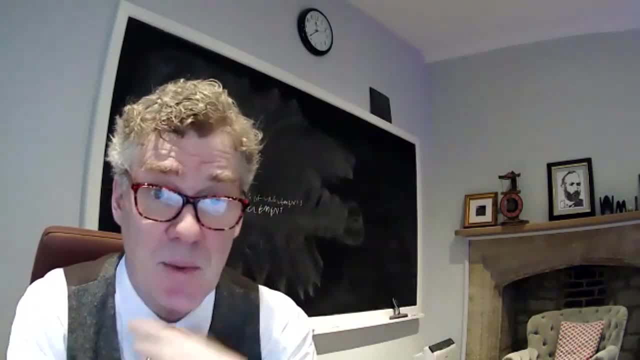 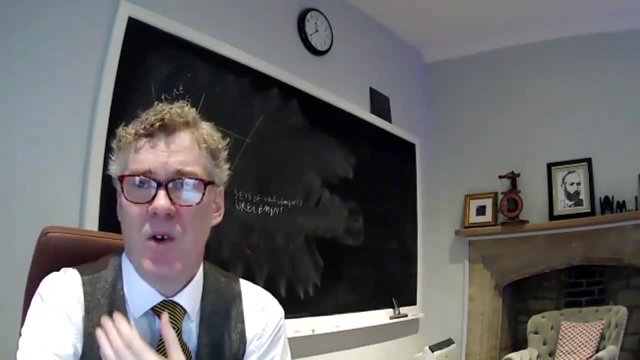 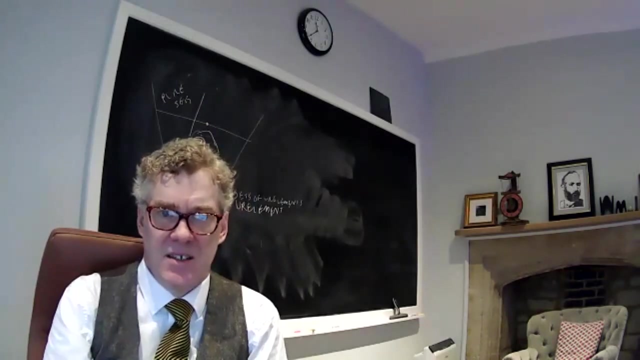 picture than what the general comprehension axiom is about, and so so the intuitive pull that we might have felt for the general comprehension principle simply falls away, and we recognize that it's not part of our understanding of how the set theoretic universe is coming into existence, and it should be. 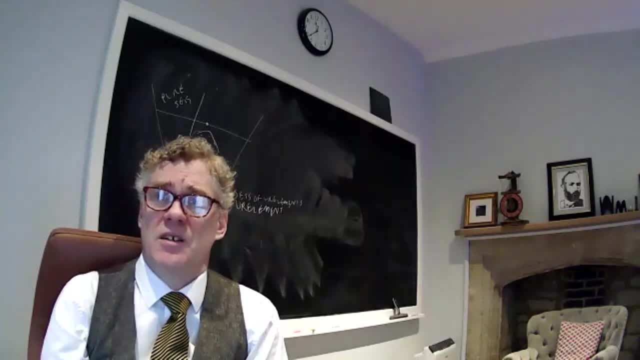 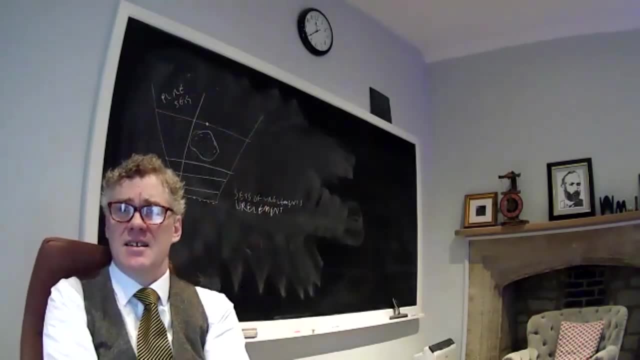 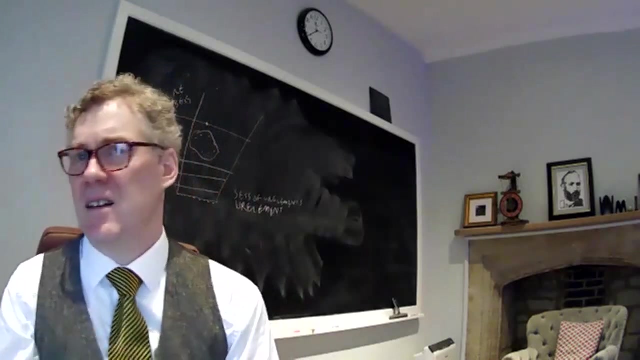 understood as a naive mistake and, furthermore, one that is very easily refuted. i view it as something like a mistake about, say, denying the antecedent. the fallacy of denying the antecedent is a logical error and everyone recognizes it as a logical error, and it's a mistake to think that somehow. 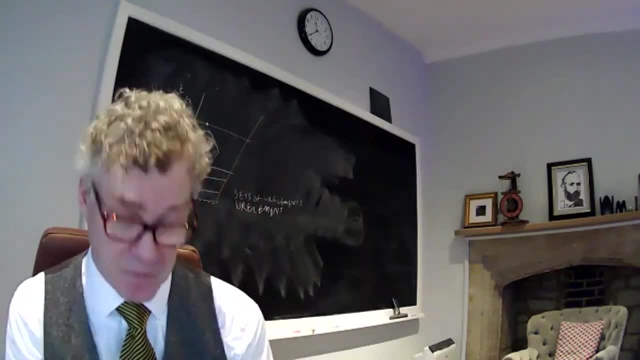 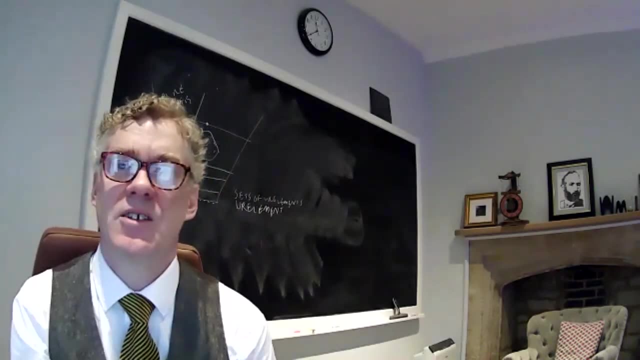 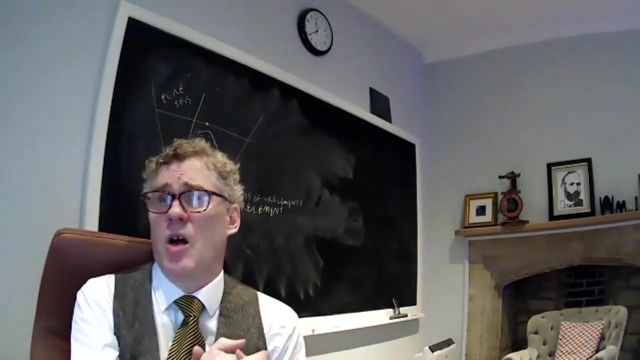 it's a correct principle to follow the law of denying the antecedent. that's the principle that says right, if you have p implies q. therefore, not p implies not q, it's just fallacious and it's wrong. okay, so then how to twentkee? to give counter examples, just like the general comprehension. 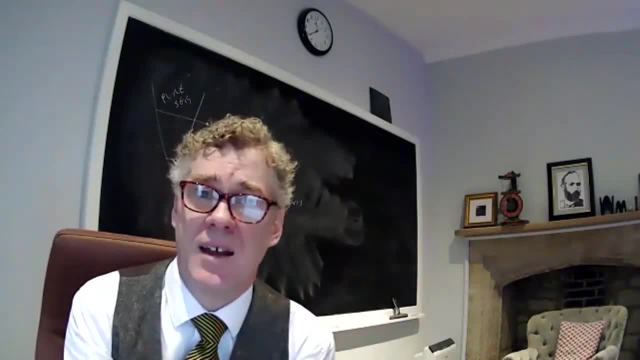 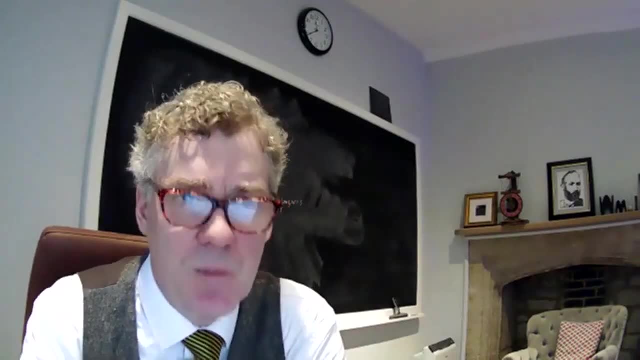 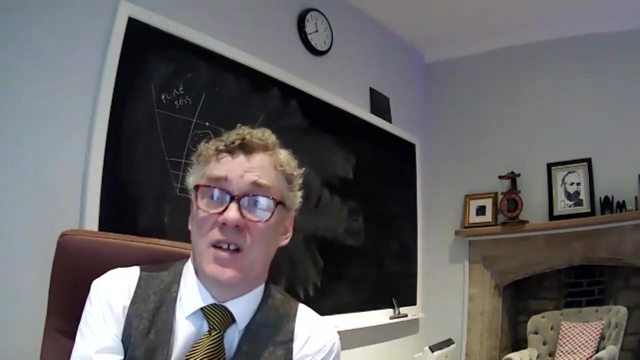 principle maybe seems plausible when you first encounter it, but russell's argument in one line shows that it's simply wrong. okay, so that the principle that we would be led to by contemplating comprehension in the context of the cumulative hierarchy is what's known as the separation axiom. separation axiom says: if you have 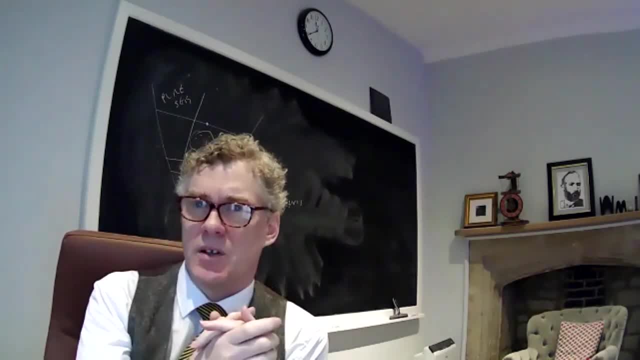 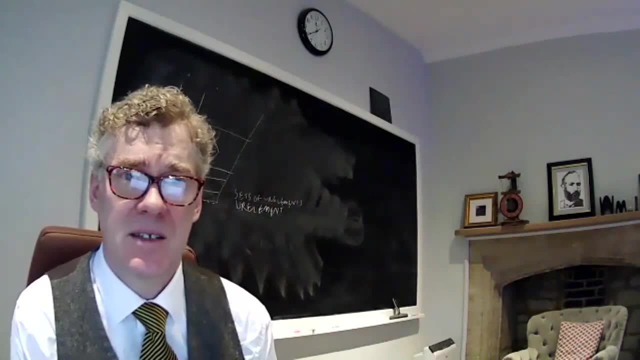 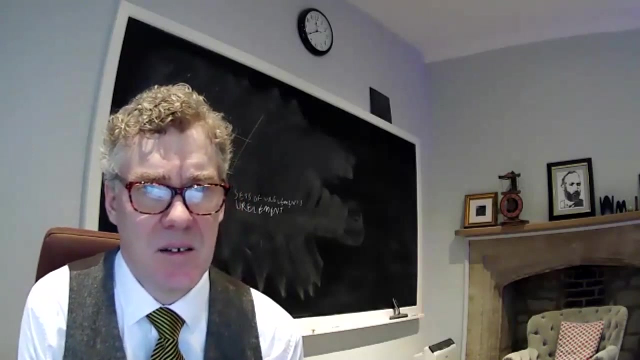 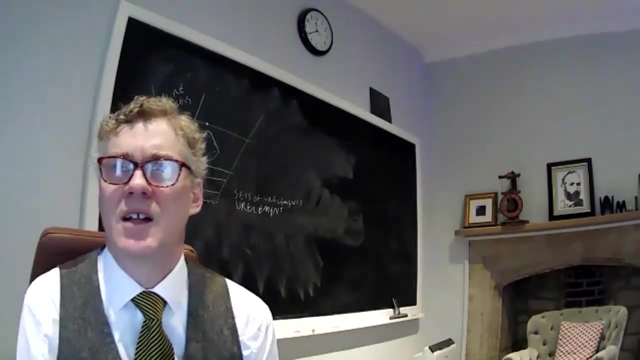 a set already set that have that property. you can separate out from any set the objects that have a property, whatever property you like. okay, this is called separation axiom, and uh um. so in sir mellow's original account of the separation axiom he he had an extremely broad concept of what counts as 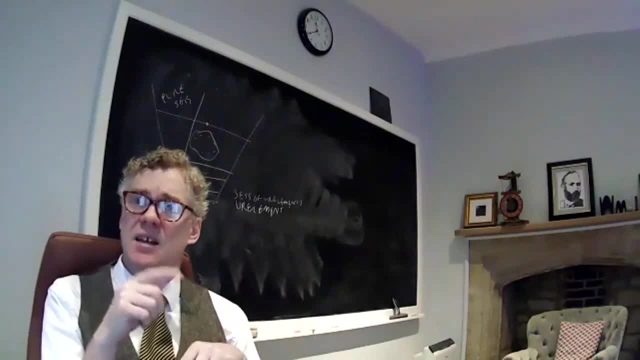 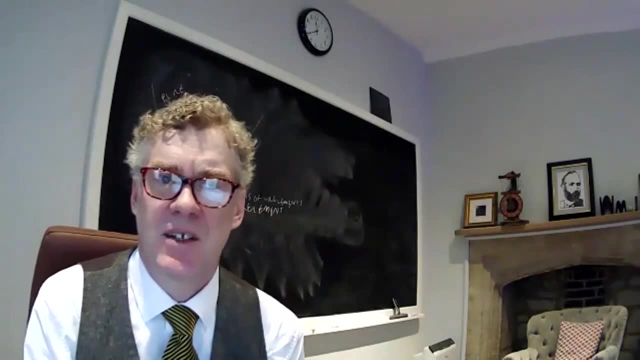 a property. yeah, so for any property you want to form the set of all x in a given set, a such that phi of x, um and and generally his axiomatization today is understood as a second-order axiomatization using any second-order property. um, but uh, some set theories objected that it's. 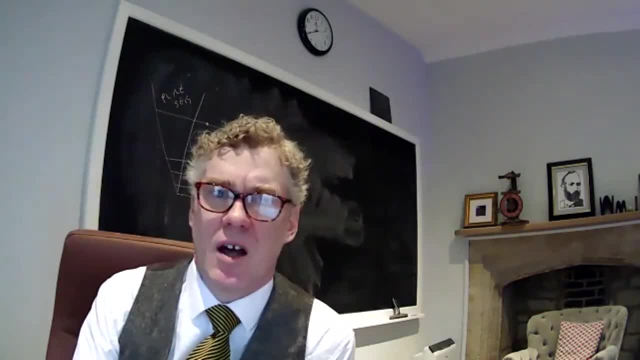 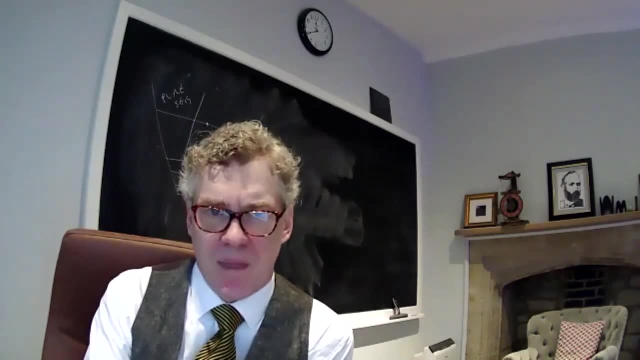 incoherent to try to provide an axiomatization of set theory using second-order logic, precisely because second-order logic itself amounts to a kind of set theory. but in the meta theory, and so today's zermelo, set theory is generally taken as a first-order theory, and we only allow 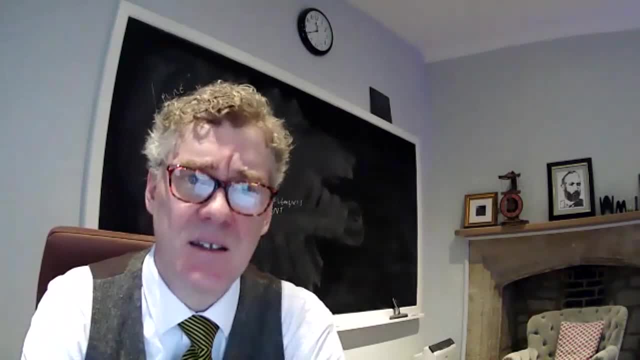 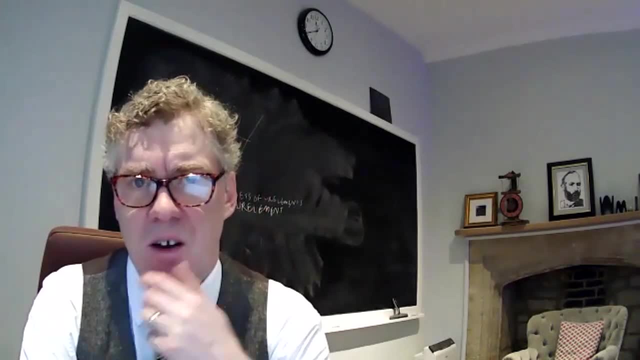 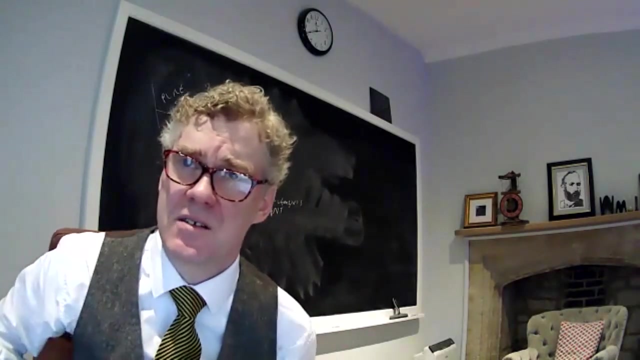 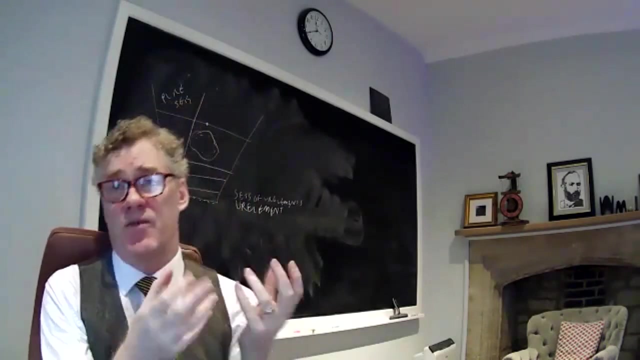 first-order expressible properties, properties expressed in the language, in the first order language of set theory itself. sometimes, mathematicians or philosophers have argued that the restriction of general comprehension to separation is a kind of ad hoc response to the russell paradox. right, so they don't agree that that russell identifies simply a simple reputation of a naive mistake. they 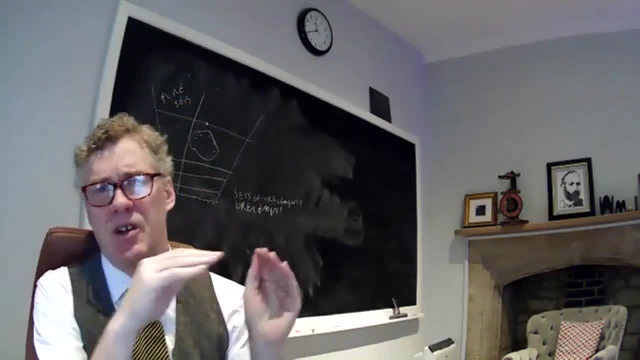 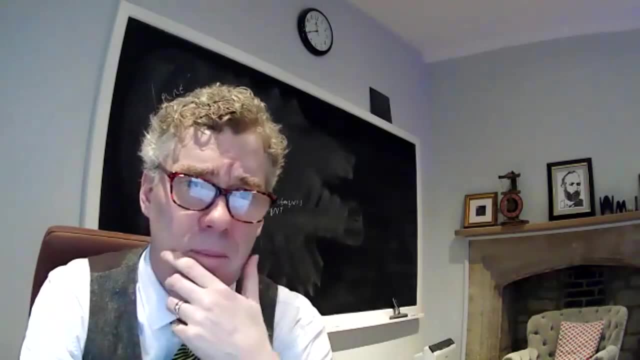 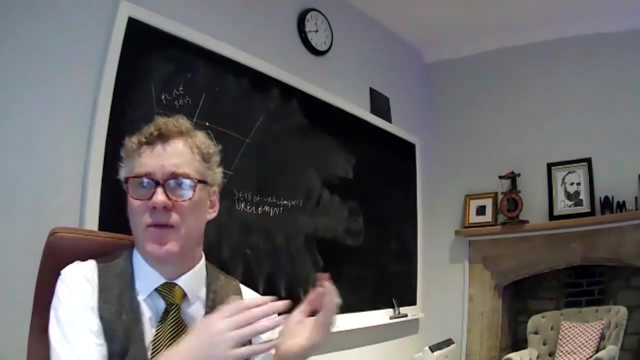 feel the pull of general comprehension, um, and they say, well, to go to separation is simply, uh, ad hoc fix and we shouldn't trust it. maybe it's still inconsistent, yeah and uh. maybe a counter argument to that um is that, uh, the, the general comprehension principle was never actually part of this cumulative hierarchy view that we had. it was. 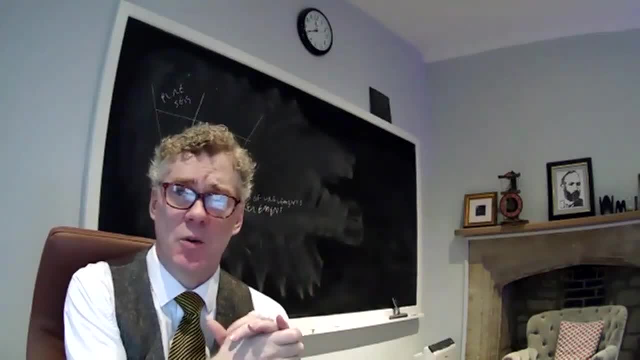 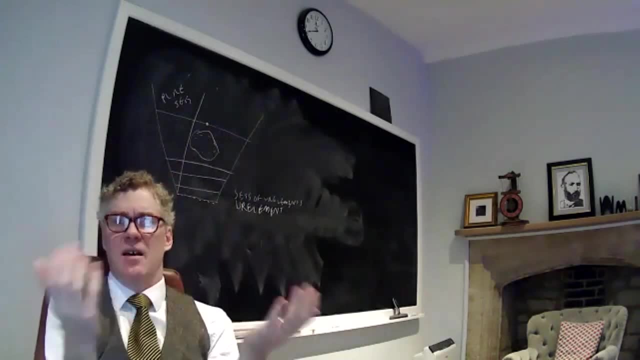 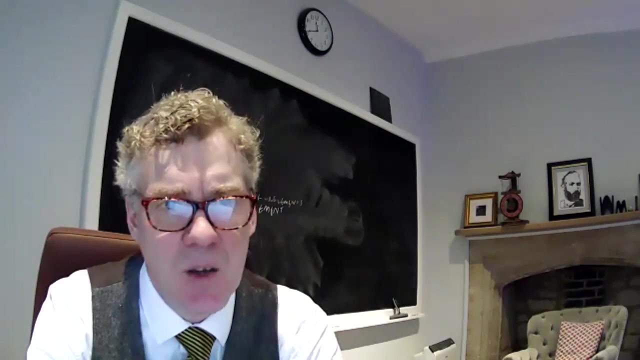 really, uh, only the separation axiom. that's justified by that view, and so the the pull that we feel towards general comprehension is really just misplaced. uh, support for the separation axiom itself, and so it's denying the ad hoc response. okay. so other people, though, um, argue differently about impredicativity, so they say um, so they they. 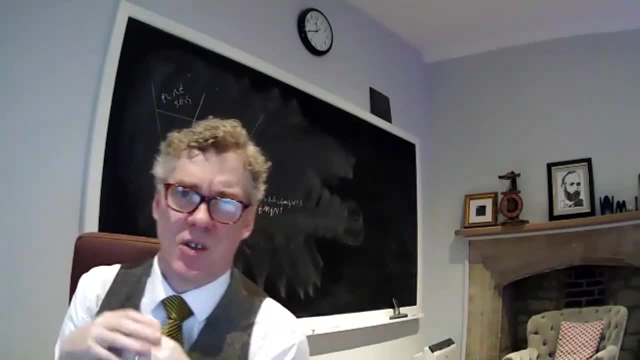 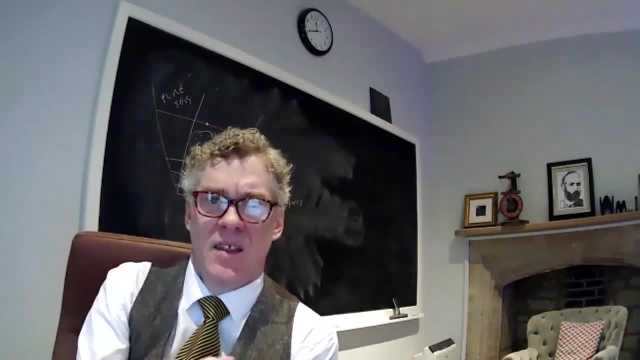 place the blame on the impredicative nature of the general comprehension principle. so a definition is impredicative when it defines an object by means of a property whose quantifiers range over a realm that includes the object being defined. okay and impredicative definitions are seen as incoherent. 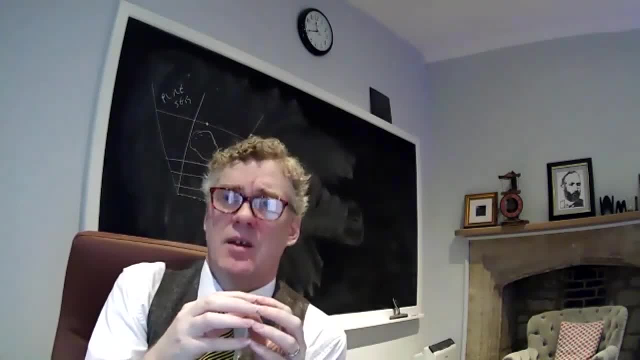 because if you're trying to define something, then it doesn't make sense maybe to quantify over a collection of some of these developments in proportion to the interpretation claim and then, over and over again, they're very different. that includes that very object that you're defining. 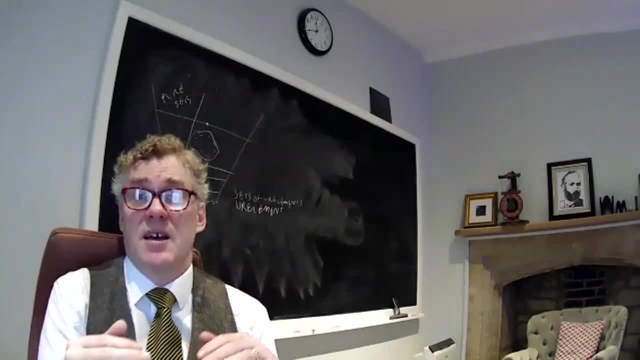 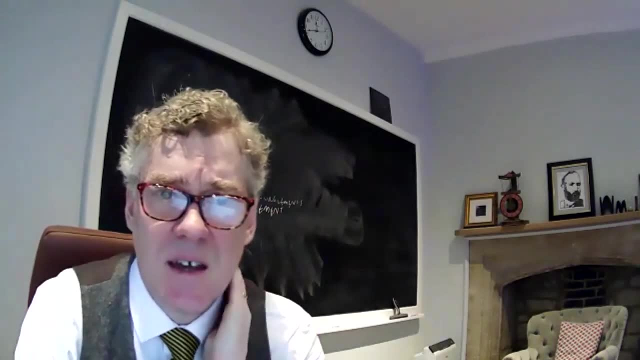 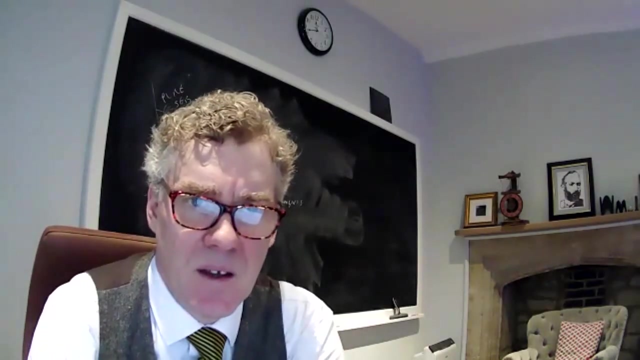 And so some people try to restrict the separation axiom to just predicative definitions instead of impredicative ones, by limiting the quantifiers or limiting the range of the scope of those quantifiers and how they might be interpreted. Okay, so it's precisely that the view. 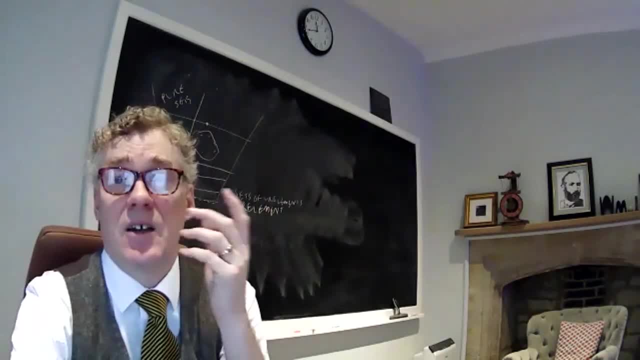 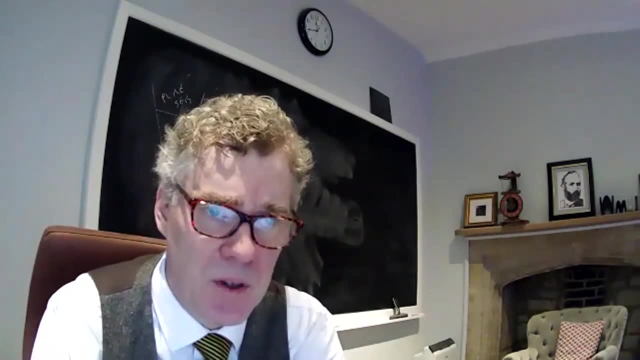 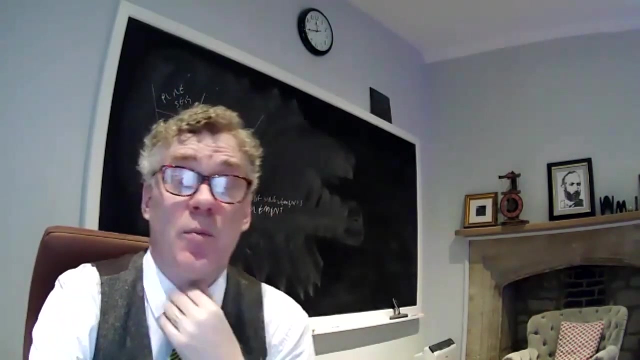 that the move from general comprehension to separation doesn't address the impredicativity objection. You have to still weaken separation further by only considering some properties. But meanwhile mathematics really abounds with routine use of elementary impredicative definitions. For example, if you take the closure of a set. 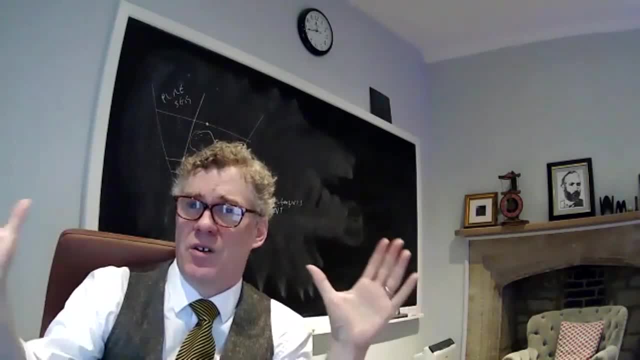 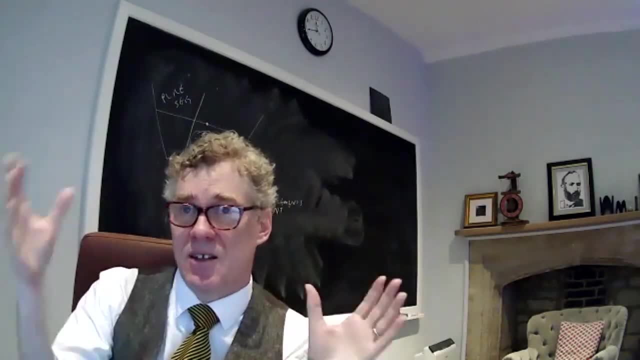 in a topological space, you can define it as the intersection of all closed sets containing that set. But that's impredicative because the closure of the set is one of those sets that you're intersecting, right? Or if you say: 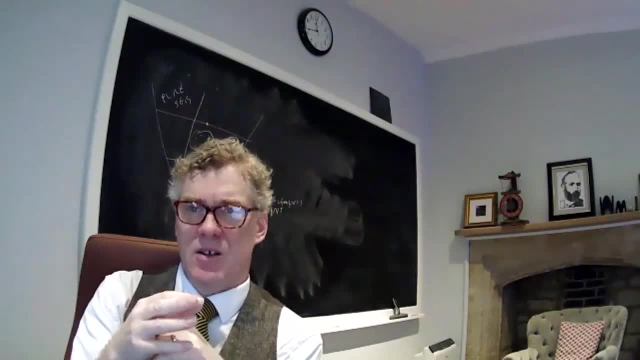 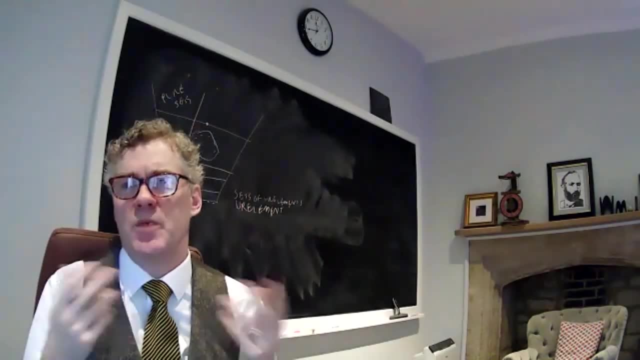 if you have a subset of a group, then the group generated by that subset you can define as the intersection of all subgroups containing that subset. But that's impredicative because the subgroup that you're defining is one of those subgroups. 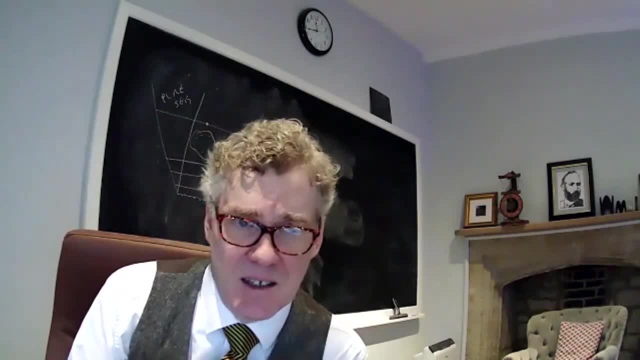 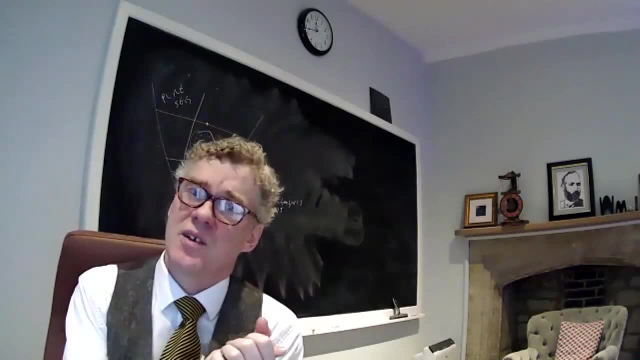 that you're intersecting right, Or even if you think about, say, defining the greatest common divisor of two natural numbers. this is impredicative. if you define it in a certain way, Okay, but in each of these cases we have a non. 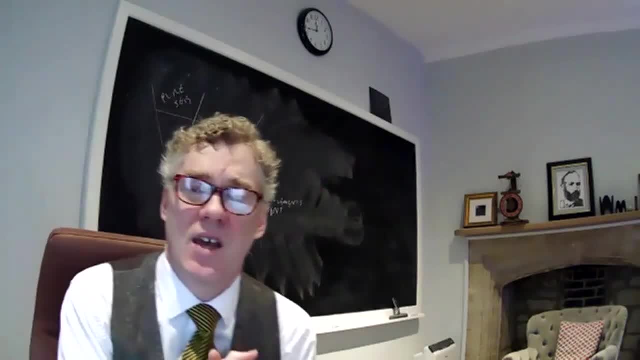 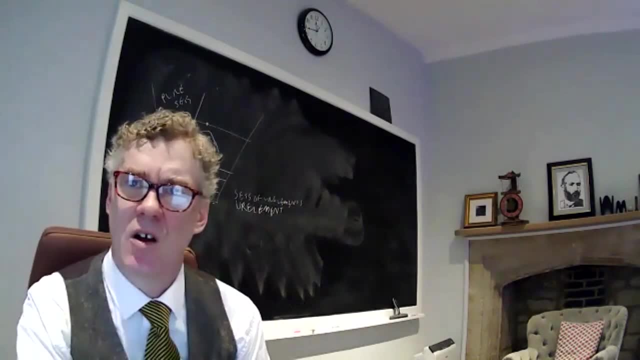 I'm sorry. we have a predicative definition, a sort of more constructive definition. In each case, the subgroup generated by an element, you can define it in terms of words and so on. And for the closure of a set, you can talk about cluster points and so on. 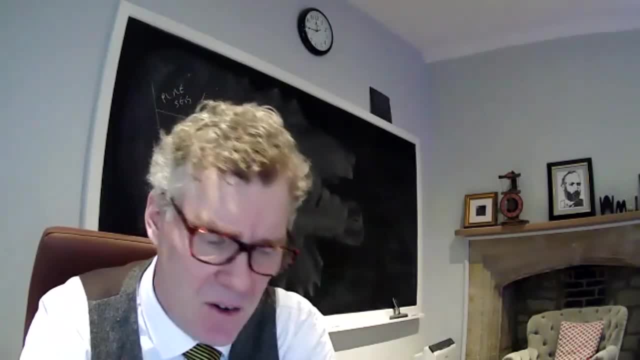 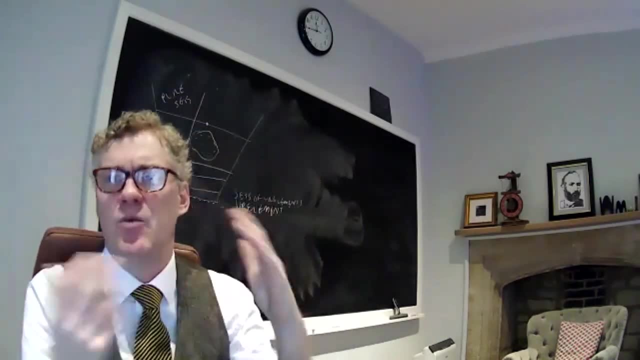 without having that impredicative nature. And so, and furthermore, I guess the oftentimes we have this top down or bottom up definition and the top down one is impredicative, but we gain mathematical insight by comparing these two definitions. 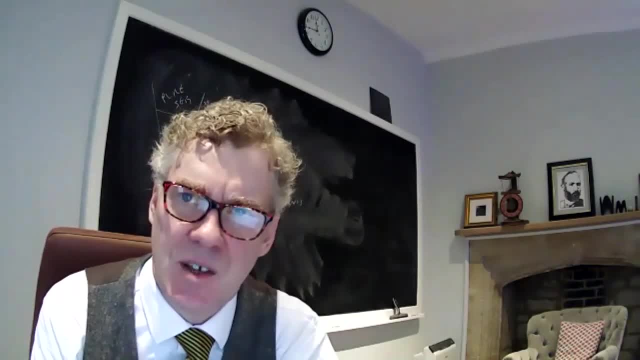 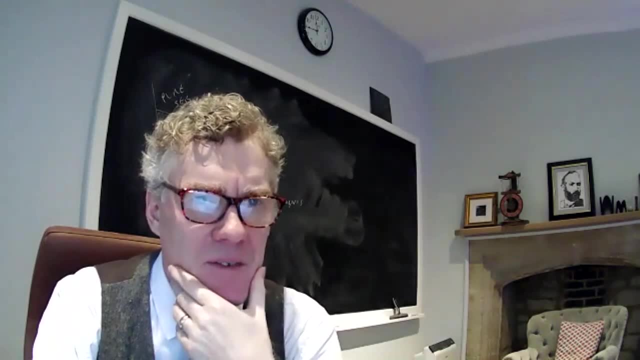 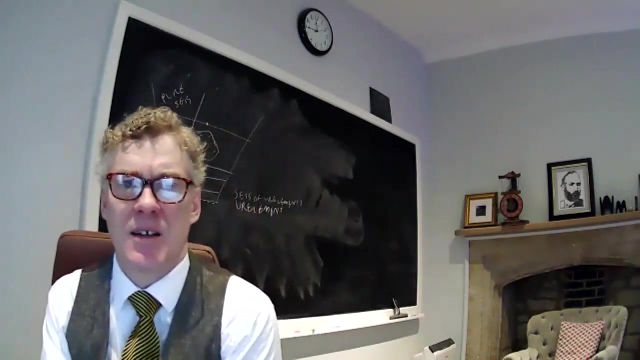 and playing off of the two different features, the natures of those approaches. All right, I want to mention that, to my way of thinking, the initial attraction of the general comprehension principle follows a pattern that sometimes occurs in logic and mathematics, And this is the pattern by which a mathematical concept 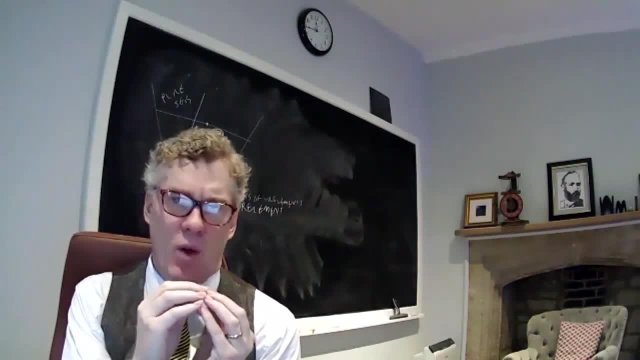 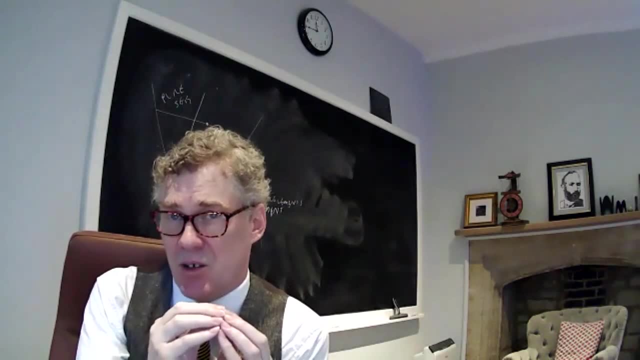 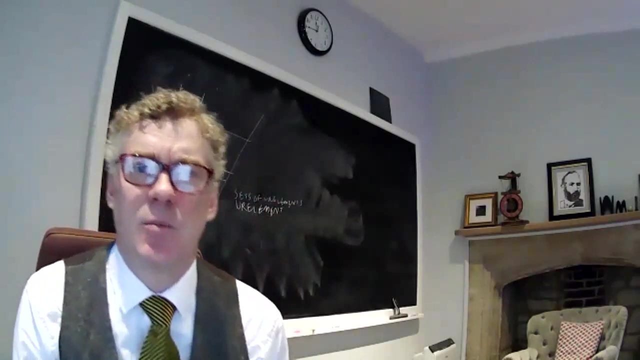 is existing and totally unproblematic when it's taking place in the context of a certain well-founded hierarchy, or each use of the concept is maybe taking a step up in that well-founded hierarchy. But when you ignore the hierarchy, then you led to paradox and contradiction. 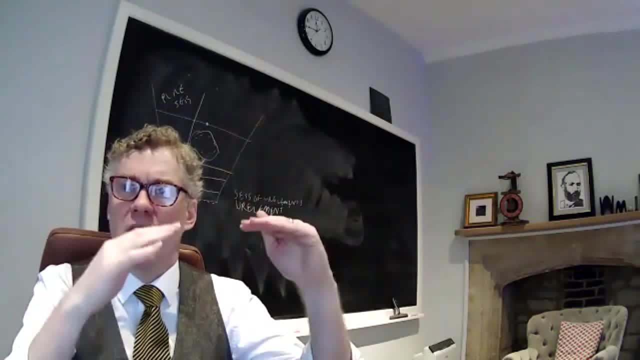 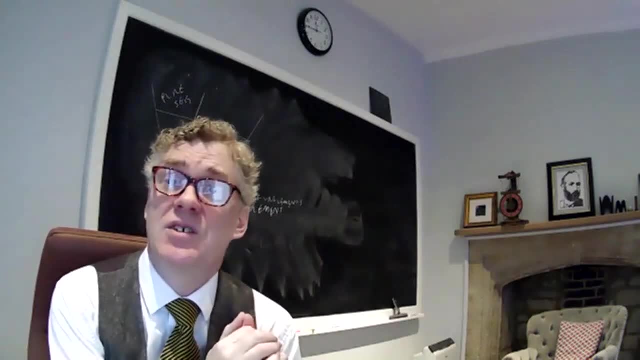 And so, for example, if we think about the cumulative hierarchy, then the sort of the version of comprehension that would be sensible in the context of that hierarchy is exactly the separation axiom. And when we ignore that context then we get the general comprehension axiom. 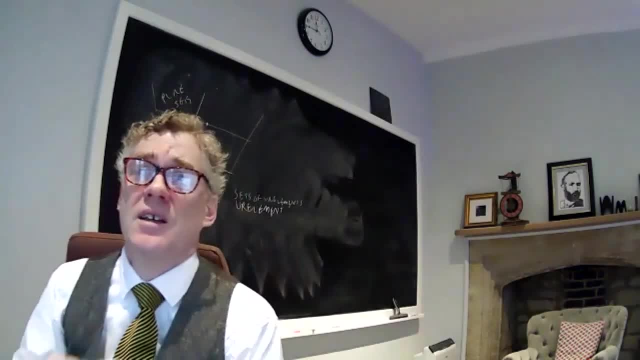 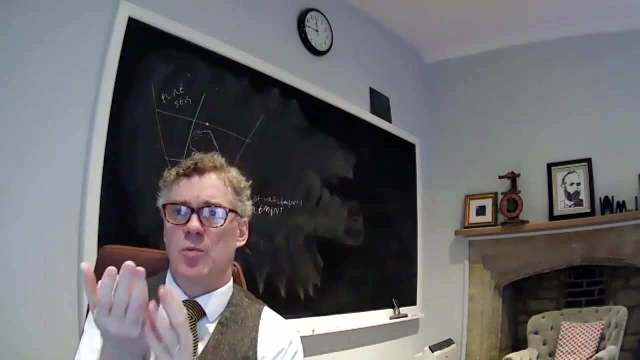 which is inconsistent Similarly in the concept of truth. So if you have any mathematical structure at all, you can always add a truth predicate to that structure, where the truth assertions are being made only about the language in the original structure and not in the language with the truth predicate. and once you do, 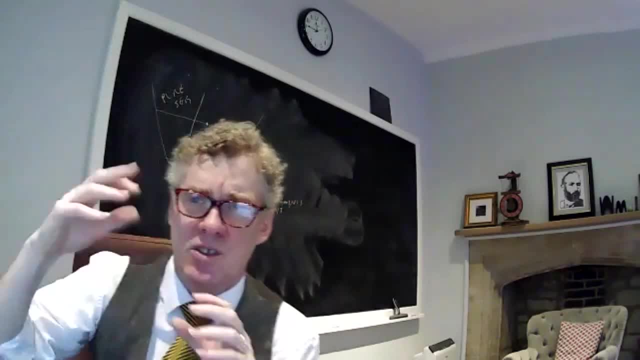 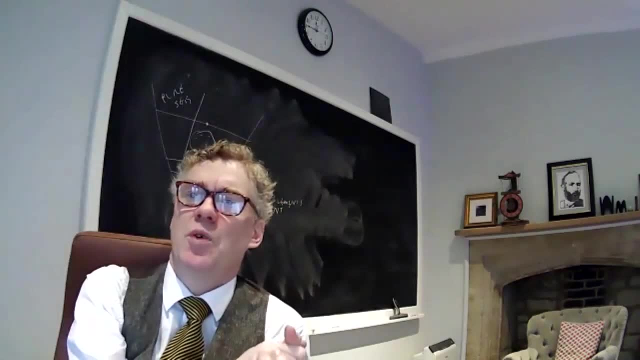 it once, you can do it again and have a truth about truth and truth about truth about truth, and so on. you can have iterated truth predicates and all of that is completely unproblematic when it takes place in a hierarchy of iterated truth predicates. but the paradoxical nature of self-referential 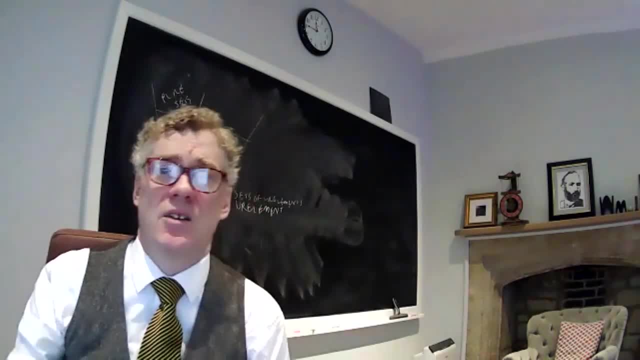 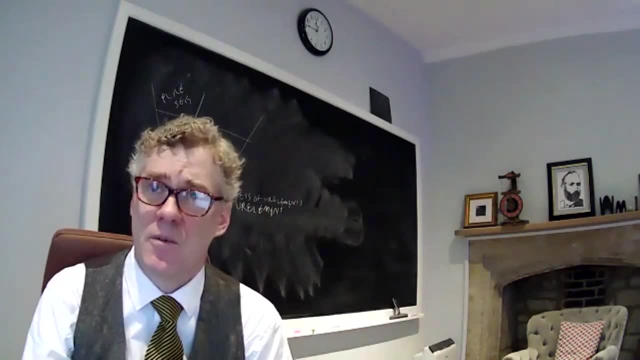 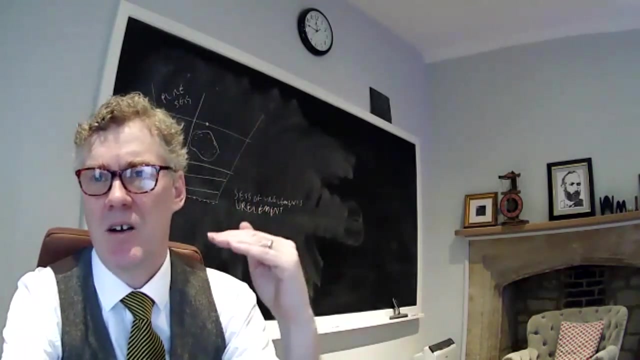 truth predicates comes when you ignore the hierarchy and you want to apply the truth predicate to assertions in the language with the truth predicate itself, and then you can form paradoxical assertions like the liar, the statement, this, this sentence is false, okay. so we need to pay attention to these well-founded hierarchies and not fall into this trap uh of uh of ignoring them. 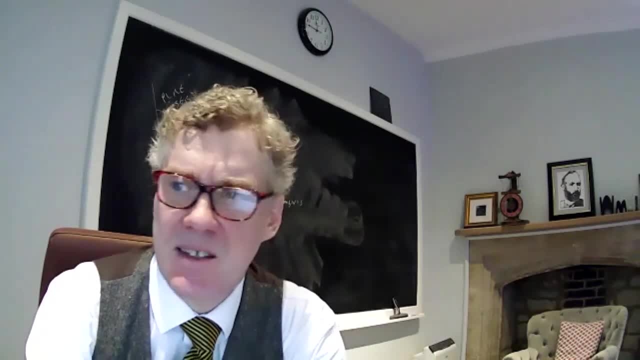 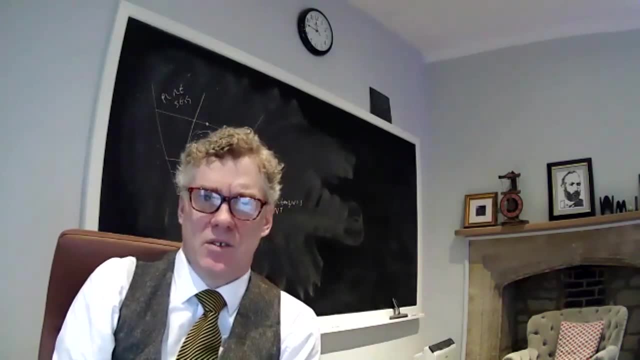 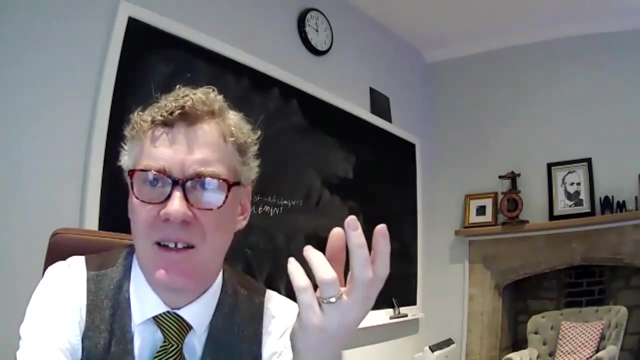 so let's talk about some more axioms. the axiom of extensionality, um, so it's uh, sets have the same elements, uh, uh, if, and only if, they're equal. so two sets have the same elements if, and only if, they're equal. so this is maybe a core set, theoretic idea, uh, but it turns out. 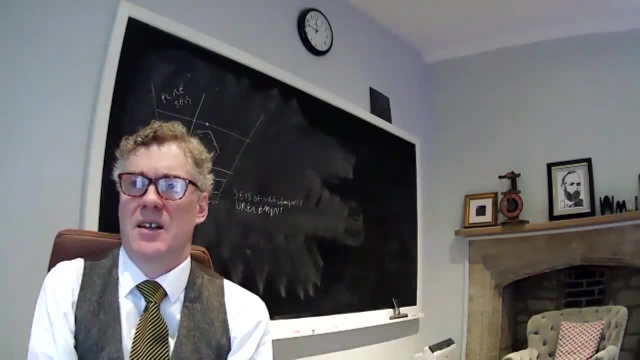 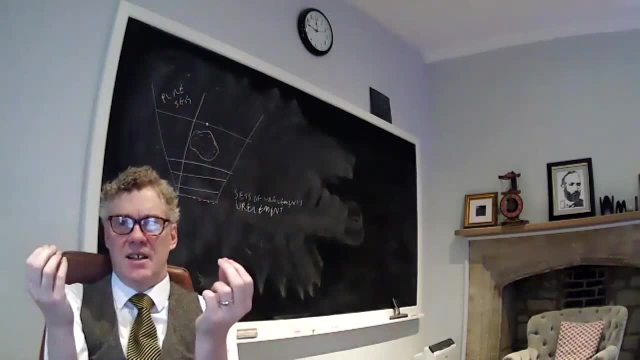 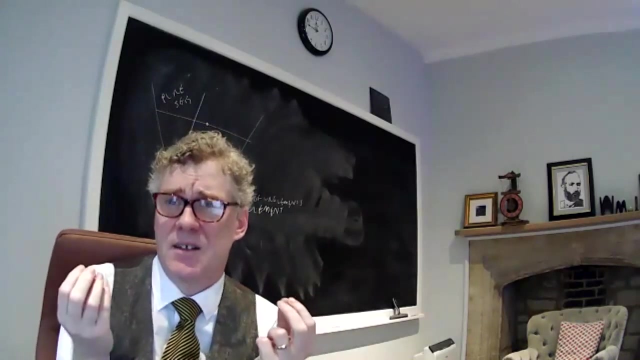 actually you can undertake quite a rich set theory without extensionality axiom, without the extensionality axiom, um. and so if you drop extensionality, then you might have two sets that have the same elements, but they're not identical as mathematical objects, and so you would want to say, well, let's say that they're equivalent, uh, um, and that would be fine as far. 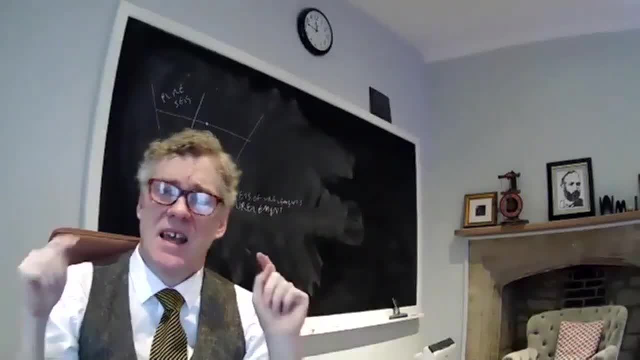 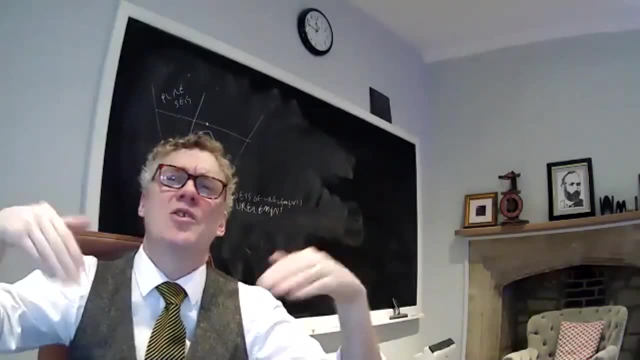 as it goes, except then maybe you have two sets and they don't have the same elements, but all of their elements are equivalent to elements in the other set. so we would want to say, well then, those two sets are are also equivalent, a sort of next level of equivalence, and ultimately, you're, you can be. 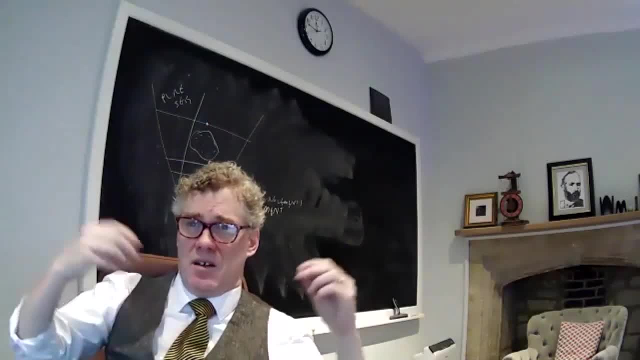 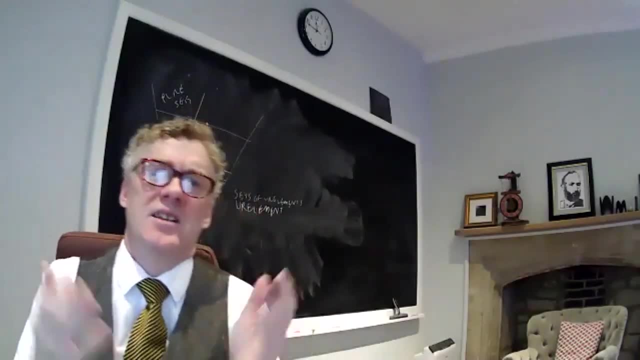 led to a notion of bisimulation, by which a sort of correspondence of sets, so that their elements are also corresponding, you know, and in this way you can recover a kind of version of set theory with extensionality, even if you didn't have a set theory, but you can recover a kind of version of 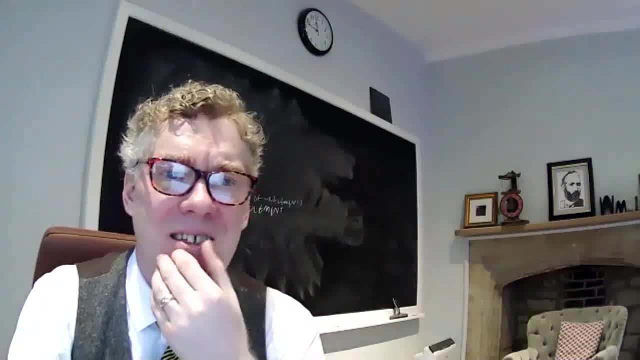 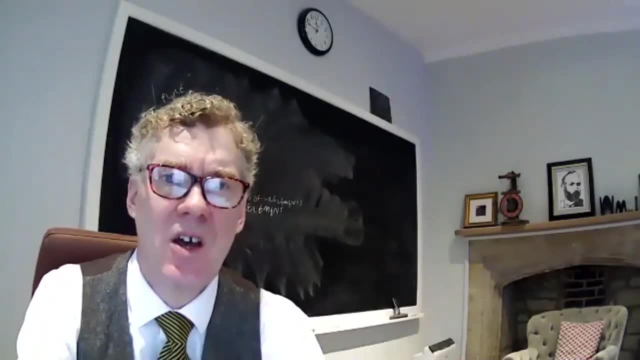 set theory and have it to begin with. so there's many other axioms of set theory. there's the axiom of pairing, which says: for any two- uh, for any two objects, you can have a pair consisting of just those two objects. or the union axiom says: for any set of sets, you can make the union of all those. 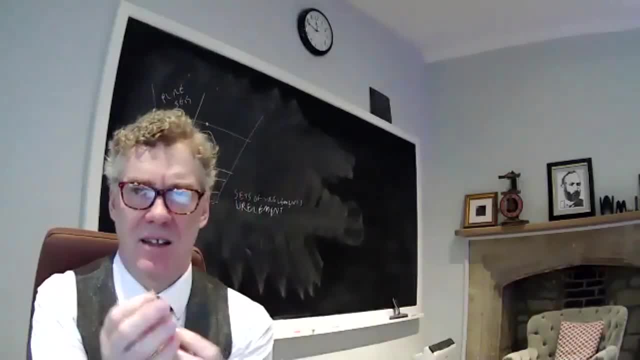 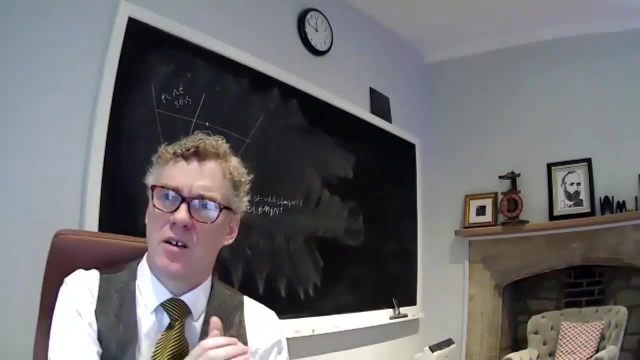 sets, or the power set axiom says: for any set you can take the set of all subsets of that set. there's the axiom of foundation, or regularity, which is expressing the idea that that cumulative hierarchy is well founded um. there's also, importantly, the replacement axiom, which we'll 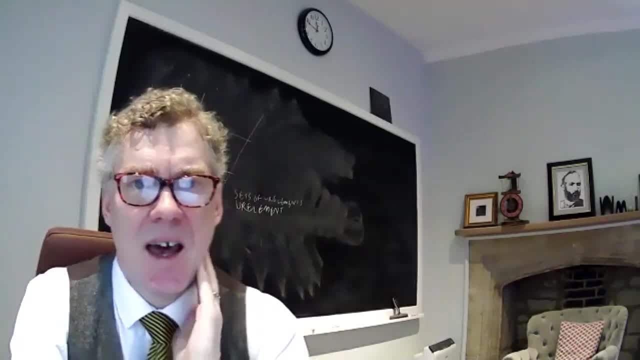 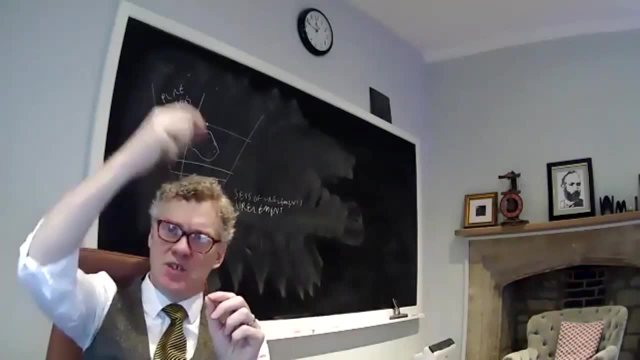 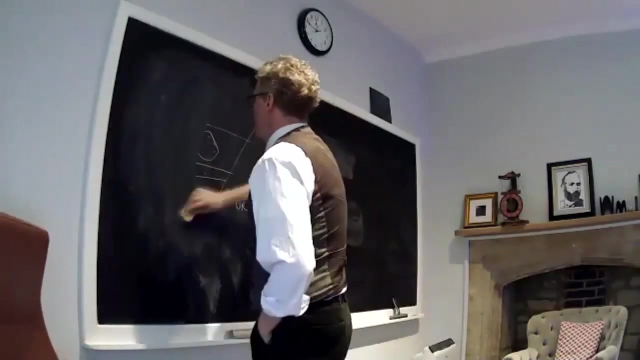 talk about in a little bit. but it was missing initially in zermelo's axiomization but was added by frankel. so the replacement axiom says: if you have a set and everybody in that set has a unique object satisfying some property, then we can take the collection of those objects. so for example, 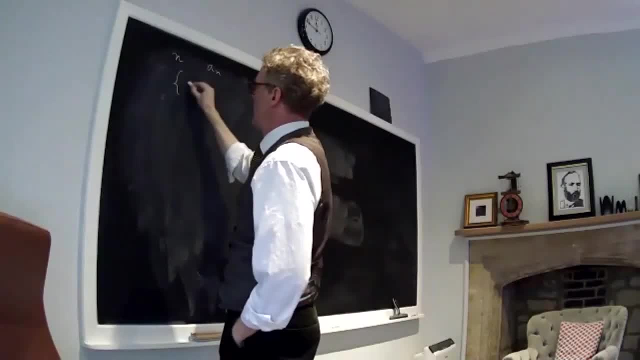 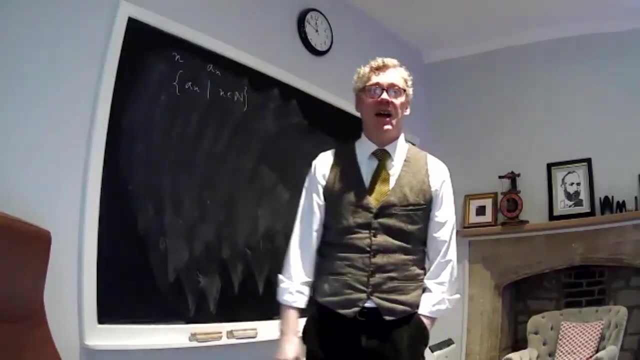 maybe you can. for each natural number n, you can define an object, a sub n. then you want to know that the set of a sub n such that n is a natural number, and then you want to know that the set of a sub i is the axiom of replacement. 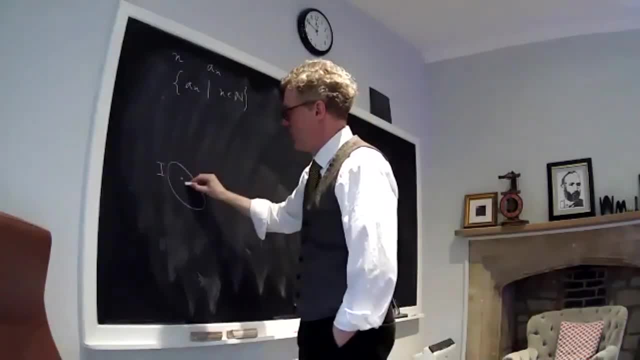 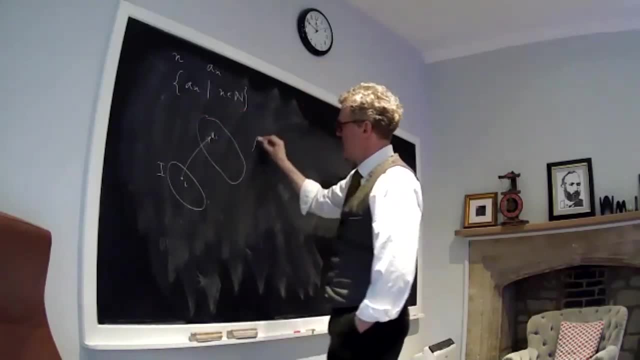 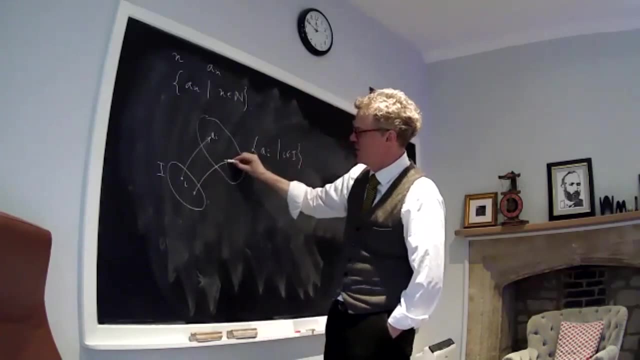 i mean in the general case. it says: if you have a set i and you know for every element, uh i, that there's some object, a sub i, then you can collect the set of all a sub i, such that i is in i, then this will exist. as i said, you're replacing each object with uh um, with the defined object that. 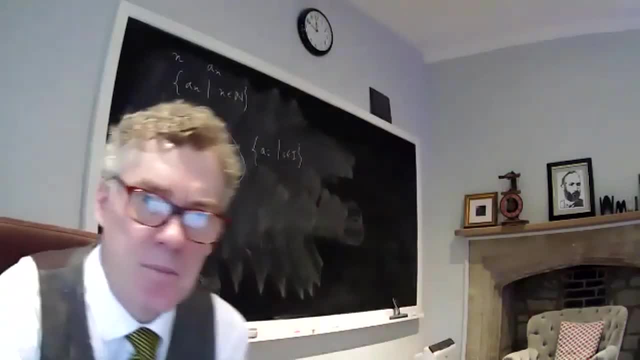 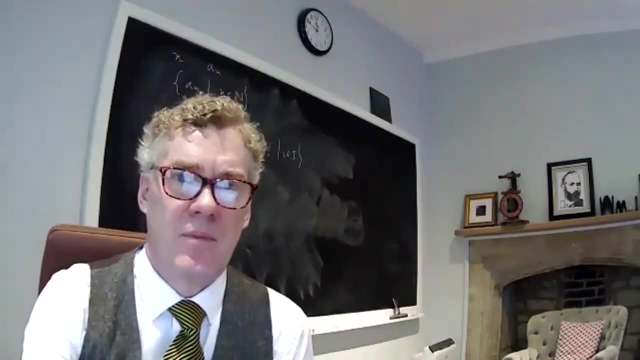 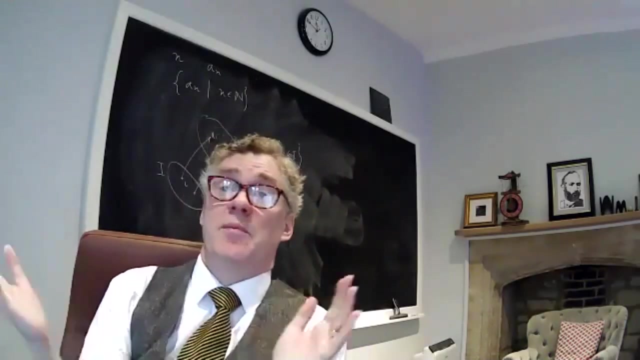 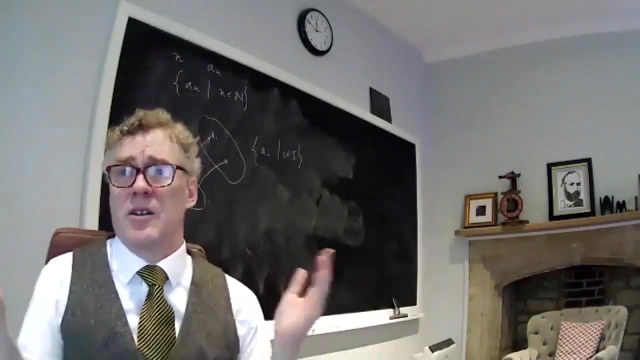 has the other property. that's the axiom of replacement. so this is very important for an argument that we gave um uh in week three, namely concerning the number of infinities. so we argued at that time that there must be many infinities, infinitely many, in fact, the, the there are more infinities than any given infinity. so in particular there 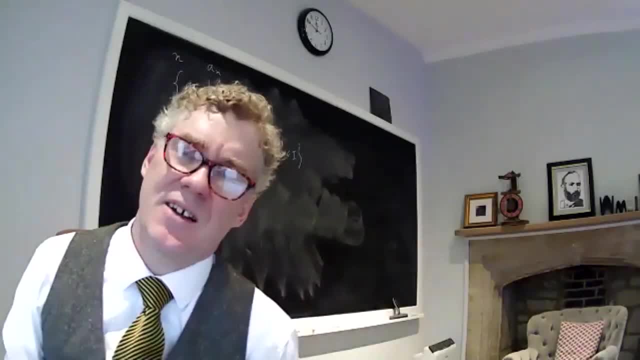 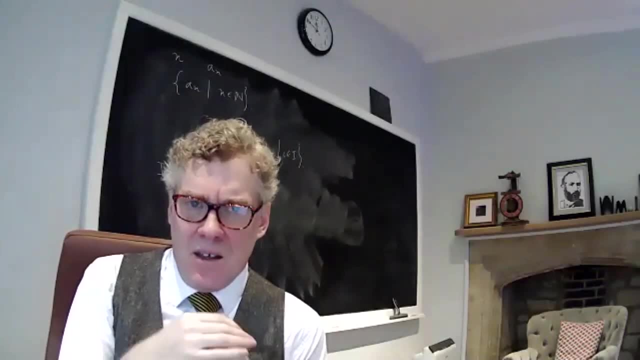 are uncountably many different infinities and so on. but actually this argument required the replacement axiom to do it, because, for example, suppose you want to take the set of a sub n and you want to take if you prove that the the olive ends. so we have all of zero, all of one, all of two. 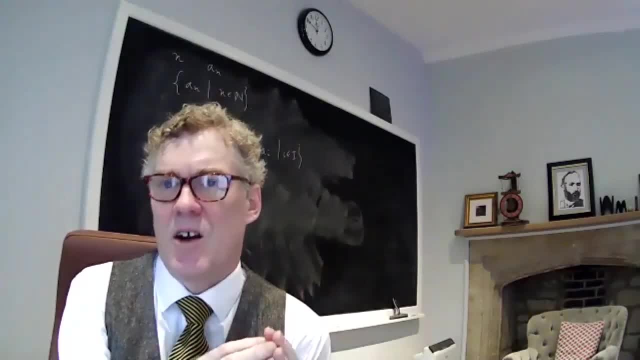 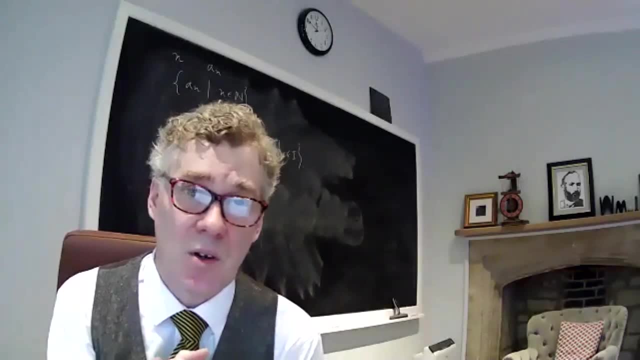 and so on. the olive hierarchy: these are the the smallest, infinite cardinal, and the next one and the next one after that, and so on. but maybe we want to make the set of all the olive ends the set of all of n, where n is a natural number. and does that set exist? well, that's exactly an instance. 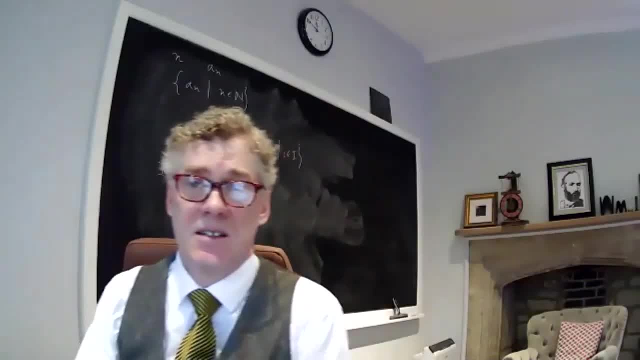 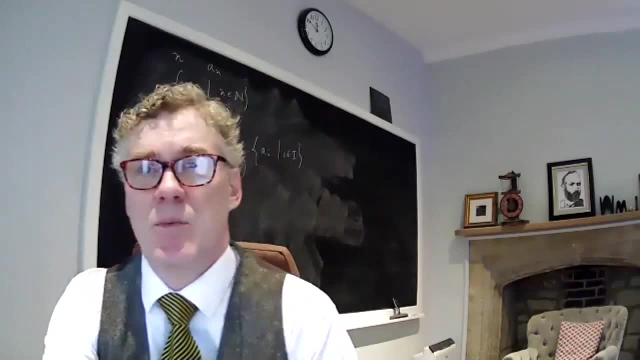 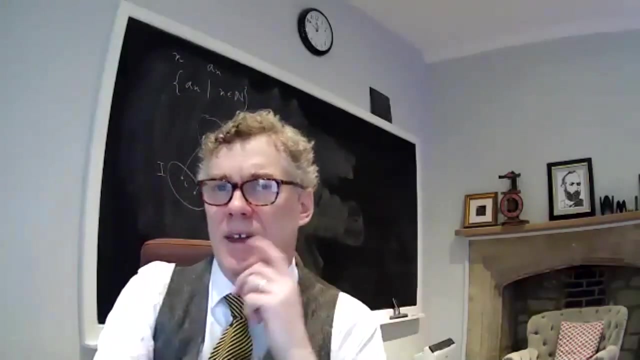 of this replacement axiom that i said, and frankel had observed that you didn't seem to be able to prove it from zermelo's original axioms that didn't have the axiom of replacement, and this is why the axiom of replacement was added. okay, well, how. how could you prove, though, that in fact, it's not provable that there are? 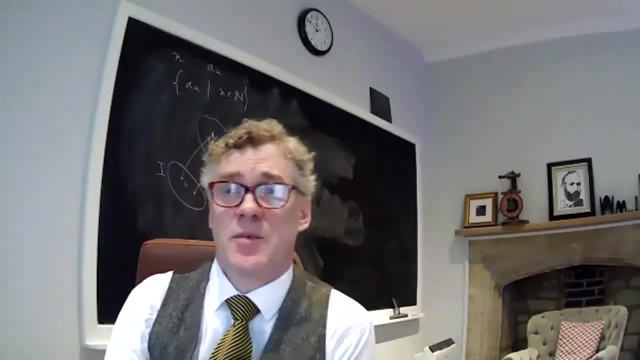 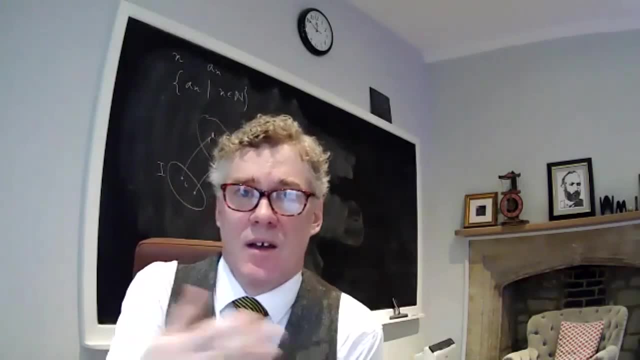 uncountably many different infinities just in zermelo's axiomization. and one way to do that is, i mean, this is a sort of metamathematical claim, the claim that you cannot prove that something in the theory. so so the the claim i'm making is that in zermelo theory, 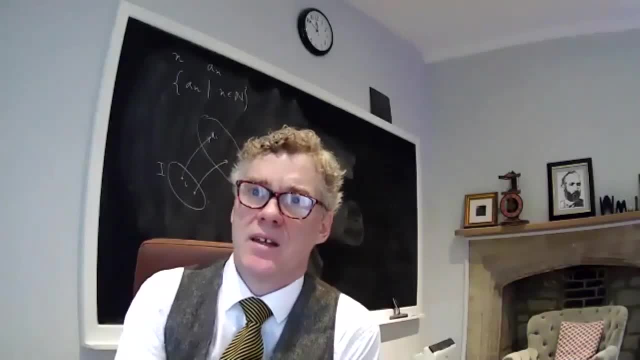 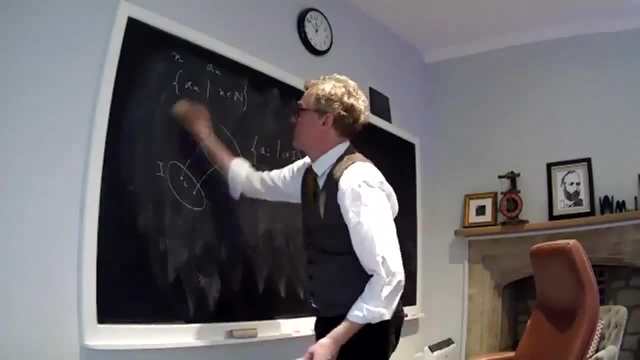 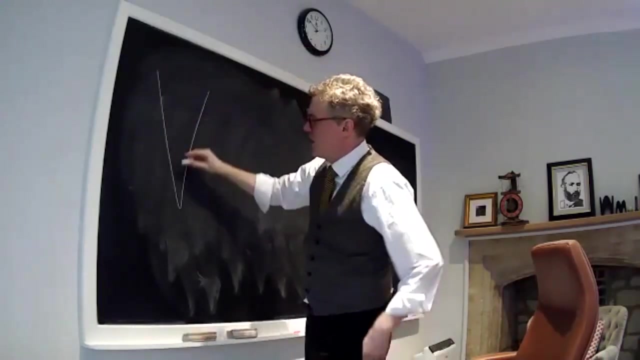 without the axiom of replacement, we cannot prove that there are uncountably many infinities, and the reason is that we can make a universe, we can make a model of zermelo's set theory in which that statement isn't true. so if we think about the cumulative hierarchy, so this: 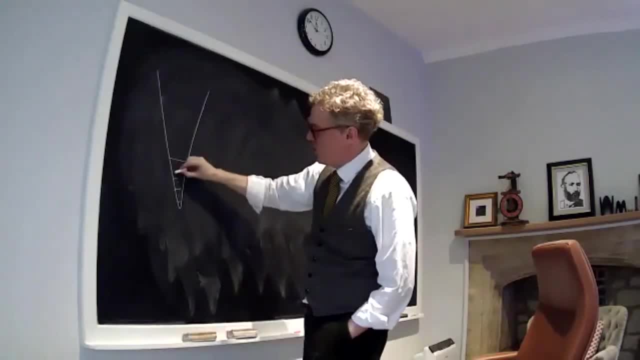 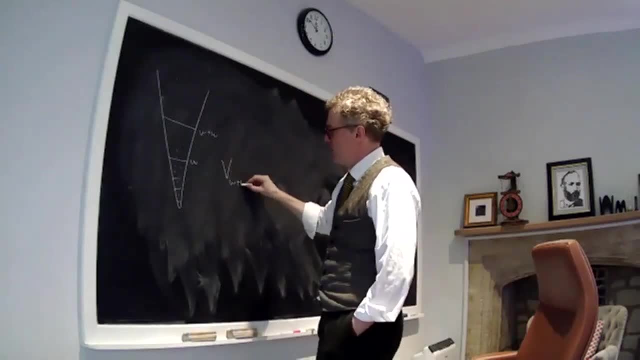 these are the the stages of the hierarchy. if we go to omega, then those are all finite sets up to stage omega and then we continue on up to stage omega plus omega. so i'm proposing to look at omega plus omega. so this is the set theoretic universe cut off at level omega plus omega. 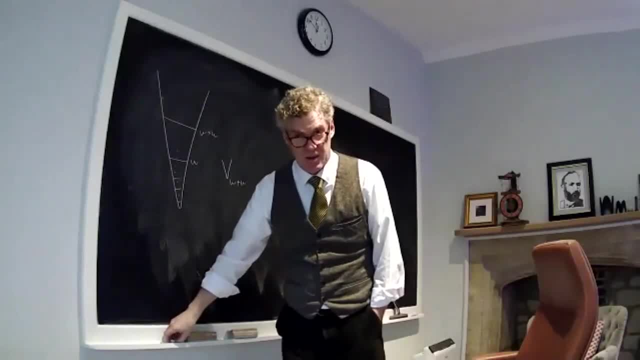 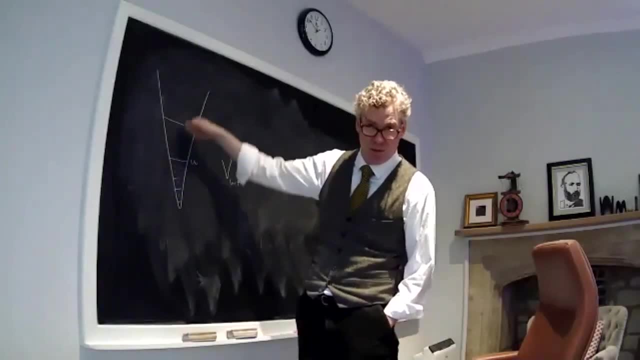 then it turns out that this is a model of all of the zermelo axioms. it's not a model of the replacement axiom because we can associate each end with the ordinal omega plus n but we cannot replace and make the set of all those omega plus n's. but it models all the other axioms and one can. 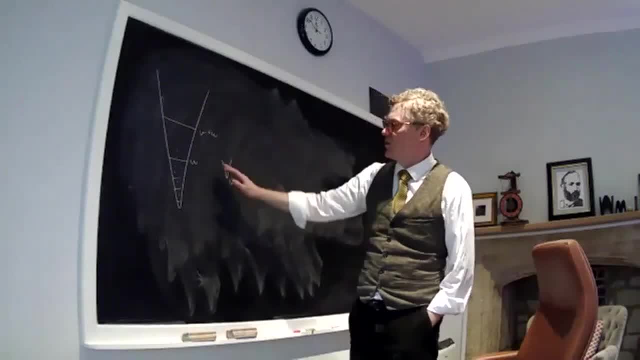 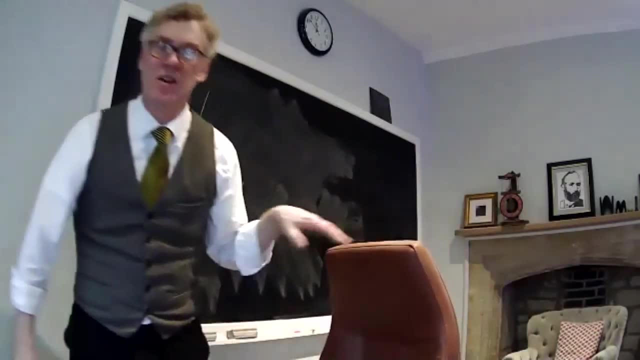 argue that if you start with the, the right initial universe, then this model of set theory will not have more than the set theoretic universe- and that's why it's called the set theoretic universe- and the olive ends existing as infinite cardinals, there will be only countably many. 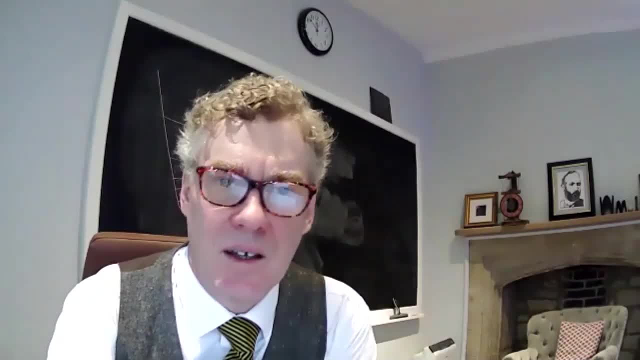 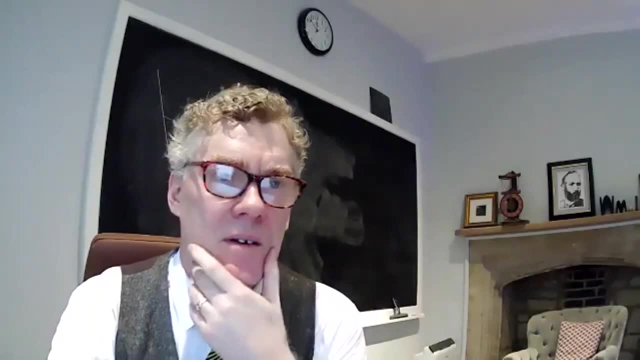 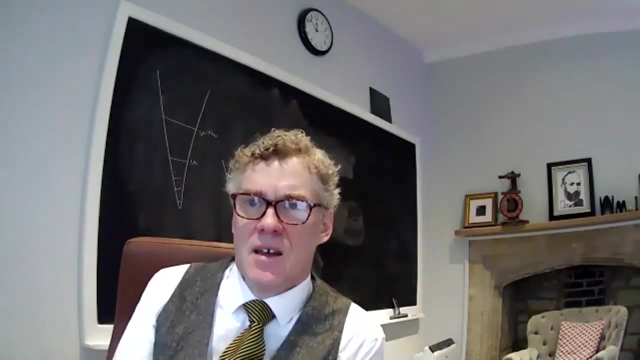 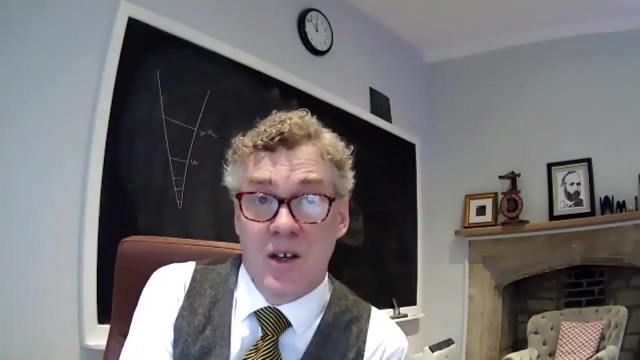 infinite cardinals in that universe. okay, if, for example, we have the generalized continuum hypothesis there. okay, we'll talk about that a bit more later. so let's move on to the axiom of choice. so zermelo formulated his axioms in 1908 because he was defending his 1904 theorem, in which he had proved that the real numbers can. 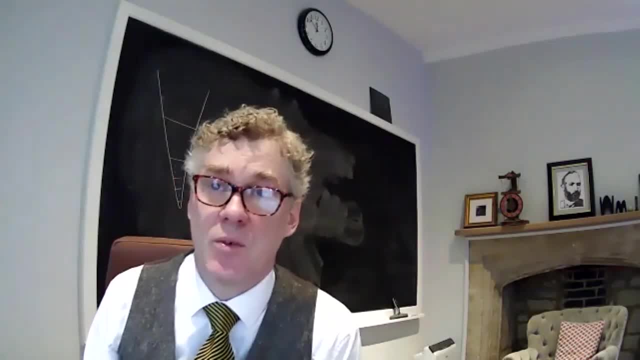 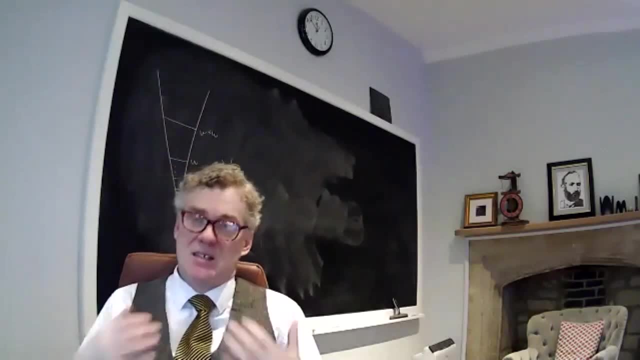 be well ordered and indeed any set of any set can be well ordered. so this was very controversial and it was attacked, and he presented the zermelo axioms in order to make make explicit what are the fundamental assumptions that he was making in his proof of the well-ordering theorem. 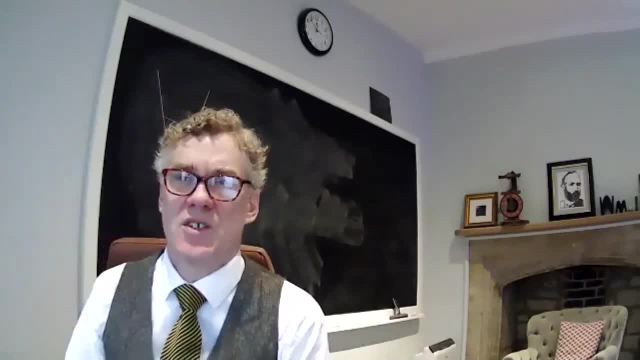 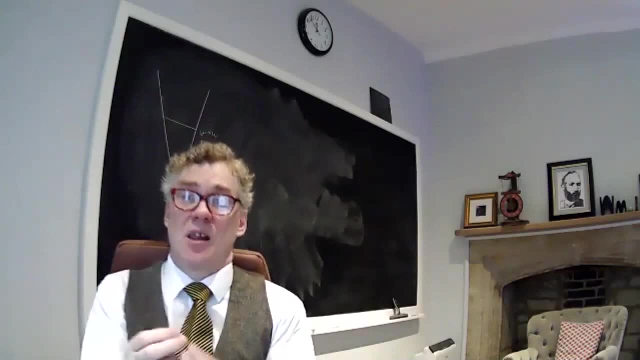 so. so the well-ordered theme says that any set has a well order. what's a well-order? it's a linear order of the set, so that every non-empty subset of the set has a least element. so there's a least element overall and the next least one, the next least one, the next least one. 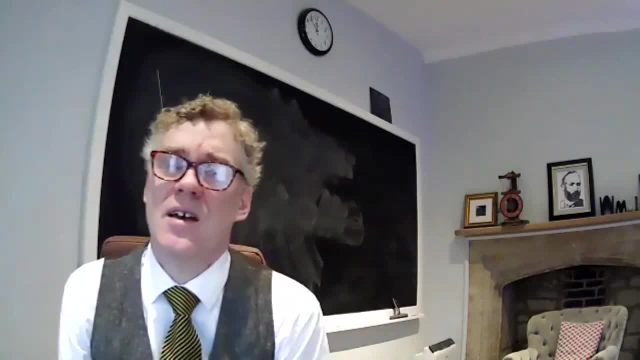 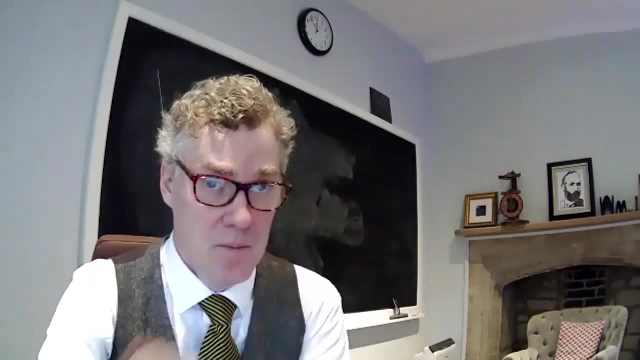 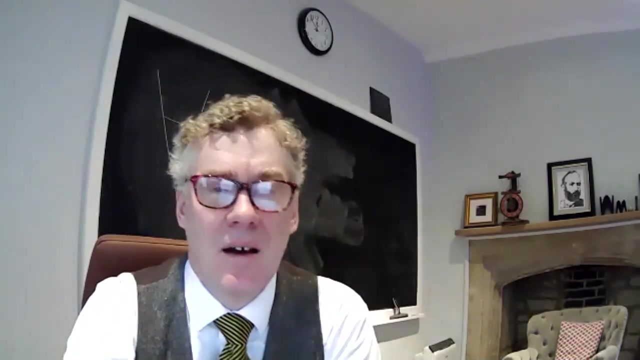 and so on, and then there's a least one that's after all those and so on, and so this is the nature of a well order. so the order type of any well order is an ordinal. so now, the problematic part of the well-order theorem was that it's difficult to imagine what a well-ordering of 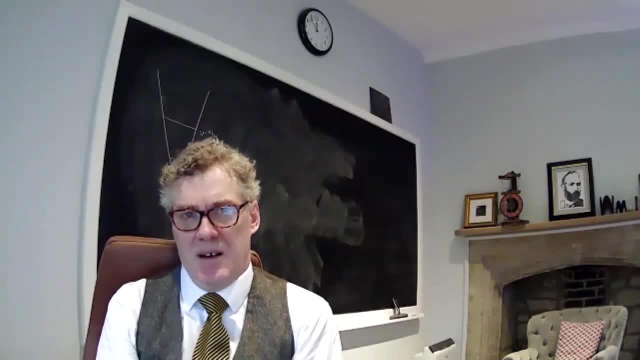 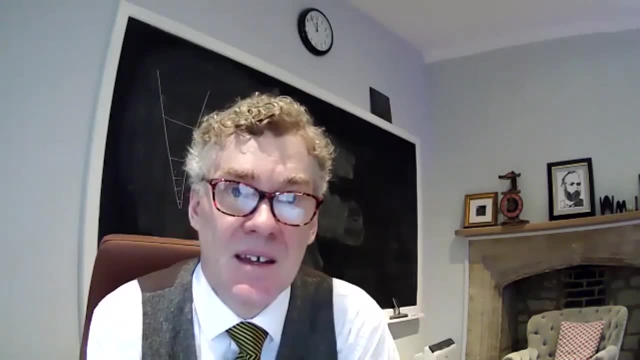 the real numbers would look like. so it doesn't seem possible to define one explicitly, so should we believe that there is one? so i mean, the question of whether you can define a well-ordering of the real numbers is not quite the same as the question of whether there is one. 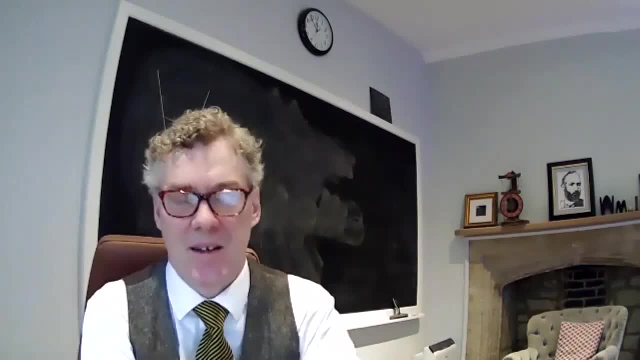 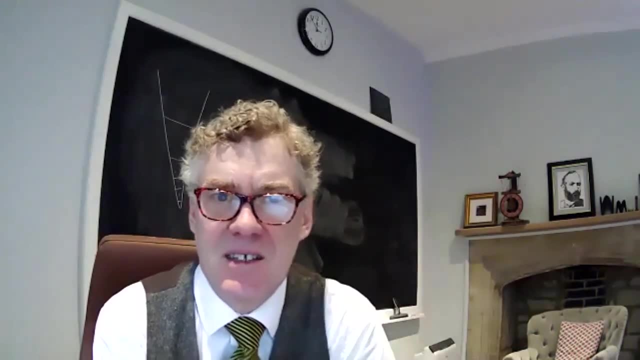 and it's a consequence of the axiom of choice that there is one. so okay, so let's let's discuss it more specifically. so the axiom of choice is the assertion that for any set of non-empty sets, then there's a choice function on the set. so that's a function. 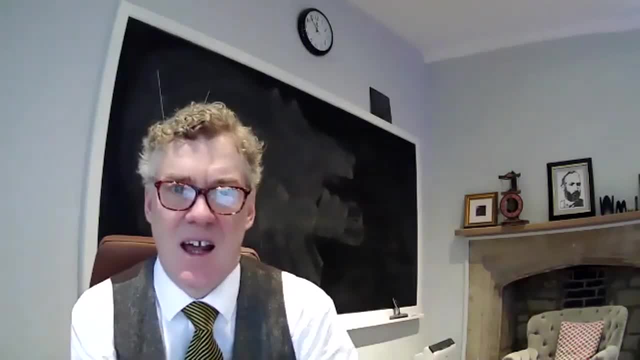 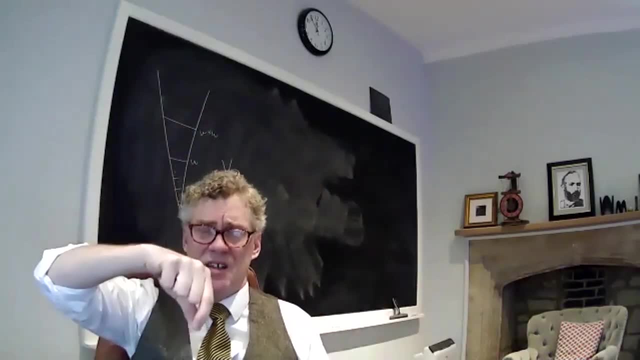 that whose domain is the original set, so that f of x is an element of x for every element of the set. so if you have a bunch of non-empty sets, then there's a function that chooses an element of each one of them. okay, that's why it's called the axiom of choice. this: 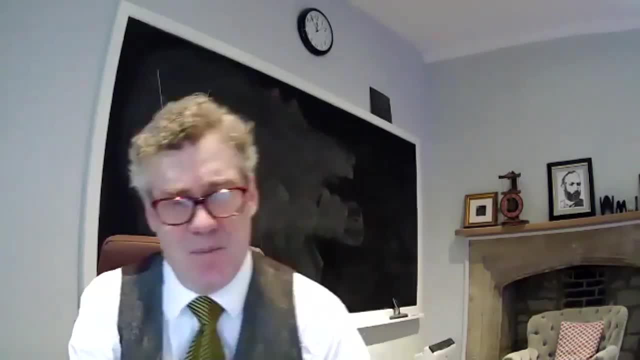 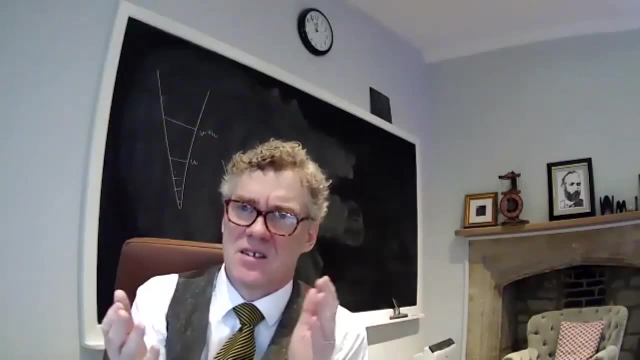 function is sort of picking and the this axiom is fundamentally different from the other axioms of set theory, all the other axioms of set theory, the union axiom, power set, and so on. it's saying it's making set existence assertions for sets that have a property that is sort of defined by. 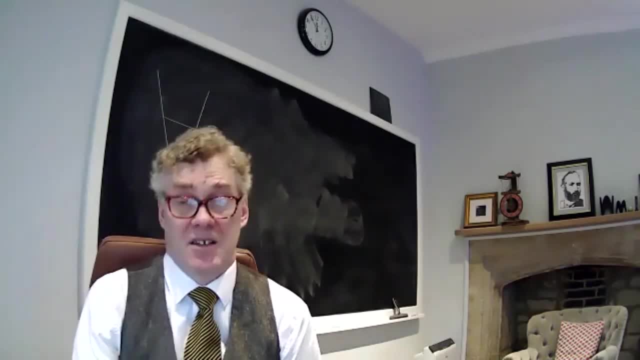 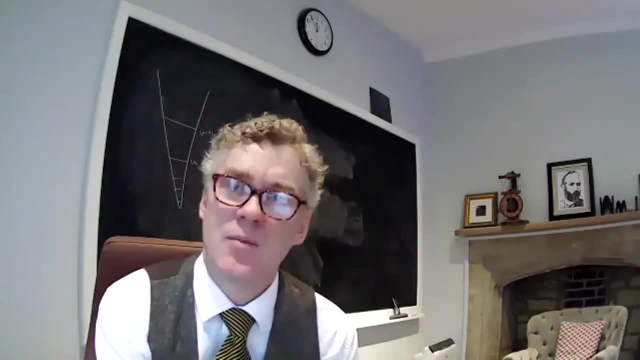 the set. so, of course, these are the most common features that are expressed in the axiom itself, and they're unique. there's only one power set, there's only one union set, there's only one pair set, and so on. there's only one subset consisting of exactly the elements with a certain property. 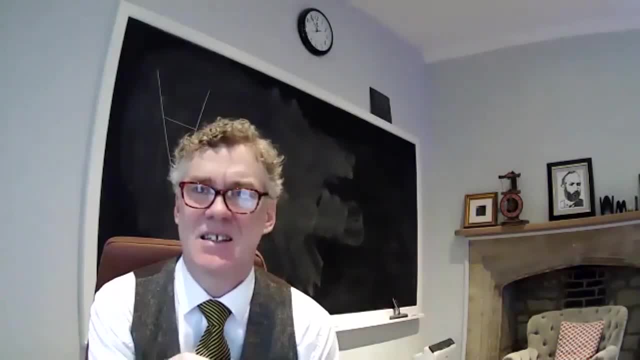 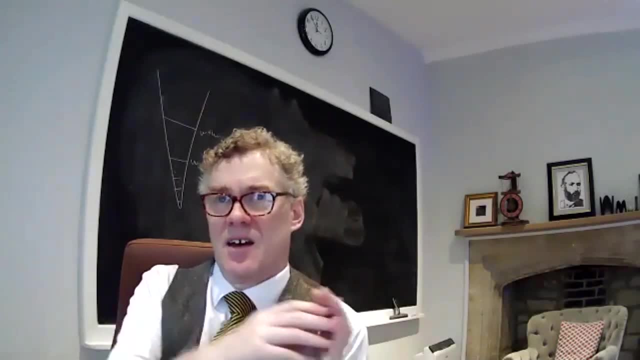 but the axiom of choice is not picking, it's not identifying or it's not making a set existence claim for a particular set. it's saying there is a way of choosing. but there's a lot of ways of choosing. in most cases, if there's one, that's going to be many typically, unless all the elements of the. 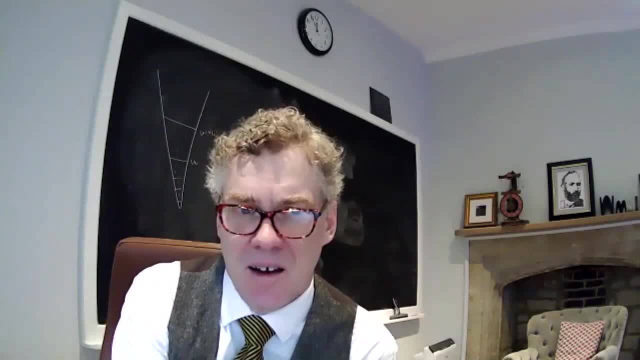 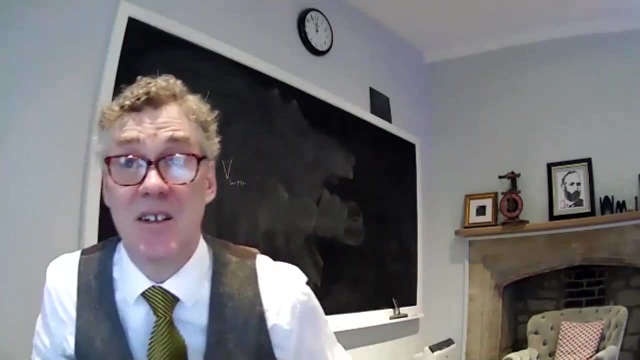 that are just singletons. And so it has a fundamentally different character, because it's telling you there is this way of picking, but the axiom doesn't tell you how to do it or even what the nature of that picking is, except that it is a way of picking an element from each set. 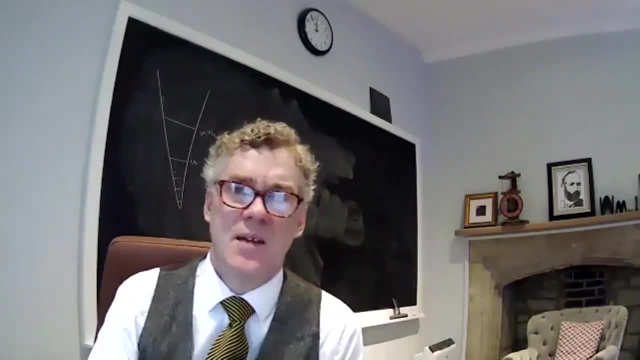 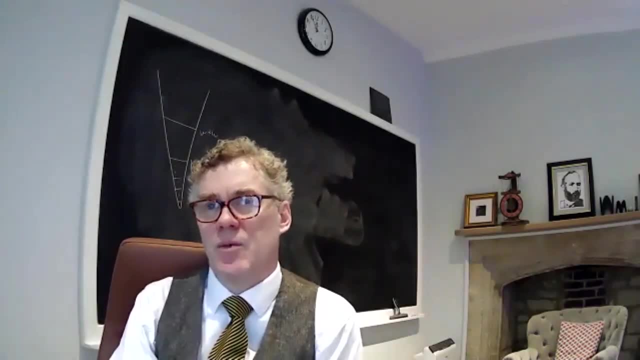 So let me illustrate this by giving this common example. Suppose you have infinitely many pairs of shoes, And so we consider each pair of shoes as one of the sets in our collection that we wanna pick. But then there's a choice function, because I can pick for each pair. 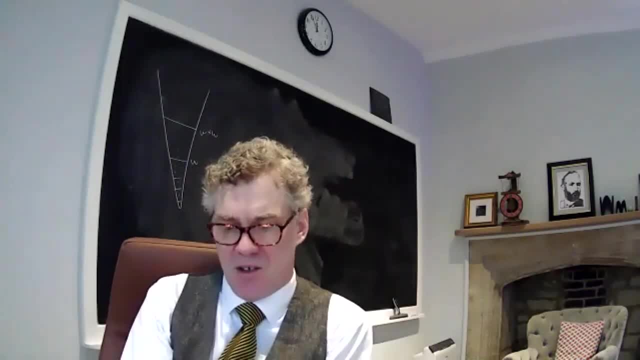 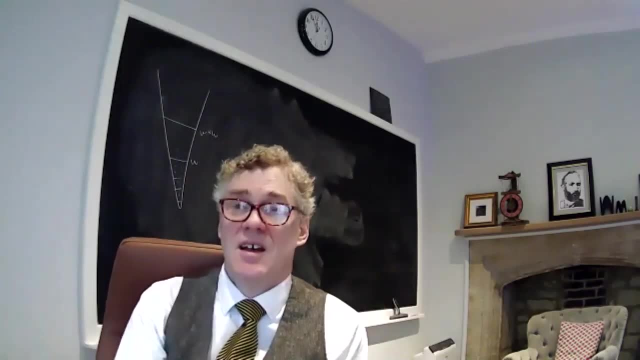 I can pick the left shoe right. If we assume that each pair of shoes has a left shoe and a right shoe, then I can have a choice function that always picks the left shoe, Or another choice function, say, that always picks the left shoe if the shoe has laces. 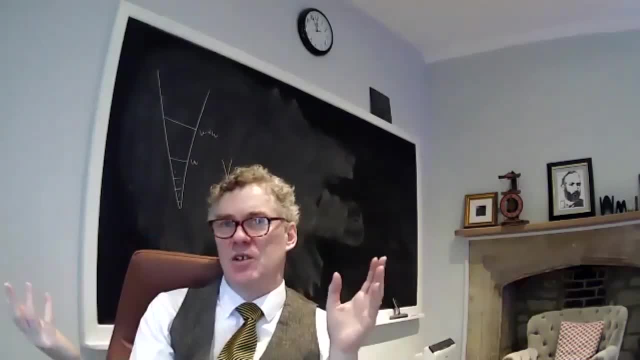 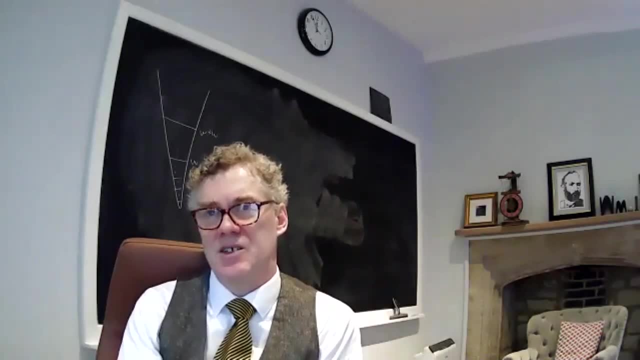 but if it doesn't have laces, then it picks the right shoe. That's a different choice function. There's a lot of different choice functions. And now suppose that you have an infinite collection of pairs of socks. okay, And within each pair, 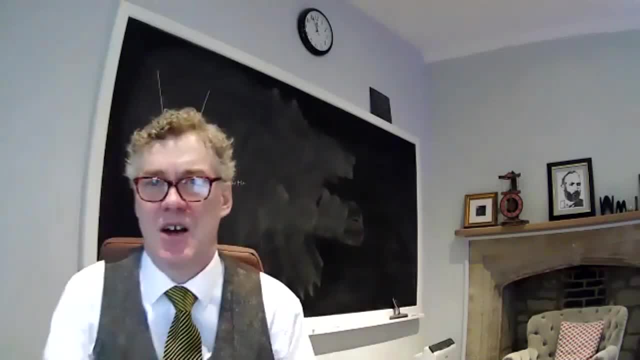 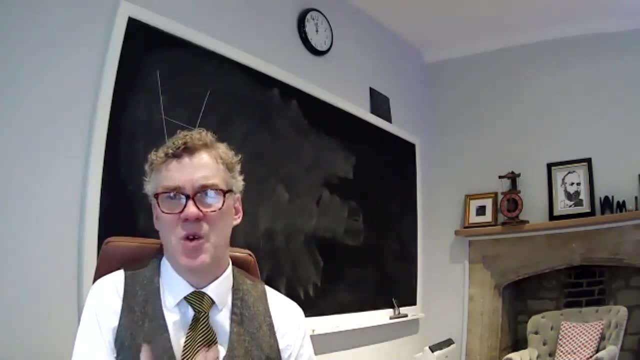 the socks are sort of indistinguishable. You know they're identical. There isn't a left sock and a right sock, There's just two socks, And we don't seem to have any way of defining or expressing or describing a way of picking. 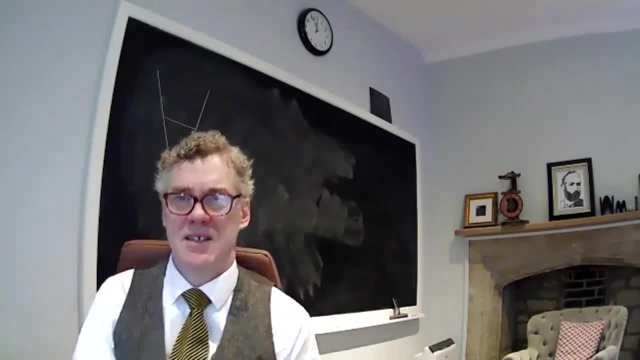 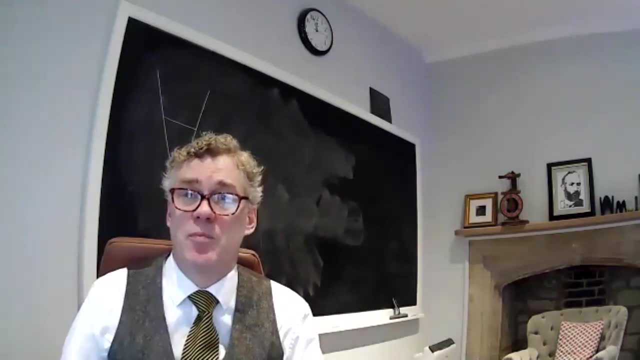 which sock it is that you pick from each pair. You know, and this is really the essence of the axiom of choice, is that the axiom of choice says: well, there is a way of picking. You just pick one from each pair. It doesn't matter how you pick it. 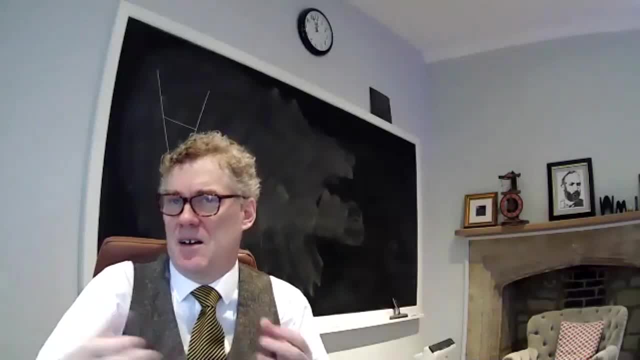 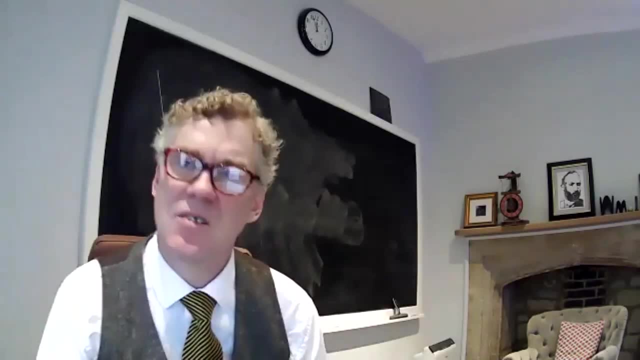 But how do we know that there is such a way of picking, you know, if we can't distinguish the socks Right? So there's oftentimes arguments that appeal to the axiom of choice have this non-constructive nature. The axiom is saying there is a way of doing it. 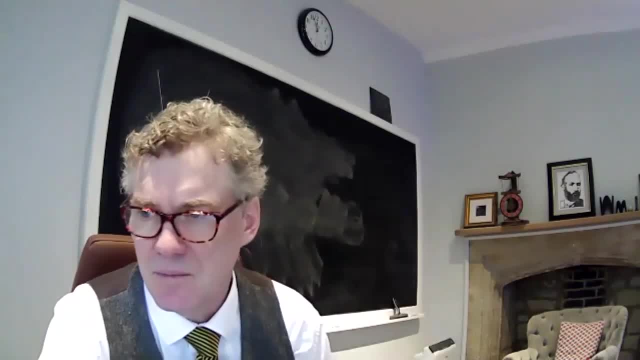 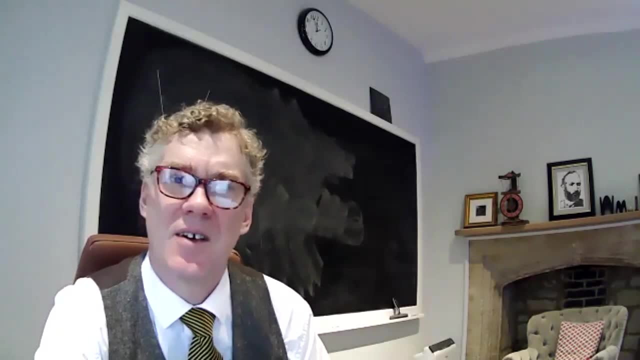 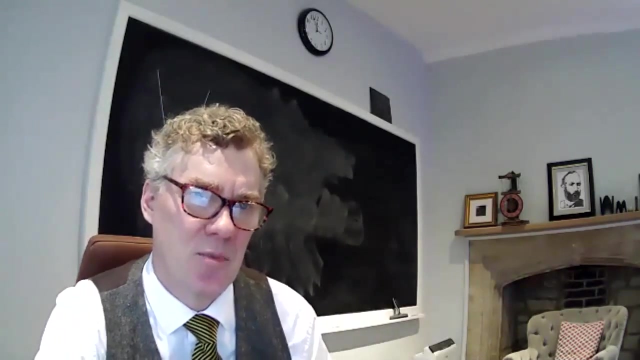 but we don't know exactly how to do it. Okay, So I'm realizing that everything is taking much longer than I thought, so I'm not gonna have time to cover everything that I thought, So let me move to the issue of paradoxical consequences of AC. 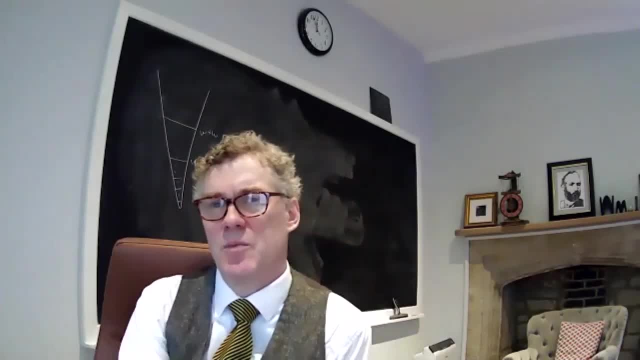 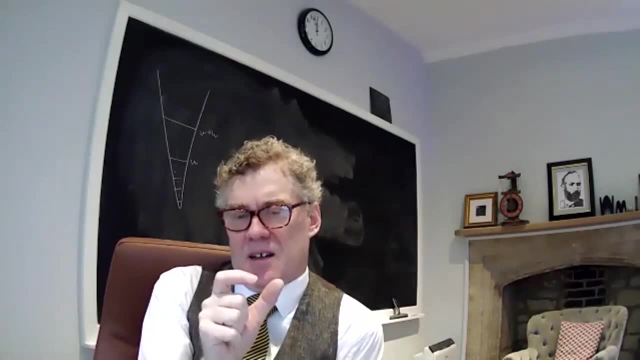 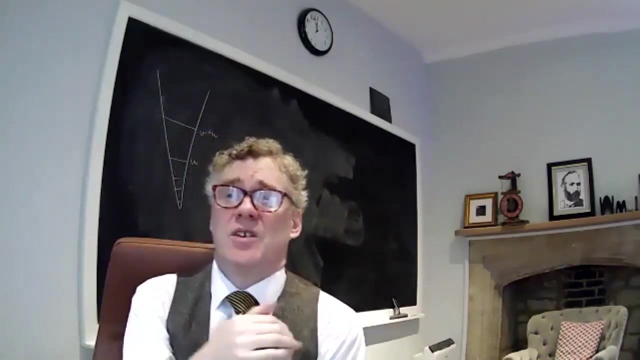 So Vitale had predicted that the axiom of choice had proved a remarkable theorem, assuming the axiom of choice. So he proved that there's a set of real numbers contained in the unit interval, such that the rational translations of that set are all disjoint and they cover the unit interval. 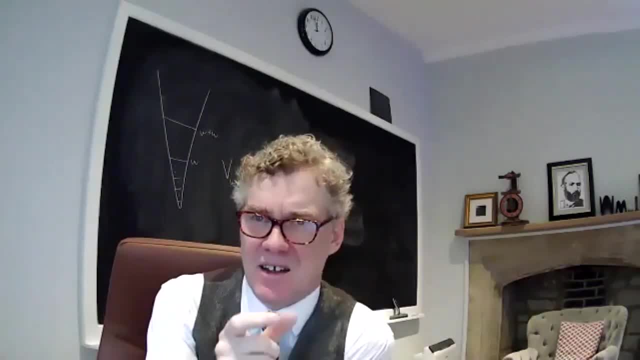 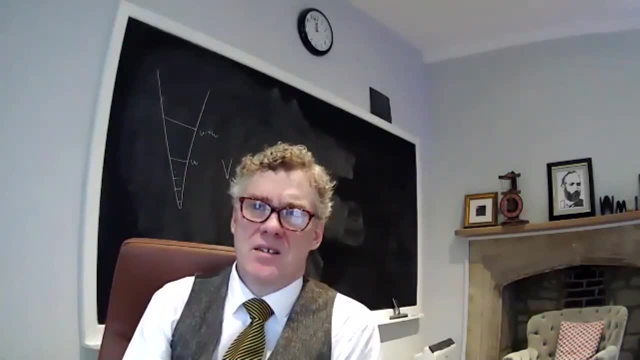 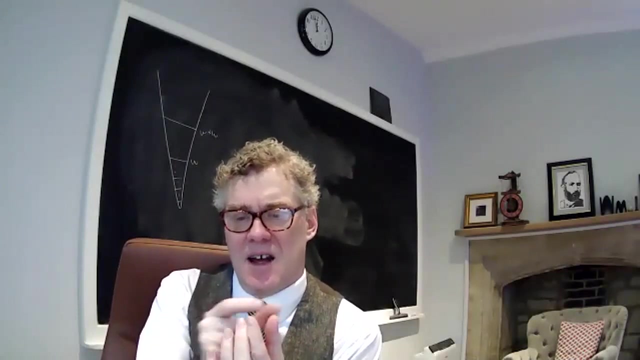 And from that it follows that the initial set can't have measure zero, because then the countably many translations of it would have a non-zero measure. But it can't have any positive measure either, because then the countably many translations of it, because they're disjoint, would add up to a number. 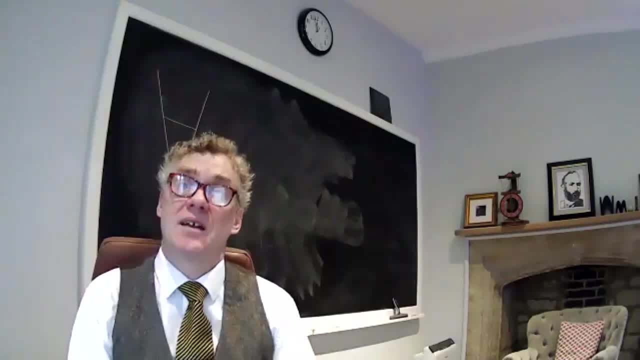 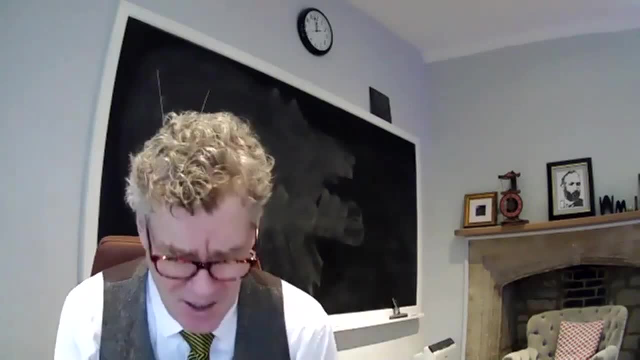 exceeding the way in which the measure of the set in which those translations exist. So therefore the set simply cannot be measurable. It cannot be Lebesgue measurable. So Vitale proved from the axiom of choice that there are non-Lebesgue measurable sets. 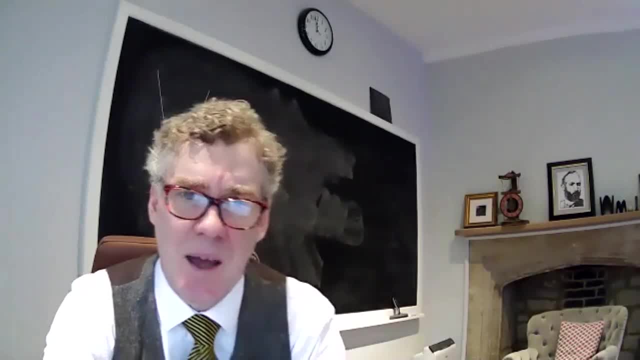 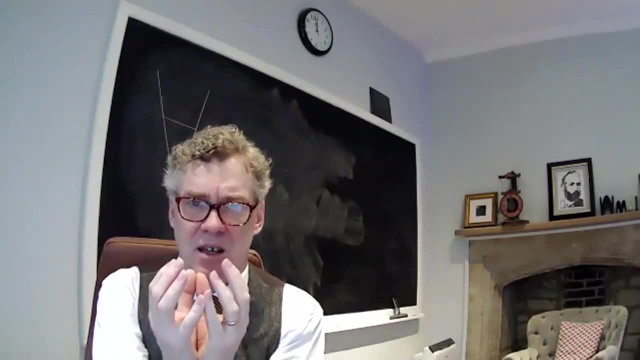 Not every set is Lebesgue measurable. A sort of more extreme example of this is the Banach-Tarski paradox, which says that if you take the unit ball in three dimensions, then you can partition it into seven pieces that are disjoint, so that with three of those pieces 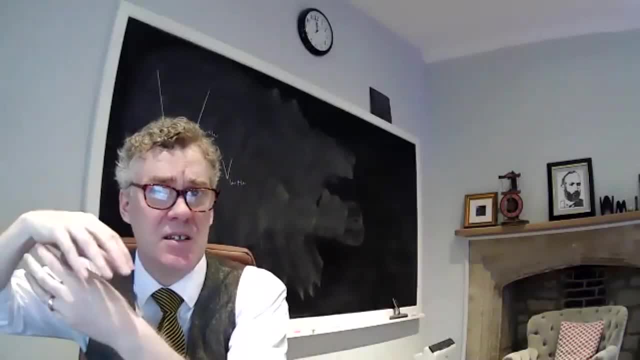 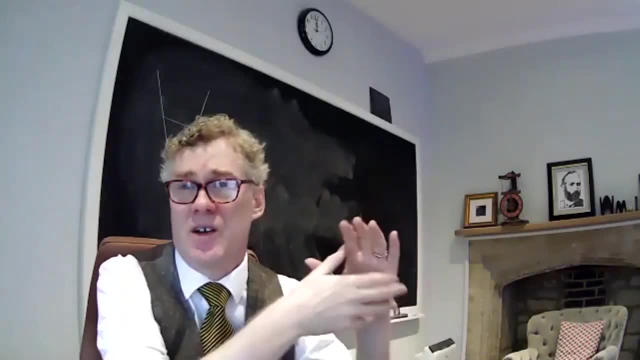 you can rearrange them through rigid motion rotations and reassemble the entire sphere again, And then also you can do it with the other four and rearrange them to make the whole sphere again without any gaps. So from one sphere we can make two without any holes. 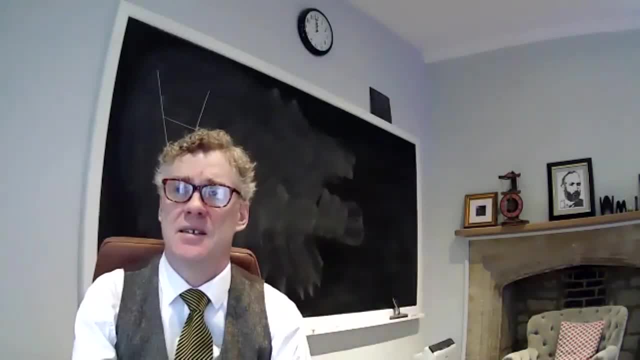 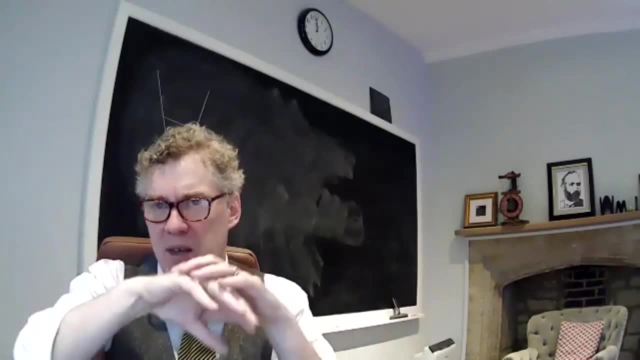 or anything by rigid motion on these seven pieces. Now, you shouldn't think of carving these pieces with a knife. It's not like you could describe them geometrically, like by slicing or something. These pieces, each of them, is totally dense in the sphere. 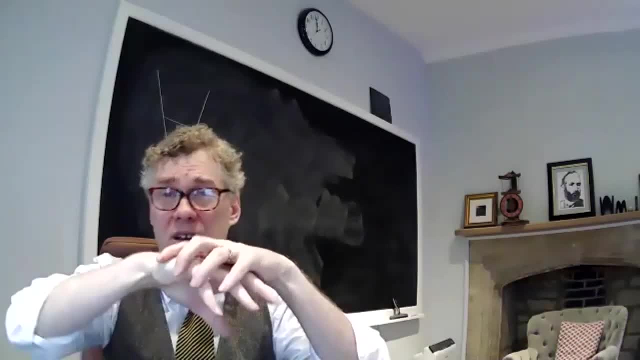 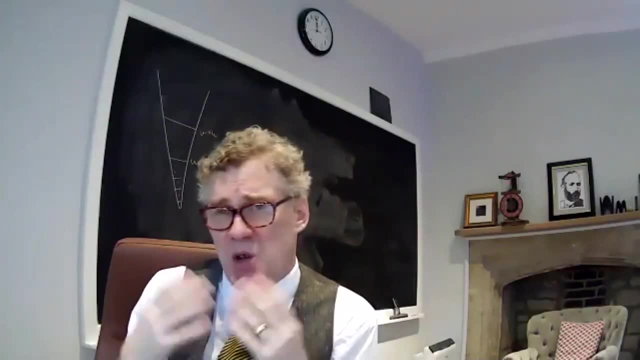 and they're all dense in each other, And so they don't overlap, And when you move them and the other one just fits in, even though it didn't beforehand, And so these are quite strange and bizarre pieces that we're talking about. 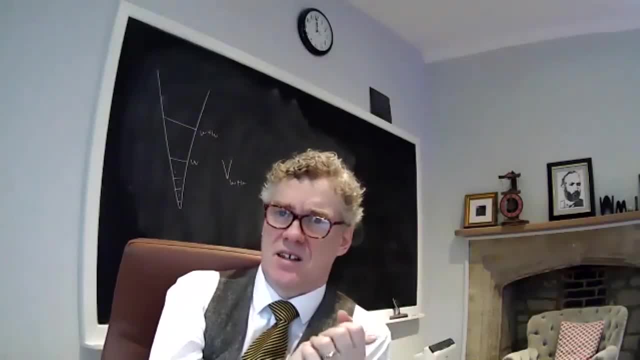 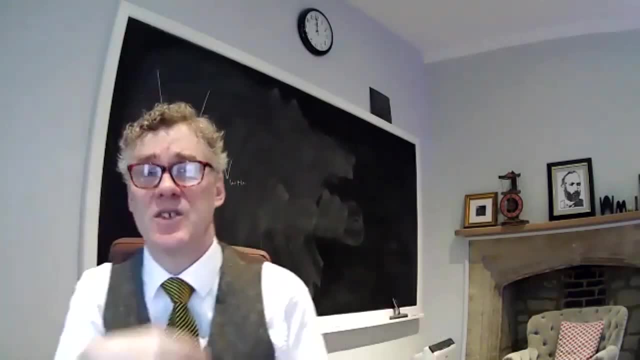 but it's kind of paradoxical that you can take a sphere into seven disjoint pieces and with three of them make the whole sphere again of the same size, and with the other four make the whole sphere again of the same size. So of course these pieces also cannot be measurable. because that process would violate the fact that measure is preserved by those rigid motions. So these kinds of examples are often given as evidence against the axiom of choice because they're paradoxical consequences of AC. There may be reason to doubt AC, but I view it as a kind of confirmation bias. 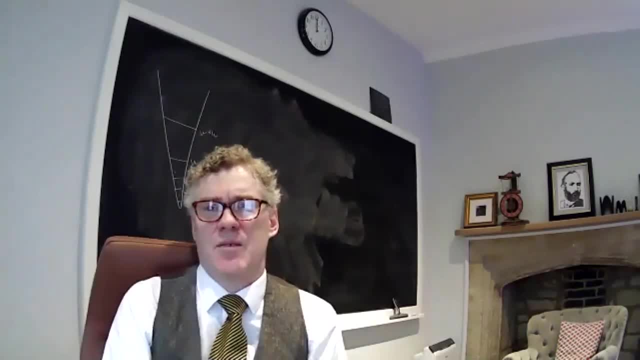 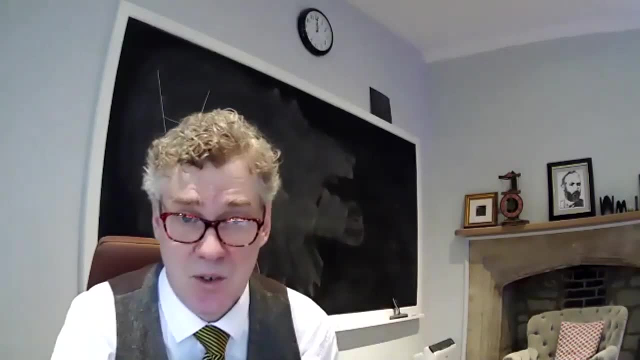 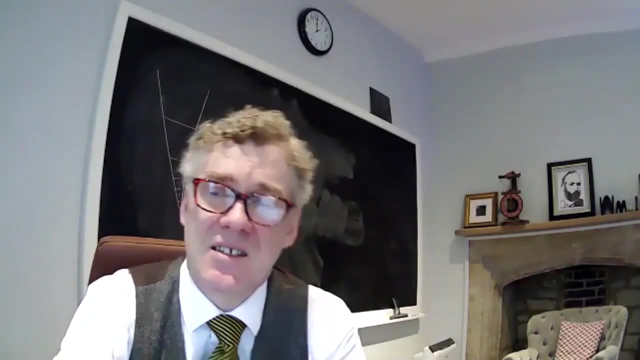 To discuss only the counterintuitive consequences of the axiom of choice without also discussing the extremely counterintuitive situations that can occur if you don't have the axiom of choice. So it makes for a kind of fair discussion, placing things in context to also discuss. 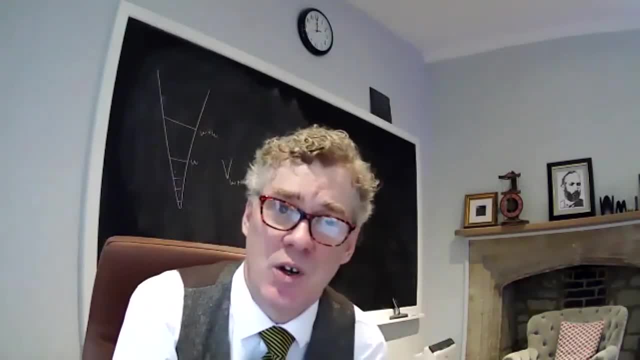 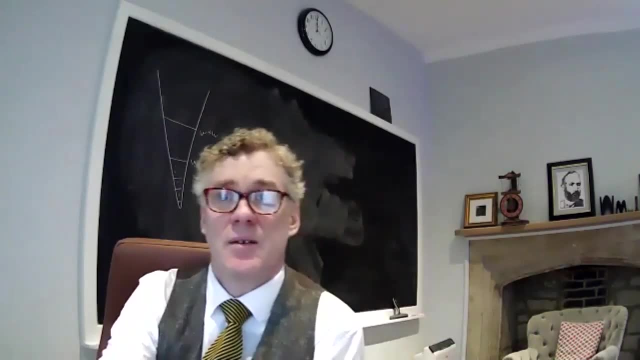 the counterintuitive things that happen on the other side. So if you don't have the axiom of choice, for example, a real number can be in the closure of a set of real numbers, but not the limit of any sequence from that, Or a function can be continuous in the sense. 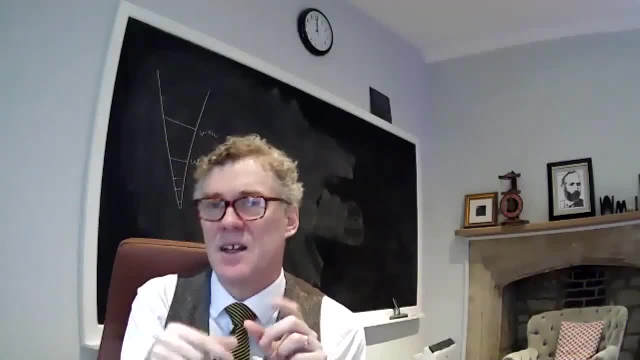 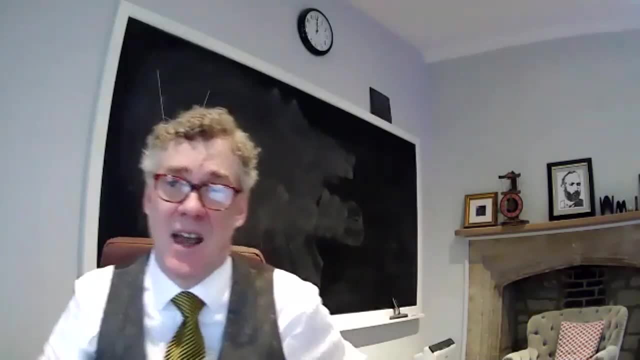 that whenever you have a convergent, whenever xn converges to x, then f of x converges to f of x. So that's commonly taken as a definition of continuity. But you can have a function with that property that doesn't have the continuity property expressed. 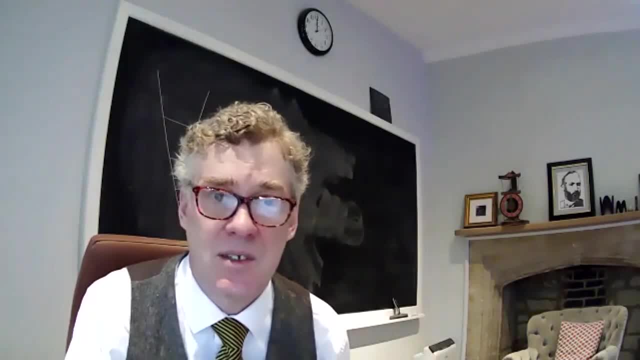 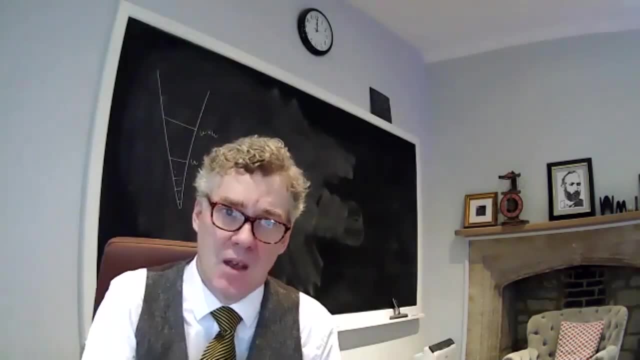 in the epsilon delta sense. They're just not the same without the axiom of choice. Or you can have without the axiom of choice, a set can be infinite but not have any countably infinite subset. Without the axiom of choice there can be an equivalence relationship. 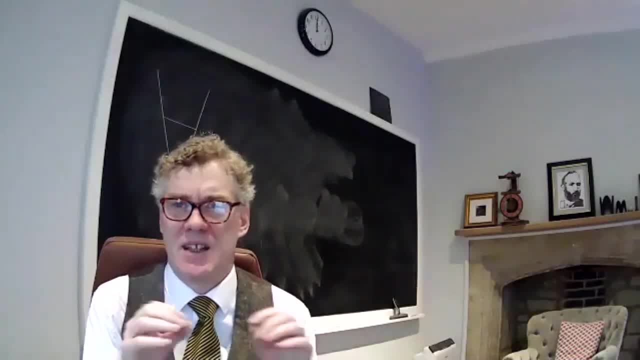 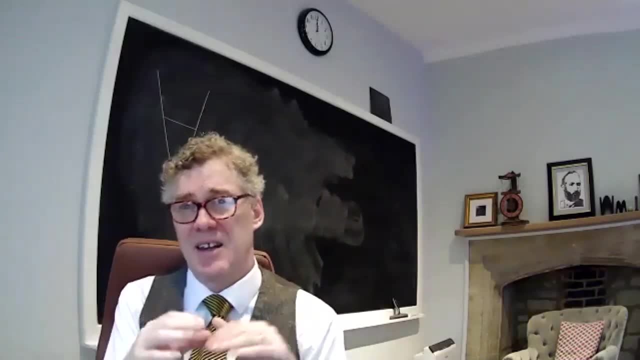 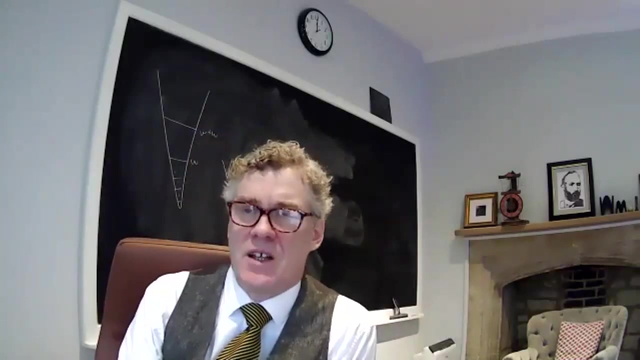 on the real numbers, such that the number of equivalence classes is strictly greater than the number of real numbers. Okay, let me say that again. So we have the real numbers, all the points. We can group them by an equivalence relation so that the number of groups 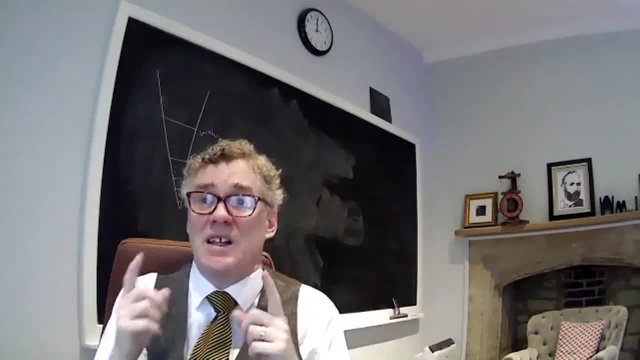 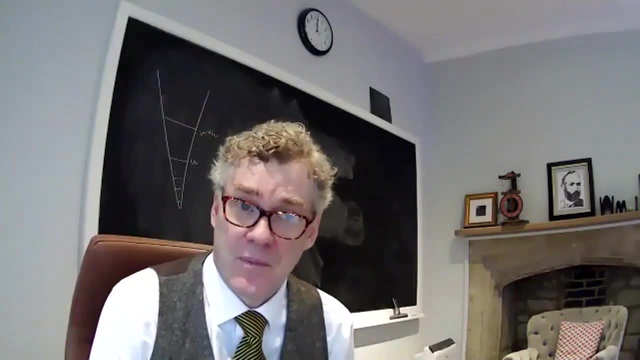 each group has many points in it. The number of groups is strictly more than the number of points. Okay, it's sort of totally the opposite of what you would expect. So, without the axiom of choice, there can be a field that has no algebraic closure. 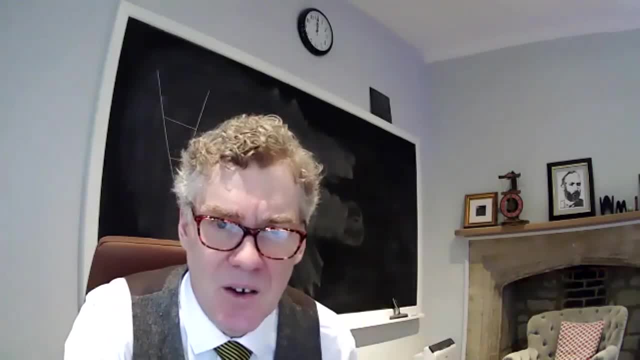 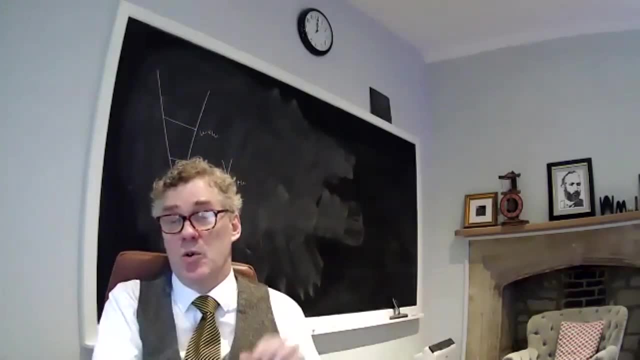 or there can be a vector space with no basis. So without the axiom of choice, the real numbers can be a countable union of countable sets, but still uncountable because Cantor's theorem does not require the axiom of choice. Okay, so I think these kinds of examples 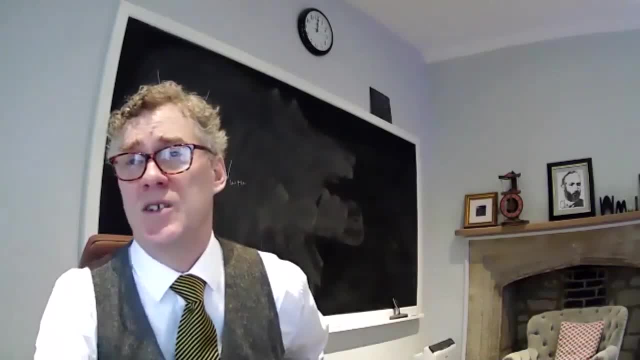 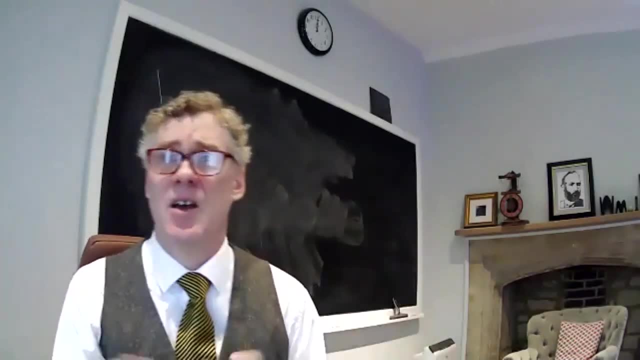 support a call for balance really in the way of discussing the axiom of choice. It's not right to say the axiom of choice is problematic because it has those problematic consequences, because the axiom of choice is unproblematic because it rules out these other weird situations. 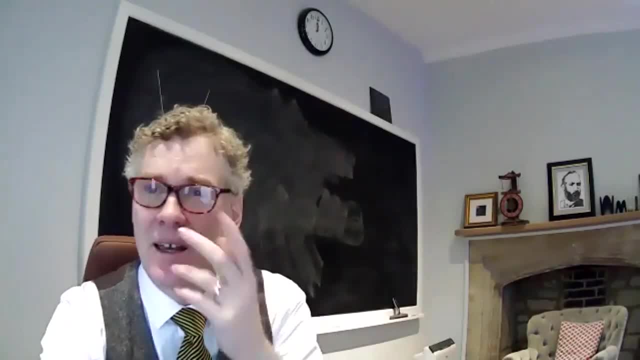 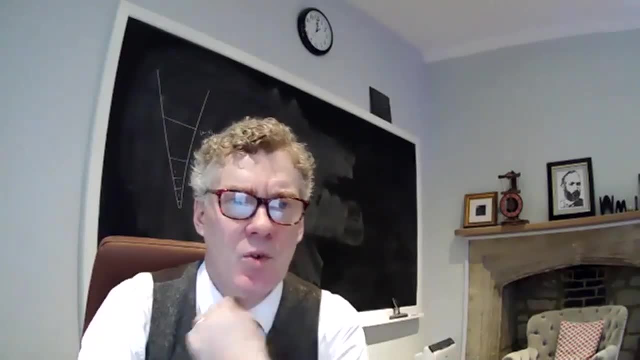 which in many cases are much weirder and more bizarre than, say, even the Banach-Tarski paradox. So there was a major foundational development when Robert Solovey proved that if you assume the existence of an inaccessible cardinal, then it's consistent with set theory. 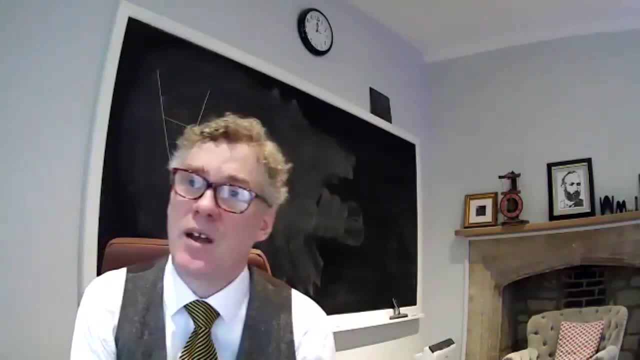 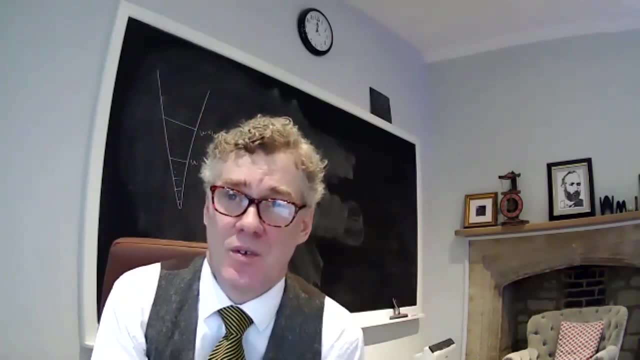 without having the axiom of choice, that every set of real numbers is Lebesgue measurable. So in other words, if we give up the axiom of choice, then we can have every set being measurable. That doesn't follow from Vitale's theorem. 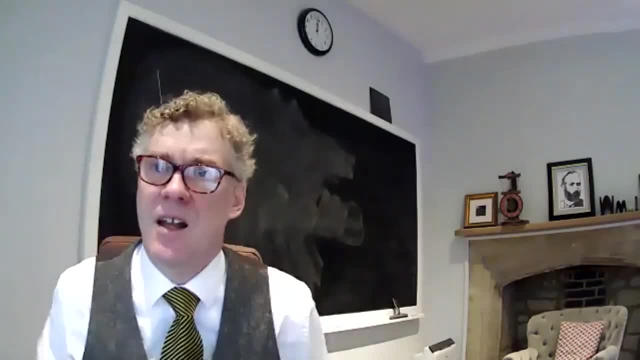 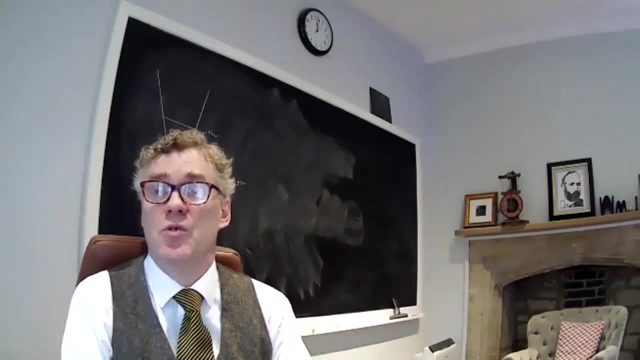 Vitale just proved that if AC is true then there's a non-Lebesgue measurable set. But Solovey proved: look, you really need the axiom of choice for that proof, assuming the consistency of an inaccessible cardinal. So Solovey has identified: 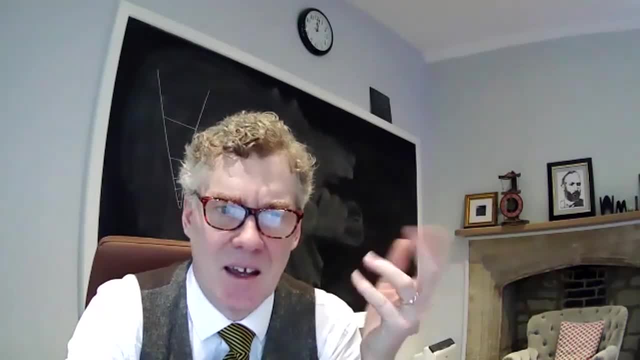 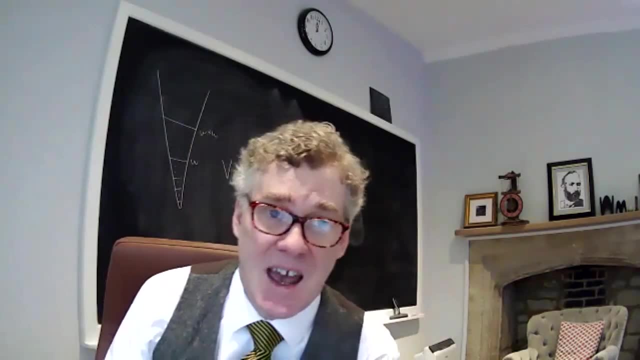 this sort of dream world for analysis, a world in which every set is Lebesgue measurable. So he once told me that what he expected after proving that theorem was that the analysts would immediately adopt that theorem, that theory, as the new foundational theory for analysis. 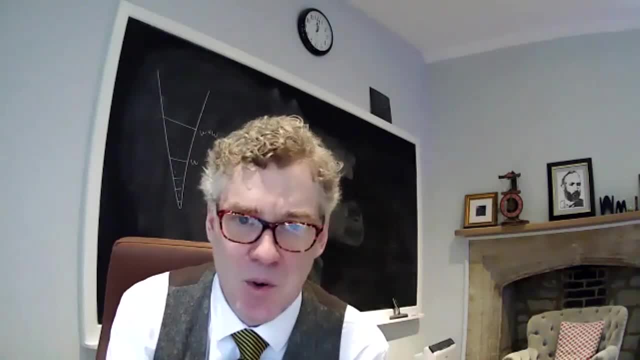 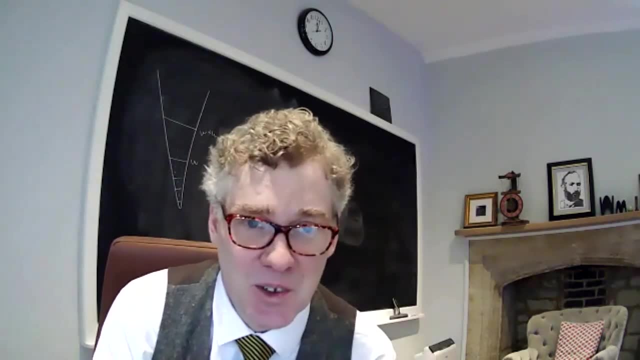 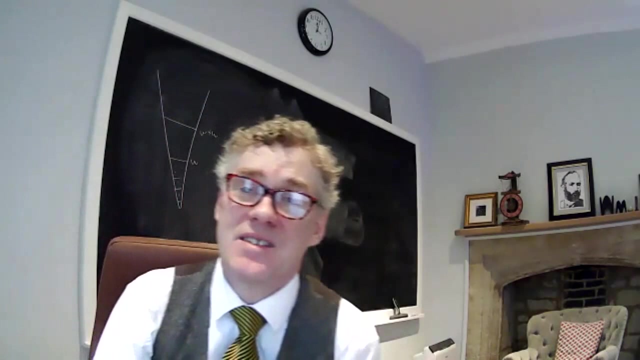 because they wouldn't have to worry about non-measurability anymore. Mathematics would be free and easy, and one might have expected him to be carried on the shoulders of the analysts, But that didn't happen. They didn't give up the axiom of choice. 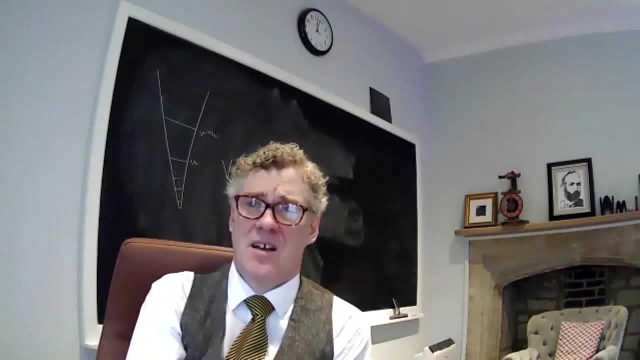 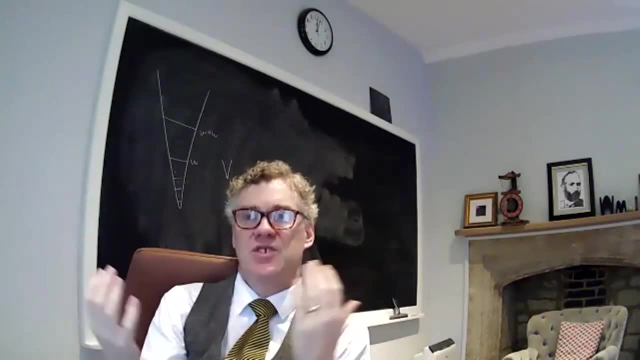 and they continued to pay attention to their sigma algebras and their worries about measurability. And so why was Solovey's theory not adopted wholesale in order to achieve this dream world for analysis? And my explanation of that is that the pull 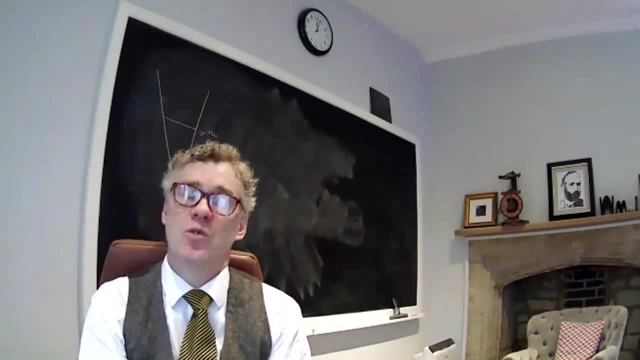 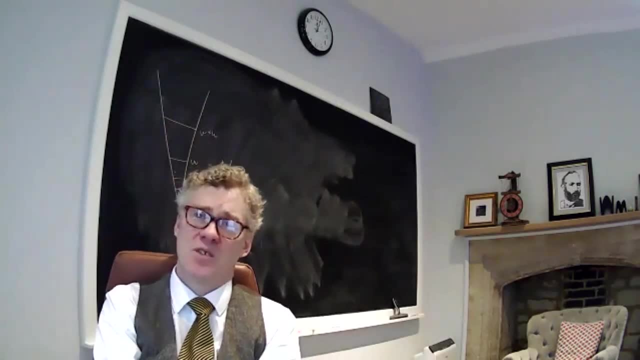 of the axiom of choice as a fundamental principle is simply overwhelming. It's much too strong. The analysts didn't want to give it up. Mathematicians in general don't want to give up the axiom of choice because there's a view that the axiom of choice is expressing a fundamental truth. 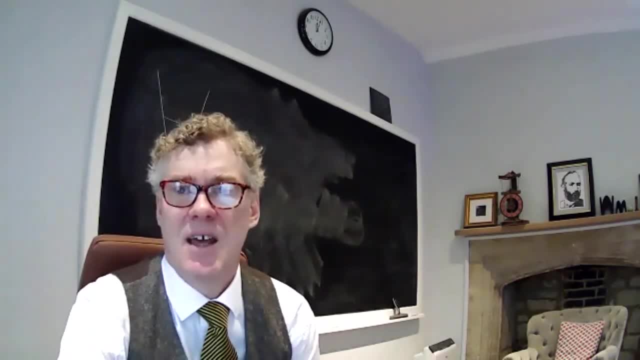 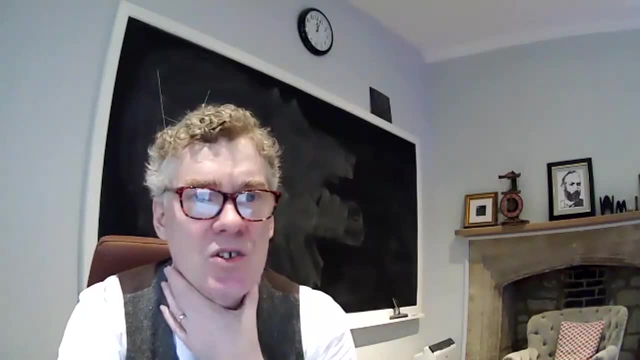 about the nature of which sets there are, And there is a set that makes such choices, even though we can't necessarily describe such a set. So let's move now to large cardinals. So these are the strongest known axioms in mathematics. 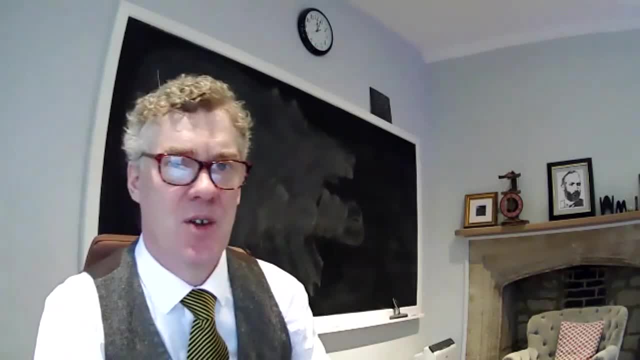 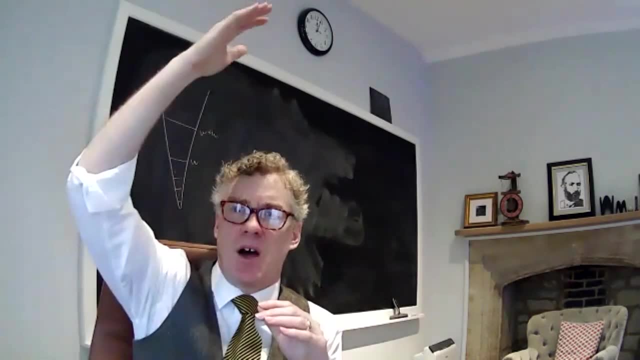 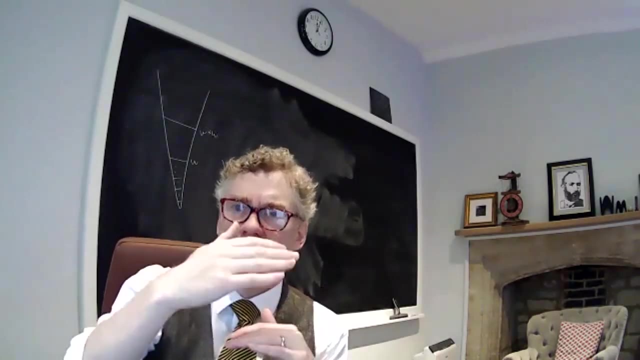 So the large cardinal hierarchy really is a natural instantiation of the transplanet tower of iterated consistency statements. So last lecture we said if you have any theory t, then towering above that theory is this, This tower of consistency strength. So we can add conti and conconti and so on. 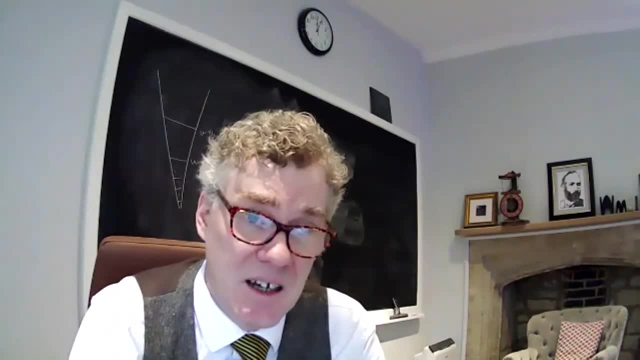 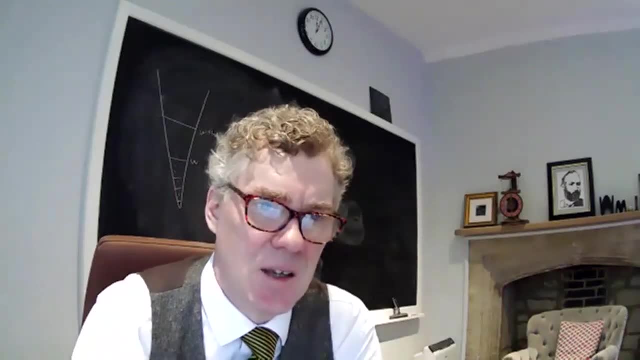 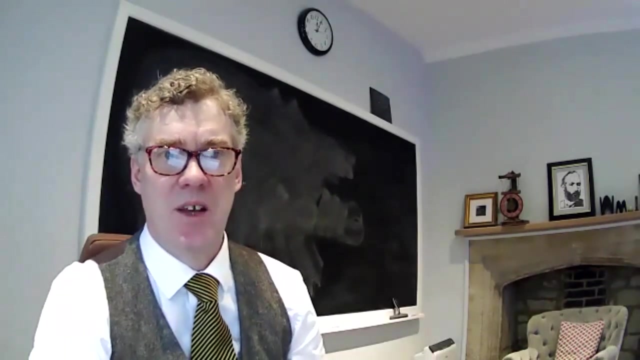 the iterated consistency assertions added on top, And the large cardinal hierarchy instantiates that hierarchy, quite naturally. Let me just mention some of the names of these large cardinals. We have the worldly cardinals, the inaccessible cardinals, hyper-inaccessible, uplifting cardinals. 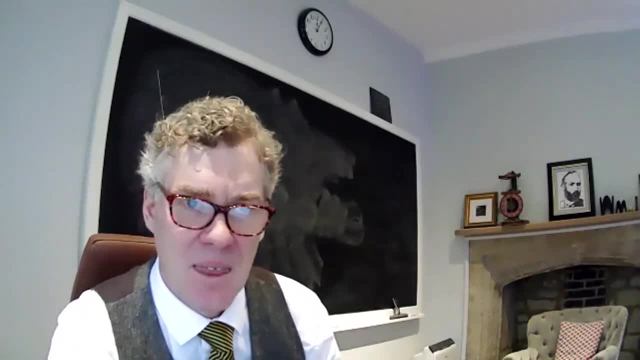 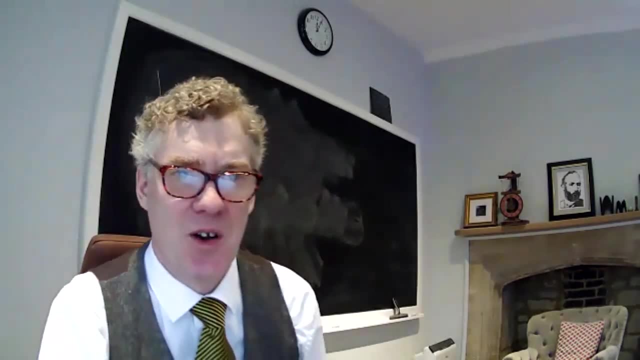 Mahler cardinals, the totally indescribable cardinals, the weakly super-strong cardinals. We have the long cardinals, the subtle cardinals, the measurable cardinals, tall cardinals, strong cardinals, super-strong, super-compact, almost huge, huge cardinals. 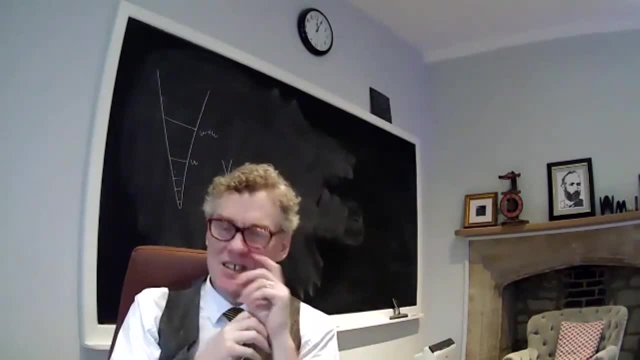 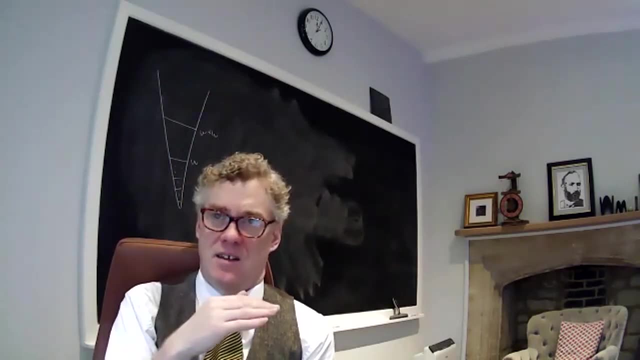 super-huge cardinals and so on. So of course these names sound kind of silly if you don't understand it. But each one of those concepts corresponds to a rather technical, set theoretic notion of infinity And the existence of those large cardinals. 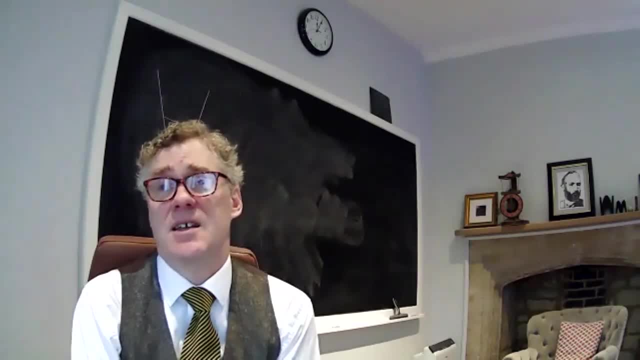 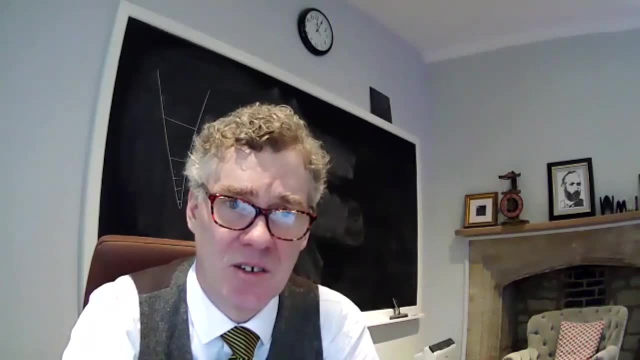 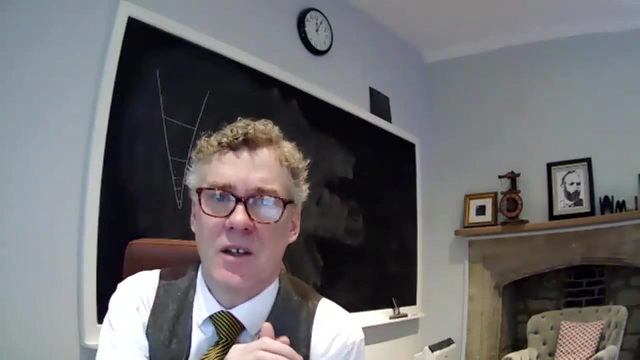 is making a certain strong statement about which kind of infinities exist, And these are all quite large. So let me try to convey the nature of some of these large cardinal axioms. If you think about the smallest infinite cardinality, Aleph, 0 or omega, the countable infinity. 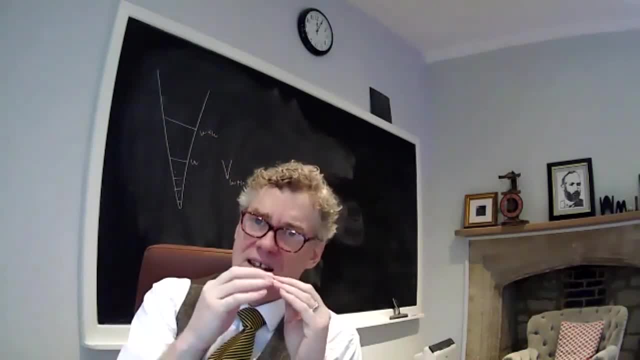 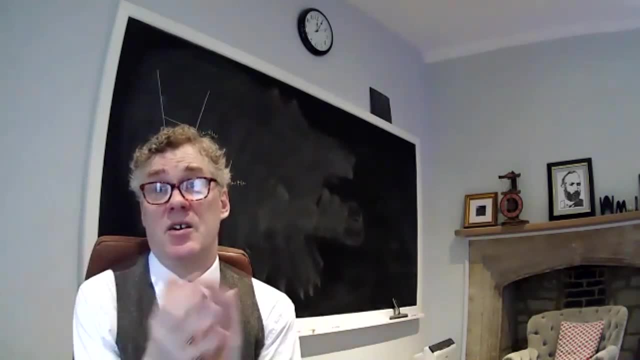 it has a certain property, Namely any set of size less than it is finite, and the power set is also finite. So, in other words, Aleph 0 is closed under the power set operation If you have a set that's smaller than Aleph 0,. 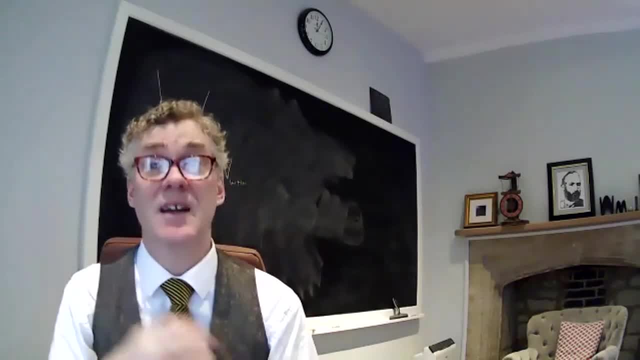 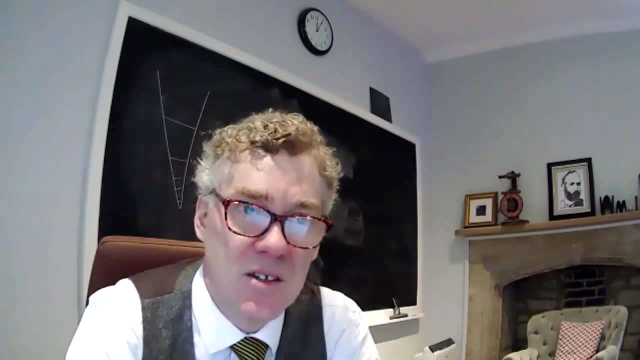 its power set is also smaller than Aleph 0. So could there be an uncountable infinity Like that? Can you have an uncountable infinity which is closed under the power set operation? So such an infinity would be called a strong limit cardinal. 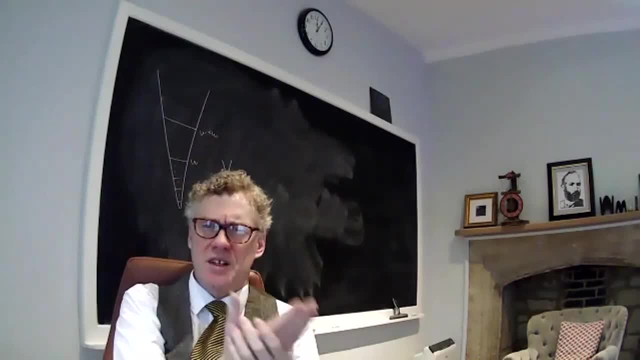 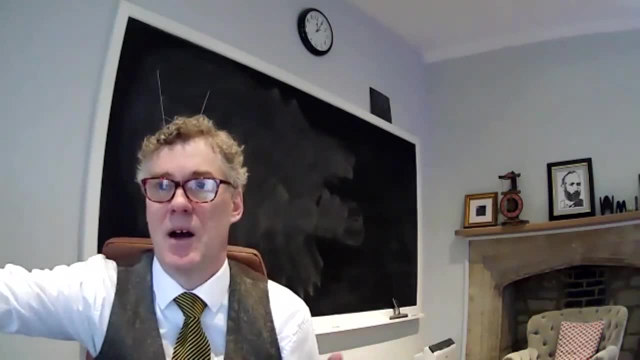 And can we make it? Yes, we can make one. So, for example, if you start with the natural numbers and you take the power set of that and then the power set of that and the power set of that, and so on, you iterate the power set operation. 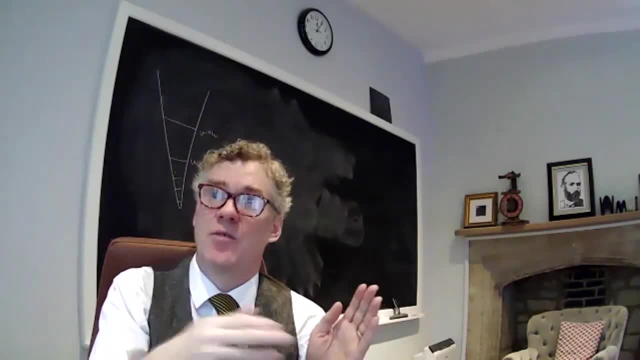 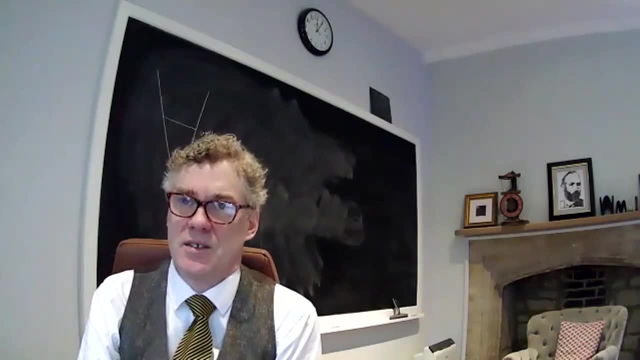 So we know by Cantor's theorem that this is getting strictly larger. Whenever you take the power set of a set, you get a strictly larger set. So if we just take the smallest infinity that's bigger than all of those ones, then it: 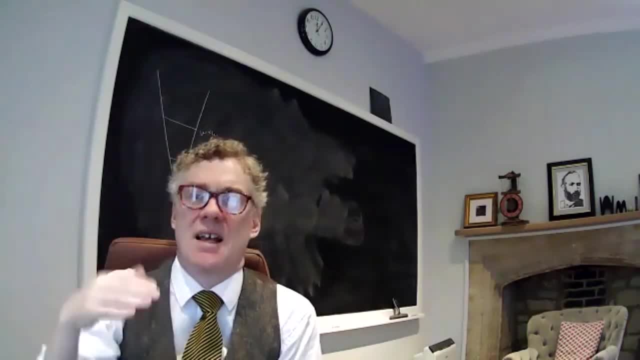 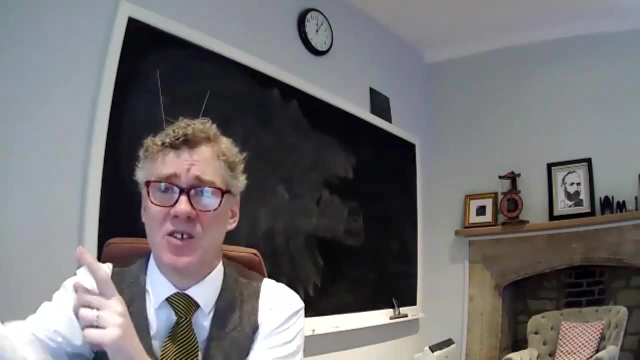 will have the property of being a strong limit, Because anything that's less than it will be less than something that appeared in my hierarchy of these iterated power sets, And therefore its power set will just be the next one, which is also less. 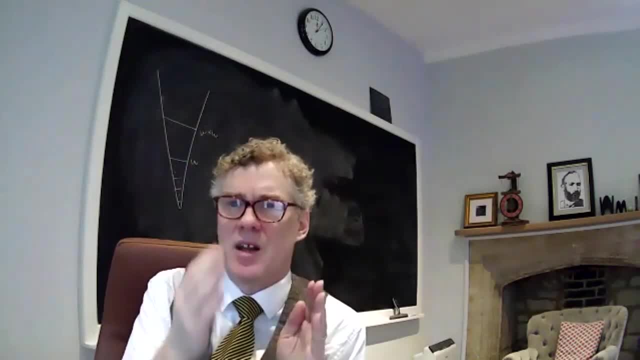 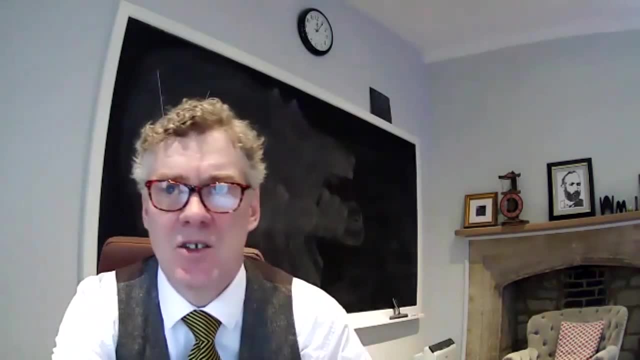 So this is the cardinal, known as Beth sub omega, because those iterated power sets are exactly Beth 0, and Beth 1, and Beth 2, and so on, as we explained, I think, in lecture three. So if we just take the smallest infinity, that's bigger than all. 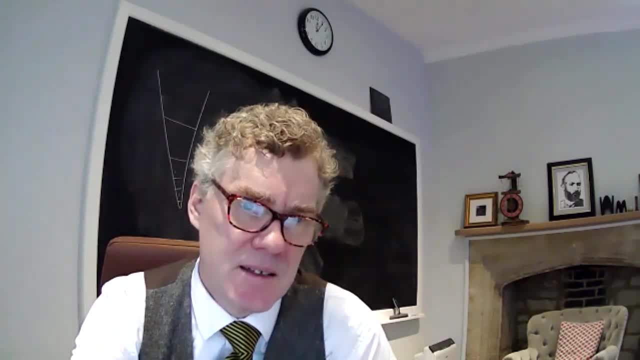 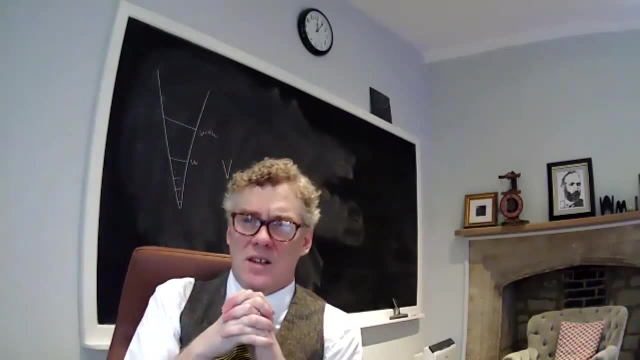 of those ones, then it will be less than 0.. So let's talk about the inaccessible cardinals. So inaccessible cardinals are strong limit cardinals, But they also have another property that all of 0 has, namely, all of 0 has the property 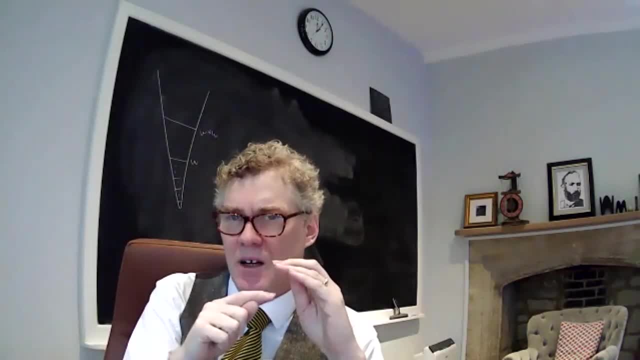 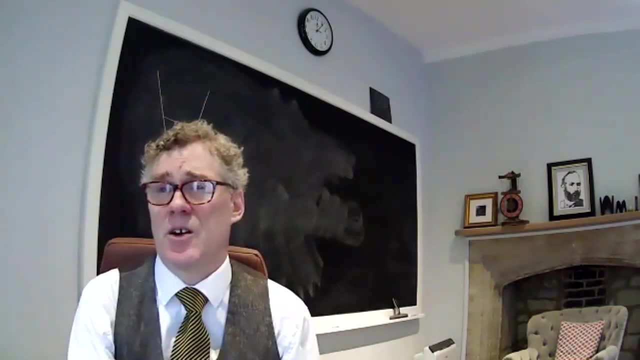 that if you have any finite sequence of cardinals below it, then the supremum is also below, Because the supremum of finitely many finite cardinals is still finite. It's just the largest one on that finite list. So that's called regularity. Regularity means there's no short sequence that reaches the cardinal, Short meaning relative to the cardinal itself. So kappa is said to be regular if any sequence of size length and less than kappa of cardinals below kappa has its supremum also below kappa. 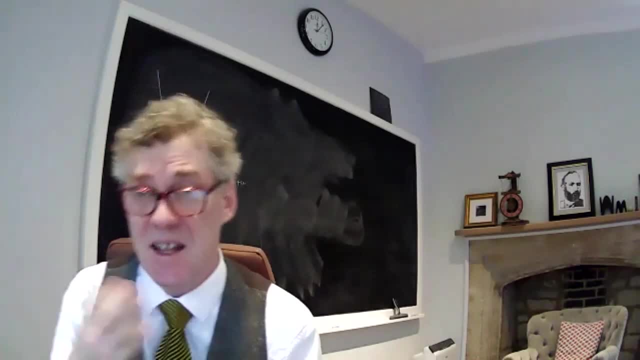 So, for example, all of 0,- I mean all of omega- does not have this property. All of omega is the supremum of all of 0,, all of 0., All of 1,, all of 2,, all of 3,, and so on. 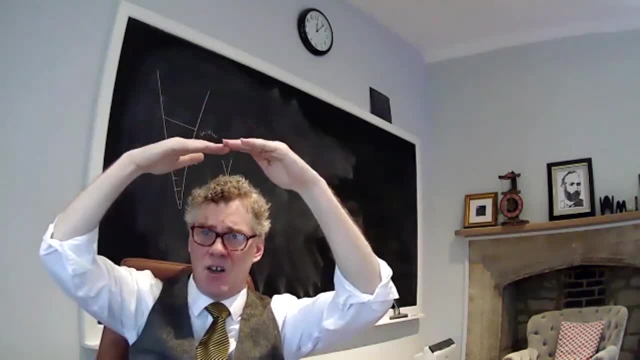 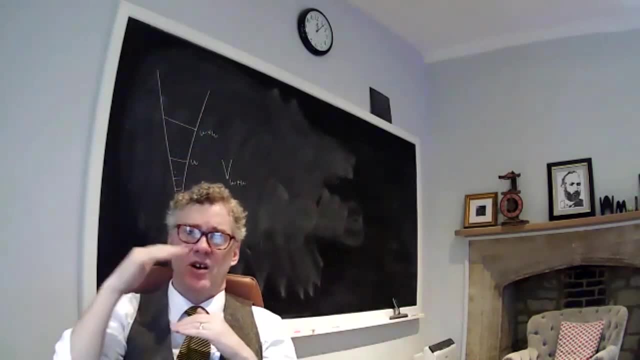 So there's an omega sequence that's unbounded in all of omega, But all of omega is much bigger than omega, So that omega sequence counts as a short sequence of cardinals, each of which is less than all of omega, But the supremum is not less. 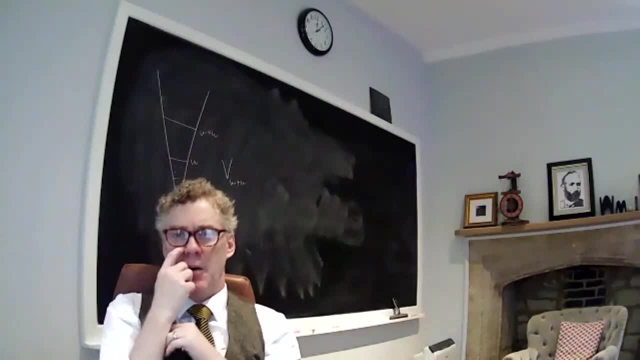 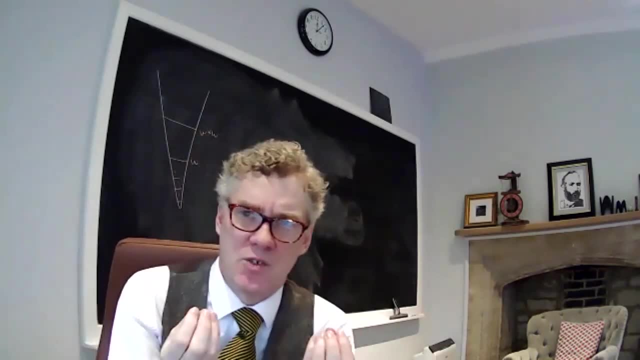 So all of omega is not regular. So what we want is an inaccessible cardinal. kappa is a regular, strong limit cardinal, So it has both of those features of all of 0. It's 0, but it's uncountable. An inaccessible cardinal is an uncountable, regular, strong limit. 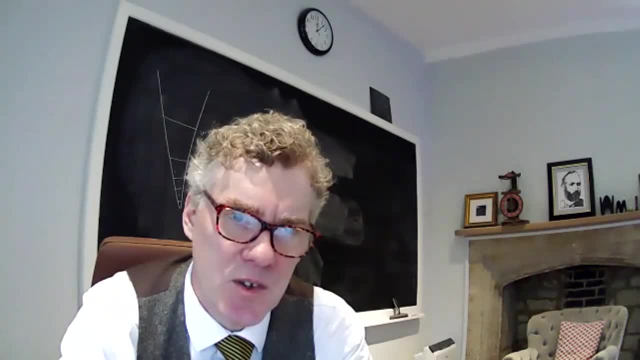 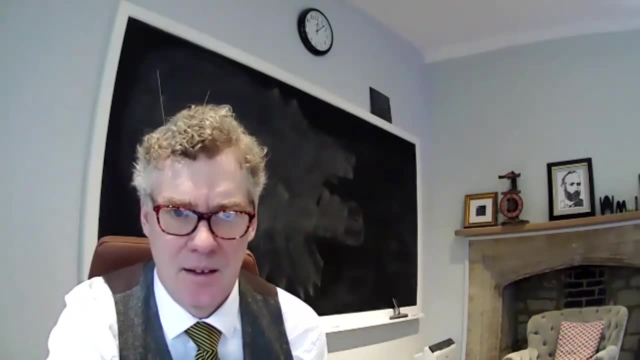 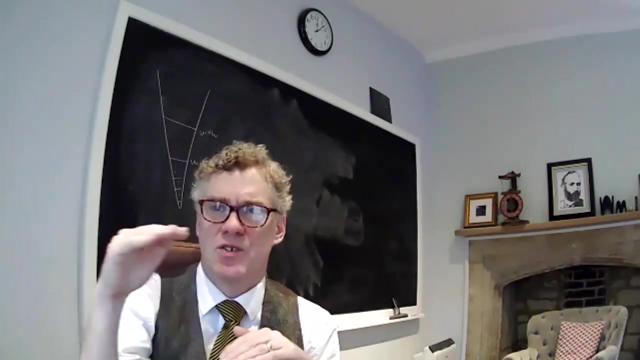 cardinal, And these cardinals were first studied by Hausdorff, So they're quite old. They were really there from the start of set theory And Zermelo had proved that if we chop off the set theoretic universe at v kappa. 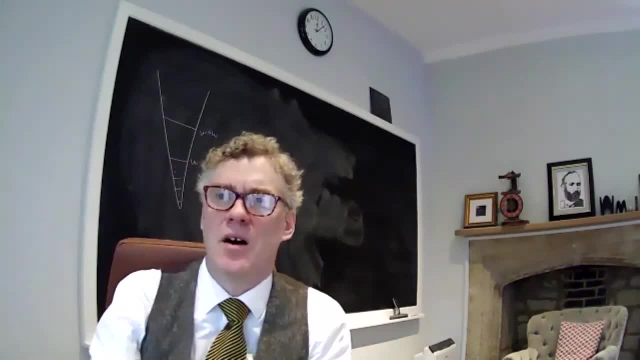 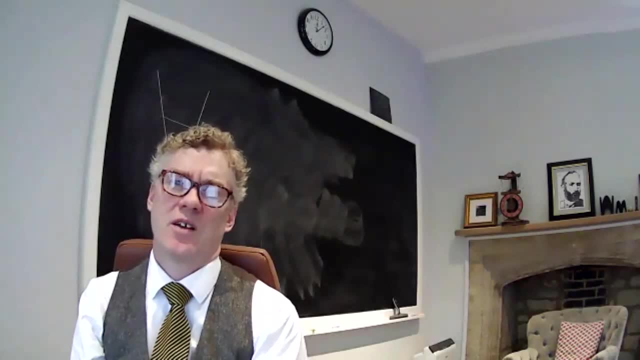 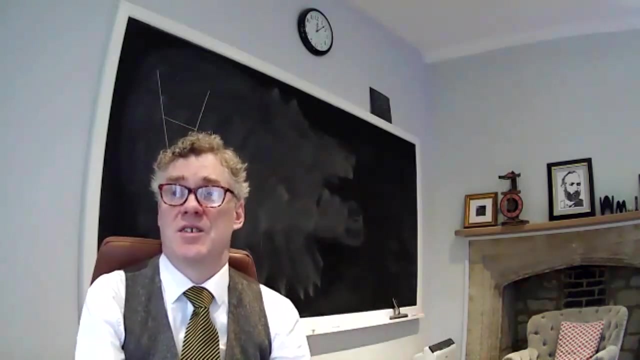 where kappa is inaccessible, then these are exactly the models of his second order ZF set theory. So Zermelo-Fraenkel set theory, the models of second order Zermelo-Fraenkel set theory, are exactly the cutoff versions of the universe. 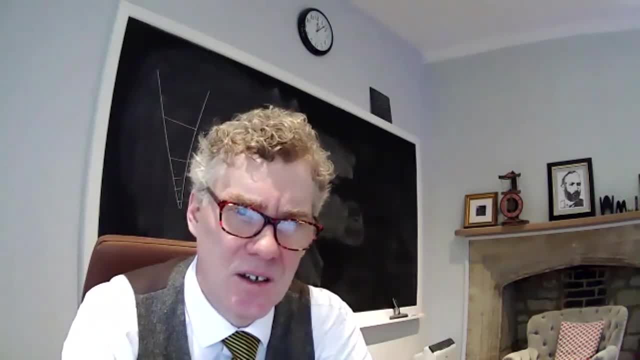 at an inaccessible cardinal, So these are also known as Grothendieck universes. They're identical with what came to be known as Grothendieck universes, So they're now called the Zermelo-Groethendieck. 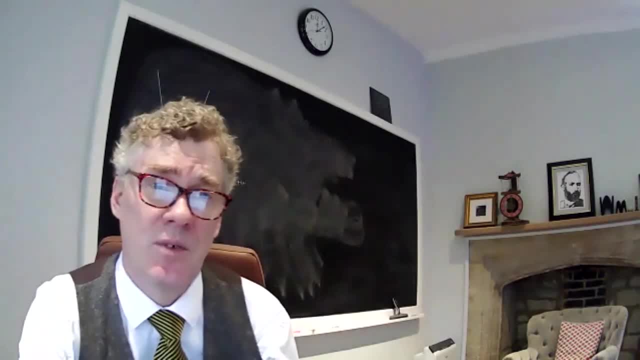 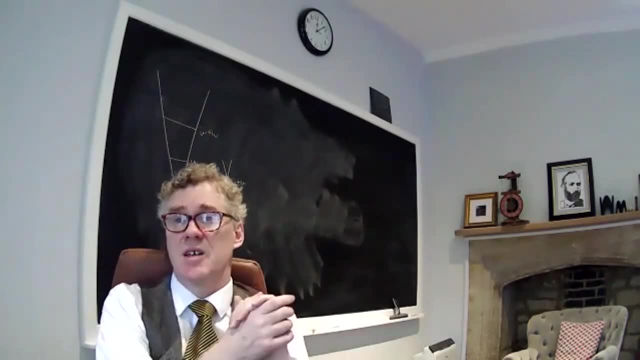 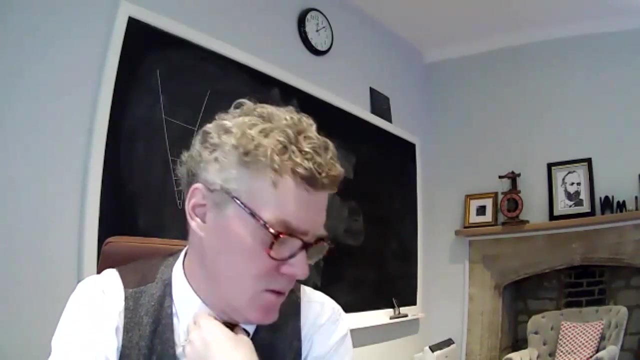 universes because Zermelo had them in 1930.. They were rediscovered really in category theory by Grothendieck and used, And they're also there- as a universe concept in the universe axiom, for example. So therefore, if we think about say, 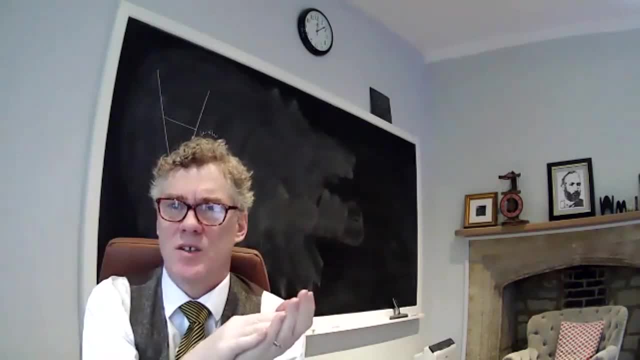 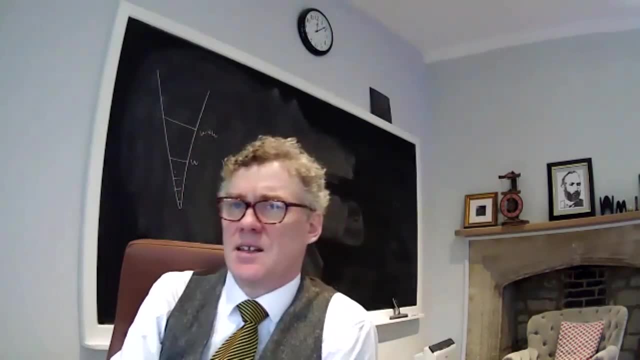 the smallest inaccessible cardinal, kappa. if kappa is the smallest inaccessible cardinal, then v kappa. the universe up to kappa doesn't have any inaccessible cardinals inside it. So therefore, if there is any inaccessible cardinal, then there will be a smallest one. 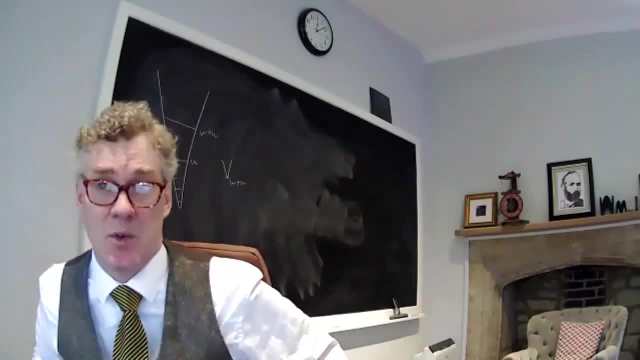 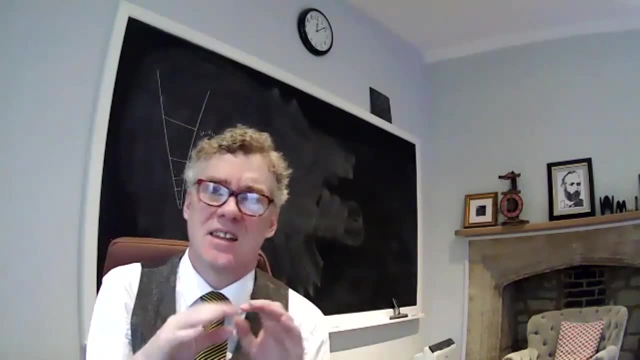 And therefore there will be a model of set theory in which there are no inaccessible cardinals, And from that it follows that you cannot prove that there are any, because if there are any, then it's consistent that there aren't, because the smallest set theoretic universe v kappa. 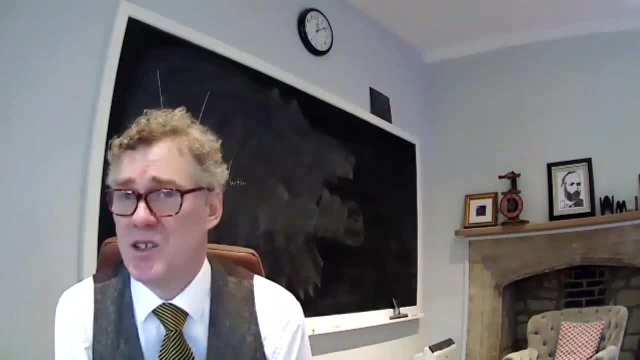 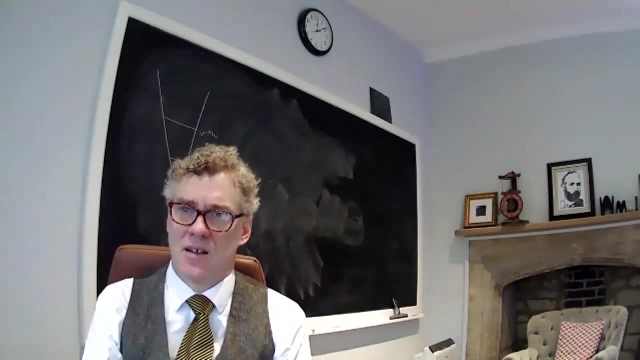 where kappa is the smallest inaccessible cardinal is a model of set theory in which there aren't any inaccessible cardinals. So therefore we cannot prove that these large cardinals exist, because if they do exist, then for any given one of them. it's also consistent that they don't exist. We can't even prove that it's relatively consistent that they exist in the way that we can for many of the other axioms that are set here. We can't prove that if CFC is consistent. 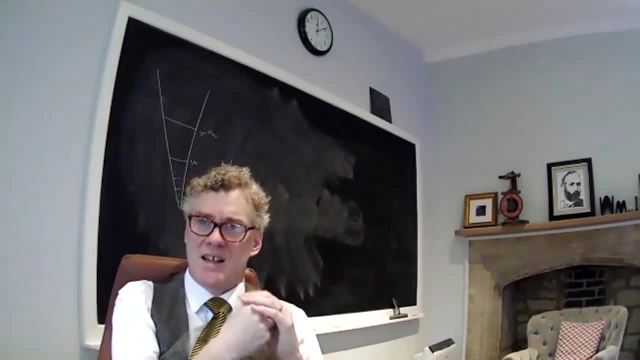 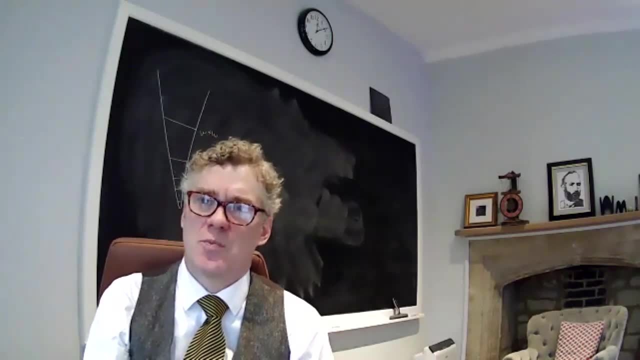 then it's consistent that large cardinals exist, precisely because not only do we get that it's consistent that there's no large cardinals, but actually that consistency assertion is going to be absolute between the original universe and the universe that we're building. 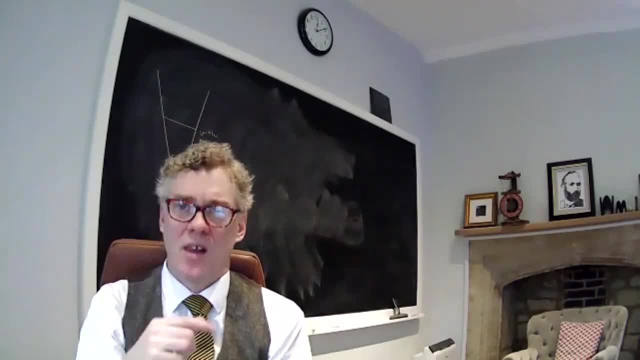 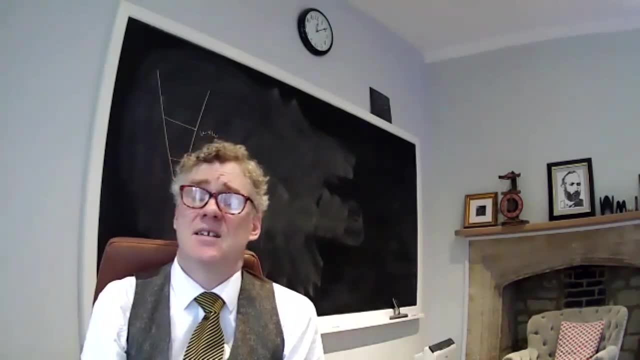 And so we would violate the incompleteness theorem if we could prove that relative consistency. So, with these large cardinals, we can't prove they exist and we can't even prove that they're consistent. And so you might say: well, what's the point then? 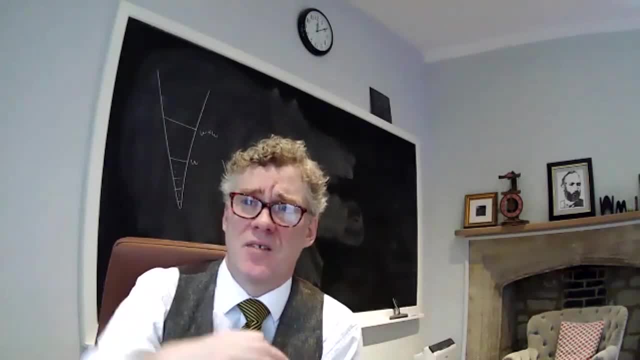 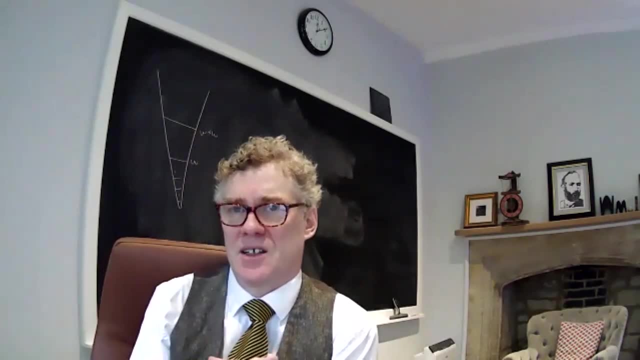 Why study this sort of totally suspicious mathematical theory of these objects that you can't prove they exist? and you can't even prove that it's consistent that they exist. And the answer to that objection is that that's the whole point Gödel told us in his incompleteness theorem. 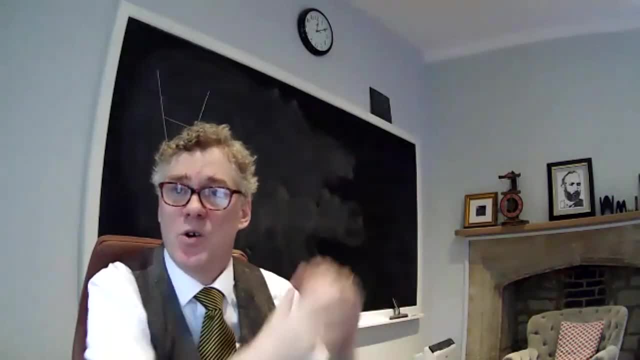 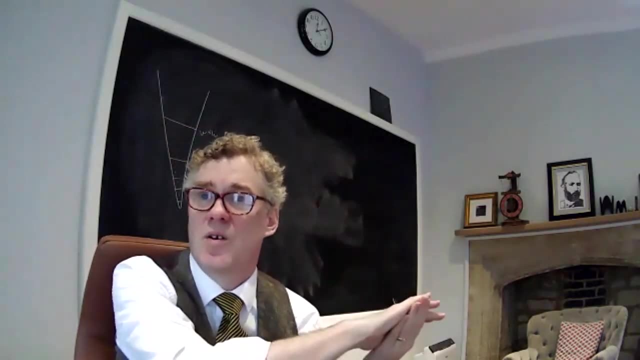 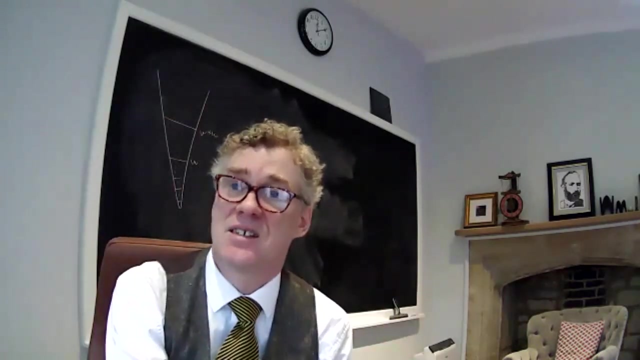 that there was this tower of consistency string towering above any given theory. And what that means is precisely that you can't prove on the basis of the smaller assumptions that the stronger ones are true, or even that they are consistent. That's the nature of the consistency strength hierarchy. 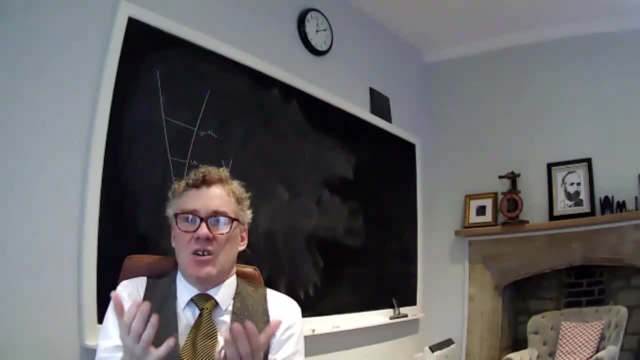 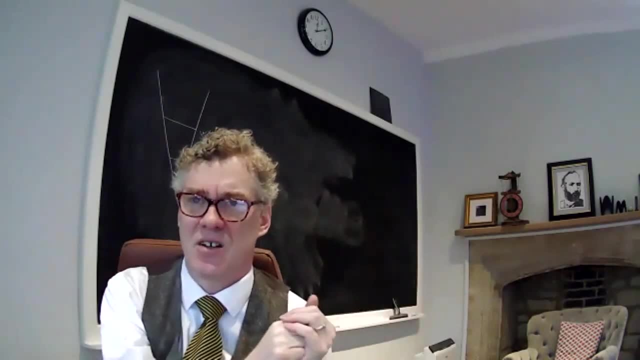 And the large cardinal hierarchy is exactly having that feature that Gödel told us would exist. But furthermore, it's doing so not with these consistency assertions and iterated consistency assertions that are totally wrapped up in the syntactic details of the logic, but rather it's doing it in terms 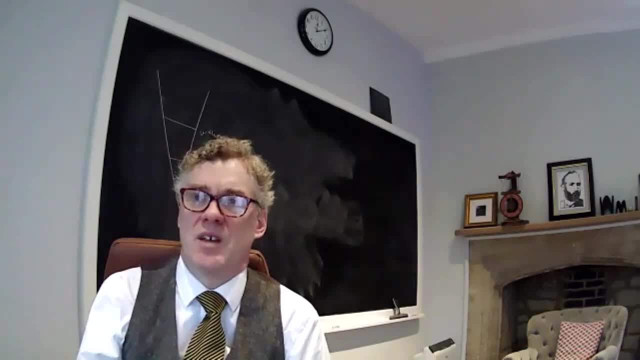 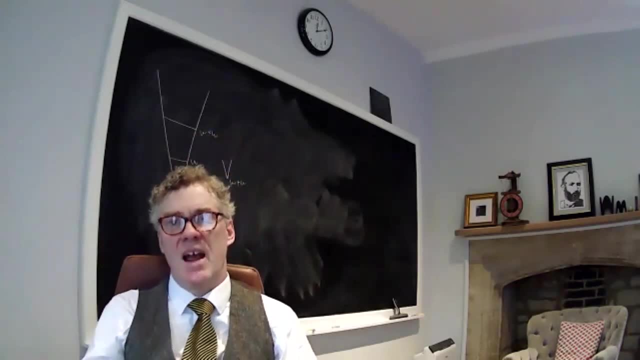 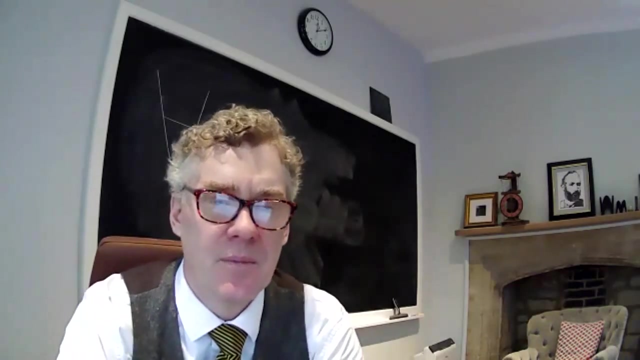 of these completely natural principles of infinite combinatorics and infinity existence assertions, And so it's really quite remarkable that we have this large cardinal hierarchy instantiating that phenomenon that we knew must be there from the Gödel incompleteness theorem. So it's not at all a problem that we can't prove. 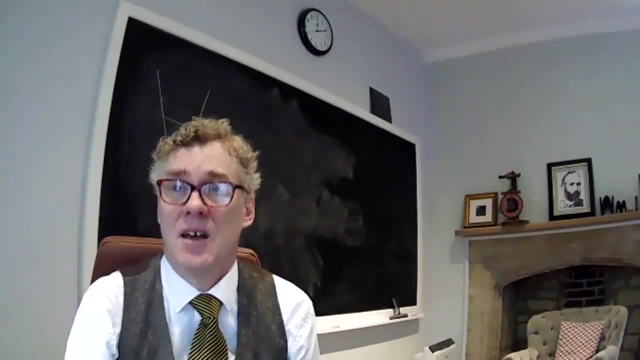 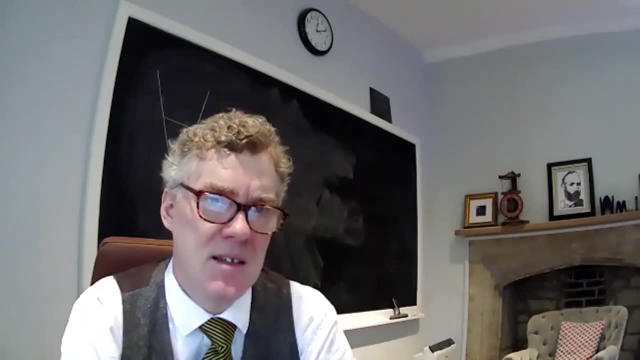 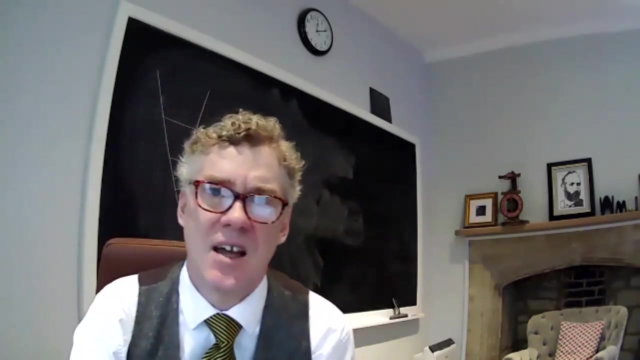 that they exist or that they're consistent. That's exactly what we expected in terms of this consistency hierarchy. OK, So One of the amazing features of the large cardinal hierarchy is that the existence of large cardinals have surprising consequences for sets down low. 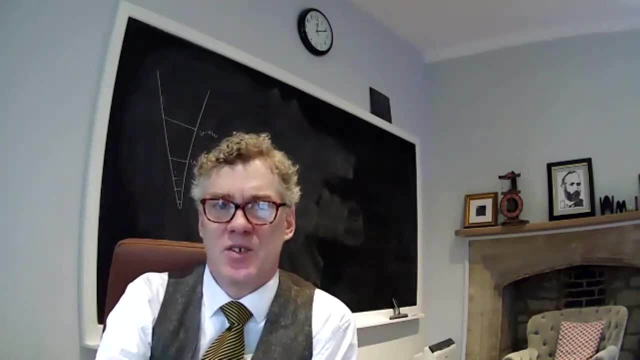 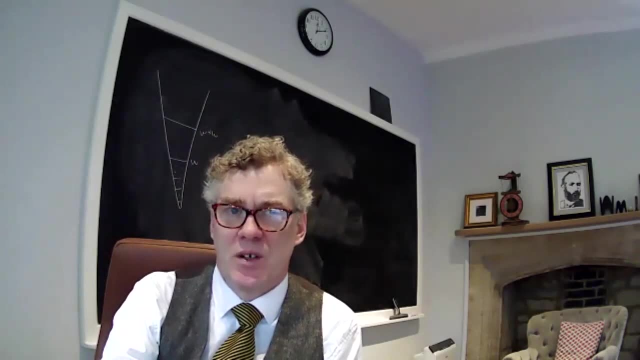 For example, if there's a measurable cardinal, then every sigma 1, 2 definable set of real numbers is measurable, And if there's a proper class of wooden cardinals, then every projectively definable set of real numbers is low-beg measurable and has the property of bear. 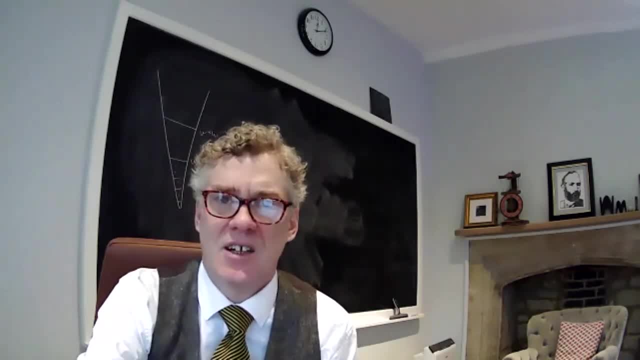 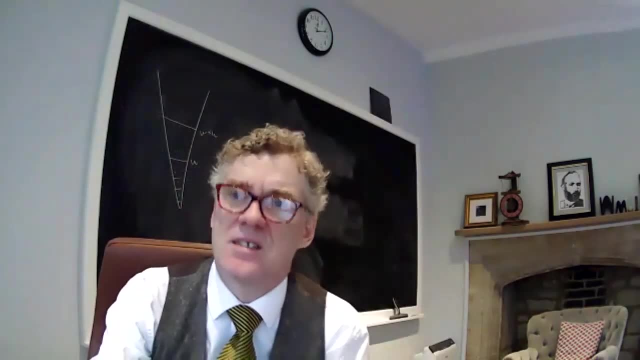 So this is just nothing short of astonishing, this connection between these extremely large infinities and definable properties for sets of reals. It's just incredible that these theorems are true And many set theorists take these kind of regularity. 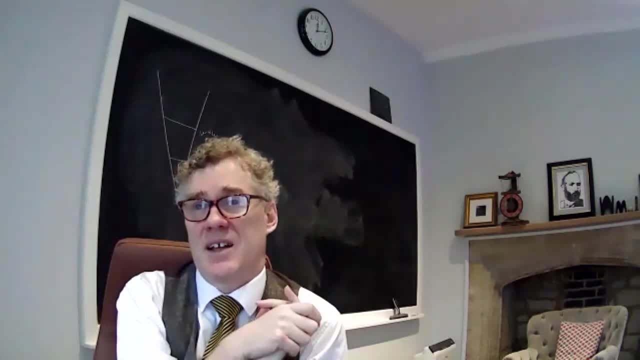 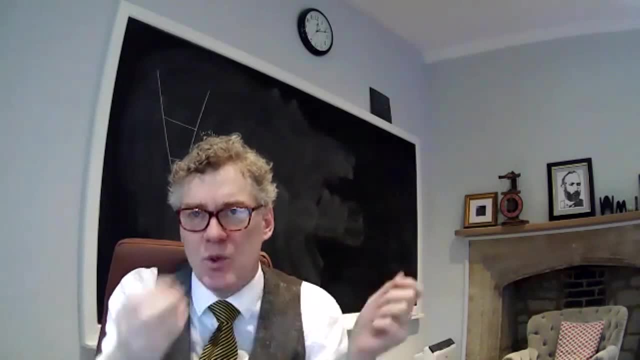 consequences to be evidence for the truth of the large cardinal axioms. They say it's a consequentialist view that the large cardinal axioms are true because we can prove from them that all of these great regularity properties hold that we like very much for sets of reals. 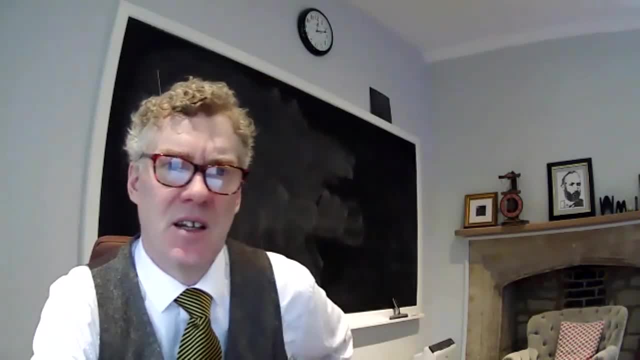 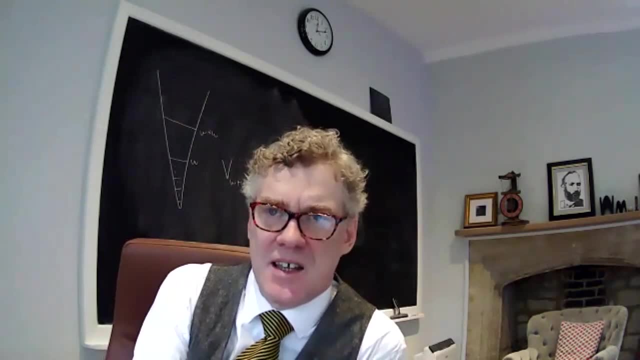 Let's turn to the continuum hypothesis. OK, OK, OK, OK, OK. So we had mentioned this in chapter 3.. So the continuum hypothesis. Cantor had noticed from the earliest days of set theory that essentially all of the naturally arising 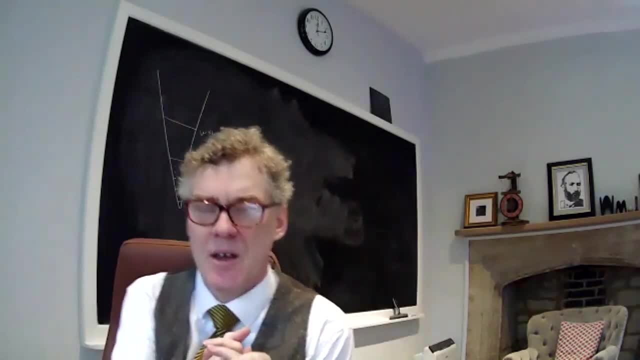 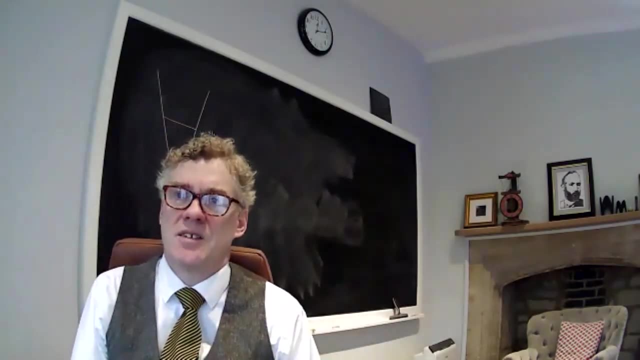 sets of real numbers are either countable or have the same size as the reals. So I mentioned already that he proved it for closed sets, but also not just closed sets, many other sets. we can prove in specific cases that either they're countable or they're. 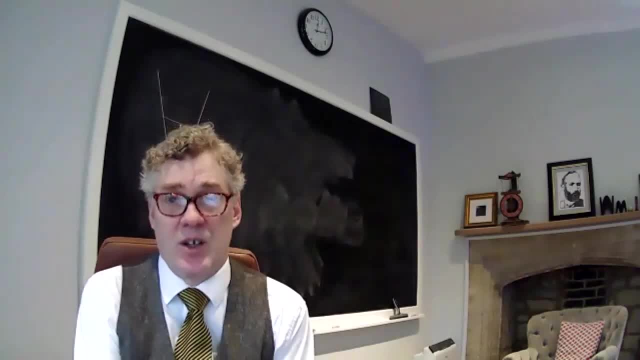 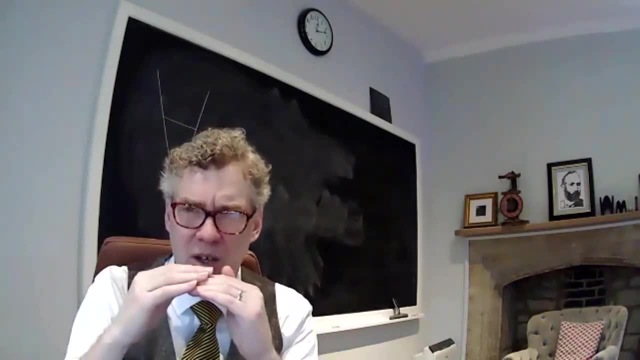 equinumerous with the real numbers. And so he had asked: is every set of real numbers, either countable or equinumerous numerous with the real numbers? Another way of asking this is: is there any infinity between the infinity of the natural numbers and the infinity of the real numbers? 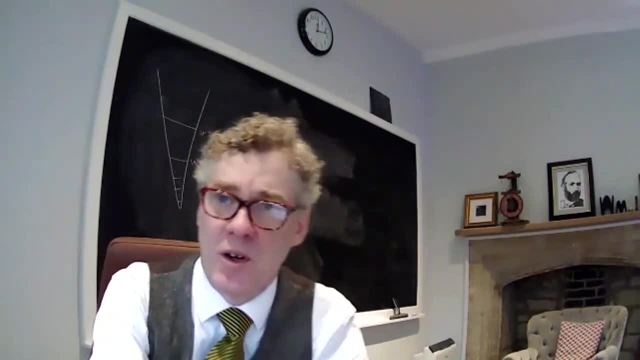 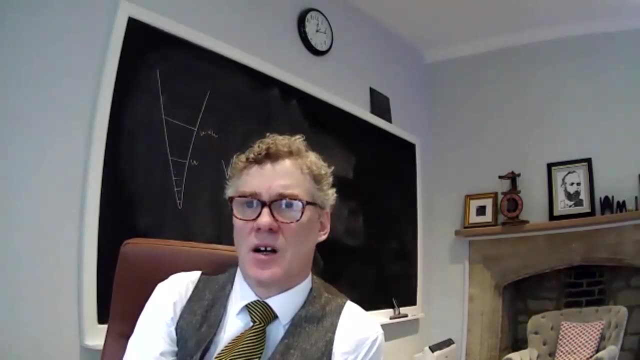 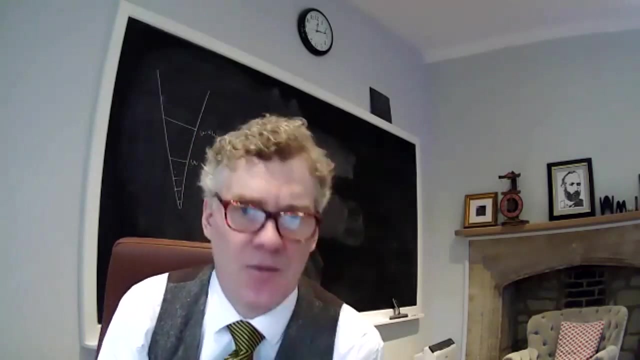 And in 1938, so this was open for decades after Cantor and it wasn't settled, partly even until 1938, when Gödel had constructed an artificial mathematical universe, a synthetic universe called the Constructual Universe, and proved that all of the Zermelo-Fraenkel axioms 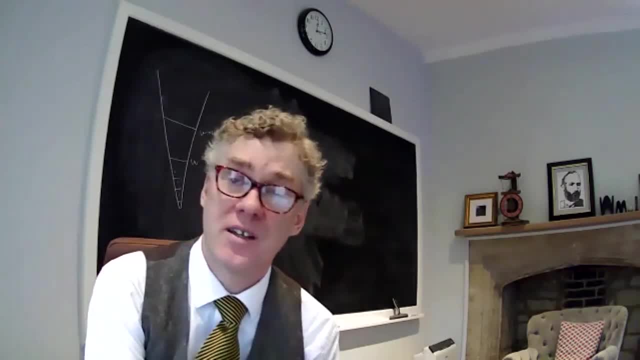 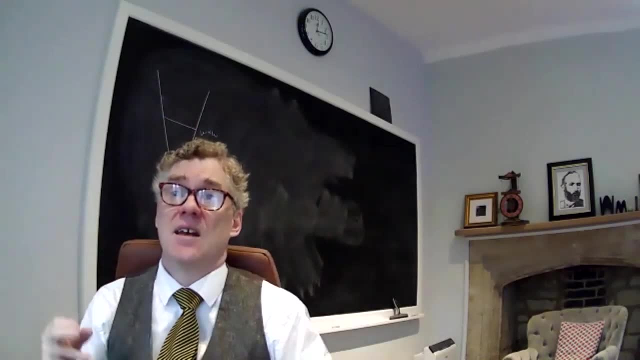 are true in the Constructual Universe, including the axiom of choice and also the continuum hypothesis. So he proved that both the axiom of choice and the continuum hypothesis are safe, in the sense that if they turn out to be inconsistent, it's because there will be an inconsistency. in set theory generally. even without those axioms They're no less safe than just the other axioms of set theory alone. But that doesn't quite answer it, because it's not like he proved that the continuum of hypothesis is true. He just proved that it could be true. 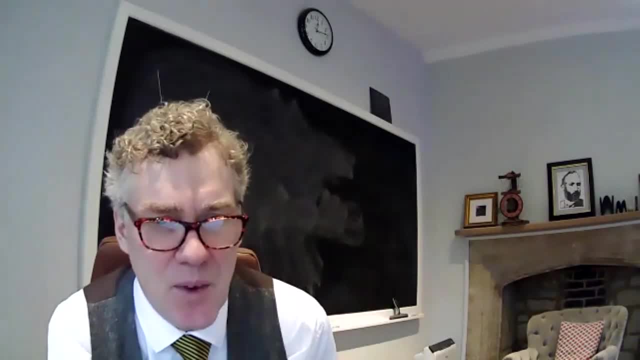 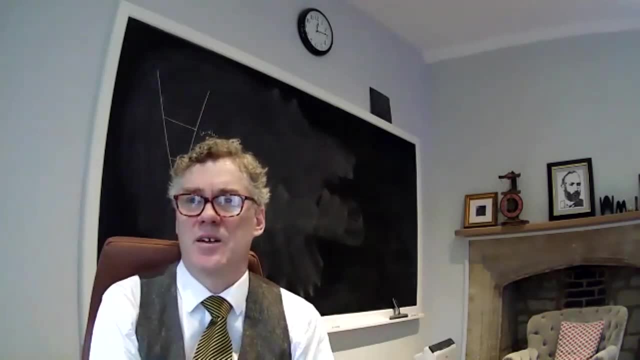 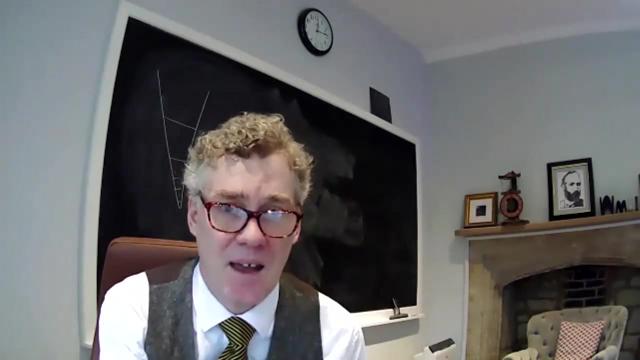 if we were in that, in that universe. So it waited until 1962, when Paul Cohen provided the complimentary answer. So he constructed another kind of mathematical universe, a synthetic universe, using the method of forcing. he invented the method of forcing to do it. 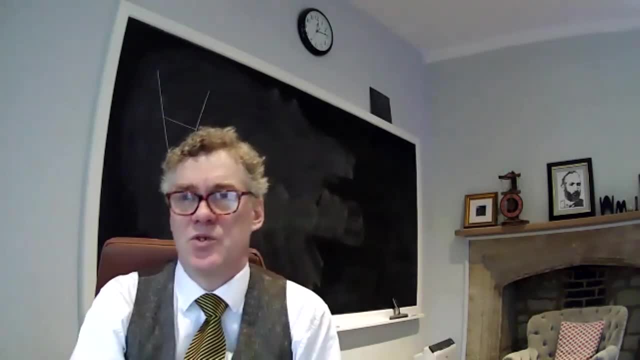 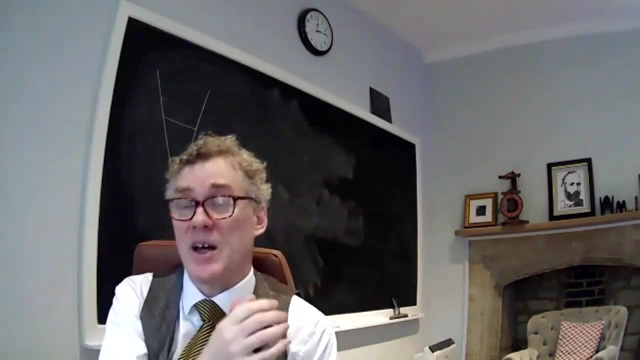 And in his model the Zermelo-Fraenkel axioms were true, with the axiom of choice, but CH was false. The continuum of hypothesis was false. So he showed how it could happen that the continuum of hypothesis fails. He also made models in which 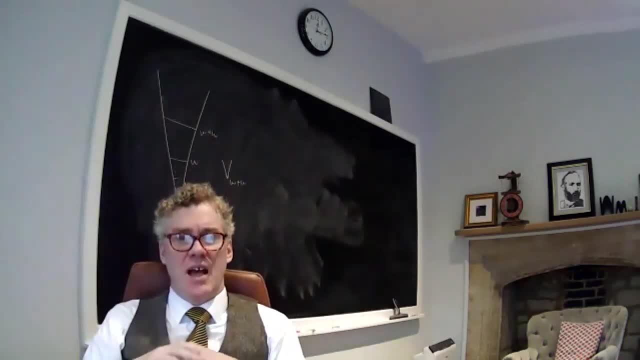 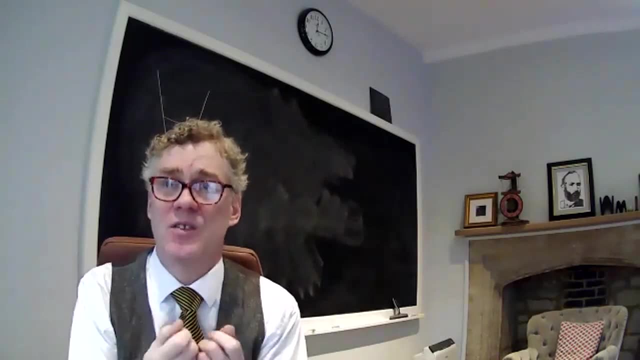 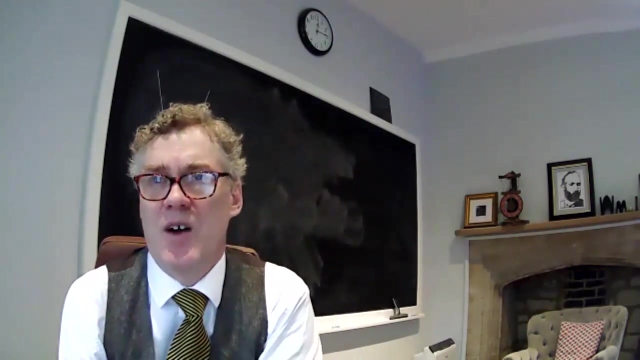 the axiom of choice fails. So what it means is that both the axiom of choice and the continuum of hypothesis are independent of the Zermelo-Fraenkel axioms. We cannot prove them and we cannot refute them either. And and subsequent developments in set theory identified. 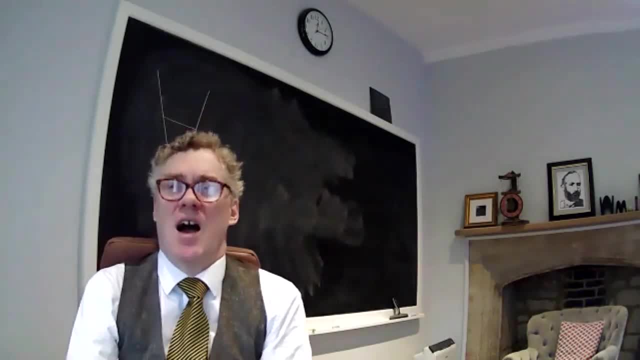 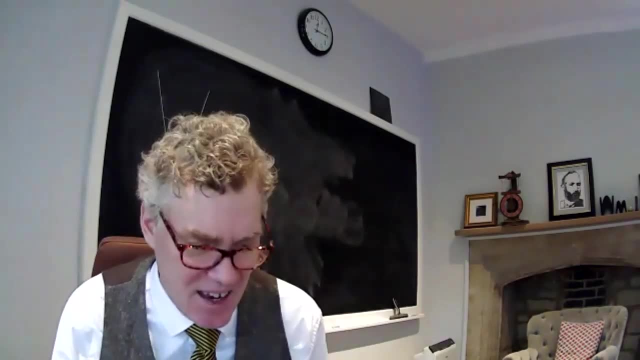 nothing less than a pervasive independence phenomenon. We have hundreds, maybe thousands of different, well, infinitely many, I guess. if you, if you schematize it So, practically, every statement, every statement of infinite combinatorics is either trivial in the sense that you can prove it easily. 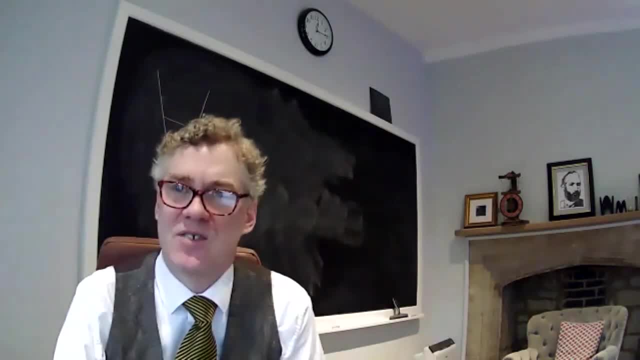 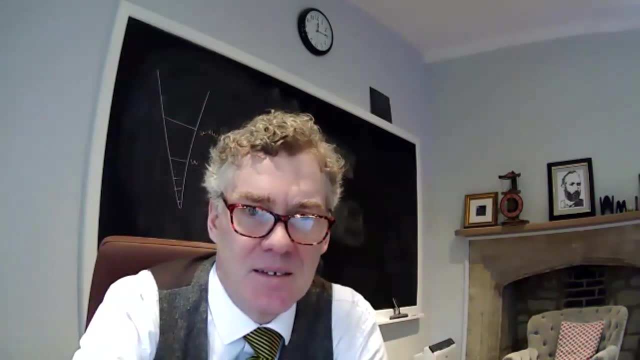 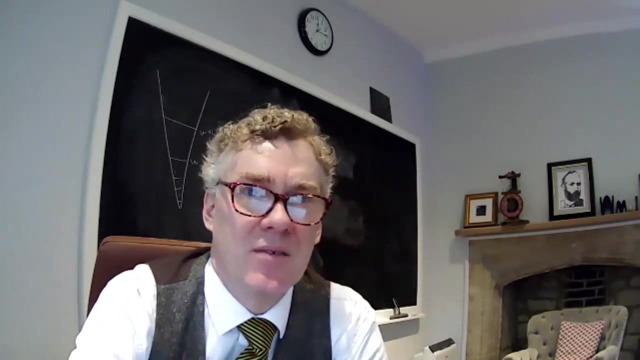 or else it's independent. We have dozens, hundreds thousands of statements, natural statements that are independent of the Zermelo-Fraenkel axioms. So okay, so this is. maybe one should think of it as the principle set theoretic discovery. 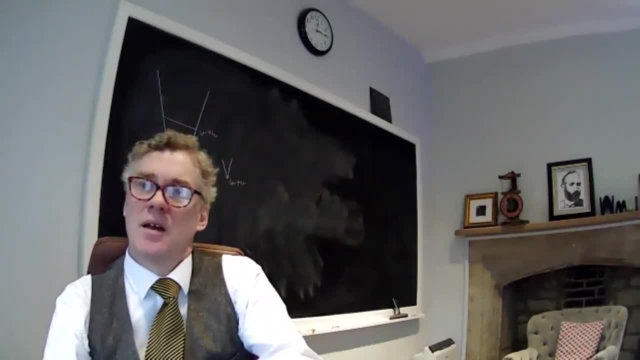 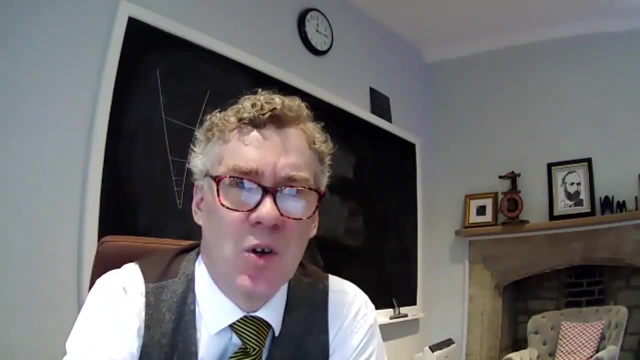 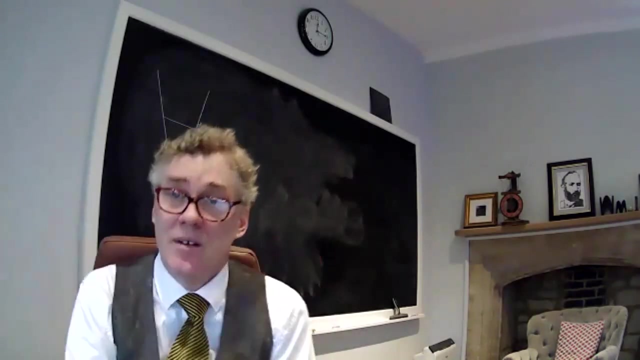 of 20th century research is the pervasive independence Phenomenon. Almost everything is independent. Okay, so fine. We can't prove this continuum of hypothesis and we can't refute it, but still, maybe mathematicians want to know, is it true? 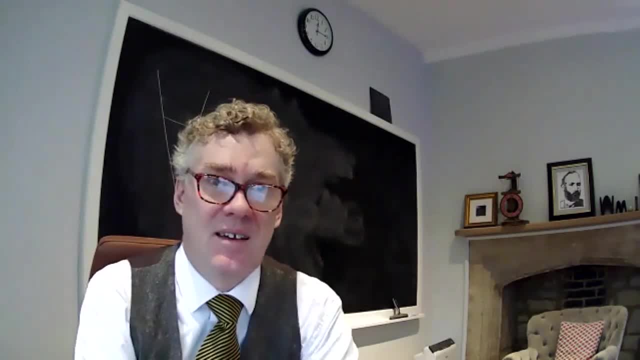 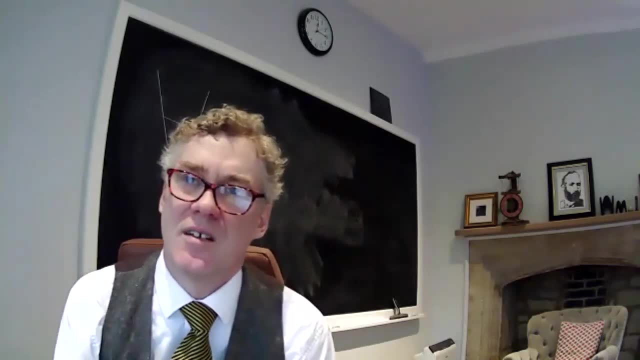 Is the continuum of hypothesis true or not? And that might seem like a sensible question at first, although it's it's a very difficult, has very difficult philosophical problems. What do we mean by true there? Well, of course, many set theorists have the idea that this: 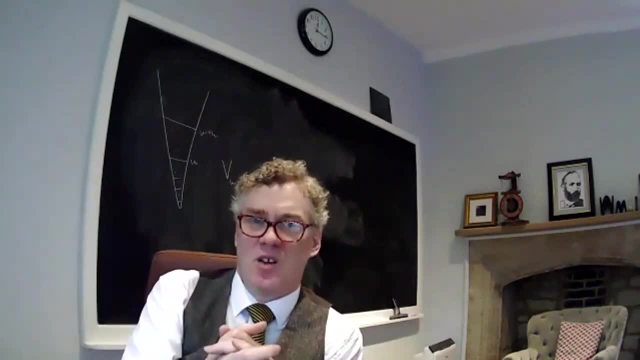 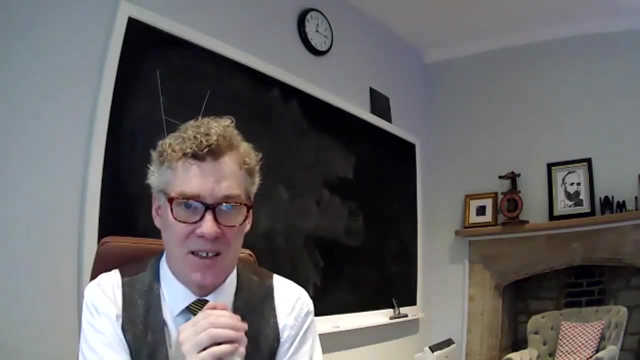 is a definite set, theoretic reality, a determinant world full of actual sets in which all the CFC axioms are true and more, And so this view is realist, right- The set, theoretic objects have a real existence there- but also singularist in the sense that there's a unique set. 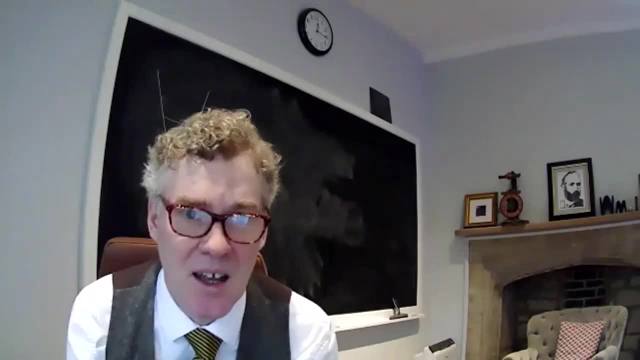 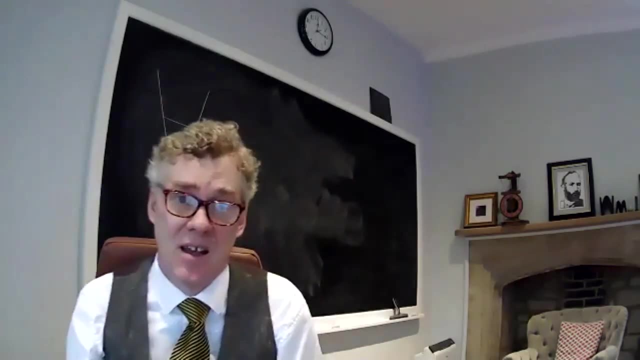 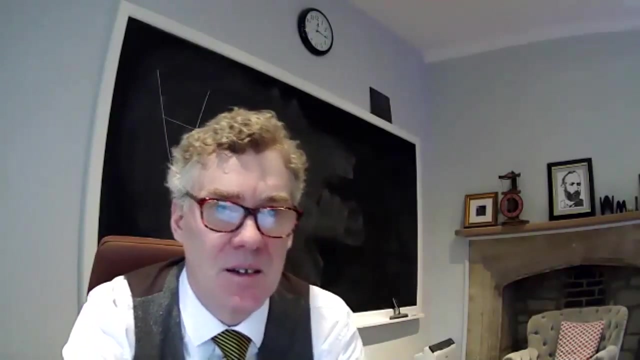 theoretic universe that we're trying to axiomatize, a unique intended interpretation, And to ask: is the continuum of hypothesis true? is really to ask: is it true there in that intended model? Yes and so so let me just mention that the Zermelo-Fraenkel theory 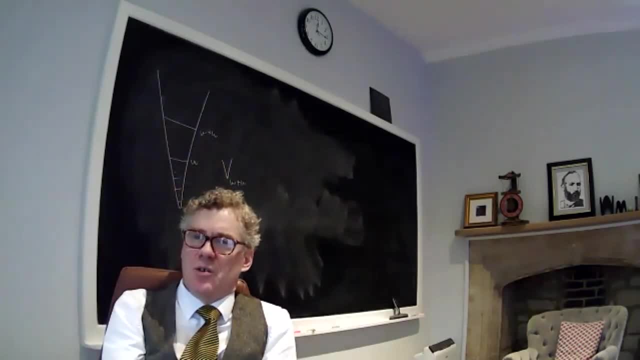 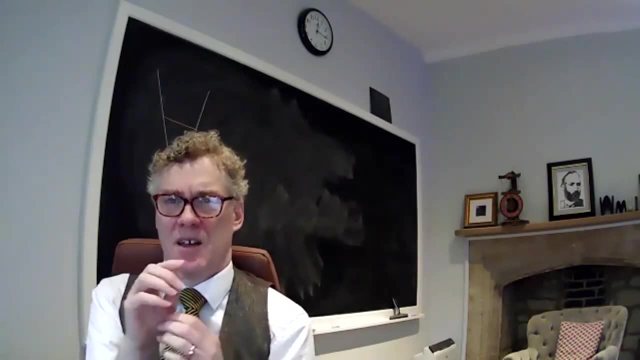 proves the rigidity of the set theoretic universe. You can prove that there's no automorphism of the cumulative of the sets appearing in the cumulative hierarchy. You can prove that because, if you had an automorphism, you can prove that there can't be a first stage. 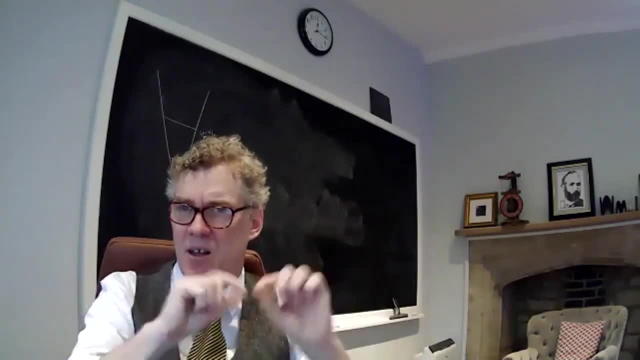 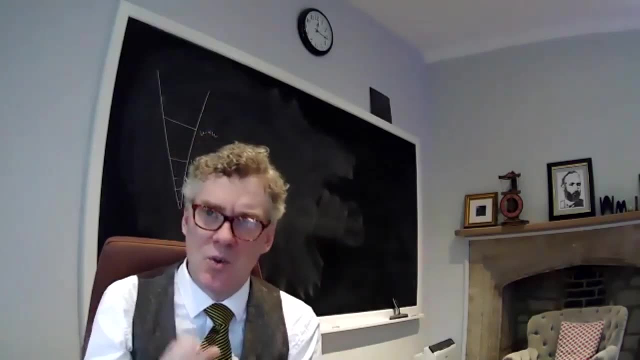 at which sets are moved, because then they all, the previous elements, would have to be fixed. And so the sets are sort of determined. You can't swap any two, You can't change them at any level. So you can prove sort of recursively. 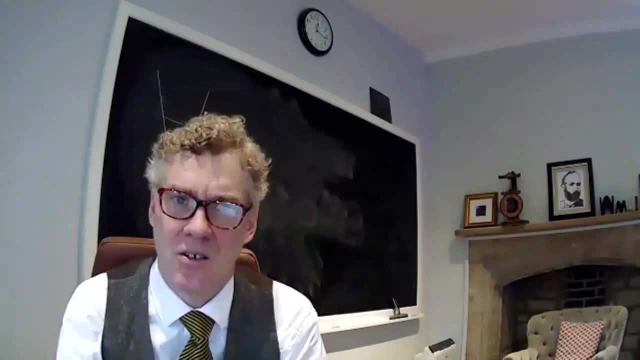 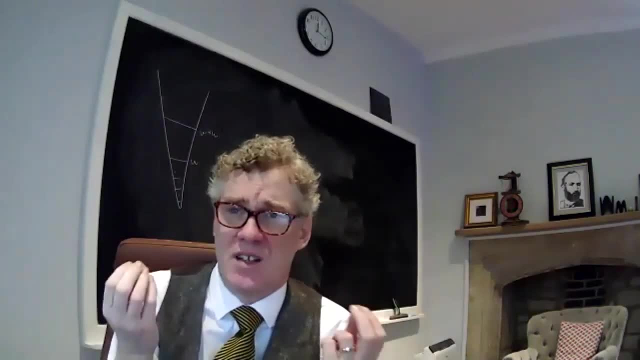 that any automorphism is actually the identity on every single set. And what that means, for example from the sort of structuralist point of view, is that in set theory any two different sets play different structural roles. They have a different isomorphism orbit. 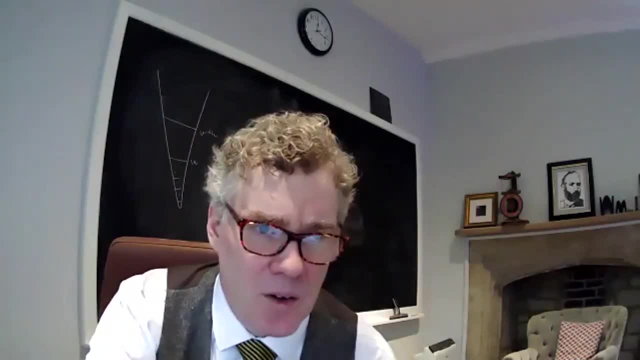 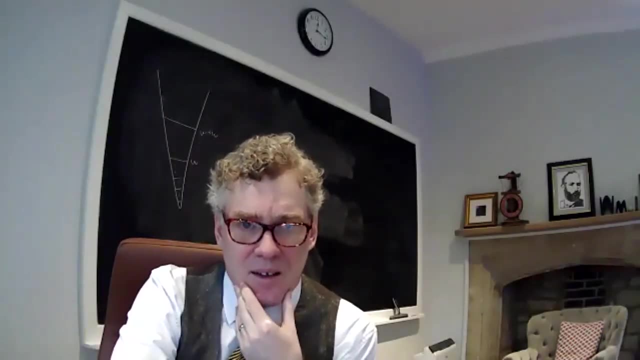 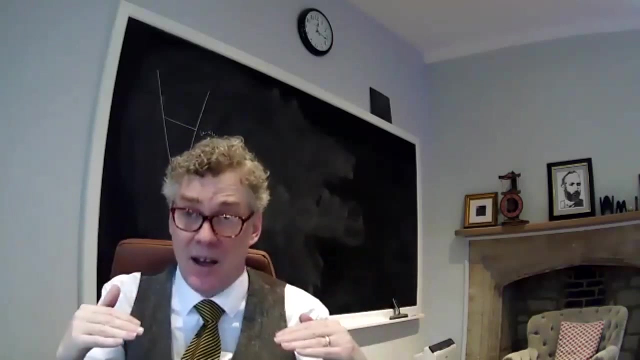 as an internal matter. Now, Martin, Tony Martin argued on essentially similar grounds that there cannot be more than one concept of set, because if we had two different concepts of set, then we could match them up by comparing their cumulative hierarchies, If the two concepts agree up to this level. 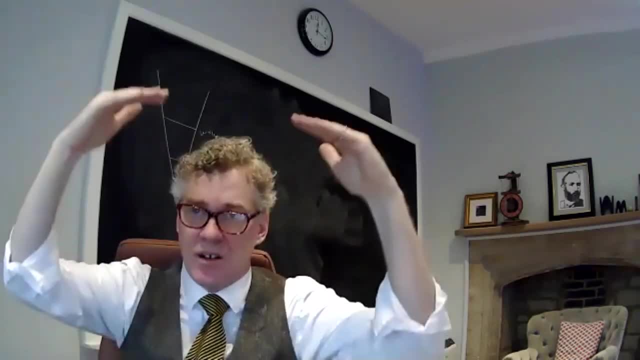 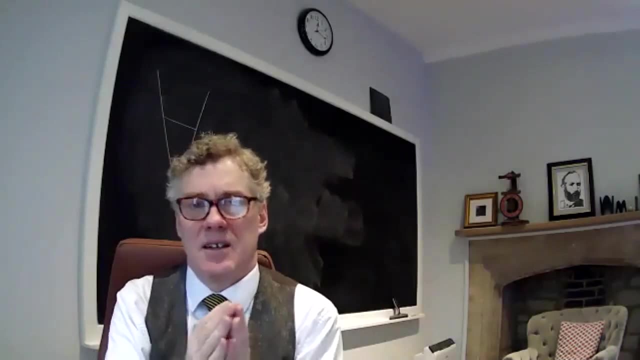 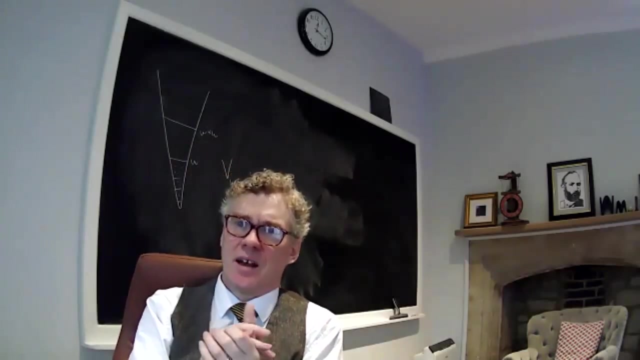 of their cumulative hierarchies, then they would have to agree on the next level, and so on. Okay, so there's a kind of similar point made by Chrysler, namely that because the set theoretic universe is determined in second-order logic by the second-order Zermelo axioms, 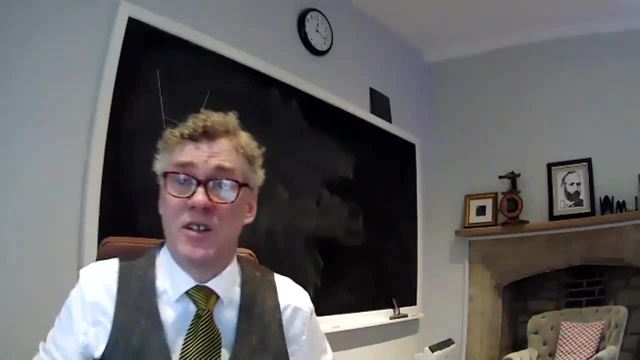 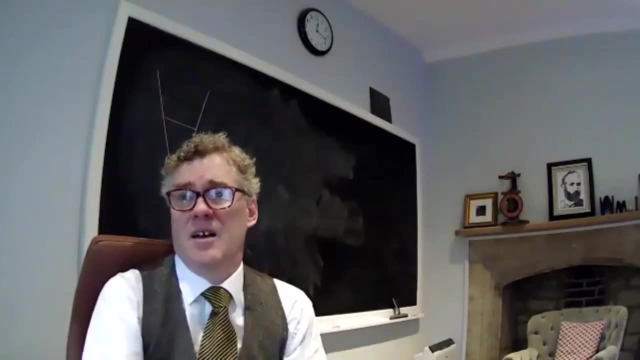 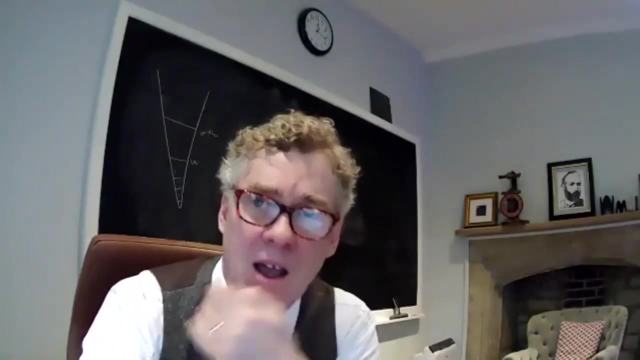 it follows that, say, the continuum hypothesis has a determinant truth value. The truth value of the continuum hypothesis is determined by second-order logic, because the truth value of the continuum hypothesis is revealed in level omega plus two in the cumulative hierarchy. Now critics view that as sleight of hand. really, 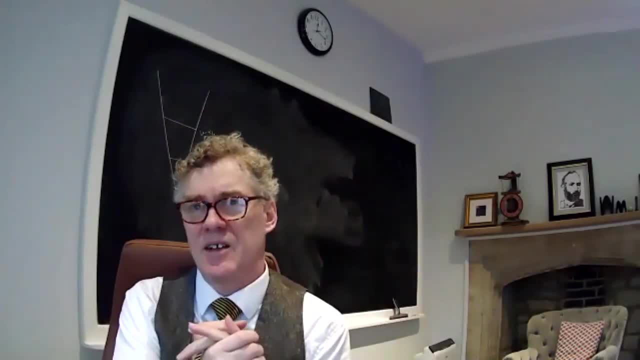 because to talk about the sort of second-order logic amounts to set theory itself in the meta theory. and so, according to Chrysler, we have a determinant truth value for CH, but we don't know which it is, because in fact we don't know which sets there are exactly. 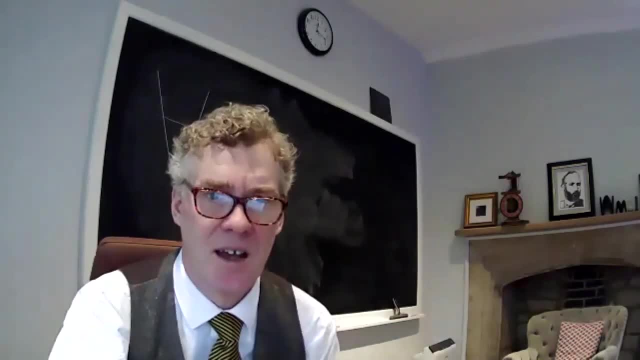 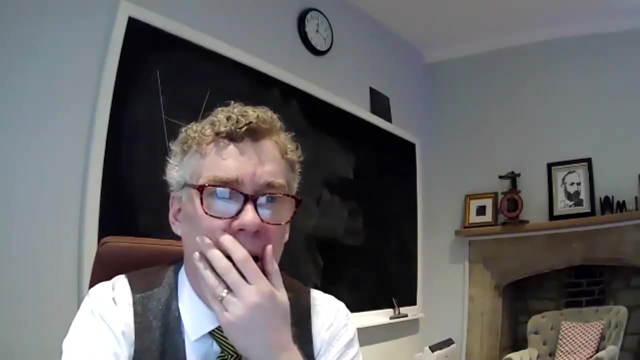 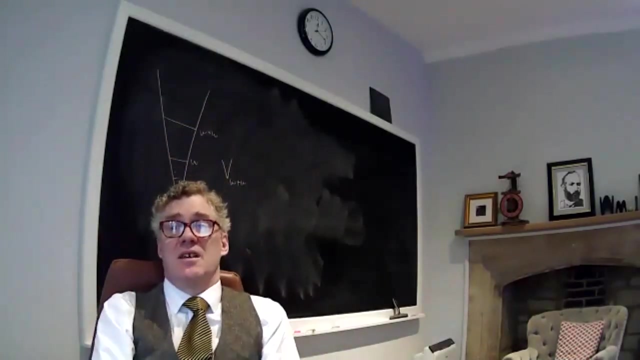 and it's amounting to the sort of independence of CH in the meta theory as a first-order matter, and so there's definitely criticisms. Okay, so what is the criteria by which we are to adopt new axioms, and can we settle the CH by adopting new axioms? 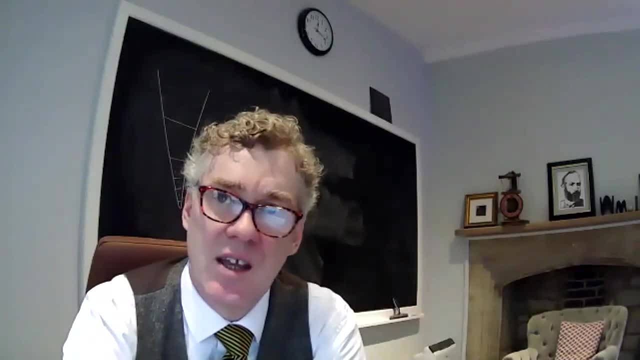 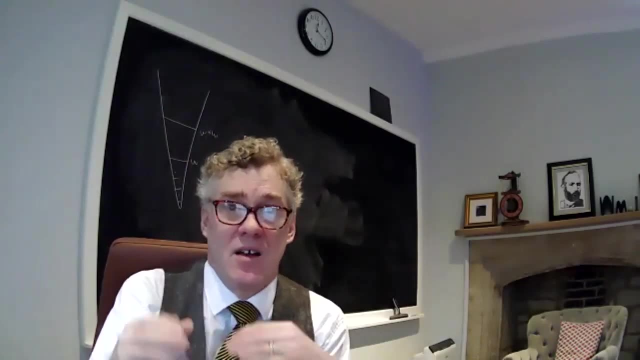 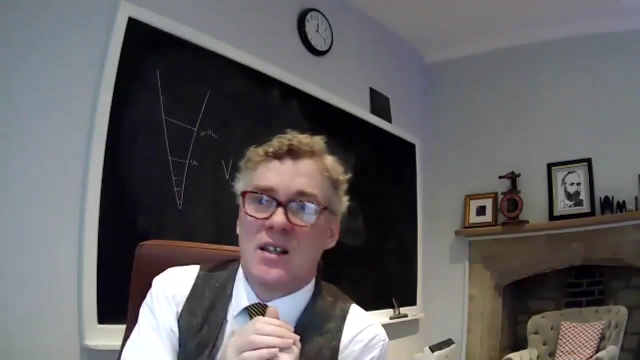 Well, one should compare the sort of intrinsic justification for axioms with extrinsic justification. so the intrinsic justification would be in support of axioms that are in accordance or conformance with our initial concept of set. so we would adopt intuitively clear principles about sets. 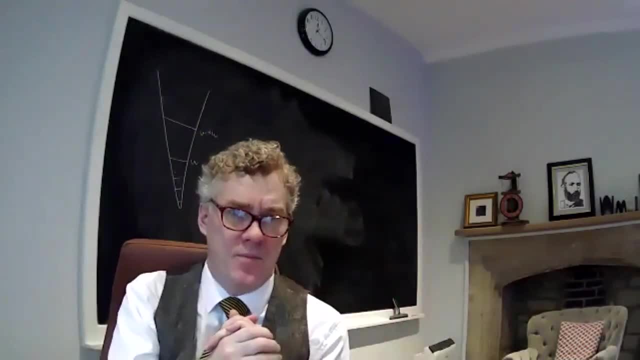 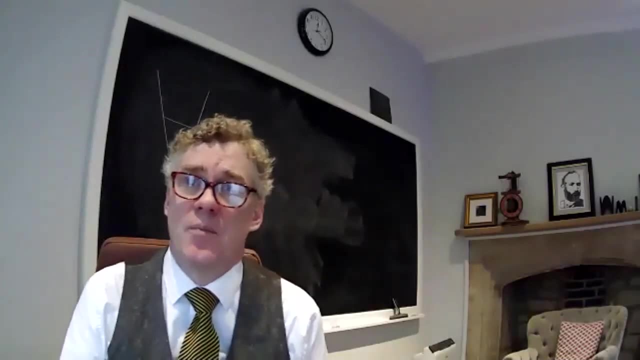 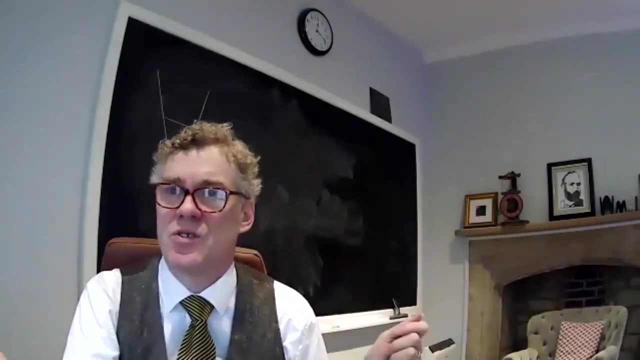 like extensionality and union and pairing, set and so on, and maybe even the axiom of choice, can gain support from intrinsic support, Because we have an intuitively clear concept of set, by which all the possible sets exist, including the ones that make those choices. 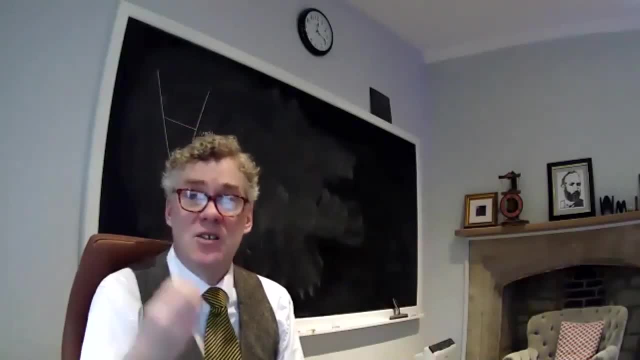 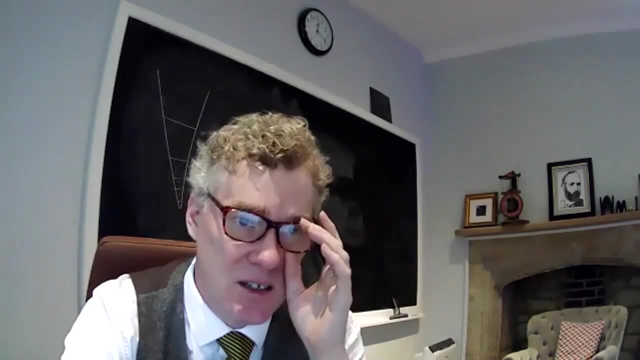 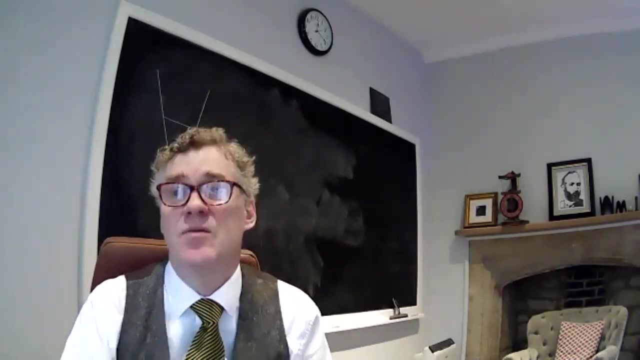 that the axiom of choice is asserting, and so one can find intrinsic grounds on which to view the axiom of choice as true. So we can contrast that with extrinsic justification, by which we judge an axiom by means of its consequences and what you can prove from that axiom. 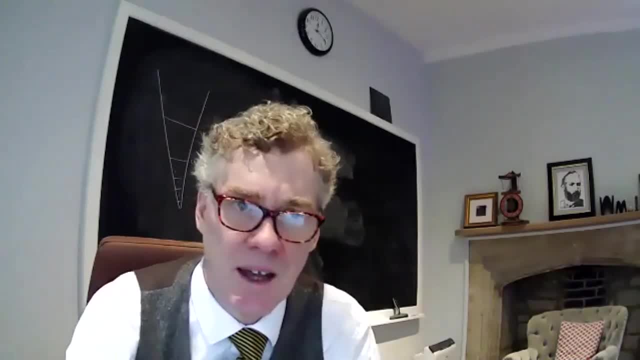 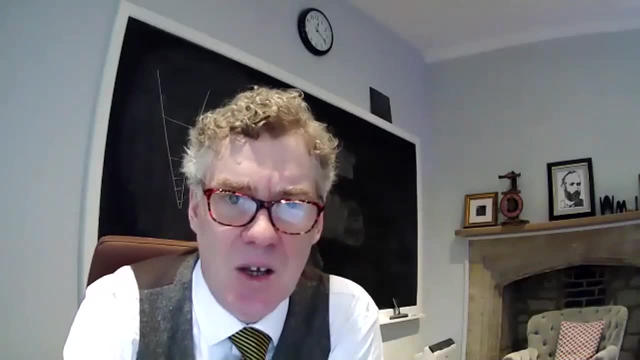 even if maybe we're lacking direct intrinsic support for the axiom. So Gödel had written on this idea by saying: famously there might exist axioms so abundant in their verifiable consequences, shedding so much light upon a whole discipline and furnishing such powerful methods. 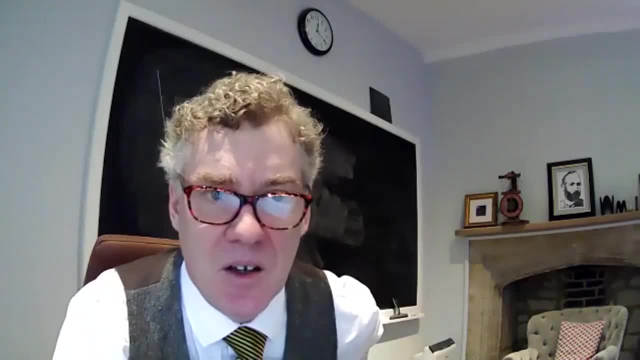 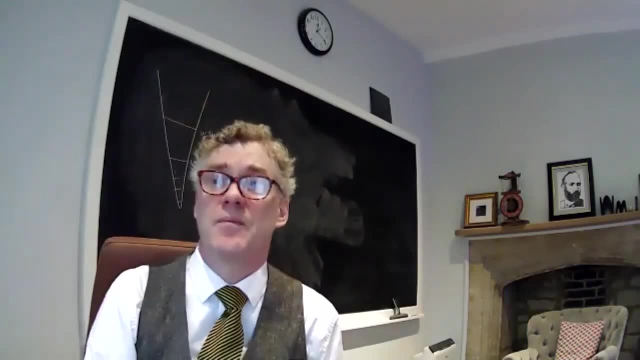 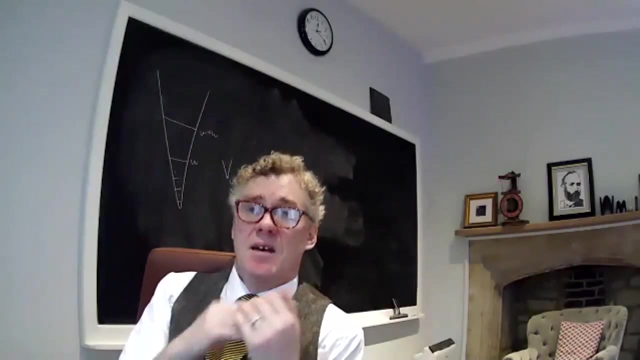 for solving given problems that, quite irrespective of their intrinsic necessity, they would have to be assumed at least in the same sense as any well-established physical theory. And so many of the large cardinal hypotheses fulfill that vision in many respects, Precisely because of those regularity consequences. 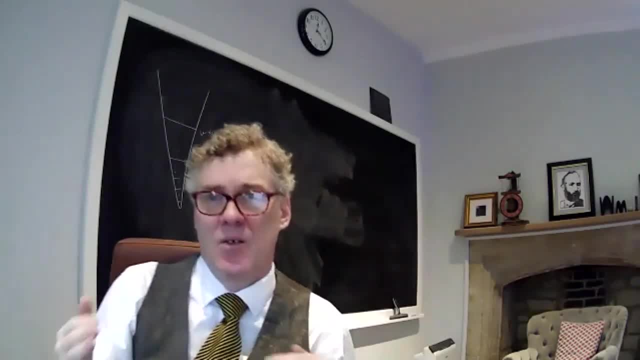 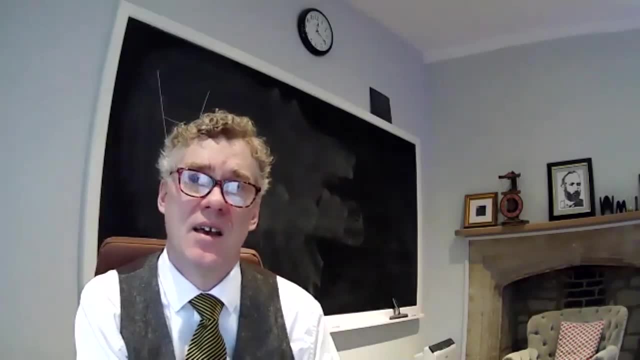 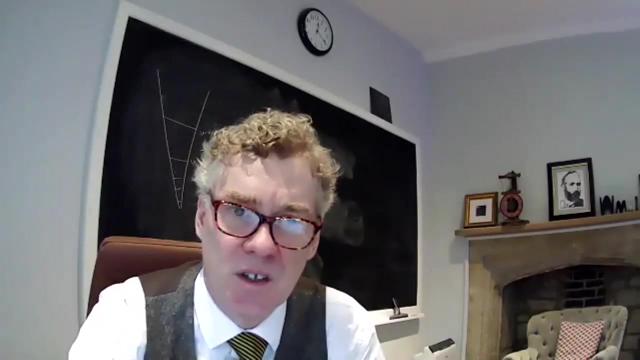 of the large cardinal axioms, and many instances of those regularity consequences are observed in practice. So we have independently verified instances of the consequences of those axioms, And so one can view that as extrinsic support for the truth of the large cardinal axioms. 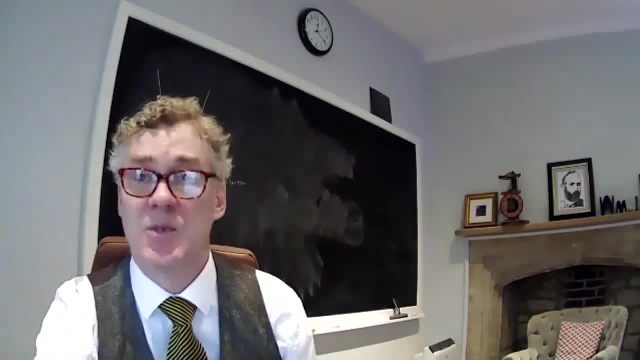 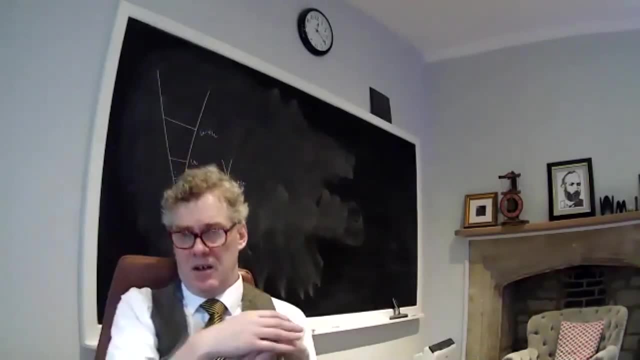 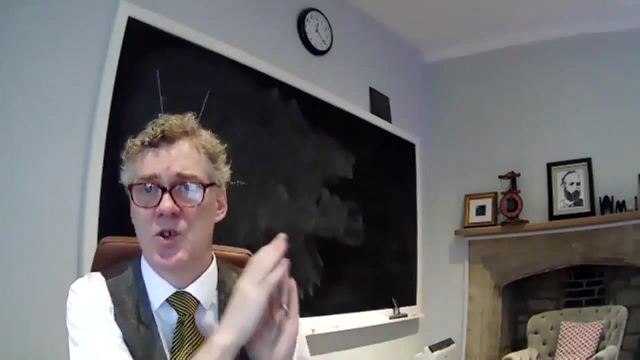 Now, Gödel had hoped that large cardinals would settle the continuum hypothesis, but this is now known not to be Correct. using the method of forcing we can prove that any of those large cardinal notions I mentioned before cannot settle the continuum hypothesis, because we can preserve those large cardinal notions. 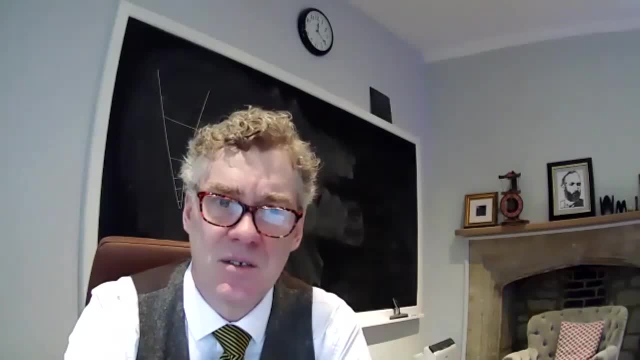 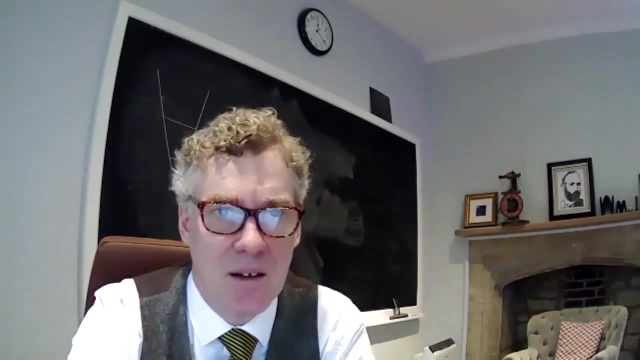 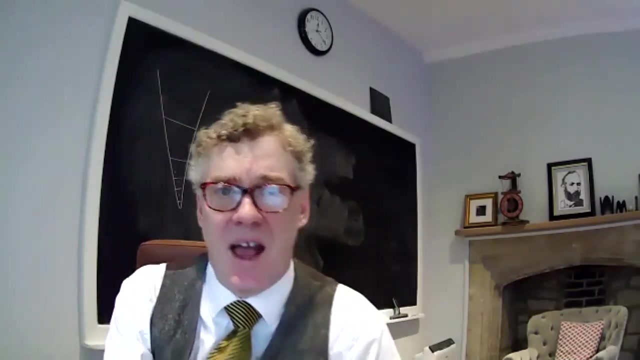 by forcing that either forces CH or the negation. So what is an axiom? What does it mean to adopt an axiom? There's been really a shift in the meaning of that term over the years, So formerly, of course, an axiom meant a self-evident truth. 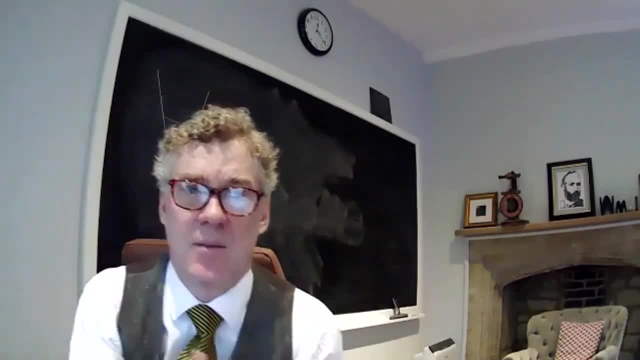 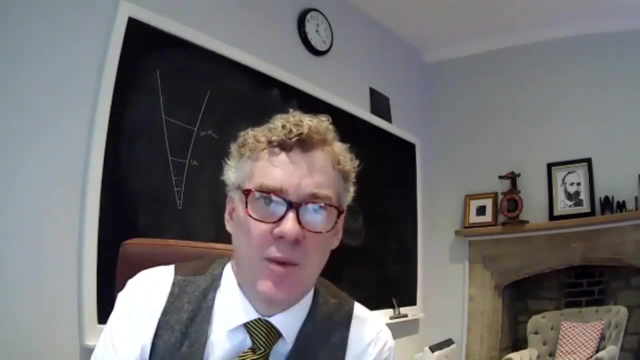 If you have a fundamental theory, then an axiom is a fundamental, rock solid truth about which we don't question. So, in geometry, Euclid's axioms are expressing the most fundamental geometric truths. Dedekind's axioms are expressing the central core. 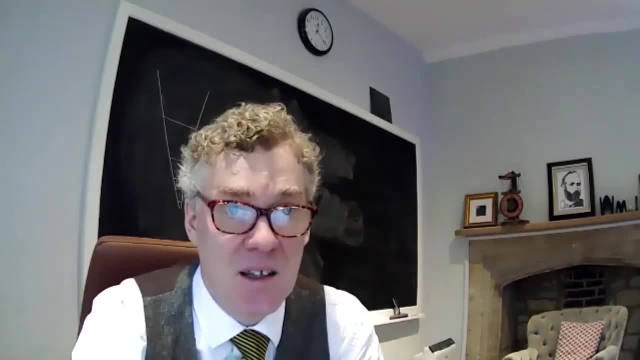 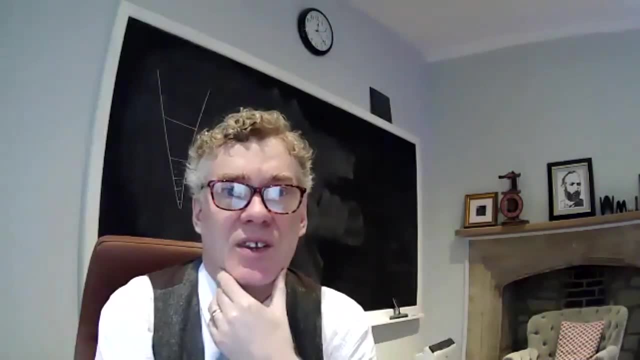 of our beliefs about the natural numbers. Zermelo's axioms are expressing the fundamental truths about the concept of set, But really contemporary set theory has become awash with diverse axioms That often stand in conflict with one another. So we have Martin's axiom. 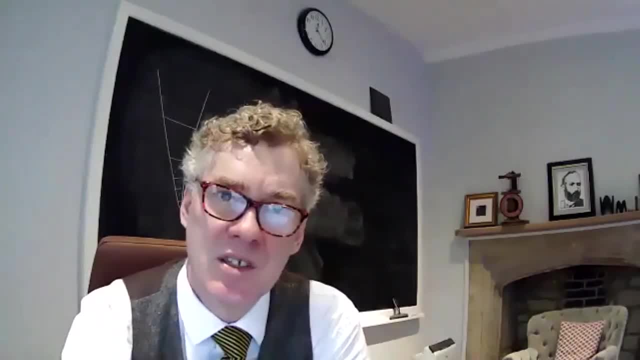 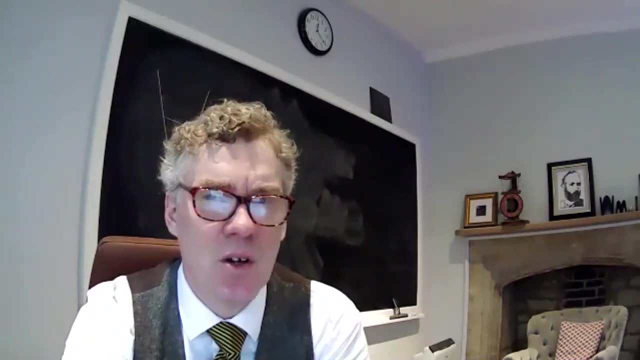 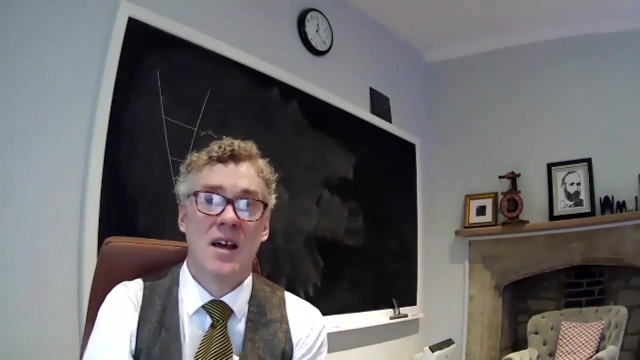 the axiom of constructability, axiom of determinacy, diamond axiom, square principles, large cardinal axioms, ground axiom, and so on. So really, the word axiom has come to mean something like a concise, fundamental principle whose consequences are to be studied. It's not carrying the connotation of self-evidently true. 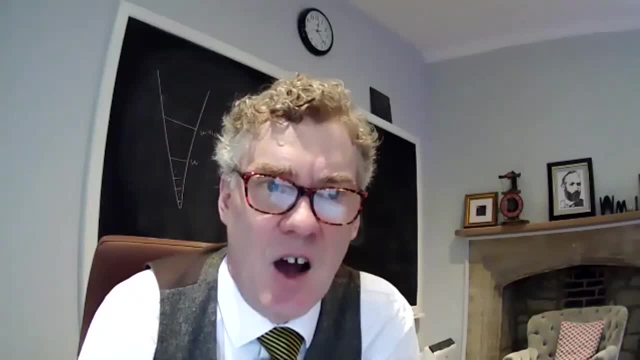 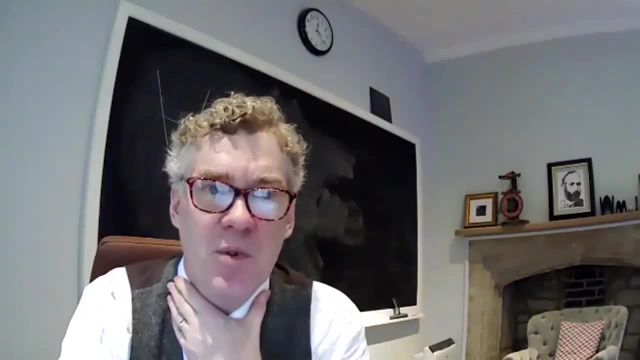 Now Pfefferman despairs of this usage. He writes: it's surprising how far the meaning of axiom has been stretched from the ideal sense in practice, both by mathematicians and logicians. Some even take it to mean an arbitrary assumption and so refuse to take seriously what purpose axioms. 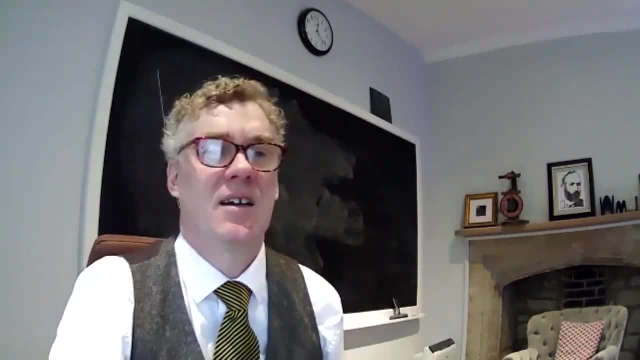 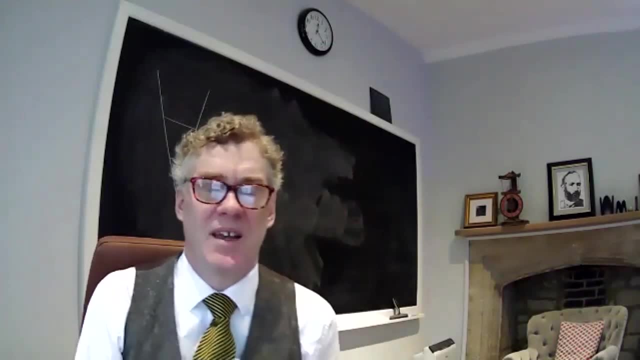 are supposed to serve. Okay. so on the other side, to my way of thinking, really, this new usage arises directly from the case of geometry, where we had the Euclidean axioms- okay, And they had the status of self-evident truths. 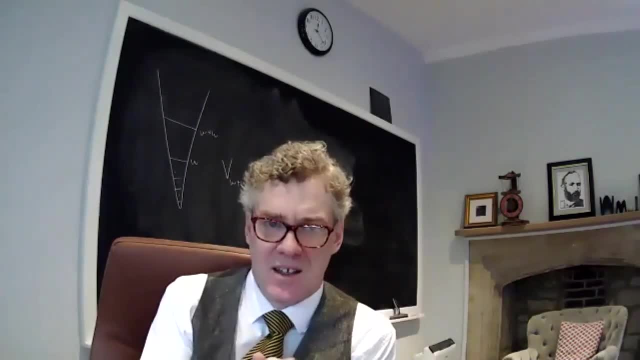 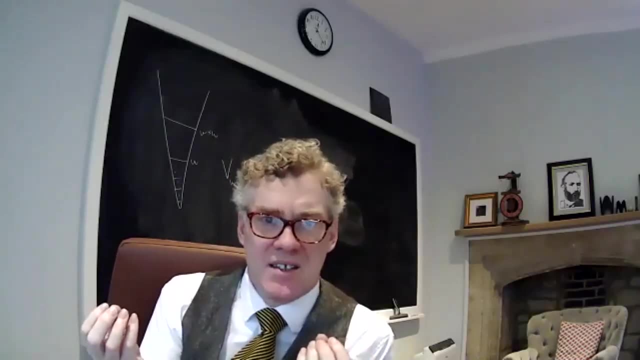 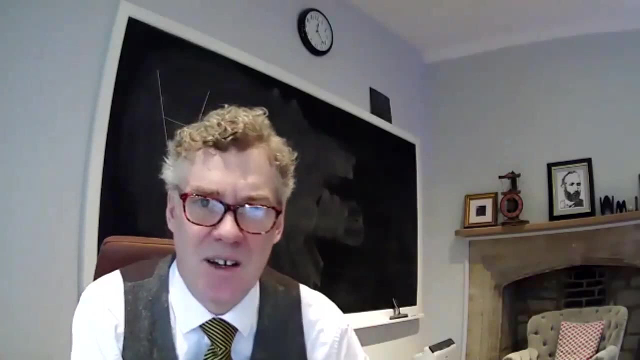 until the discovery of non-Euclidean geometry, of course, tempted us to the alternative incompatible axiomatizations. And so now in geometry, we're considering diverse theories. Each of them has axioms, but those axioms are in conflict with one another. 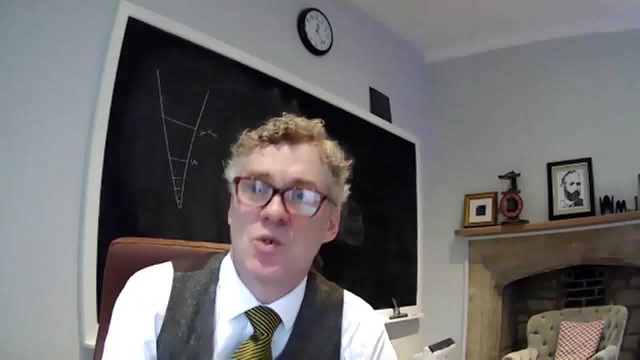 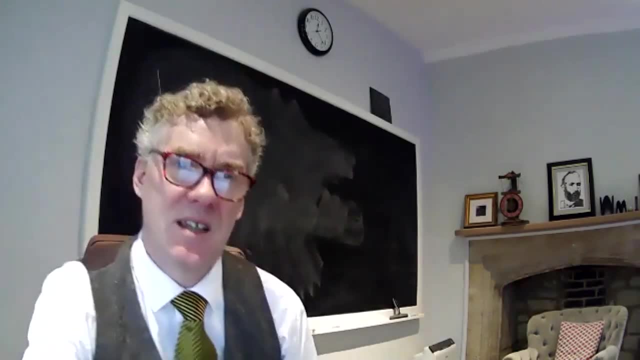 And so we no longer think that there's an absolute geometric truth about whether the say parallel postulate is true. Is it a fundamental truth or not? Well, in Euclidean geometry it's an axiom, but in non-Euclidean geometry it's not. So we're not going to be able to say: oh well, this is true, It's a fundamental truth, or not? Well, in Euclidean geometry it's an axiom, but in non-Euclidean geometry it's an axiom. 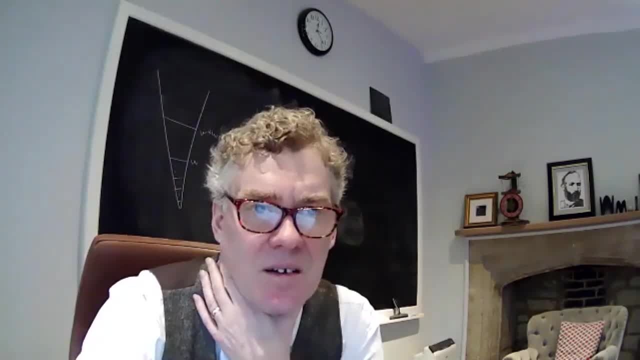 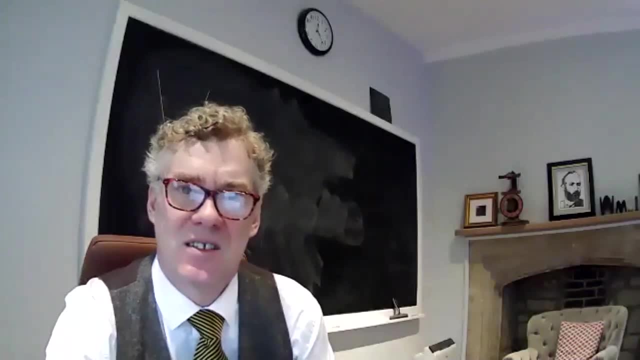 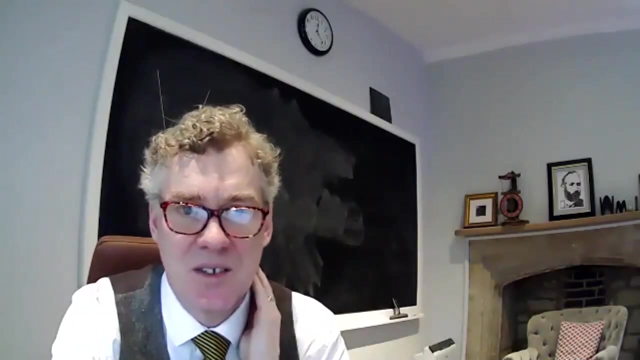 It's a fundamental truth or not? Well, in Euclidean geometry it isn't, The negation is. So, rather, the role of the axioms is to identify succinctly expressed geometric assertions that point at the differences in the theory, And so this is the contemporary use of the axiom. 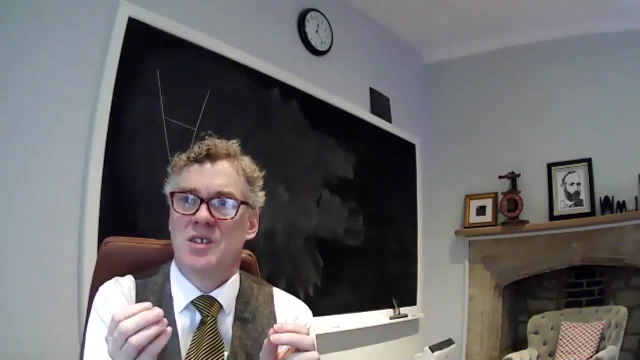 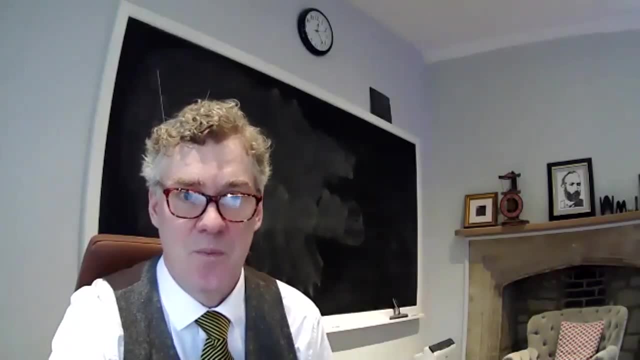 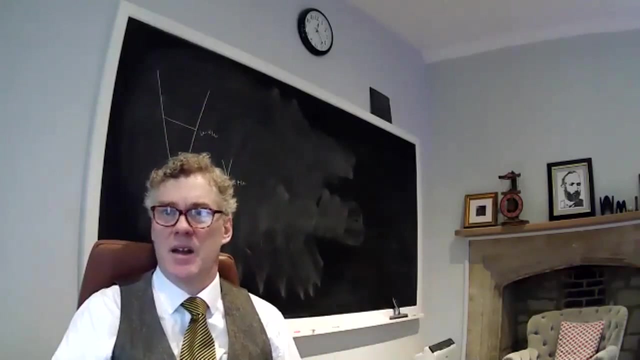 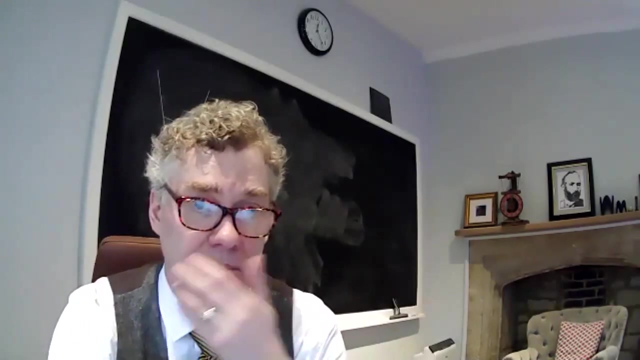 So in set theory we identify clear statements of principles, set theoretic principles that have interesting consequences, And that may be true, but we're not asserting that they are self-evidently true. Okay, so we have this vast spectrum of set theoretic possibility. because of the independence phenomenon, practically everything is independent and we want to know how should we extend our theory so as to add new axioms, and by what criteria should we be using? should we be doing so? 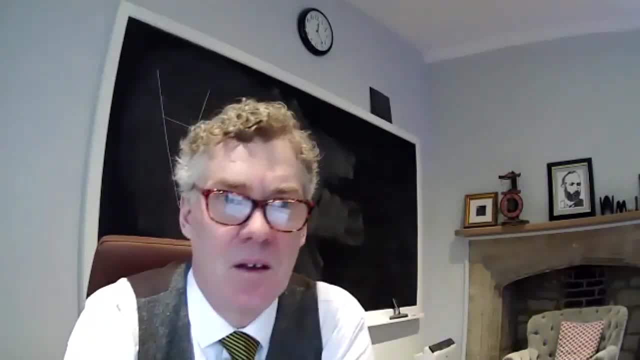 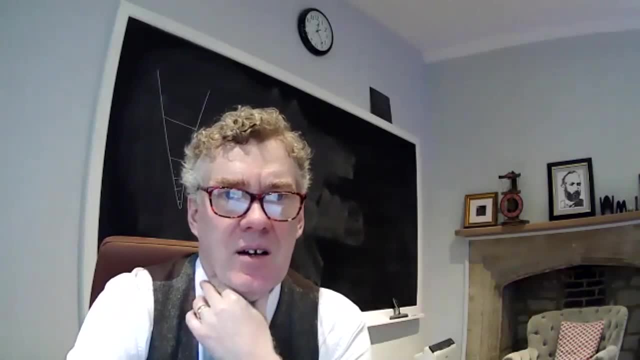 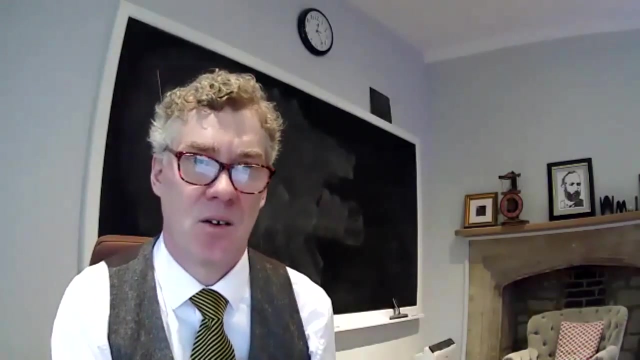 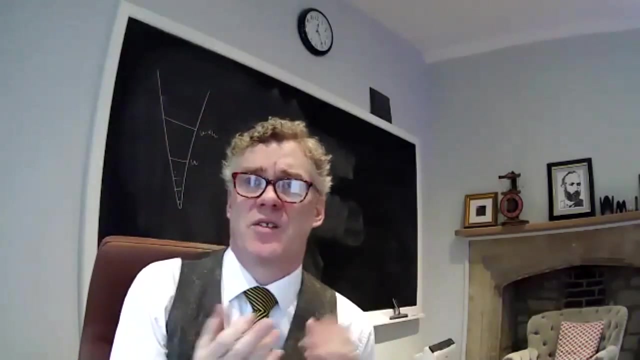 So so okay. so one of the central unresolved questions that I find to be at the core of the foundational dispute is the question of whether it's better to have strong axiomatic foundation or a weak one. So, for example, you can easily find mathematicians objecting to the replacement axiom by saying: look, we don't need the replacement axiom for most of the development of classical mathematics. 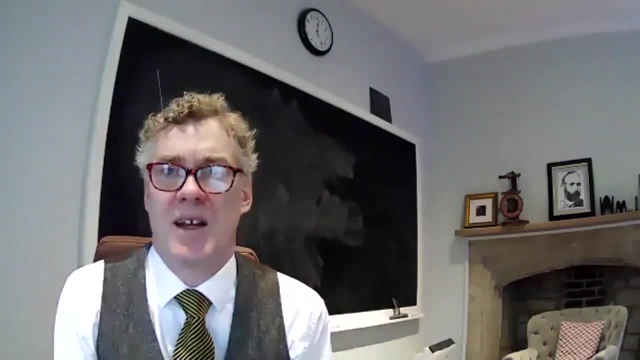 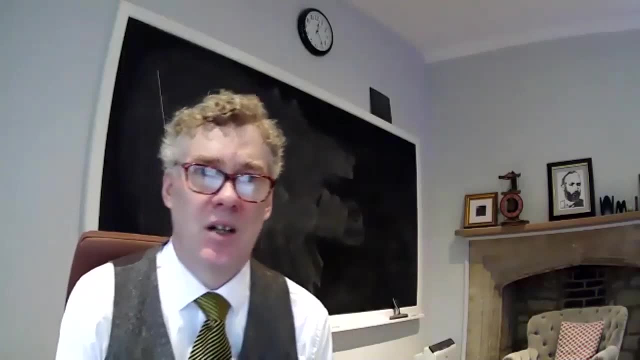 So the vast bulk of mathematics can take place in a much weaker axiomatic framework without the replacement axiom, and we can just work in Zermelo's system, or even much weaker. and so is that a good thing to get rid of the replacement axiom, or do we want? 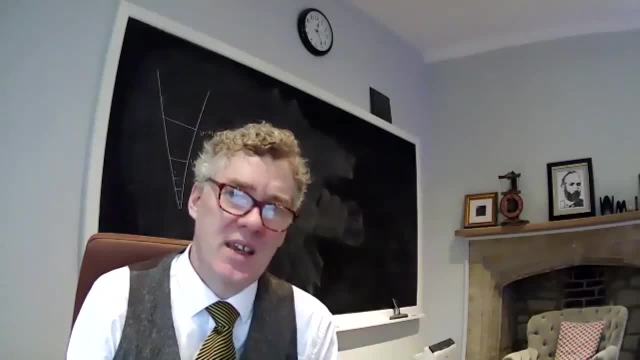 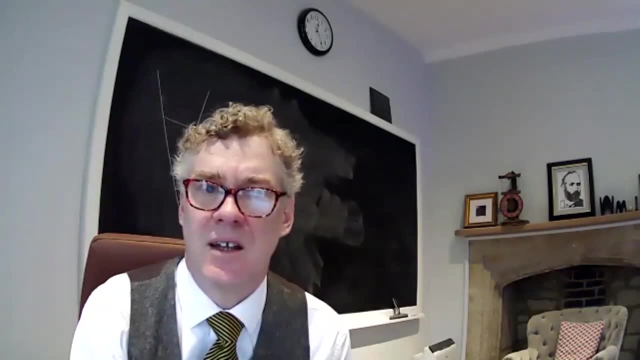 So do we want the axiom system to be as weak as possible or as strong as possible? So Steele argues that the strongest foundations will win out in the end, not the weakest. So he says what is important is just that our axioms be true and as strong as possible. 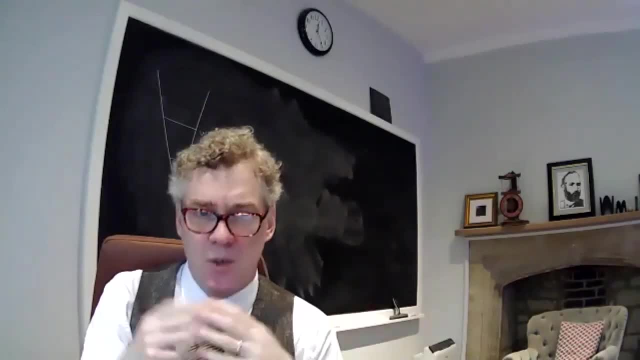 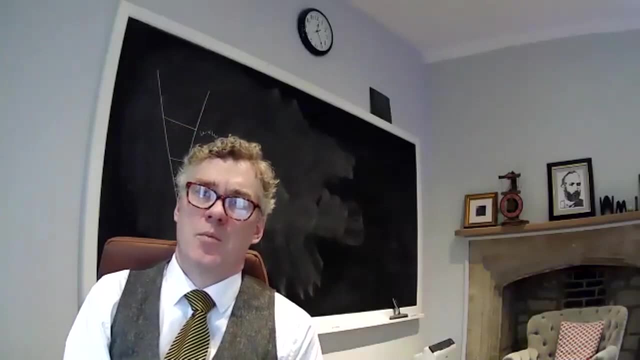 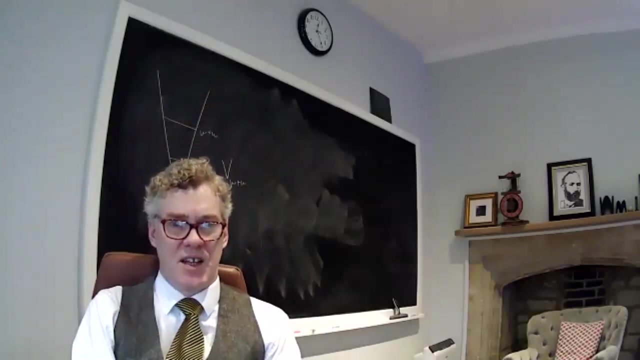 And so from this view, one wants to see the fundamental principles that will enrich our mathematical knowledge and providing those deep insights. At the moment the large cardinal axioms are the strongest known principles in mathematics that we have. So these axioms identify a rich structure theory for sets of real numbers, and that's a structure theory that's not really anticipated by any competing foundational. 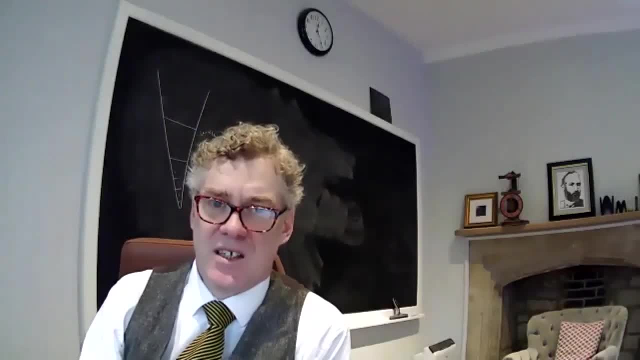 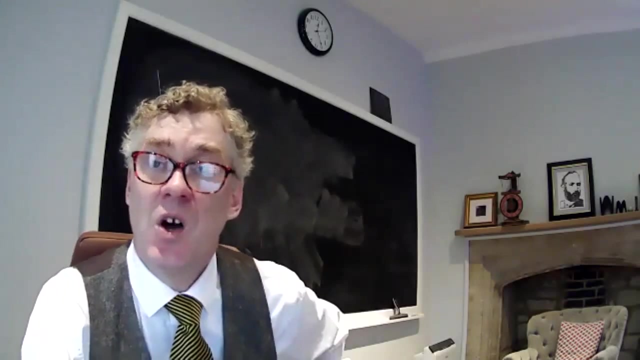 system. and ultimately, Steele argues that those consequences will be the reason that large cardinal, set theoretic foundations will endure, because any successful foundation of mathematics would ultimately have to incorporate the large cardinal hypotheses and their consequences In order to explain the mathematical phenomenons that flow from those axioms. 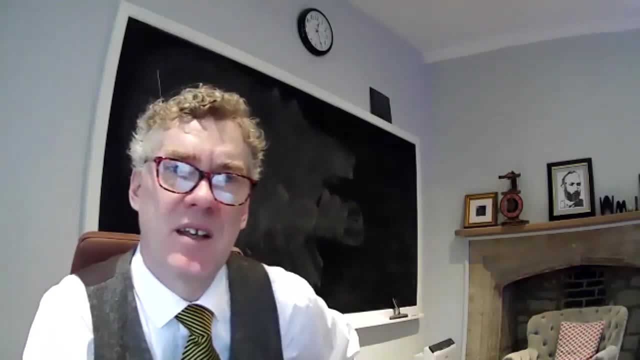 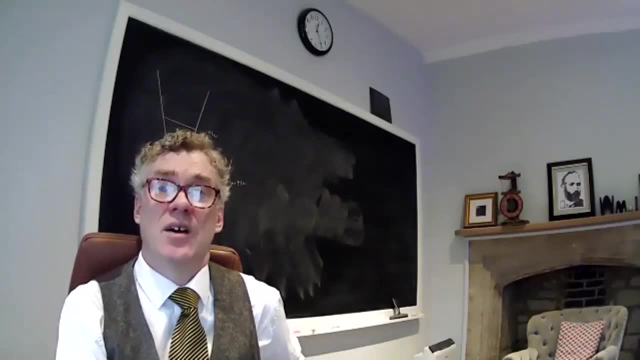 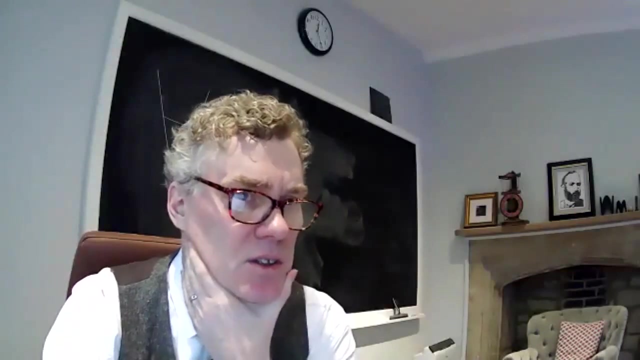 Okay. so I think, though, this issue about weak versus strong is something that hasn't really been explored sufficiently by philosophers, and I strongly encourage you all to engage with that issue. I think there's quite a bit of room there for philosophical discussion. So, Saharon Shelach. in contrast, 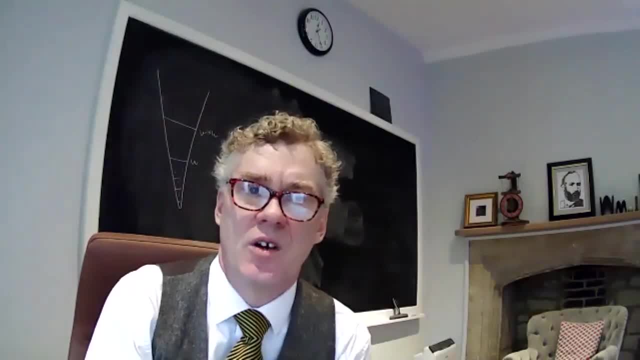 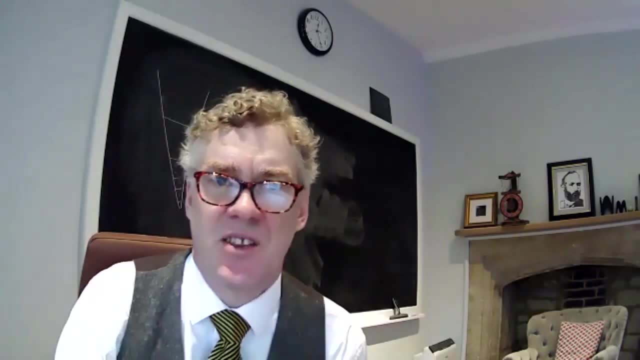 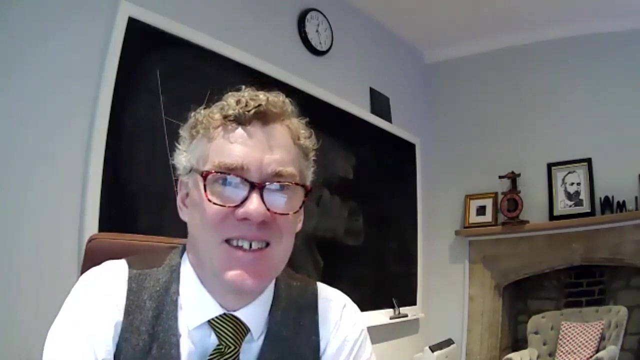 despairs at the idea that we're going to find compelling new fundamental principles. So he says, he writes. some believe that compelling additional axioms for set theory will settle problems of real interest will be found or even have been found. It's hard to argue with hope and problematic to consider arguments which have not yet been suggested. However, I do not agree with a pure platonic view. 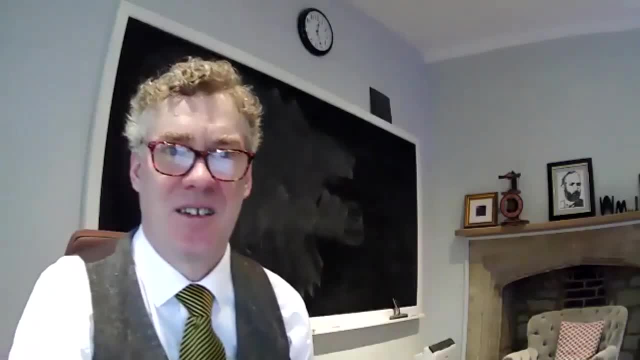 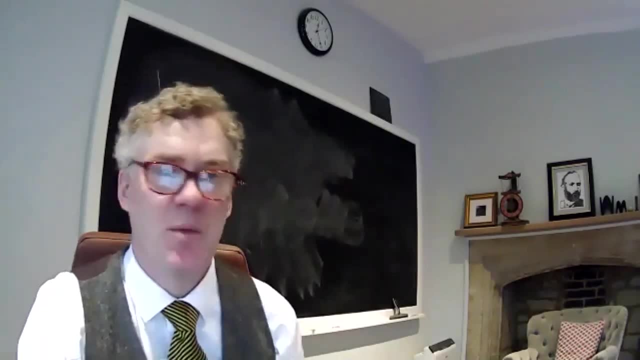 that the interesting problems in set theory can be decided, and we just have to discover the additional axiom. So he says: my feeling is that ZFC exhausts our intuition, except for things like consistency statements, And so for him a proof means a proof in ZFC. 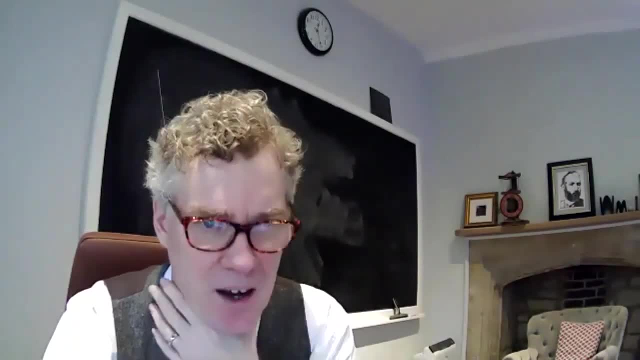 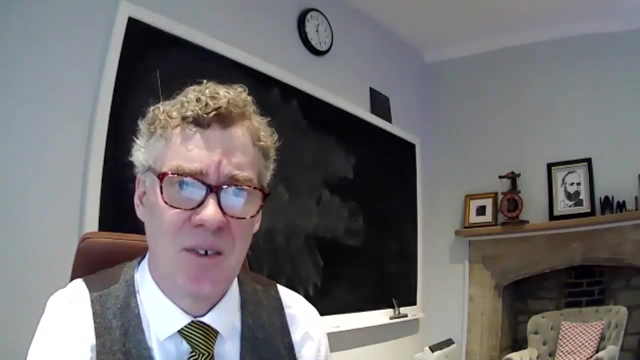 Pfefferman argues, on the other hand, that mathematics does not need new axioms. So he writes: I'm convinced that the continuum hypothesis is an inherently vague problem that no new axiom will settle in a convincingly definite way. Okay, let me now finally. I know I'm going way over. 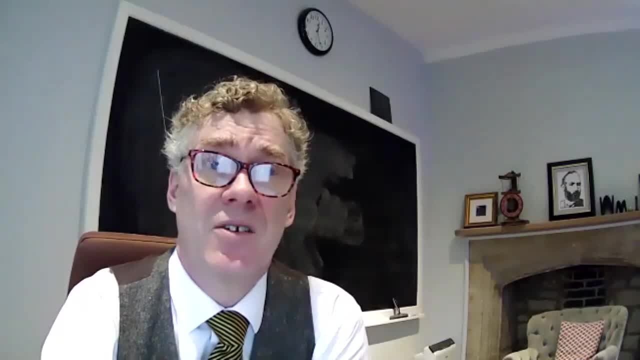 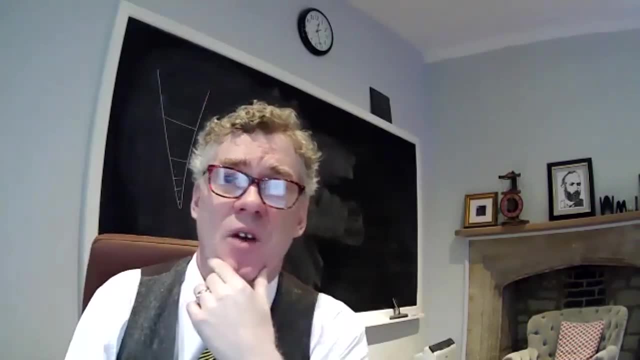 Let me finally come to the multiverse view. There's an ongoing vigorous debate in the philosophy of set theory. So, according to set theoretic pluralism, there's a huge variety of concepts of set, each giving rise to its own set theoretic world. 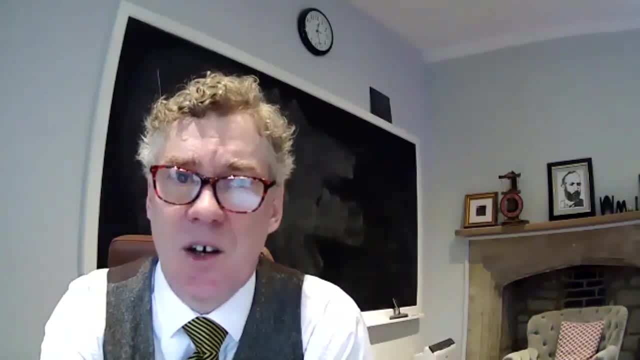 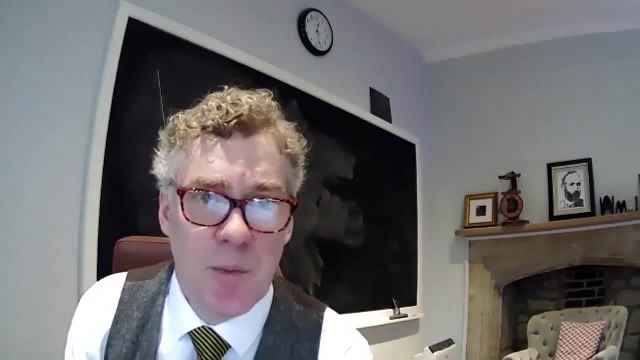 So I've described the situation by writing. As a result, the fundamental objects of set theory have become the models of set theory, and set theorists move with agility from one to another. Set theory appears to have discovered entire cosmos of set theoretic universes, revealing a category of theoretic nature for the subject. 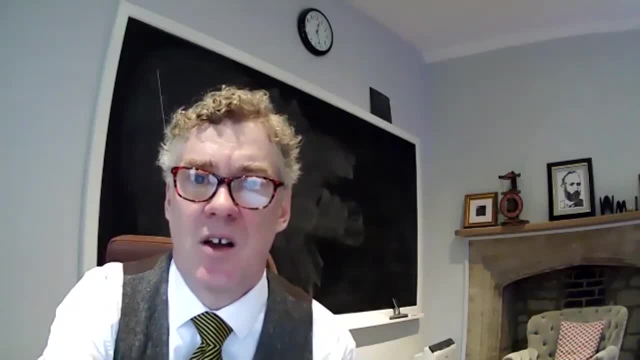 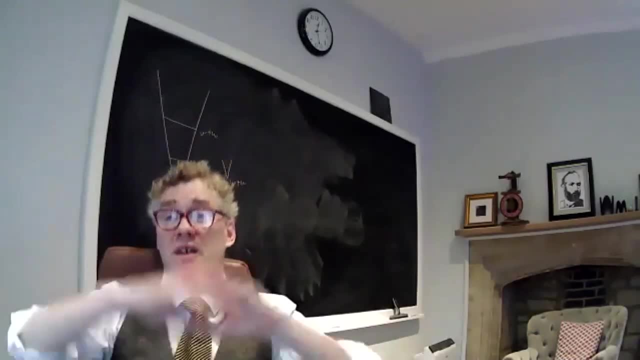 In which the universes are connected by the following: by the forcing relation or by large cardinal embeddings in complex commutative diagrams, Like constellations filling a dark night sky. So the point is that we have all these different concepts of set and we can construct different models of set theory from one another. 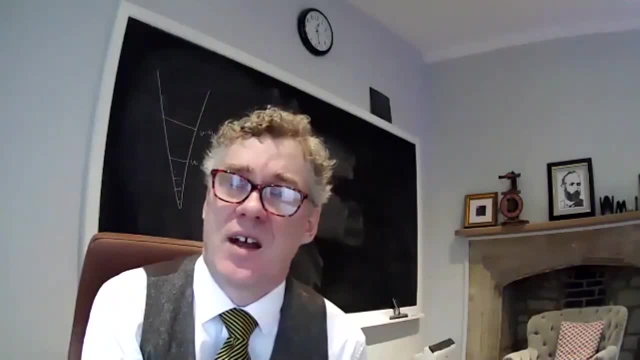 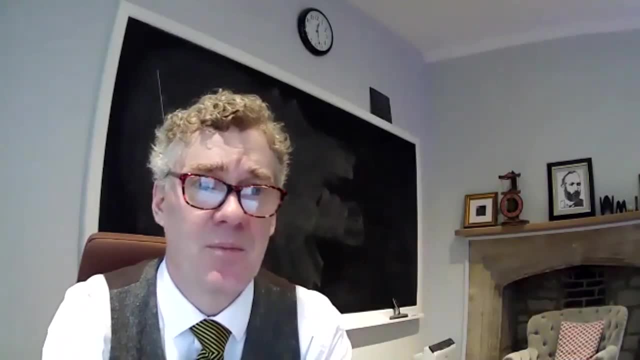 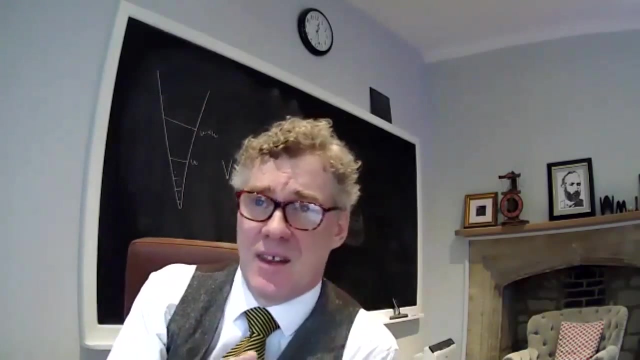 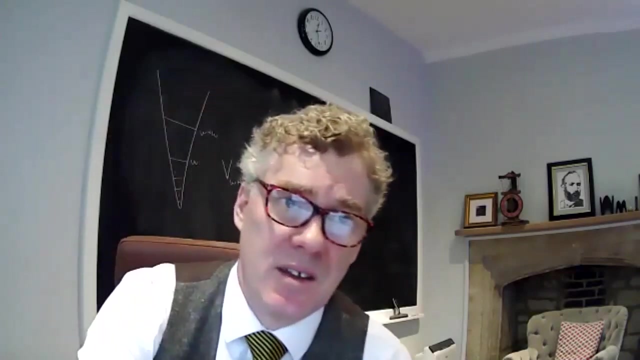 In order to realize specific set theoretic relations amongst those models, and it's really quite remarkable in many respects this is what set theory has become about, So one might hope for a kind of dream solution of the continuum about. this is: what we really want is a principle that would have an intrinsic support, sort of intrinsically justified principle that also settled the continuum hypothesis. 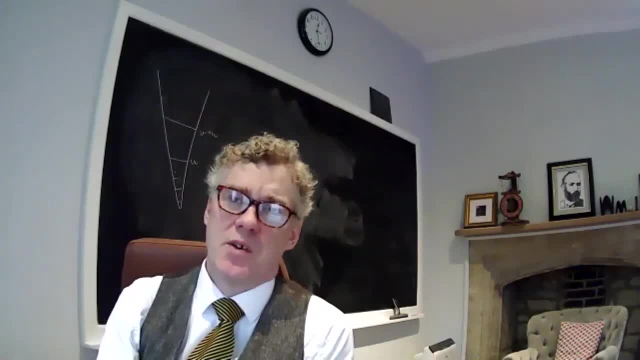 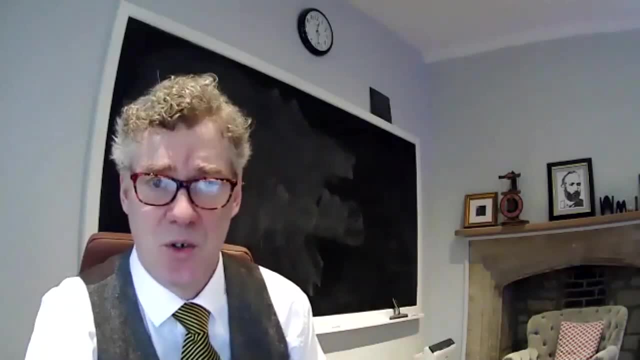 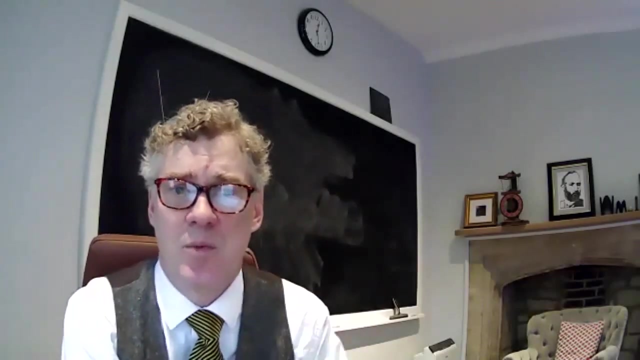 But I have argued that this is now impossible because of our experience with all of these other set theoretic worlds, in some of which the continuum hypothesis is true and in others of which it's not true, And so on. the multiverse view, the conditional hypothesis, is a settled question. It's incorrect to describe the CH as an open problem. 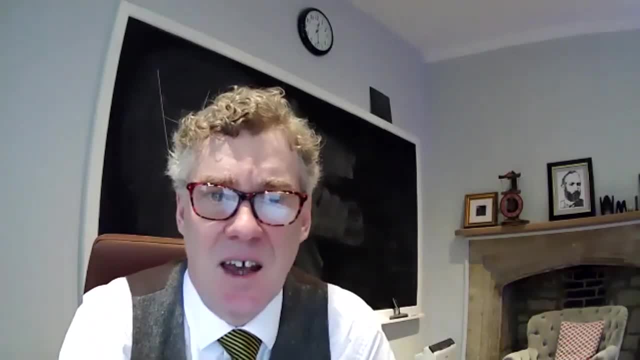 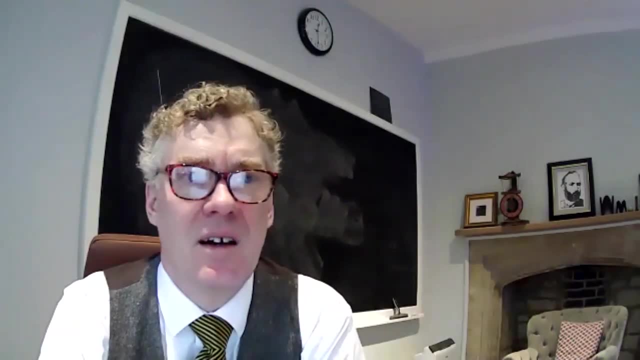 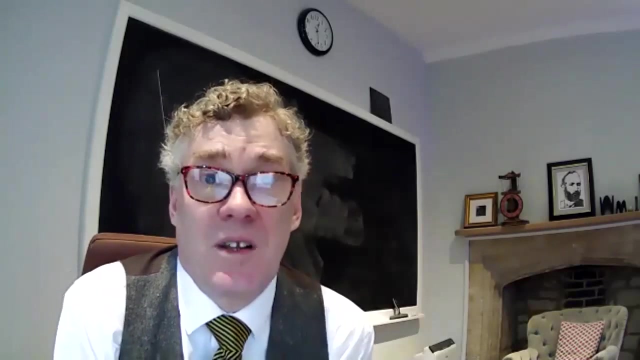 The answer to CH consists of the expansive detailed knowledge that set theorists have gained about the extent to which it holds and fails in the multiverse. Let me also mention the analogy between this multiverse perspective and geometry. This is really a very strong analogy between the pluralist nature of set theory and the established 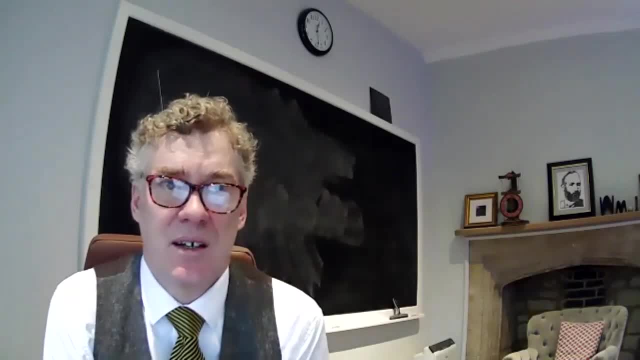 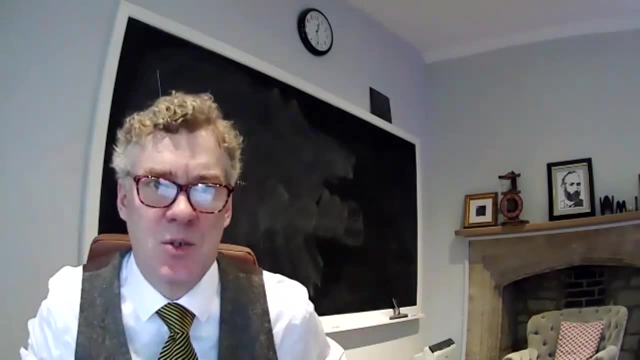 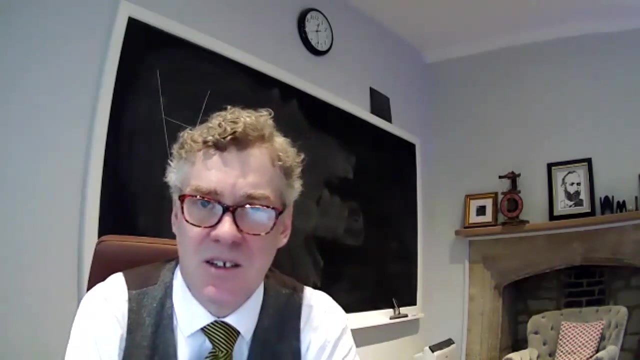 plurality in the foundations of geometry. So for thousands of years, of course, mathematicians studied geometry and thought of geometry as the study of the one true geometry. It had a singularist nature until the discovery of non-Euclidean geometry, and then the singular concepts splintered into distinct, separate concepts of geometry and mathematicians realized: hey, 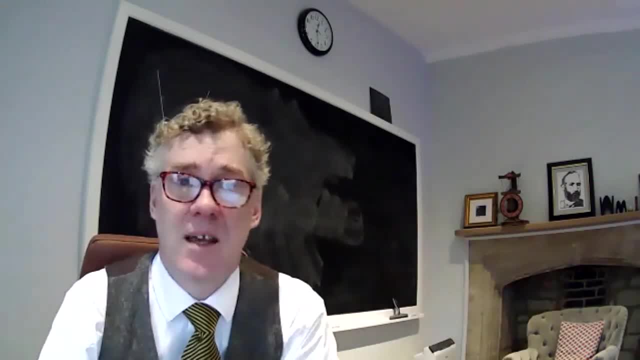 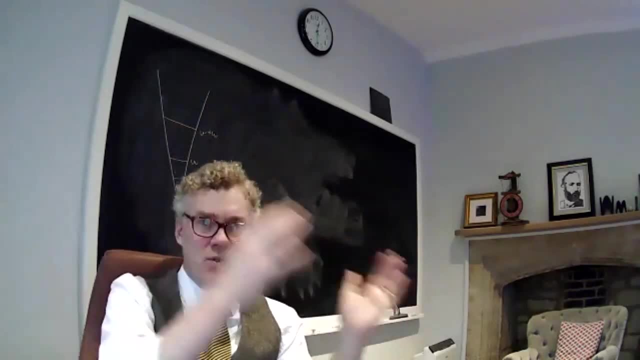 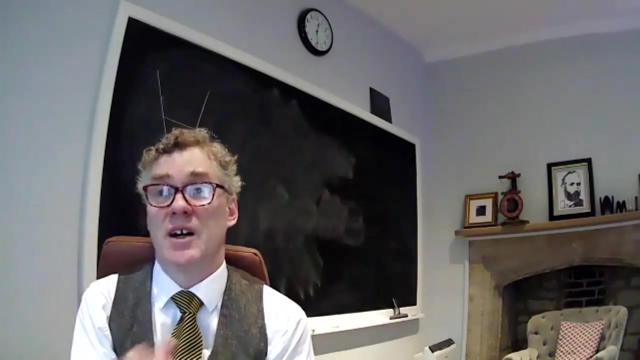 the subject is really about these different, incompatible concepts of geometry, And it was no longer sensible to ask questions Whether the parallel partiality is true, but rather whether it's true in this geometry or in that one. And similarly, in set theory. it's not sensible to ask whether the continuum hypothesis is true or not. You ask: is it true in this set theory or in that one? 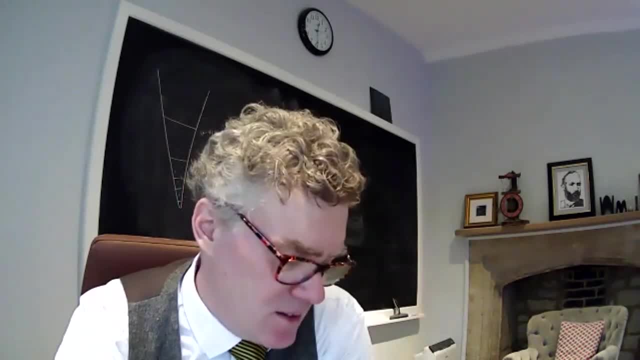 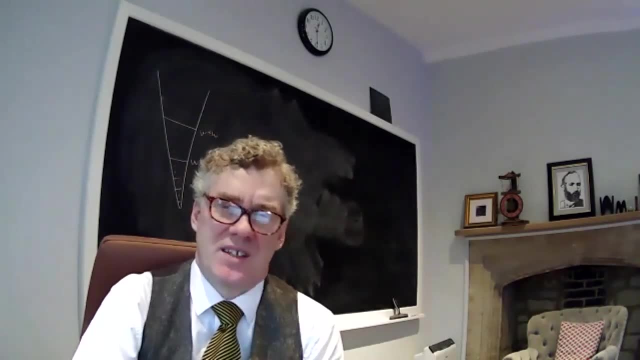 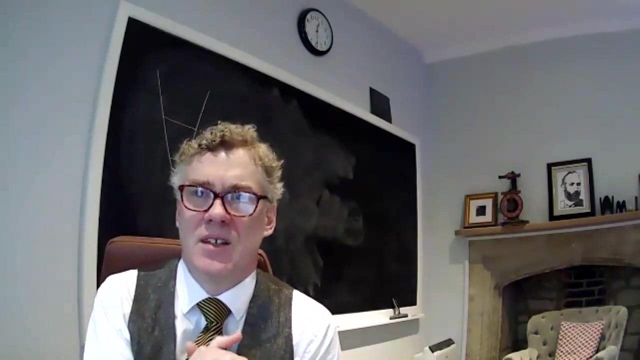 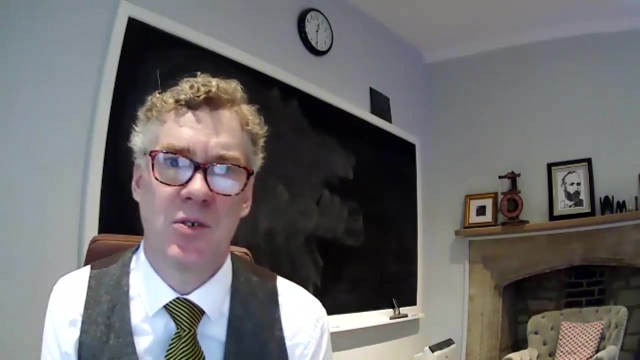 So that the term Platonism used to carry decades ago. So I remember when someone would describe themselves as Platonist, they were also intending to express that they believed in the singularist view, in the universe view that there's a unique, final, platonic universe in which set theoretic statements would achieve their absolute truth value. 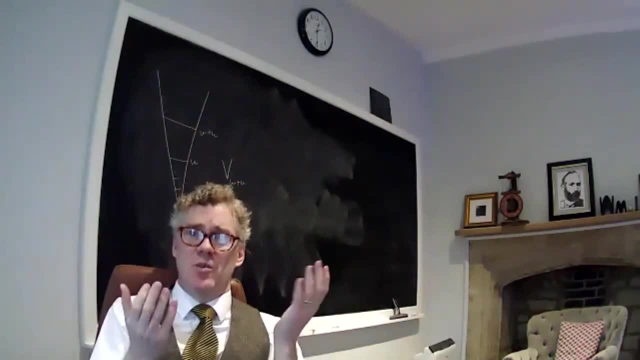 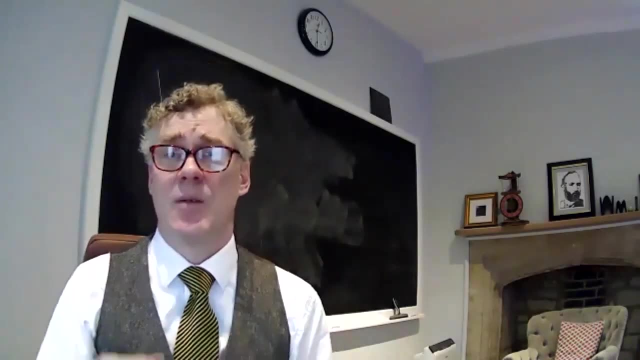 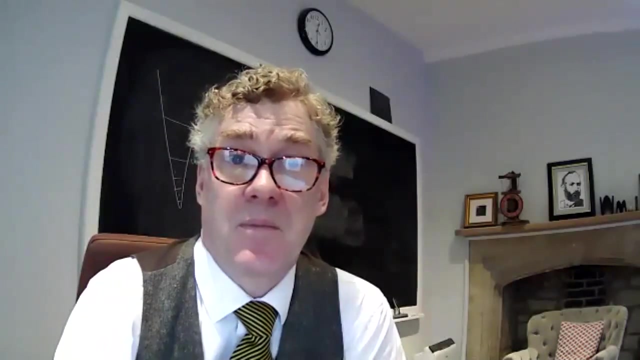 But today that usage has relaxed somewhat and one should view: Platonism is really about mathematical realism. It's about the real existence of the mathematical objects rather than about the uniqueness of the set theoretic realm in which those objects exist. And in an extreme form there's the concept of plenitudinous Platonism. Mark Ballagher's view. 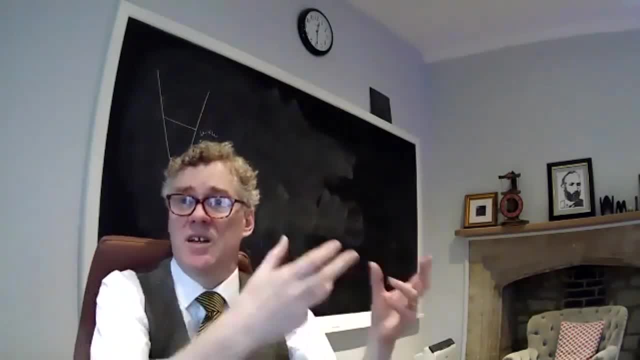 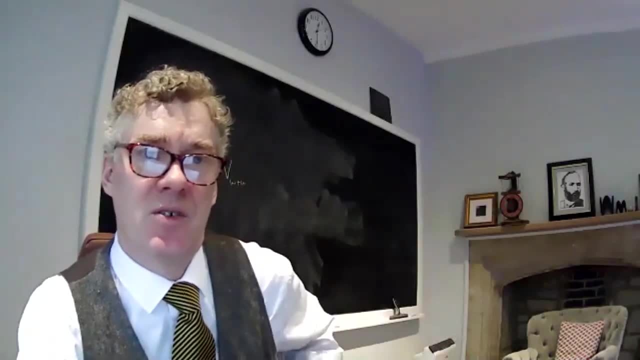 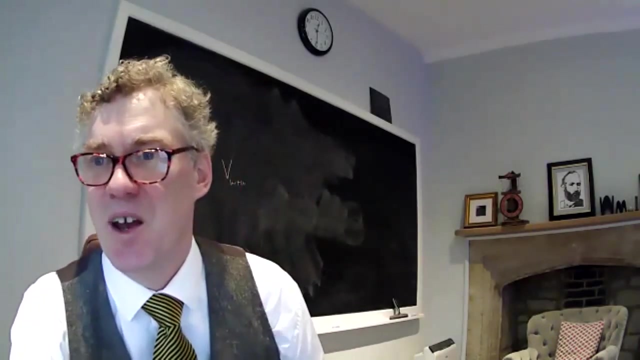 Plenitudinous Platonism is asserting. it's a kind of Platonism because it's about the real or genuine existence of the mathematical objects, but there's many different models or realms of those structures. Okay, I guess that's it. That's all I had to say. I'm sorry, I went way over and I'm sorry for the technical difficulties at the beginning. 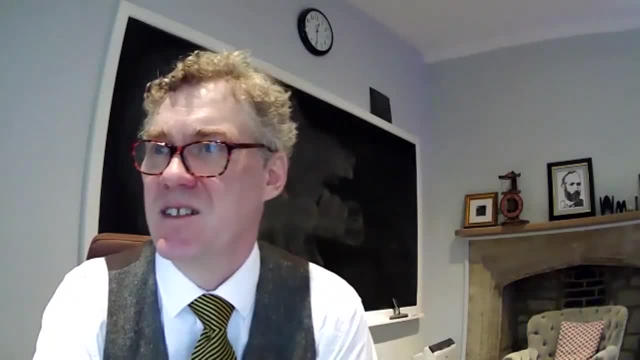 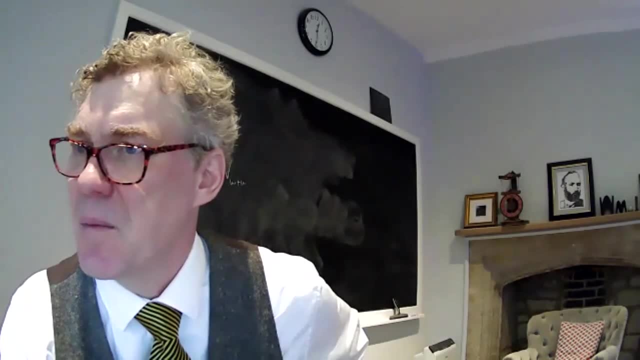 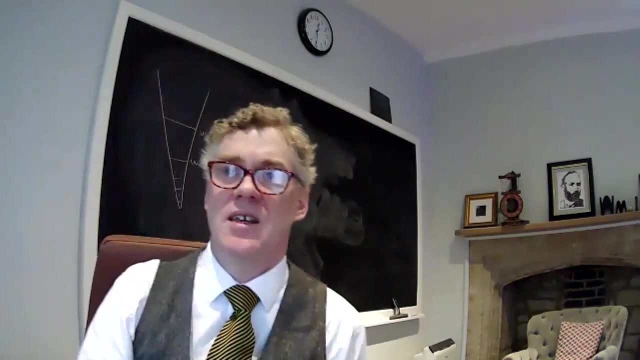 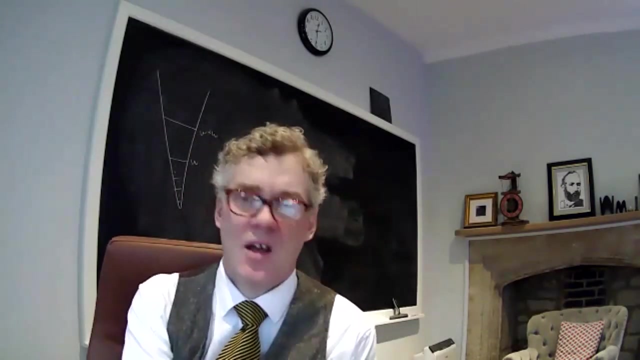 But we can open it up for discussion and questions. now, Let's see, I see some in the chat, So why don't I address those? Someone says, oh, okay, let's see. Someone says: what does it mean to talk about models of ZFC? Well, the ZFC is the Zermelo-Fraenkel set theory with the axiom of choice is a first order theory. We can write down the axioms exactly, just similar to the way that we write down the axioms of, say, piano arithmetic. 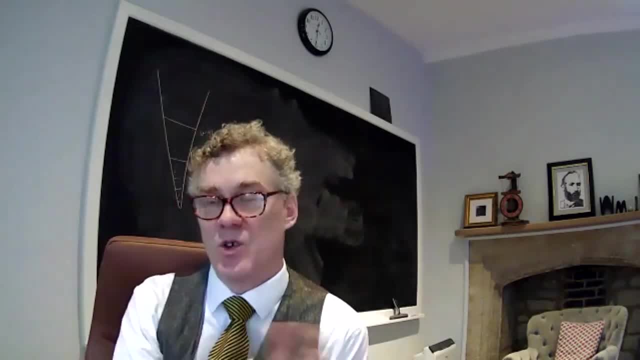 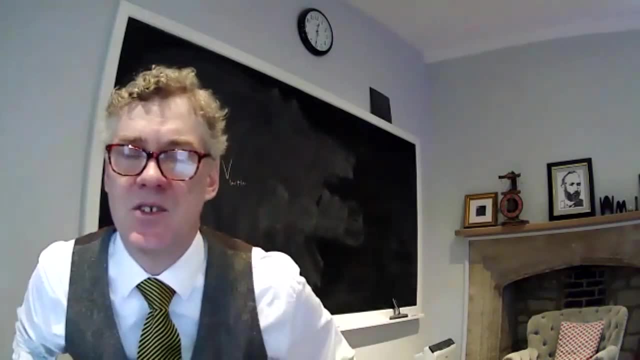 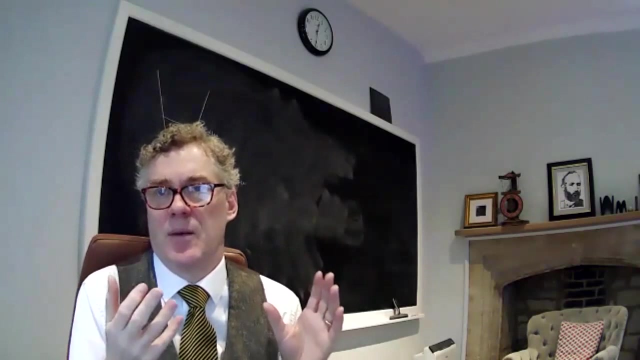 or the axioms of group theory or field theory or whatever, And so it's a first order theory. And so we have a concept of a model of ZFC. The language is just the epsilon relation. So ultimately a model of ZFC is a set, a domain, with an interpretation of the set membership relation on that domain that such that that membership relation obeys the axiom, So it should satisfy extensionality and union and pairing and so on. 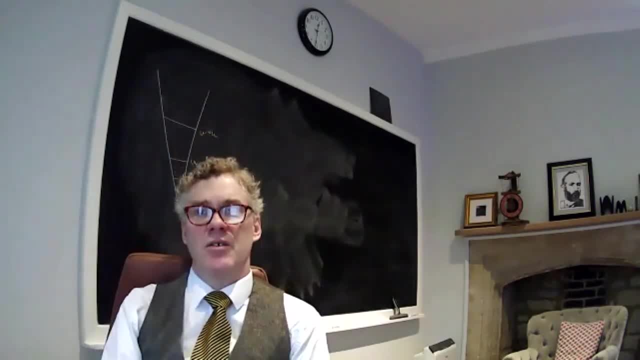 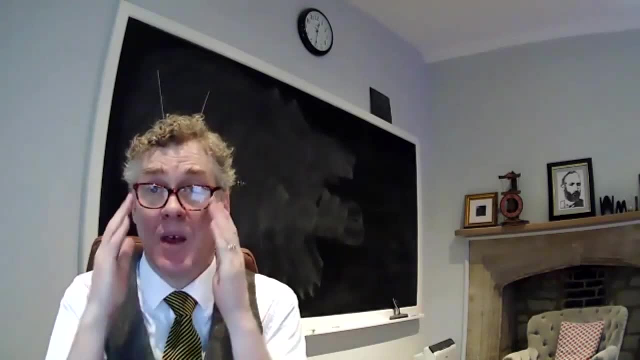 So when we say a model of ZFC we just mean a model of that theory and we can analyze it, model theoretically and apply Levenhans-Scholem theorem And so on and do model theoretic constructions with those models. But on the other hand it's sort of 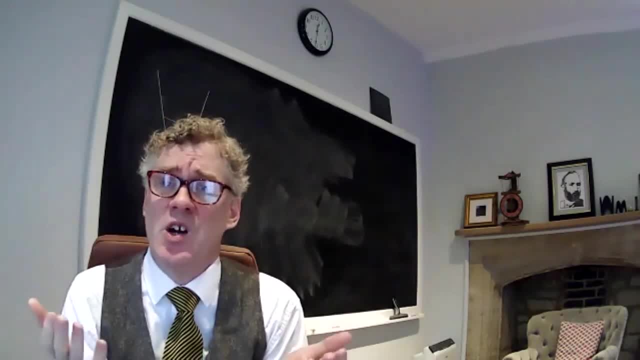 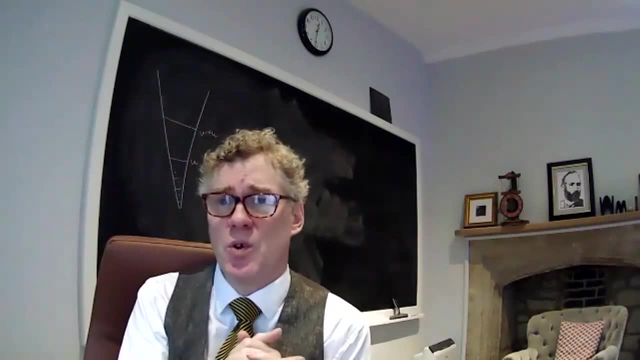 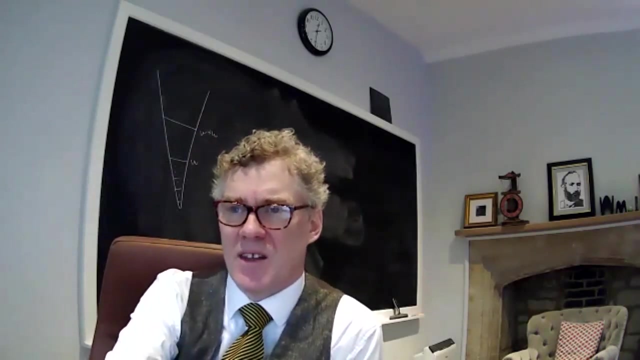 a model of ZFC is also a set theoretic realm And we can imagine jumping inside that model and living a kind of mathematical life inside that model, because ZFC proves that the real numbers exist and the complex numbers and the topological spaces and so on, All the kind of mathematical, classical mathematical ideas that you might have are generally provable in ZFC. 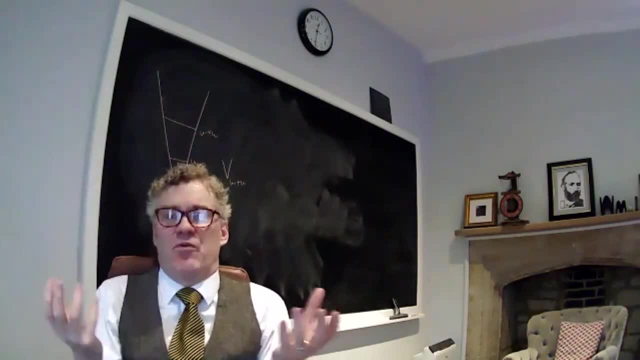 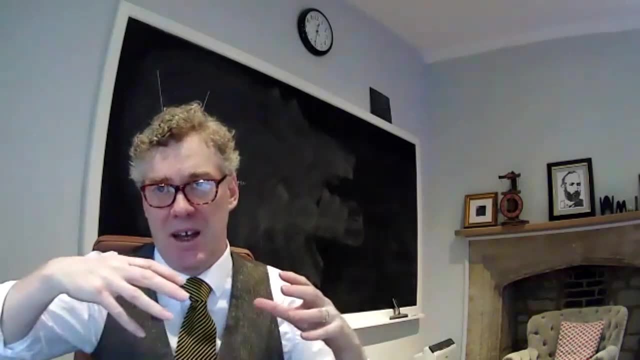 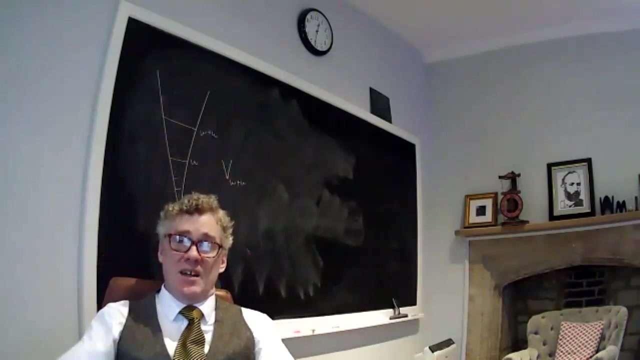 And so we can imagine living inside that model and having a full and rich mathematical life. And so that's what makes it sort of philosophically robust and satisfying is that we can from above look at those models of ZFC and apply model theoretic methods to construct different one, And at the same time we can imagine living inside them and living a kind of mathematical life inside there. 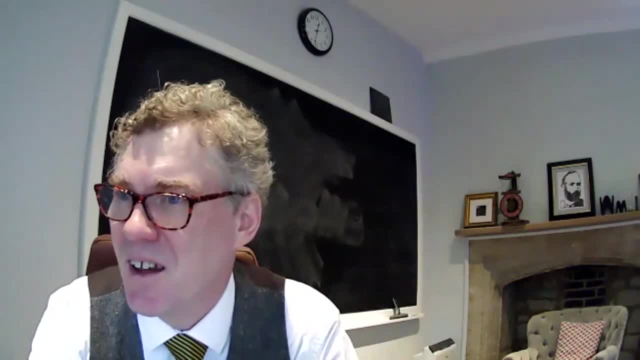 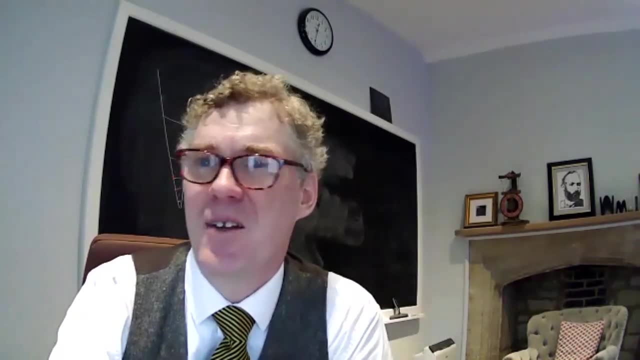 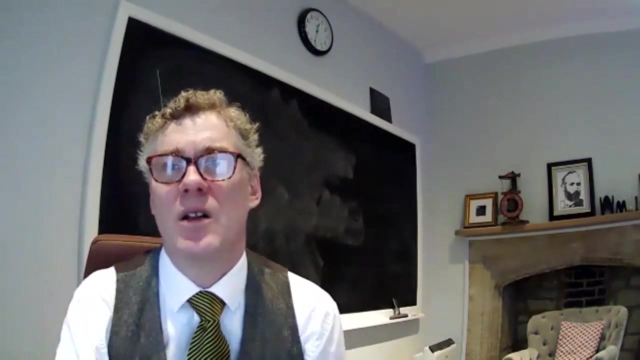 I'm not sure if that answers your question or not. Okay, Are there any other questions? I'm sorry I went way over on time, I apologize. Please go ahead and unmute yourself if you have any comments. Can we imagine mathematics without set theory? Well, 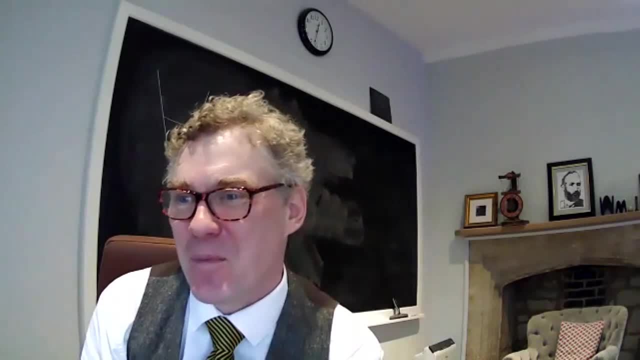 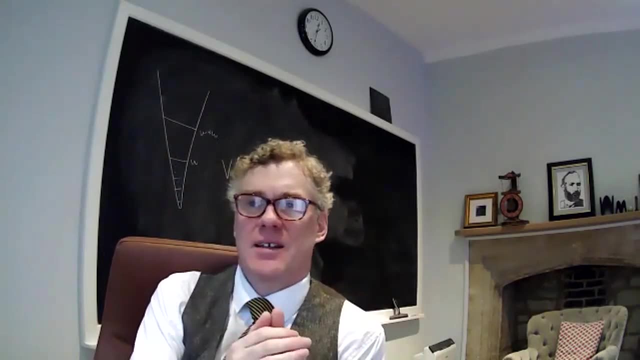 I can't. No, I don't know. Of course, sometimes, when one is considering set theory as a foundation of mathematics, then it's important to recognize that of course it's not the only foundation and there are other foundations. the category theoretic foundation. 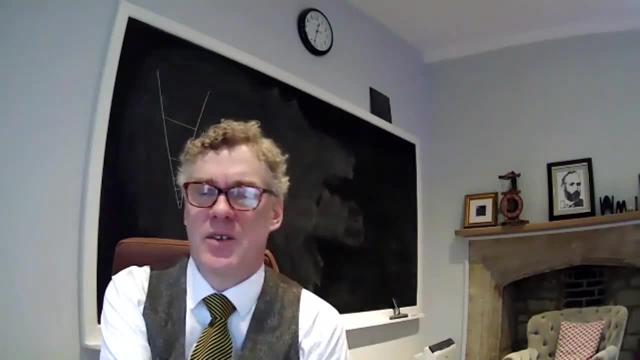 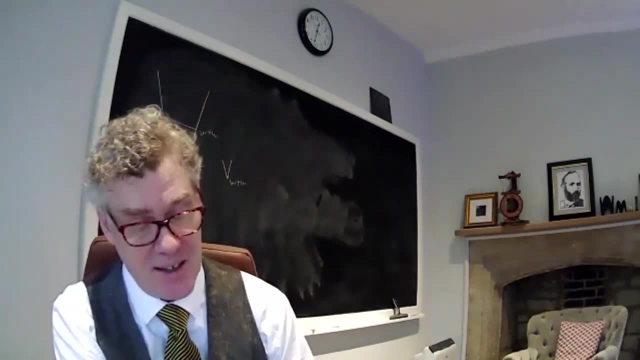 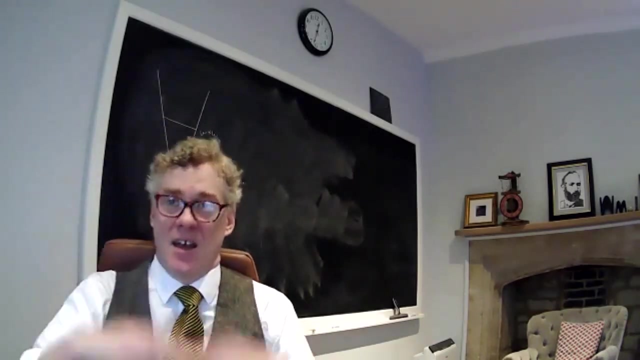 or say type theoretic foundations and so on, And everyone agrees that there are these alternative foundations of mathematics, But that doesn't mean that those alternative foundations, that somehow you don't have set theory anymore, because set theory is also, as I mentioned at the beginning, a mathematical subject. It's a mathematical subject and it's also serving the role as foundation. There's these two roles. 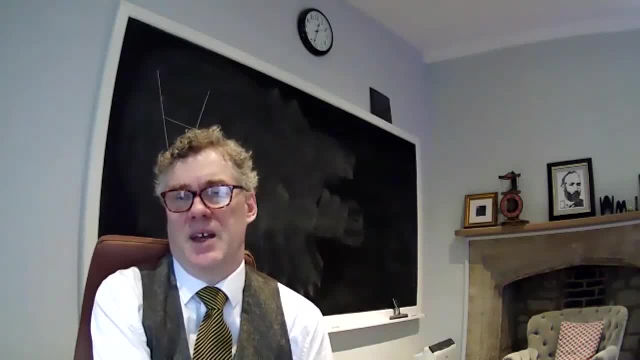 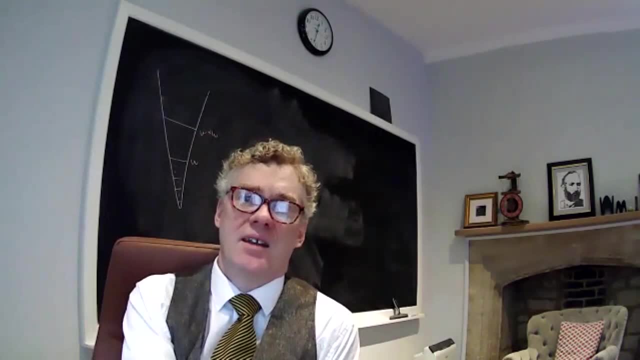 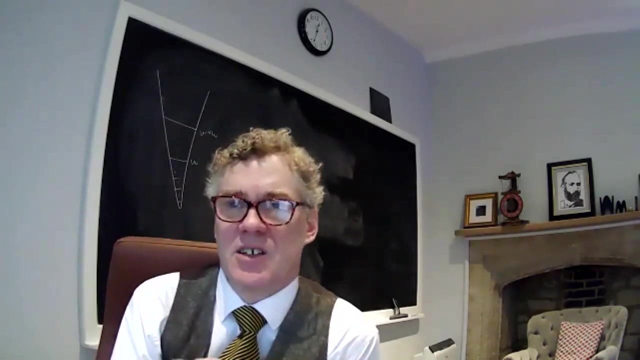 So if you have a different foundation of mathematics, then it should be able to talk about set theory also, Because set theory is a mathematical subject And so any mathematical structural idea that's laying a claim to being a foundation of mathematics should also be able to be a foundation for set theory. 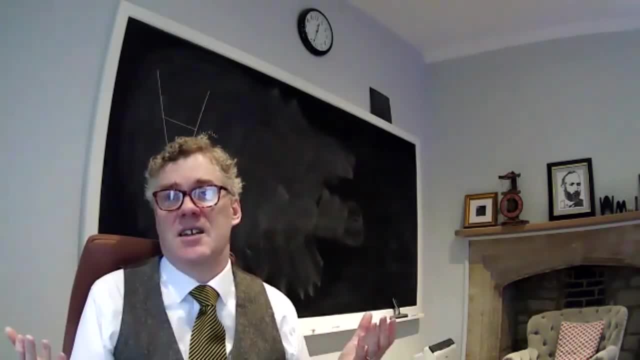 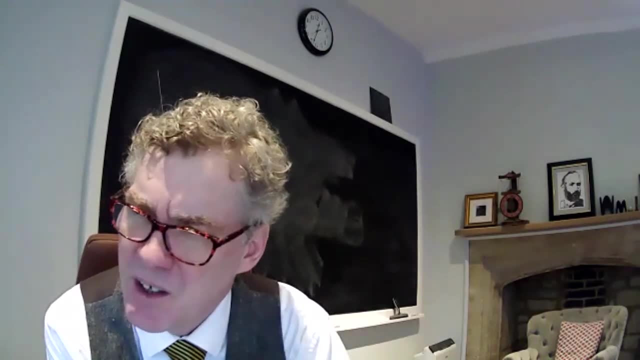 because that's part of mathematics. I mean just in the sense that it's also going to be a foundation for algebra and topology and so on, all the other parts of mathematics. So I'm not sure what you mean by imagining mathematics without set theory. 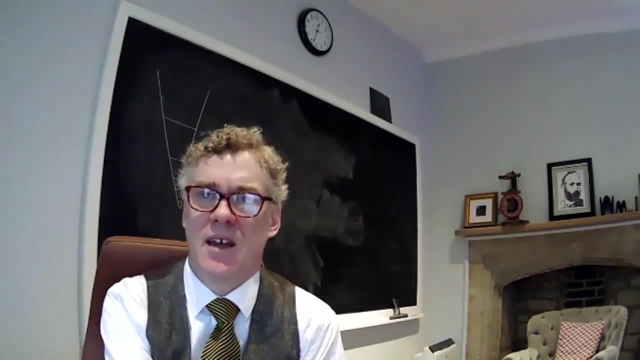 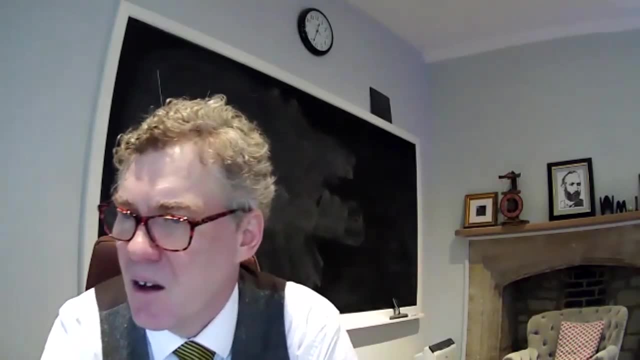 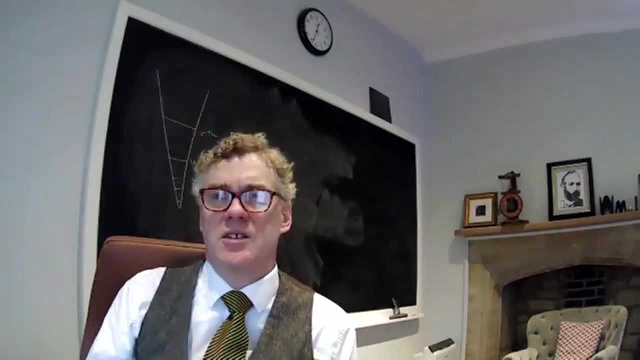 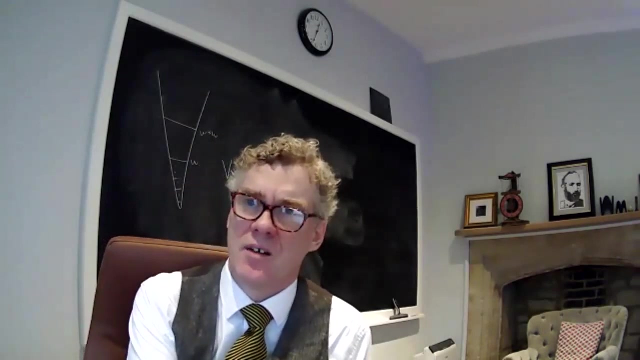 I mean, of course there are other kinds of mathematics that don't explicitly engage with set theory. So I can imagine those parts of mathematics and there's no set theory in those subjects. Okay, what is my intuition of mathematics without a C? Okay, so without the axiom of choice, Right? So there's a very rich subject developed studying the nature of set theory without the axiom of choice. There's many, many papers written and conferences and so on about set theory without the axiom of choice and the nature of it. Usually one doesn't want to give up the axiom of choice completely. You want to retain sort of fragments of it, like maybe you want countable choice, which means the axiom of choice for countable families. So if you have countably many non-empty sets, then you should be able to pick an element from each one of those sets That's countable choice. 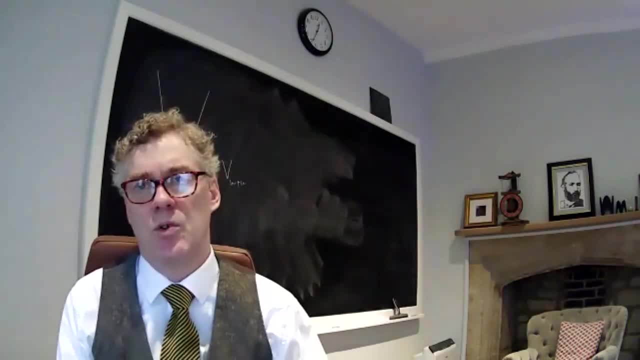 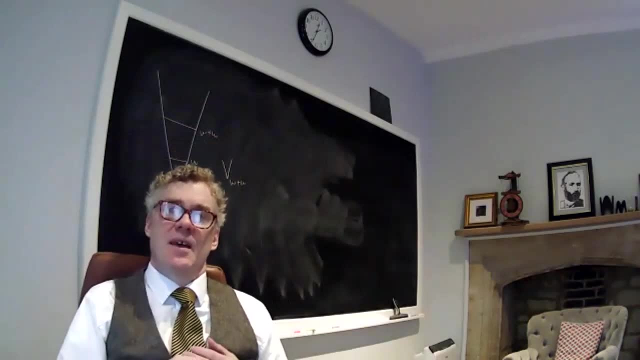 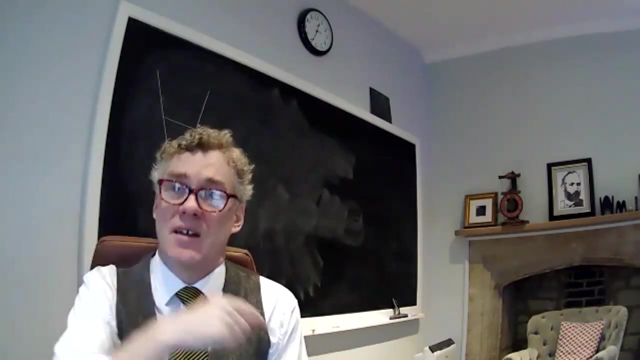 But actually many arguments that seem to involve countable choice actually involve a slightly stronger principle called dependent choice, which is the principle that says you can make countably many choices in succession, where the later choices depend on the earlier ones that you made. So, for example, if you have a tree, say, 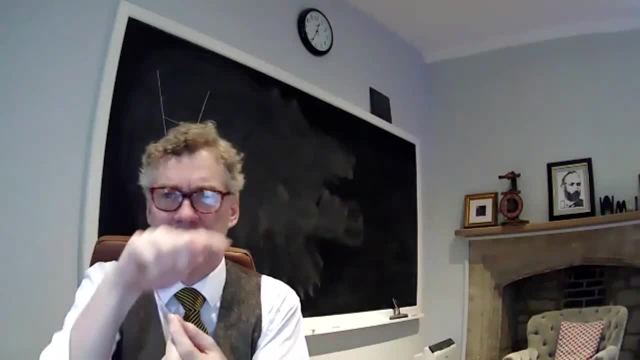 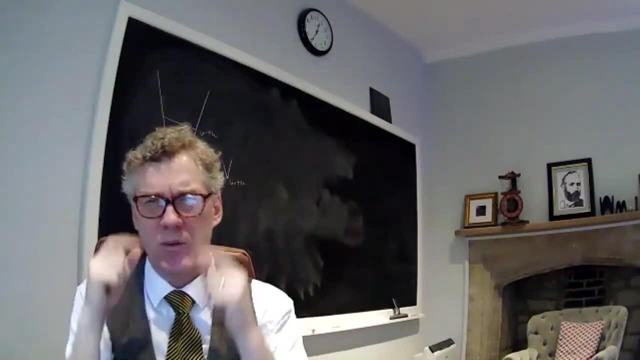 and it doesn't have any leaves. okay, it has a root node and there's some successors and those have successors and so on, but there's no terminal nodes. then well, if there's no terminal nodes, you might want to say, well then you can find a branch. 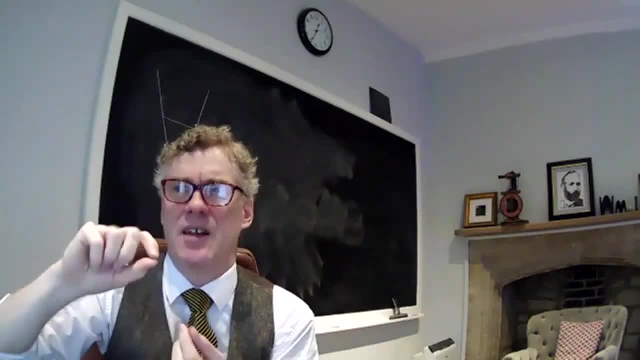 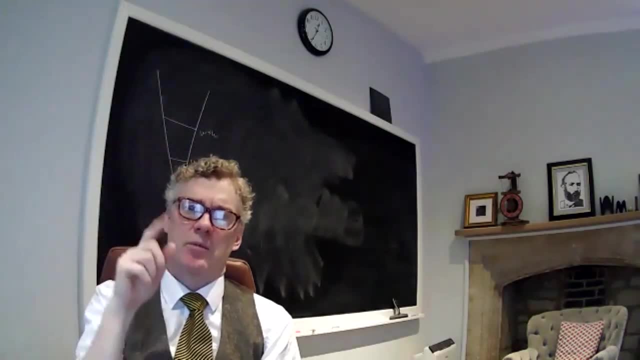 An infinite branch. right, You can just pick any successor and then from that one pick any successor and from that one pick any successor, and so on. But that's not an instance of countable choice, even though it seems like we made countably many choices, because the whole tree won't be countable maybe. 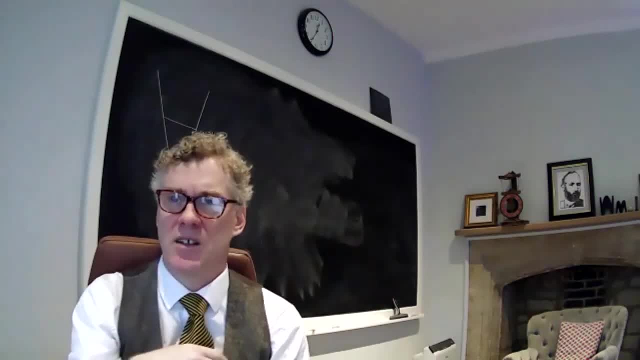 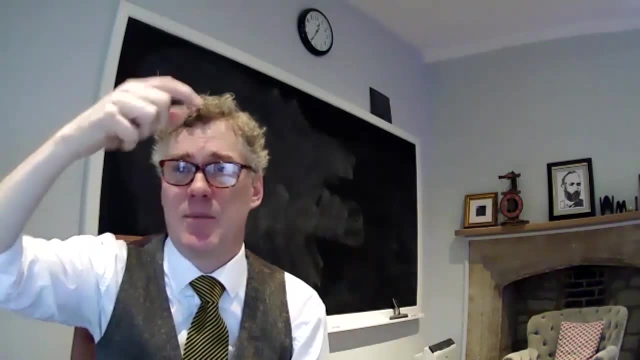 So we don't have a countable enumeration of the nodes. If we did, we could always just pick the least one in the enumeration, But I'm making countably many choices in succession, and which choices are to be made at the next step depends on how I made my choices to get to that node. 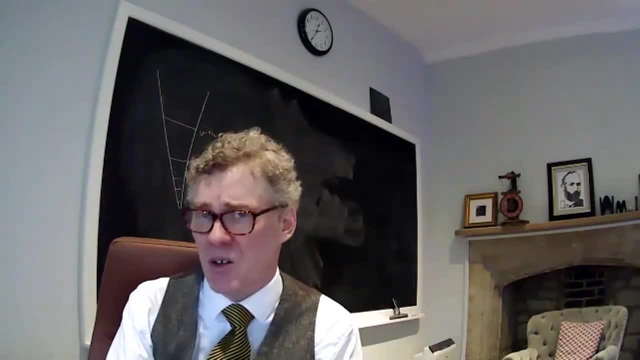 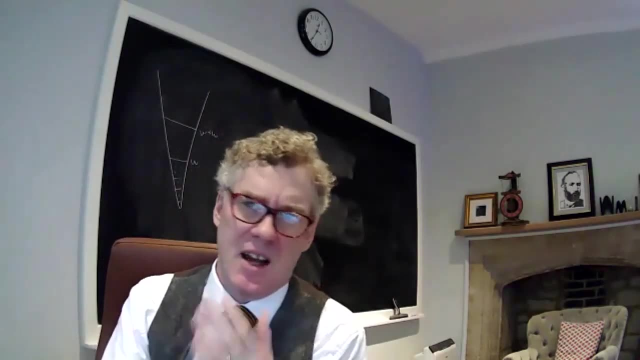 This is called the principle of dependent choice and it's strictly stronger than countable choice, And this is the principle that you really want when you're doing measure theory. If you don't have dependent choices, then you're not going to have a good theory of Lebesgue measure. 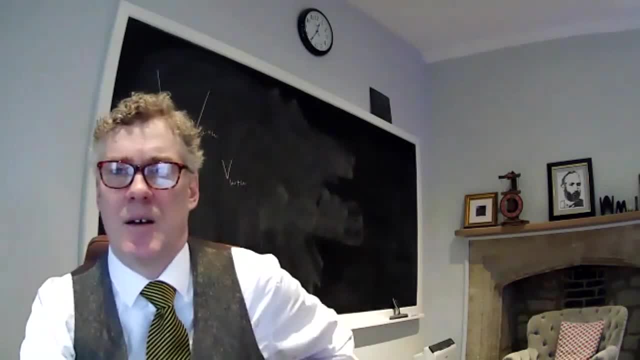 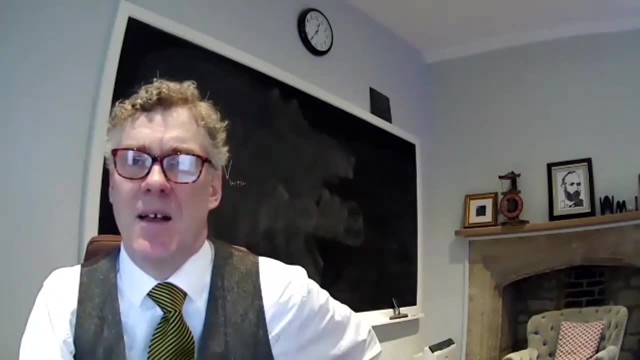 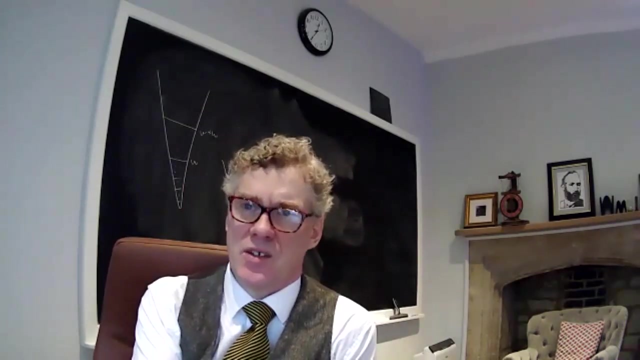 It's strictly weaker than full choice, but it's still not provable without any choice principle at all. Okay, my intuition about mathematics without AC is that I think mathematicians are routinely instinctively assuming that using something like the axiom of choice all over the place, maybe even without realizing it. that's the danger: particularly countable choice, or even DC. 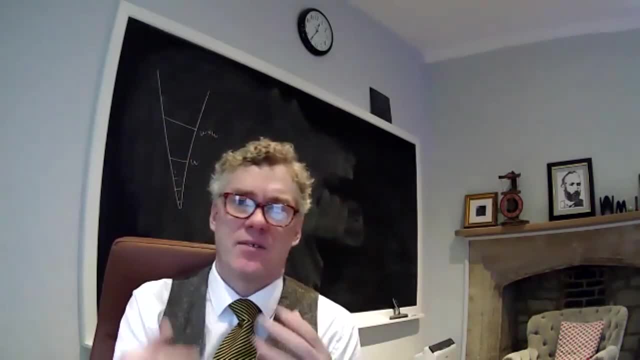 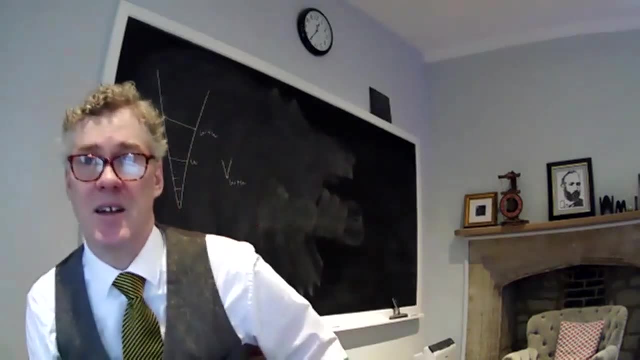 And so to give it up completely, I think is a very dangerous thing, because we'd have to really pay attention to when we were maybe accidentally using the axiom of choice in our way of understanding a certain mathematical idea. I mean, just like the idea of if you have a tree with no terminal nodes, then it has a branch. 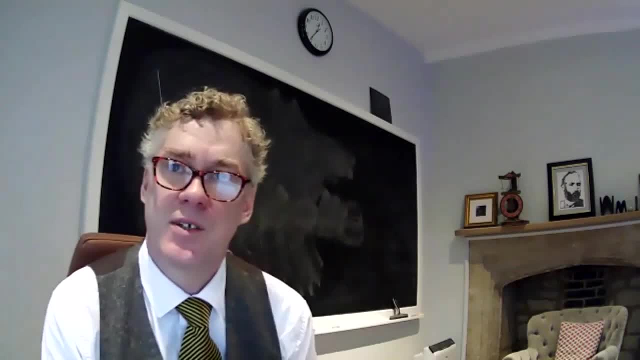 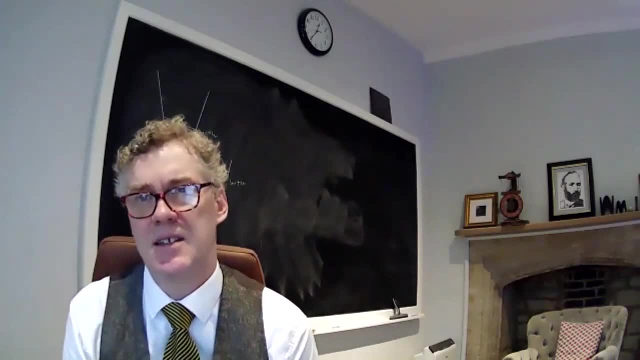 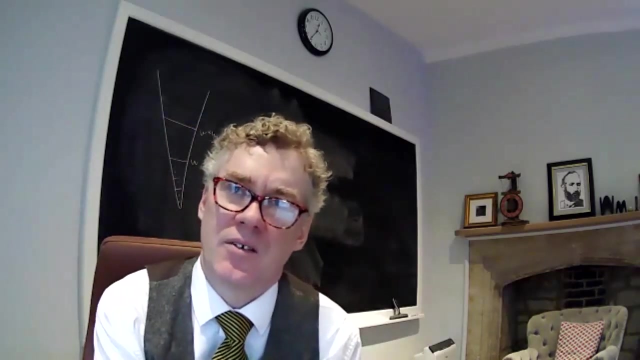 which you can't prove without if you drop the axiom of choice completely. And I think this is maybe part of the explanation about why the analysts didn't adopt Solovey's theory, because they weren't really willing to give up that intuition that we have about the truth of the axiom of choice, and they would rather. 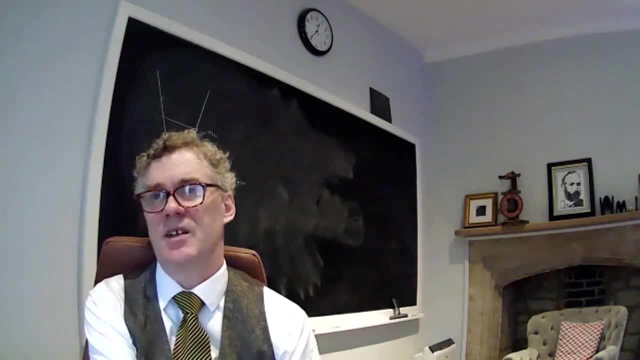 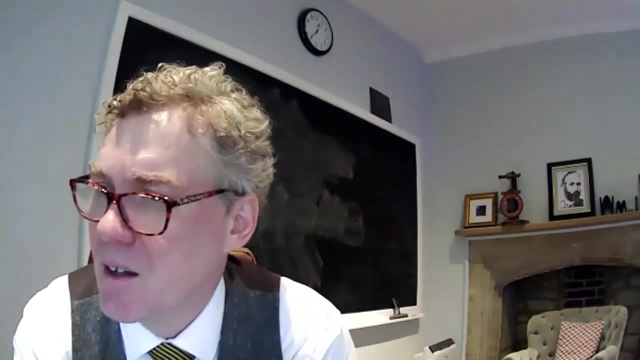 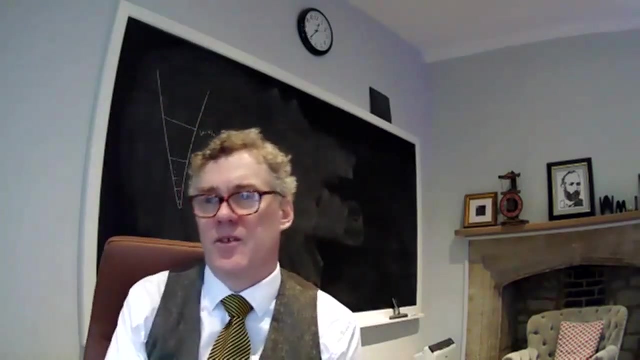 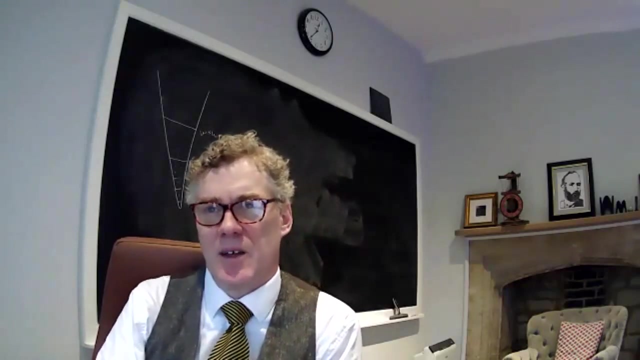 pay attention to whether sets were measurable and have sigma algebras and stuff, instead of worrying about whether or not they were mistakenly using the axiom of choice. Okay, let's see. Do constructual mathematics need set theory? Well, so there are, I mean. well, I don't know if they need it, but one can undertake set theory or essentially any mathematical enterprise in constructivism. 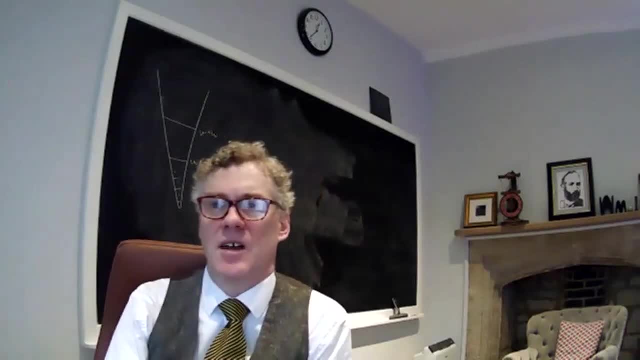 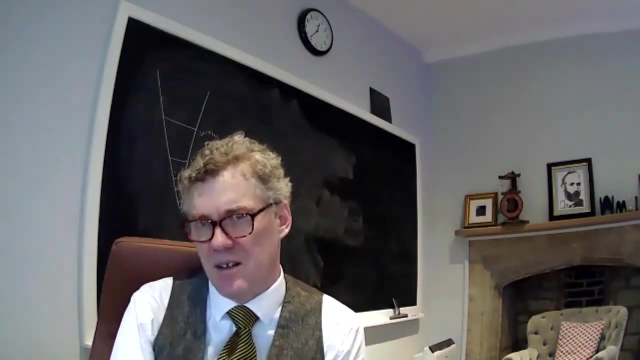 So if you're a constructivist or you want to use only intuitionistic logic, then you can have a kind of set theory. There's an axiomatization called intuitionistic ZF, So IZF. In intuitionistic logic only you can develop set theory. 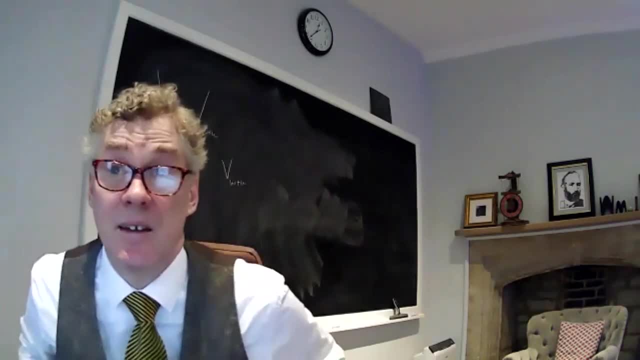 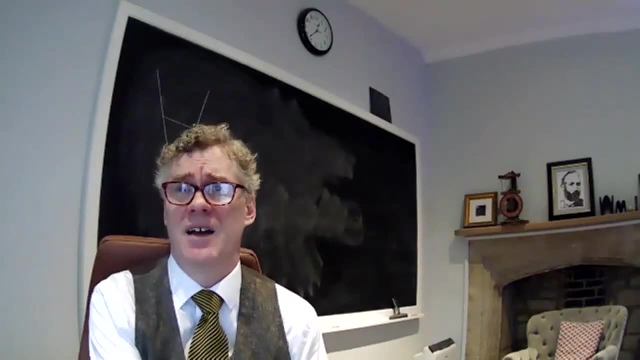 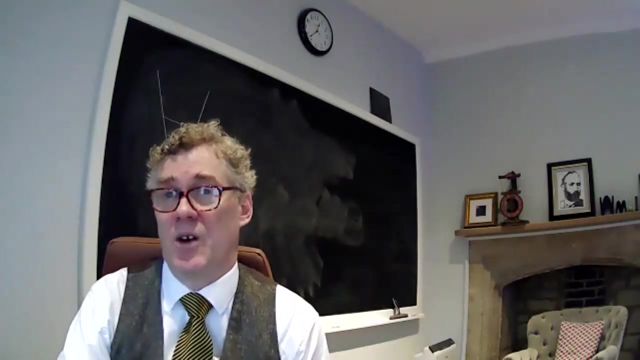 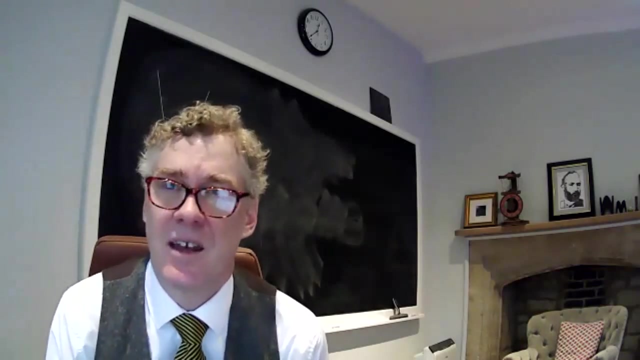 And so there's nothing incompatible about set theory and an intuitionistic logic. However, the axiom of choice in intuitionistic logic, the axiom of choice implies the law of excluded middle, And so you would then recover classical logic if you also give yourself the axiom of choice. So, generally, if you're doing constructive logic, set theory, then you won't have the axiom of choice, because if you did, then it would turn out to be equivalent. 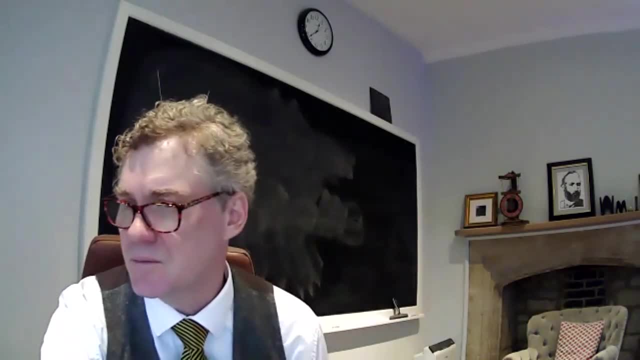 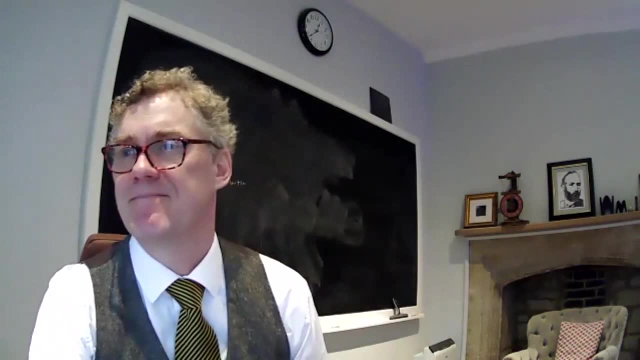 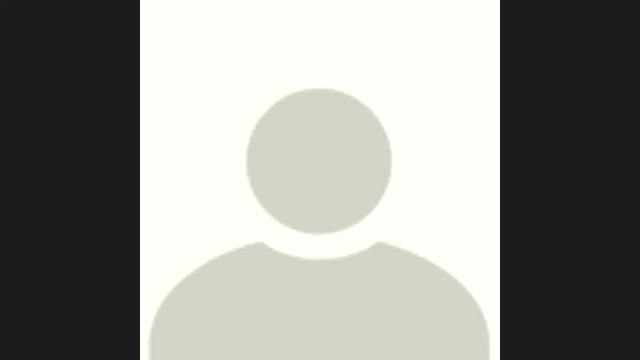 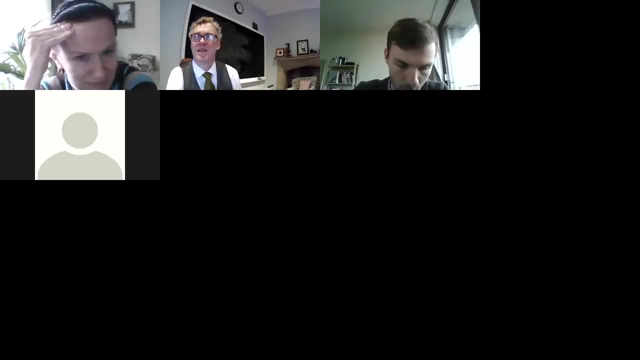 to the classical logic. Okay, any other questions? Joel, can I ask you a question? Sure, go ahead. Robin, I was wondering about when you were talking about the large cardinal hierarchy you were saying it's kind of a natural consequence of the idea of incompleteness and there is this hierarchy of consistency statements. 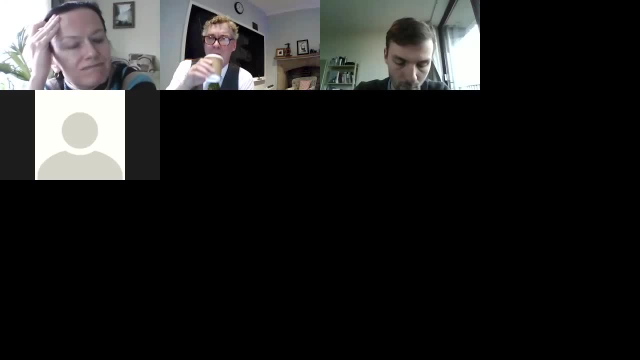 Yes, But I was wondering- I guess I haven't thought about this before- why isn't there something corresponding to the large cardinal hierarchy for, say, PA? Why isn't there a hierarchy of natural statements of higher consistency strength? What is the difference between PA instead of C with respect to this hierarchy? 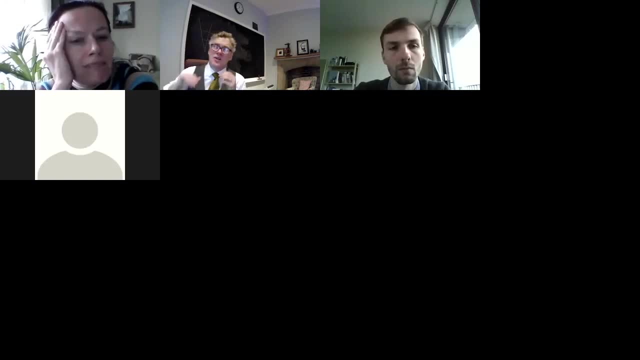 So that's an extremely good question. I really like that question a lot. So on the one hand, we can translate the There's a kind of arithmetic residue of the large cardinal hierarchy that comes just from the consistency assertions. right, The large cardinal hierarchy is asserting actual existence of these enormous infinities. 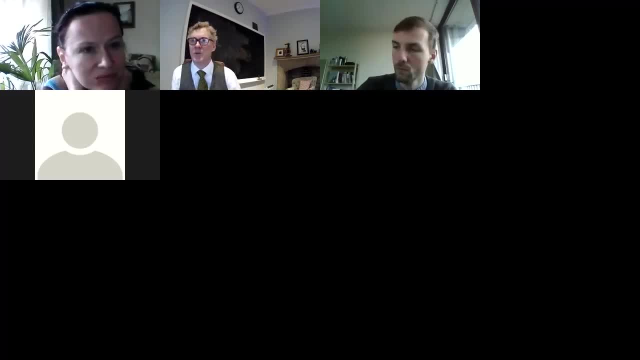 So of course we can't express those ideas directly in arithmetic, because the infinities aren't in the realm of piano arithmetic. But the consistency assertions are, because a consistency assertion about a theory is an arithmetic assertion, right To say that a certain theory is consistent. 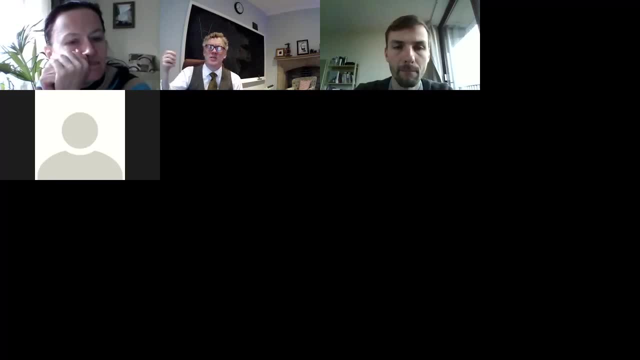 To say that a certain theory is consistent is to say there's no number coding of proof of a contradiction from that theory. That's an arithmetic assertion. And so we have this large cardinal hierarchy, you know inaccessible and measurable and super compact, and so on. 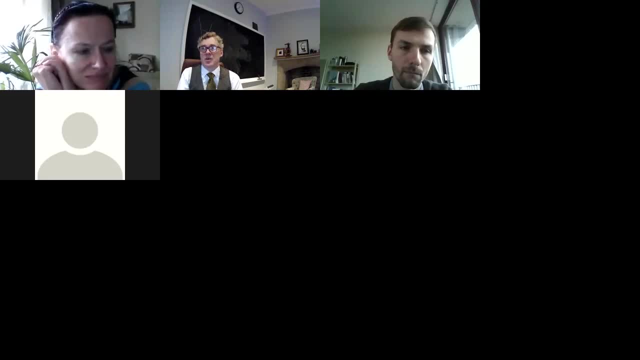 Then the consistency assertions about the existence of those large cardinals is an analog, a kind of shadow of the hierarchy over arithmetic. So that's one way of answering your question. is that Because if the large cardinal hierarchy is natural, then so are the consistency assertions? 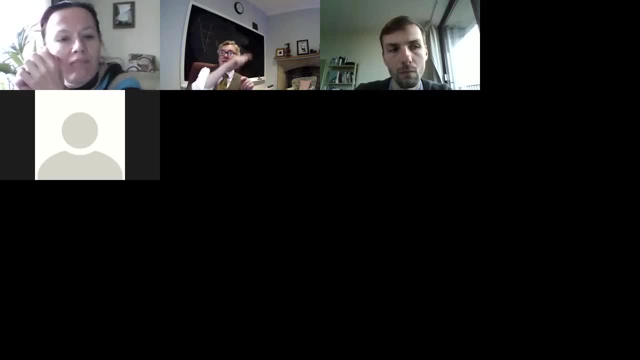 And those consistency assertions do form this consistency tower over piano arithmetic. So it's one way of answering. But other people object. So Steele, for example, has argued against that conception, saying: look, we don't want to replace the actual large cardinal hierarchy just with a consistency hierarchy. 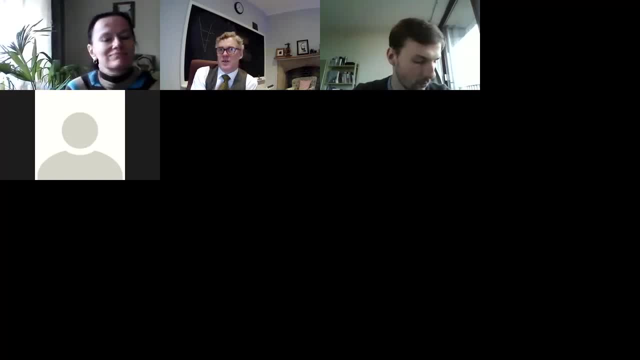 Because the, For example, the consequentialist justification of the large cardinal axioms, The fact that the large cardinals are giving us all these regularity consequences for definable sets of real numbers is evidence for the truth of the axioms, not just evidence for the consistency of the axioms. 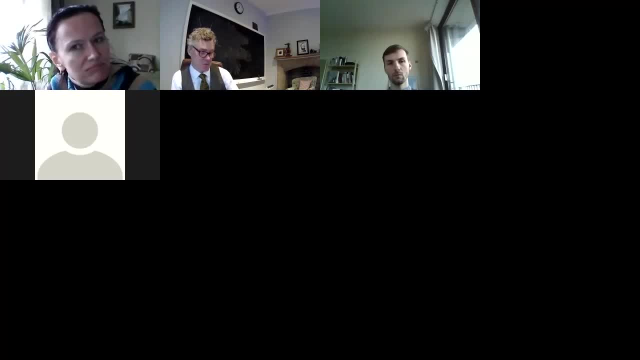 I mean, this is how Steele argues- that it's kind of, It's an instrumentalist dodge to replace the large cardinal assertion itself with the mere consistency assertion, that That those large cardinals exist, And so one should really think about it as a kind of a mere shadow of the real thing. 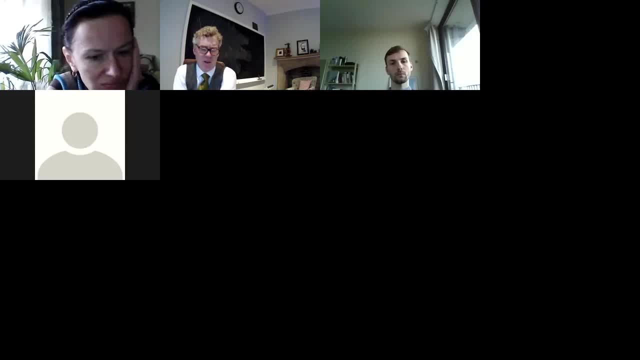 But it is taking place in arithmetic. Okay, But it's not clear whether that fully answers your question, Because you might have expected. look, I want a natural hierarchy of arithmetic, a genuinely arithmetic assertions, not just merely consistency assertions about set theoretic assertions. 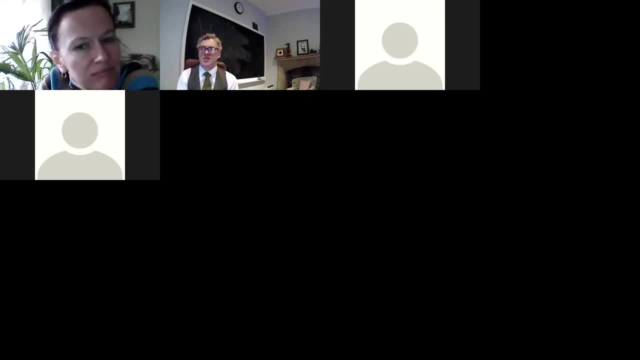 I want genuinely natural arithmetic assertions. I want natural arithmetic assertions that are forming this consistency, strength hierarchy, And there the situation is much less satisfactory. I mean, we have a few instances of it. We have, like Goodstein's theorem that I mentioned last time. 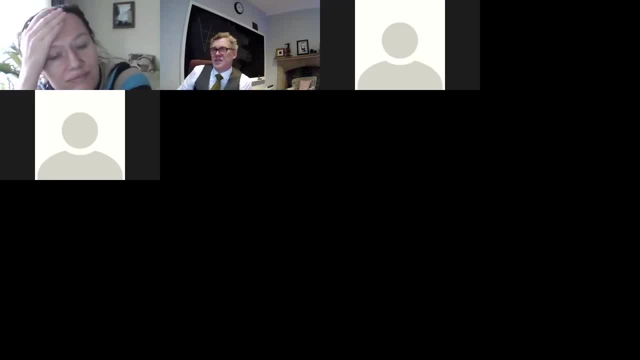 And there's other ones, And also there's sort of ordinal denotation systems. I mean the claim that this notation system is well ordered, or that one is well ordered, and so on. Those ones can give you sort of these hierarchies. 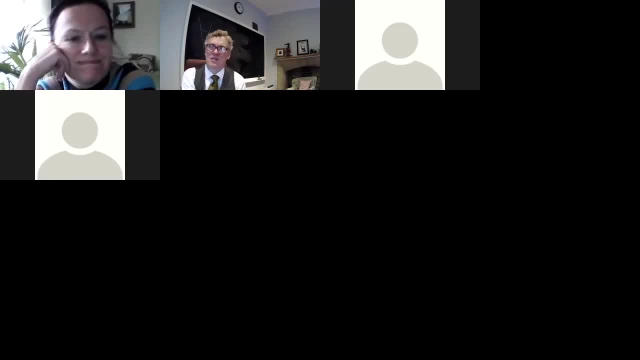 Over arithmetic And they would have this character A little bit of it, And so maybe that's the best kind of answer to make, But it's simply much less robust than it is in set theory. It's a great question. Any other questions? 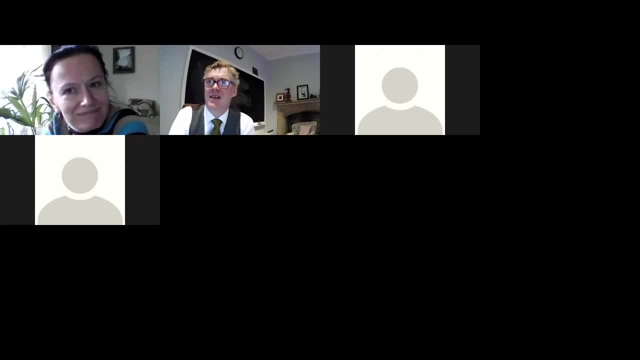 Let's see What will be future topics for the series. Today is the last lecture of the series. It's week eight And it's the term ending, So I'm sorry. Oh, someone asked when is the next lecture, But I'm sorry. 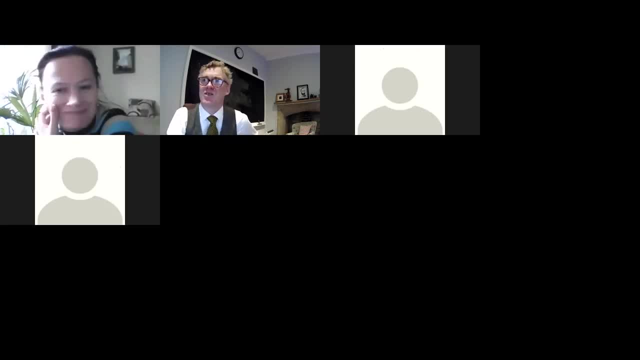 This is the last lecture And I'll put it on YouTube, So it's been a great term And thank you all so much for coming to the lectures And good luck in the future. Thank you so much, Professor. Thank you. It was a pleasure to have everyone.